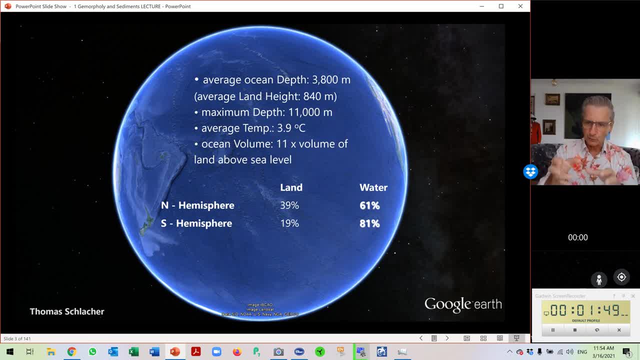 you would actually level the sea floor, so there is no deep sea trenches or no undersea mountains. everything is just flat. you actually get to about 4,000 meters plus minus, So the ocean is enormously deep. The average ocean depth is 4,000 meters. Most people don't actually know that It. 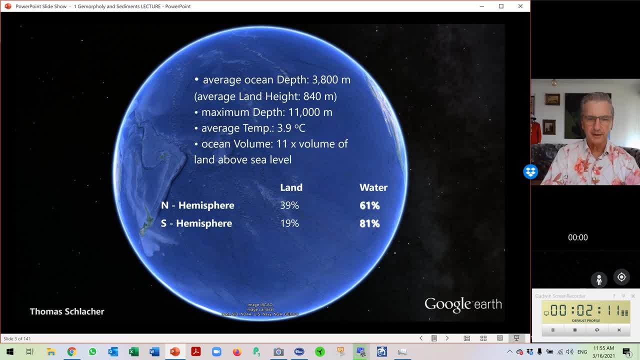 goes down deeper than Mount Everest, rises above the land And most of the global ocean is actually very cold. We are talking about roughly 4 degrees And if you measure the volume of water, well calculated of course, it is 11 times of all the land which 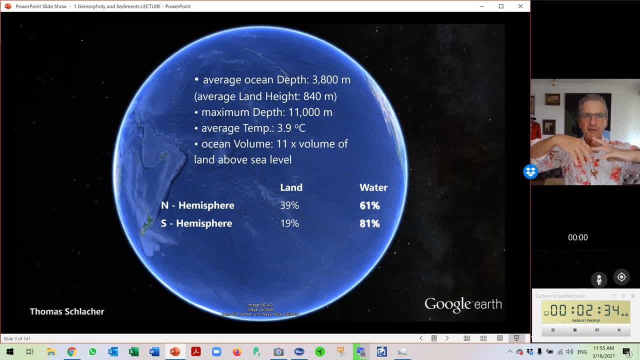 sticks above the sea surface. So we have a vastness, a voluminous, basically feature here on our planet and it is called the global ocean, And particularly so in the southern hemisphere, as this illustrates enormously nicely. So, basically, one-fifth is land and, you know, four-fifths is water. So we literally and truly live on the blue planet. 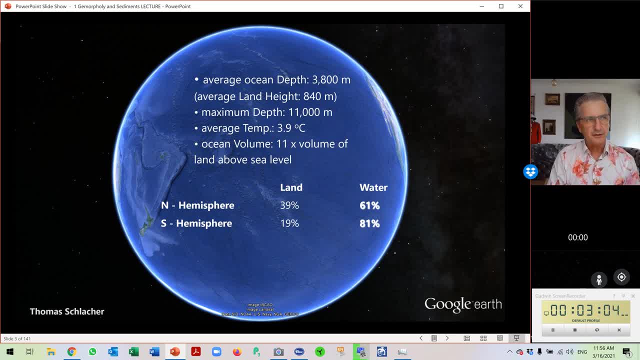 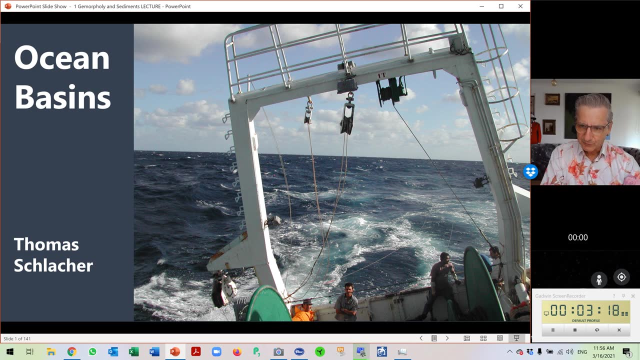 And it took humanity quite a long time to actually discover most of that, Because seafaring technologies were primitive for a very, very long time. Now, if you actually go back, if you go back here, this is one of my favorite shots, It's you know. 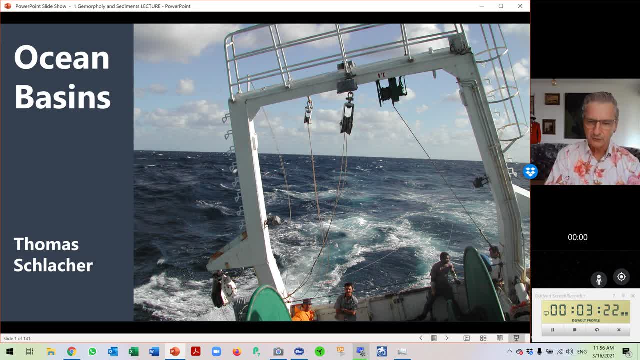 one of my favourite shots. It's, you know, one of my favourite shots. It's, you know, one of my favourite shots. It's, you know, you know, about 20 years old and it's taking a French research vessel down from New Caledonia. 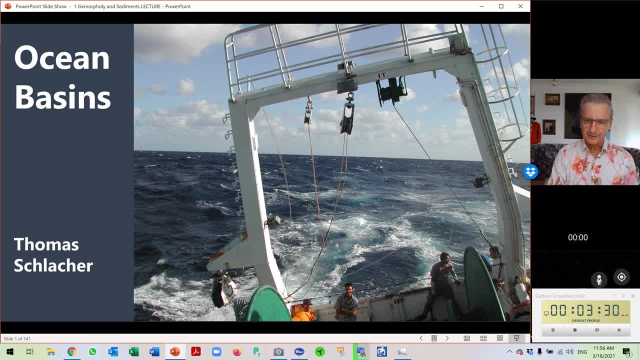 to New Zealand along the Norfolk Ridge. and you can see it's a fairly small boat and it pitches in rows. you know, except for me and Bertrand, all the other scientists couldn't actually go out because they were too seasick. so you see, the South Pacific island cruise. 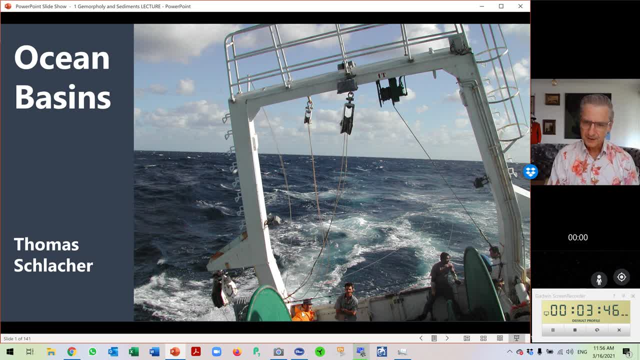 here and Jean-Luc and Philippe from France, and that image, you know, always reminds me of a very, very, you know, poignant sentence my friend Monty Bright, from Scotland, once, you know, pronounced at his conference. there was this question like what is the biggest technology technological advancement you have seen in your career? and people said, ah no. 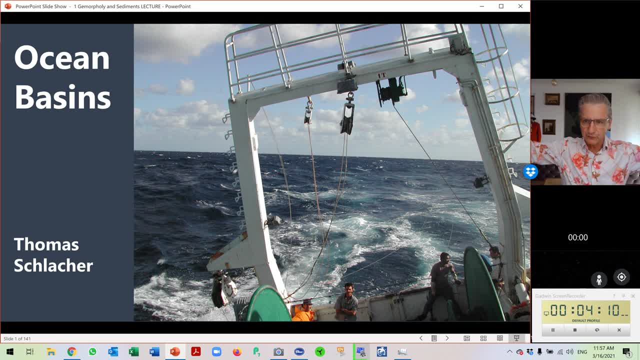 we got, you know, underwater robots and we got cameras and we got big ocean vessels and Monty said no, no, I don't think so. Actually I think it's GPS because for the first time about you know 30 years, we knew where we were. there was always a big problem going out on vessels for millennia and actually 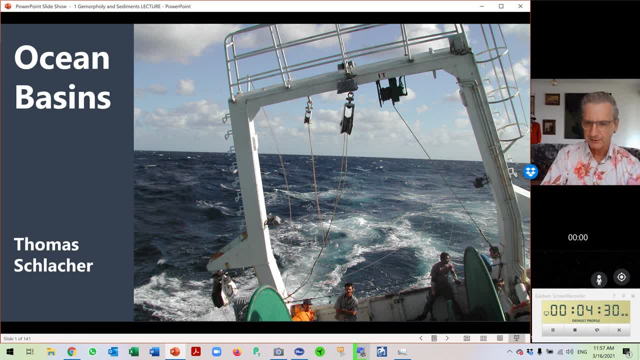 we once had a catastrophic electrical failure on the boat and the French sailors used a sextant. it was fascinating, so we navigated back from Hawaii using a sextant. never mind, we basically, as humanity, have a lot to learn, and we have a lot to learn, and we have a lot. 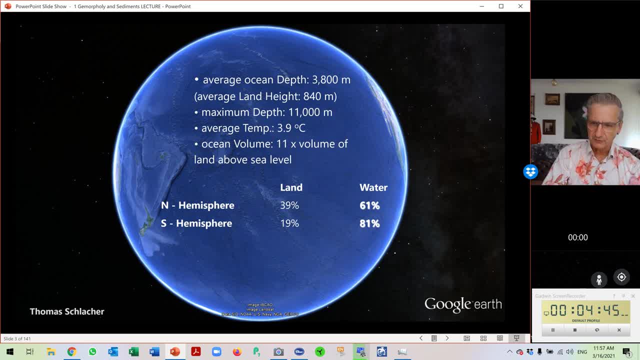 to learn and we have a lot of culture where we can truly understand the human species and say: you know, you know, it's a half mandarine, it's a half human. So in many ways, and it's a very difficult thing for us as Americans, because we actually 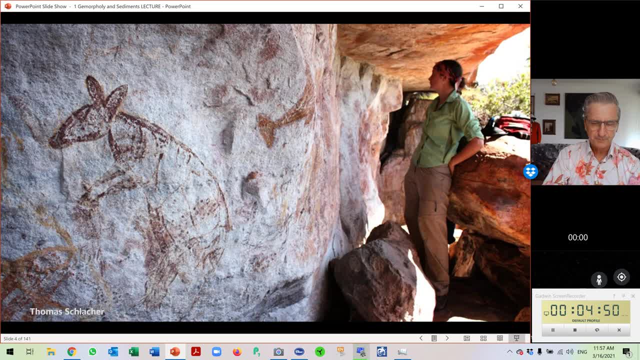 that's how we are as an individual. Humanity had a long association with the ocean, but it was actually a very difficult one, at least for you know, as Western cultures. When we actually talk about discovering things- and I want to be absolutely clear about that- it's a very weird concept and I think it's a completely wrong concept which we actually 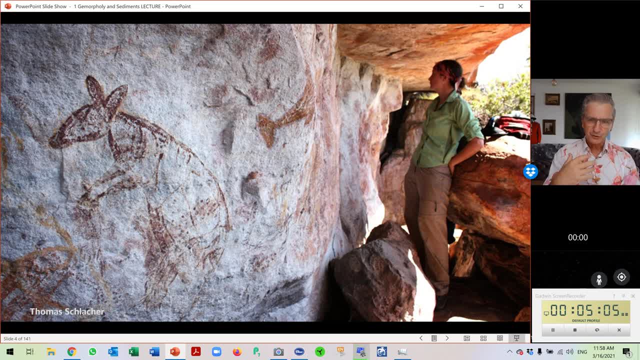 have embodied in Western culture. because what is actually quite odd, and few people think about it- Everywhere the right explorers, the White explorers, the Royal explorers, They literally just do it: Cook Flinders, you name them. they already made native people. They were actually there. 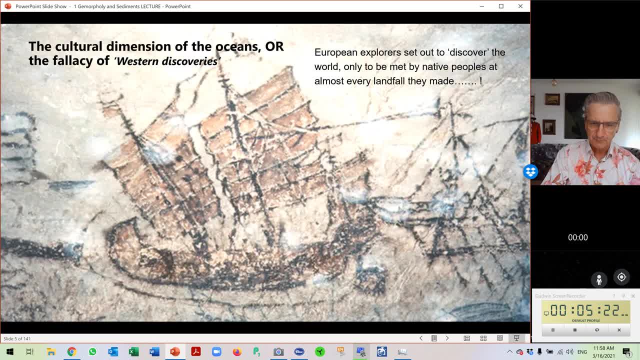 many, many thousands of years before them. And here we actually see a painting from North Arnhem Land in the top of Australia about possibly some Chinese chunks which basically came there a few hundred years ago, But the point is they were already there. 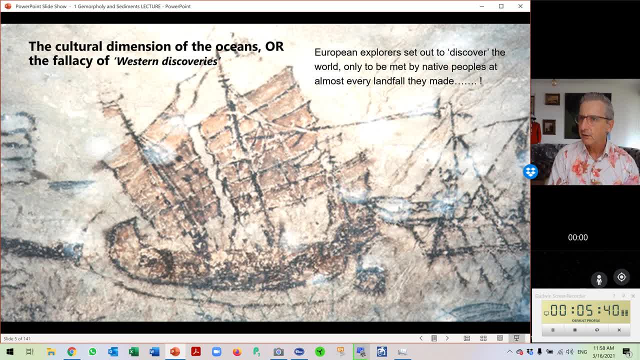 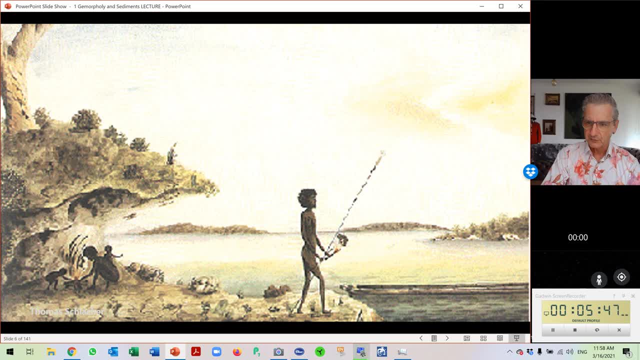 living there and literally caring for country and making a sustainable living from it, And pretty much the same thing happened in Australia. I mean, we all have statues of Captain Cook and stuff like this, But again, when they landed in Sydney Cove they were. 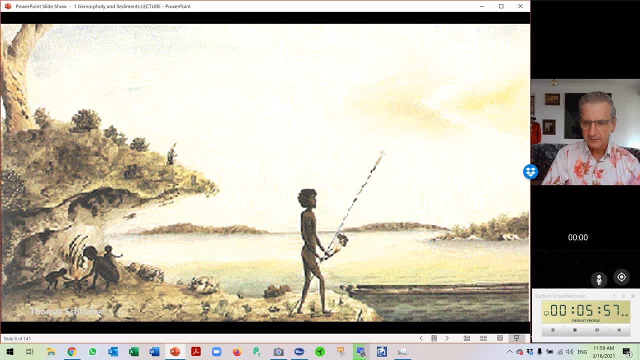 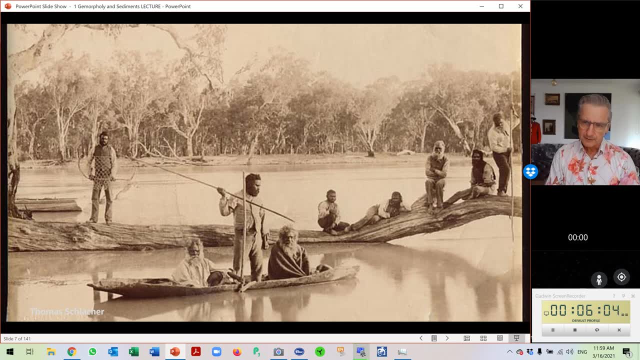 the indigenous people who probably came there at least 50,000 years before them And, of course, throughout colonization. you know we had a very, very mixed impact- you know, we have to be honest- and sometimes a very, very horrific one. So when we talk about ocean, 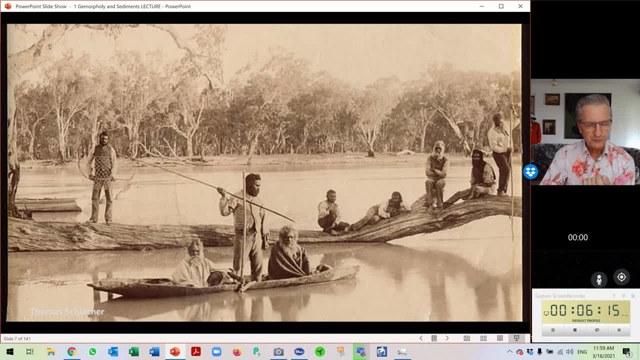 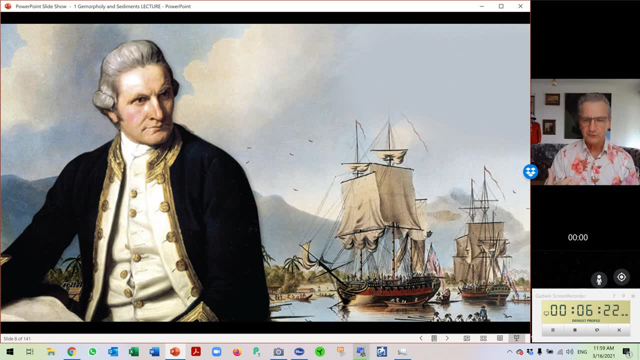 exploration and finding new features. be very, very careful that all of that is mostly framed in the context of a white, Anglo-Saxon, basically, culture. And we have this. you know very, very, you know dashing looking, Captain Cook. you know probably, you know thinking quite. 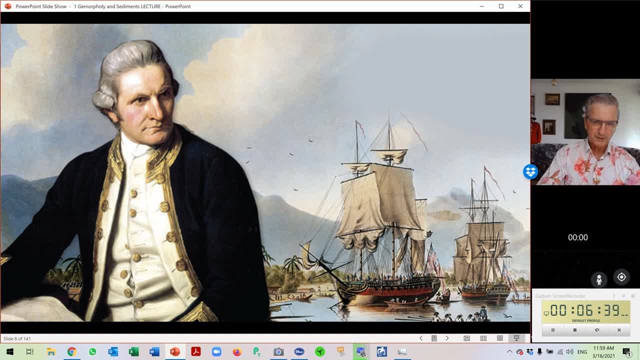 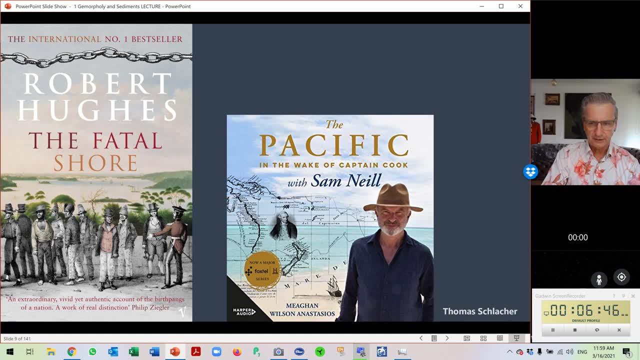 deeply about the next century. We're not talking about the next discovery or where he can get more room from, But be careful that this is a picture which actually is changing dramatically, and so it should. I urge all of you to actually read the book called The Fate of Shore And just about two. 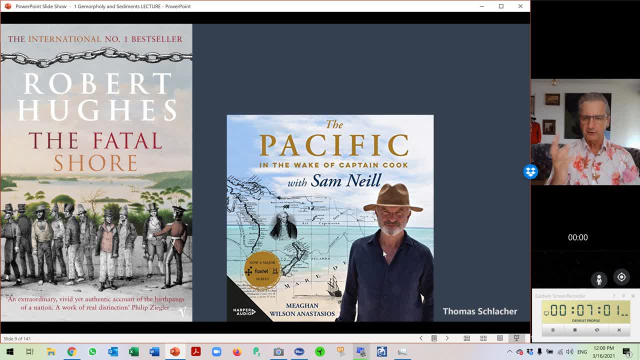 months ago or a month ago, Sam Neill. everybody has to love Sam Neill. if you're living in New Zealand or Australia, Yeah, And Sam Neill has a wonderful new series. you can watch it on SBS on demand, or you can buy the audio book, or you buy the book called In the Wake of James Cook in the Pacific. 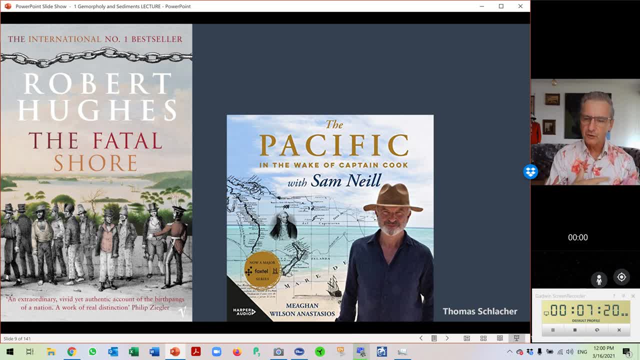 And it addresses in a very, very typically insightful, entertaining and yet very sensitive way what Sam Neill can bring to the story, those kind of issues of the Western cultural dominance of discoveries. So let's be just very, very careful about that. 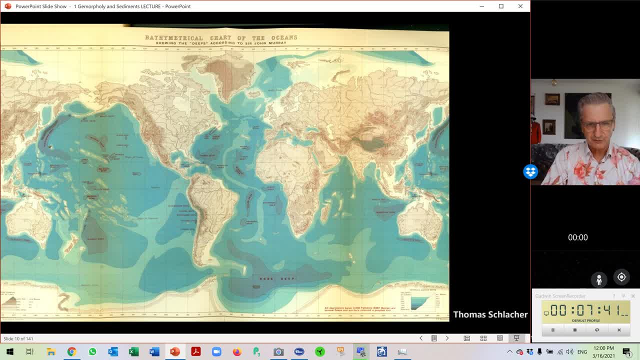 Now, and this is a chart of the ocean published about 50 years ago And very, very oddly- you would not believe it- it didn't really show terribly much. What it did show is like: yeah, there were, you know, a few very deep bits in the ocean. 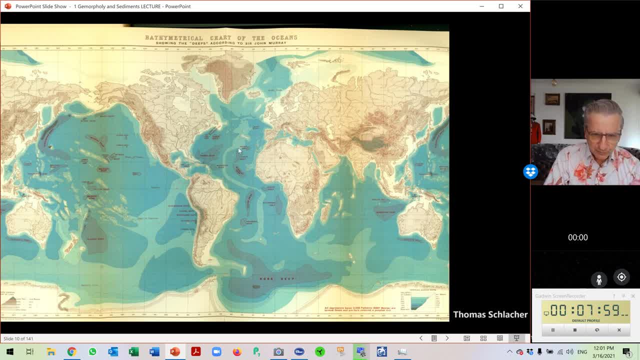 There were some very shallow ones, And look at this snaky bit going up right in the middle of the Atlantic. They knew most of, they knew all of the Pacific Islands by that. But then Most of it is colored in this just sort of general blue because basically we didn't know what was on the seabed. 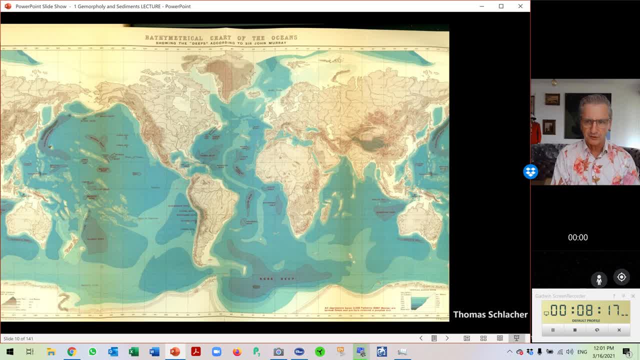 And I have to say, about 25 years ago I did my first deep sea project out of Fiji and I bought an Admiralty chart- We didn't have some at the time and it actually had a sounding here and then 100 miles over there from the Challenger Expedition and from some of Charles Darwin's records, because he basically, of course, went into the Pacific. 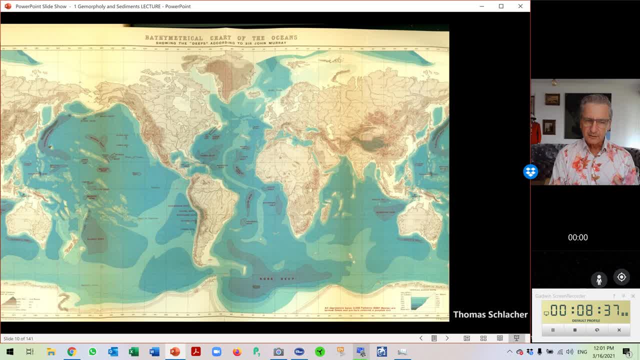 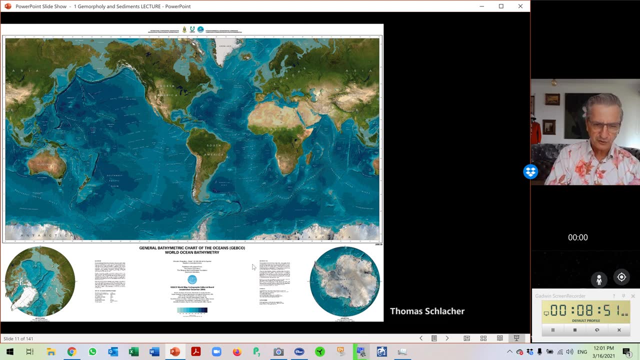 And in between there was just guesswork. So The exploration of the ocean floor is an enormously young endeavor. It's no different than exploring properly the surface of the moon. Nowadays you can go and download the General Batomatic Chart of the Oceans. 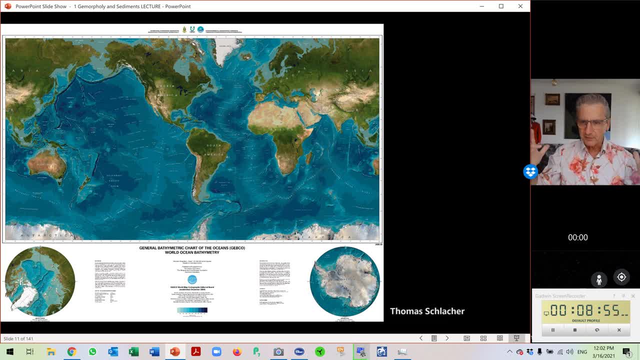 It's available for free and it comes down in a 20 megabyte file so you can print out a really, really big one if you wanted to. It is actually quite fascinating because we now can see that the ocean floor isn't flat. 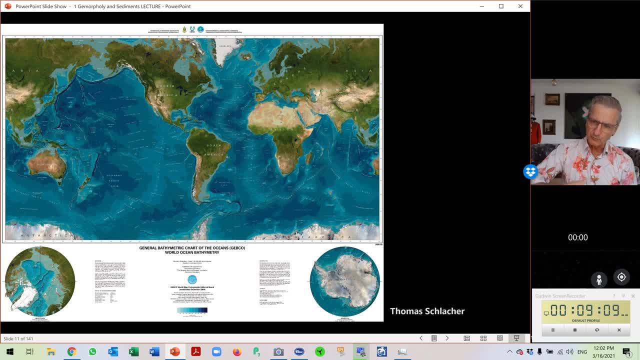 It is more variable. it got more rugged terrain, it got bigger mountains, it got bigger valleys than anything we have on land. So if you think the Himalayas are impressive- and they are impressive to our eyes- we got much bigger mountains, we got much longer mountain chains and we got much more coverage of really really incredibly diverse terrain in the oceans. 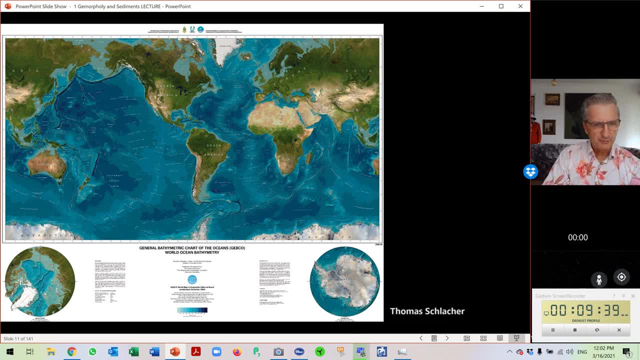 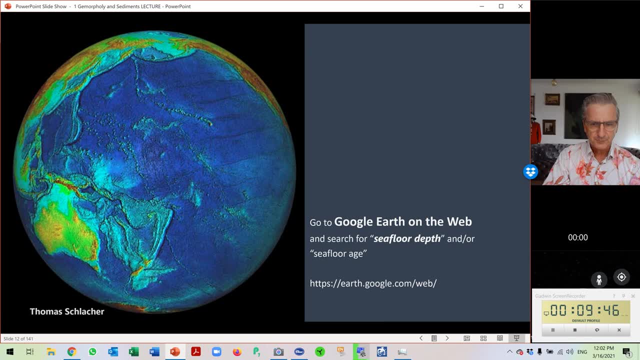 So that is to many people a little bit of a surprise, And this is only about. you know, 30 years ago was when we published that particular chart. So one thing I love you know. there's mixed feelings of course now about Google. 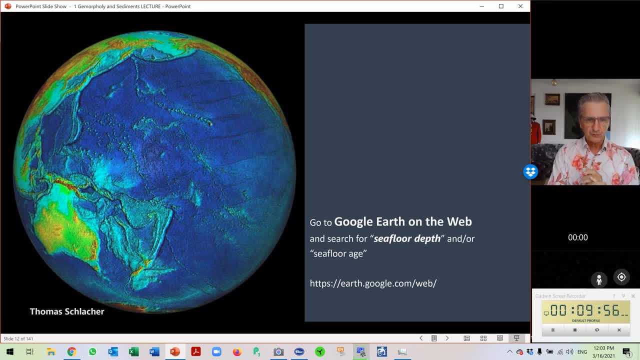 And I think we all have very strong opinions about that in Australia. Facebook and Google: you know dominance of the Internet and social media landscape, but that we did good things as well. You can go into Google Earth on the web and you can play around here. 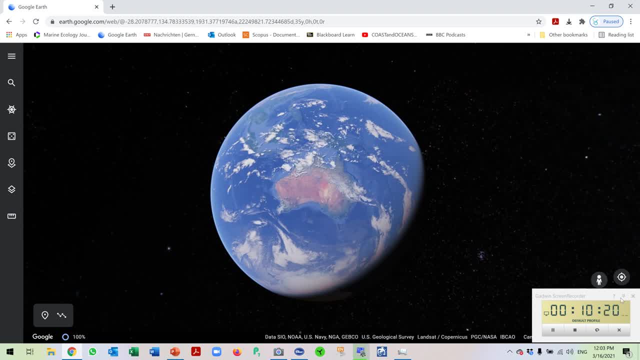 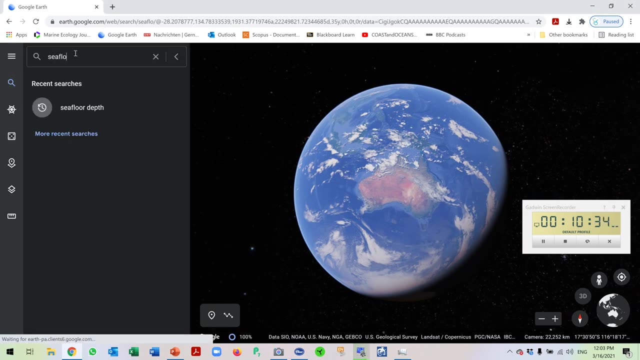 Oh, here's Australia, Let's go back. Go, Just get rid of this thing here. Get rid of this, And you can go in here and you type Sea floor depths and it actually takes you to know us in our most accurate model about the. 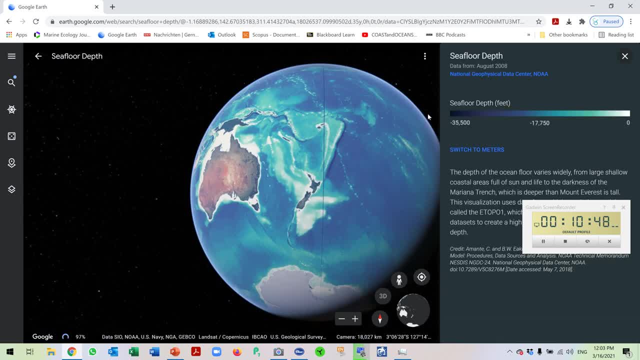 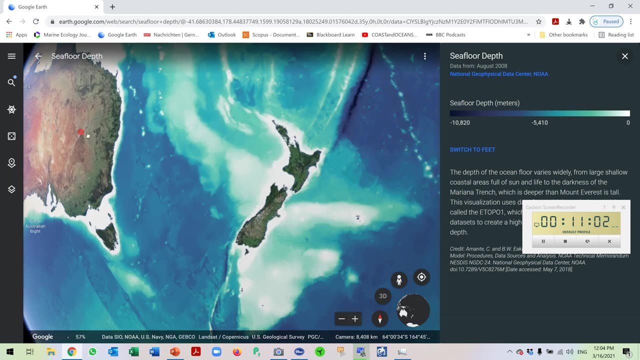 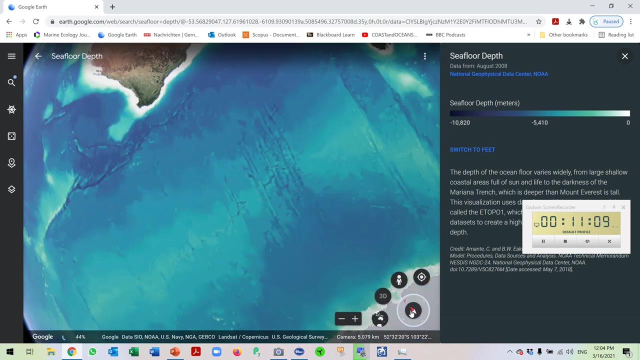 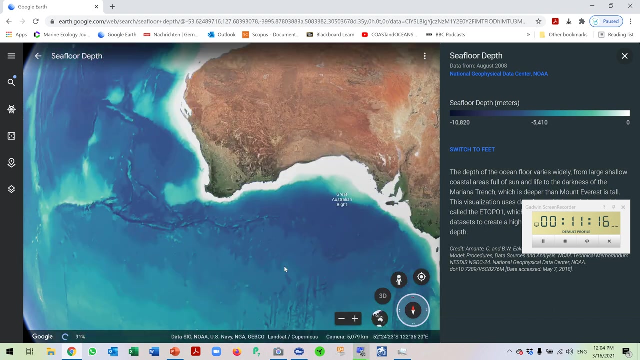 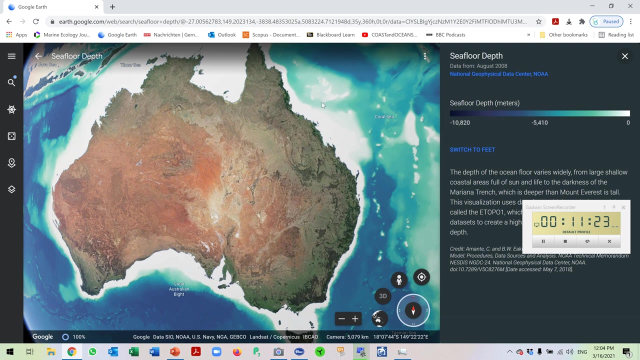 electromagnetic depth of the ocean and you can actually do the meters and we are not living in the 16th century anymore and if you actually look around here, just in our neighborhood, what you actually discover very quickly is: but what we see very quickly is we got a big continent and the continent actually has 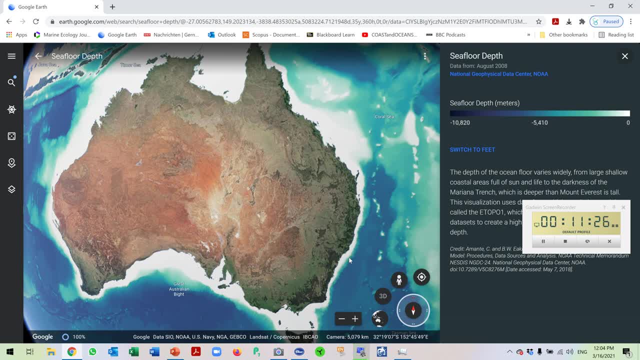 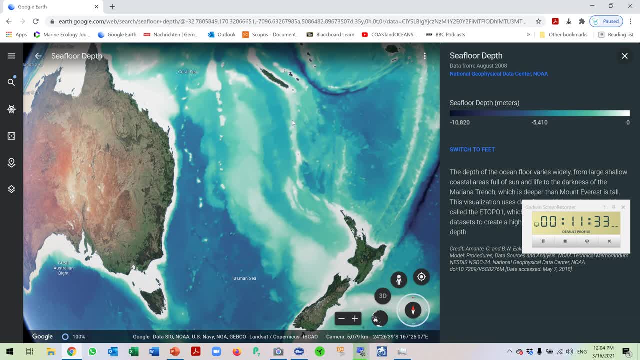 when we go over towards our neighbors. here we see New Caledonia sitting on a. here we see New Caledonia sitting on a. here we see New Caledonia sitting on a ridge, and as which actually extends all ridge and as which actually extends all. 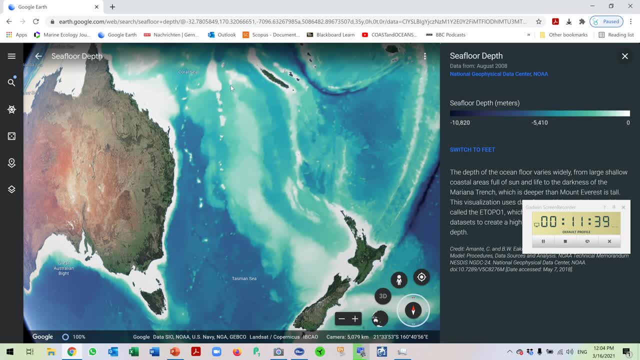 ridge and as, which actually extends all the way to New Zealand. we've got another the way to New Zealand. we've got another the way to New Zealand. we've got another ridge, here in the middle called the Lord ridge, here in the middle, called the Lord ridge, here in the middle called the Lord Howie Ridge. and then we got Siemens. 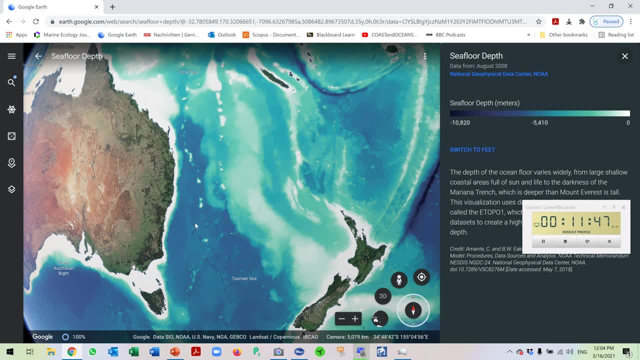 Howie Ridge, and then we got Siemens Howie Ridge, and then we got Siemens coming down here. we're gonna chain off coming down here. we're gonna chain off coming down here. we're gonna chain off white speckly things. so if you go a white speckly things, so if you go a 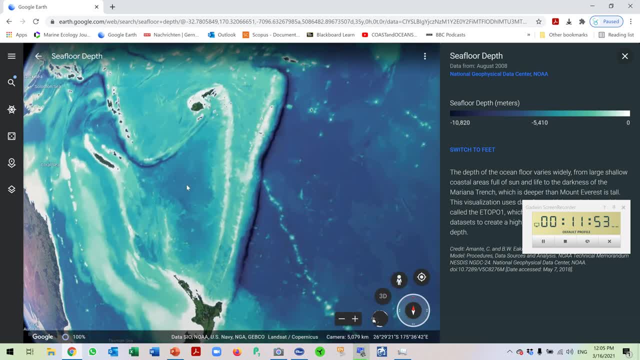 white speckly things. so if you go a little bit further over there, you see little bit further over there, you see little bit further over there, you see something very, very dramatic, and that is something very, very dramatic, and that is something very, very dramatic, and that is those are. this is when one or two and 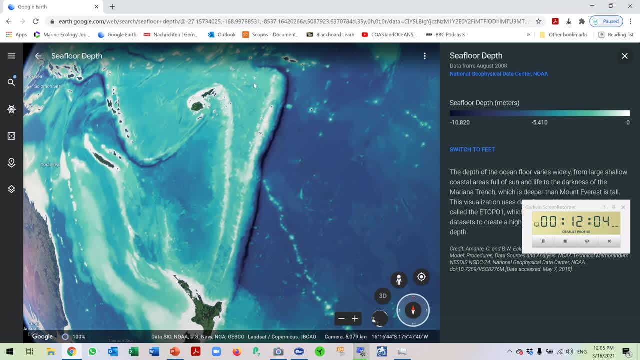 those are: this is when one or two, and those are this is when one or two. and this is two big islands of Fiji and you, this is two big islands of Fiji, and you, this is two big islands of Fiji, and you go over to Tonga and you sail out a. 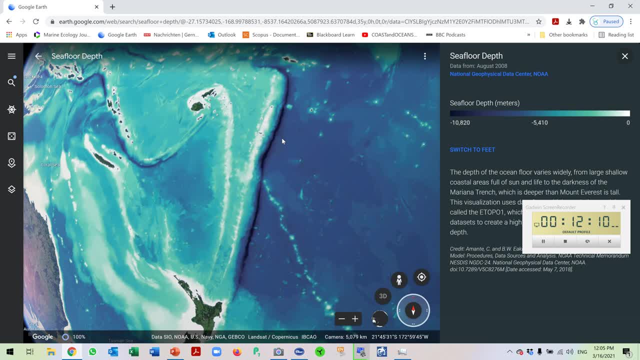 go over to Tonga and you sail out a go over to Tonga and you sail out a little bit there and then actually the little bit there, and then actually the little bit there, and then actually the ocean plunges down to about you know, ocean plunges down to about you know. 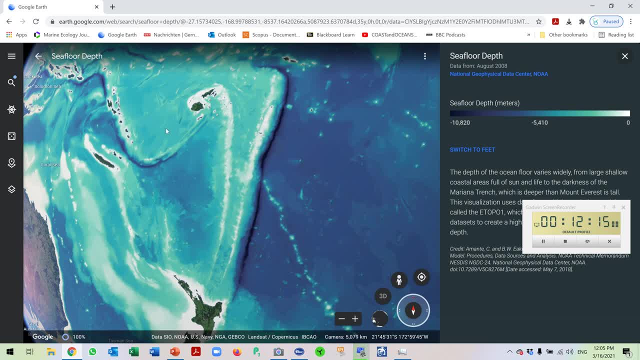 ocean plunges down to about, you know, 10,000 meters in the Kermadec trench and 10,000 meters in the Kermadec trench and 10,000 meters in the Kermadec trench and you can go around the world now. 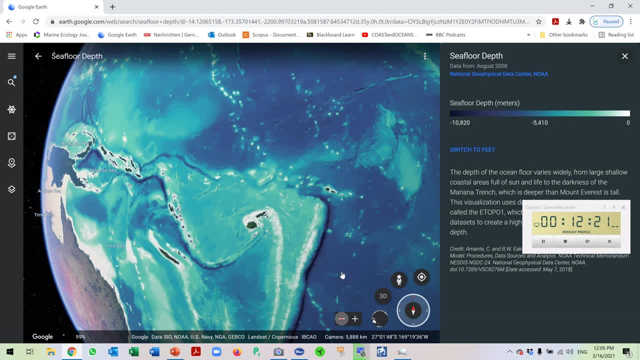 you can go around the world now. you can go around the world now exploring the sea floor, exploring the sea floor, exploring the sea floor from the comfort of, from the comfort of, from the comfort of your home armchair, traveling whatever you, your home armchair traveling whatever you. 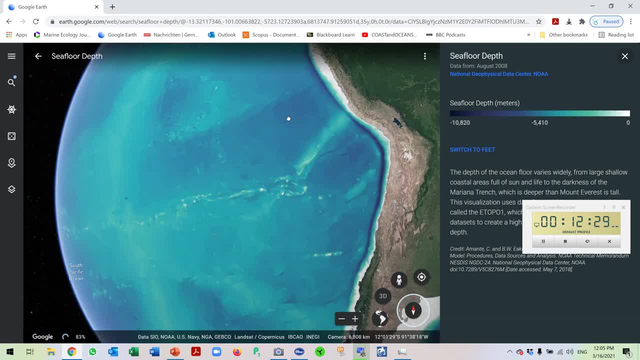 your home armchair, traveling, whatever you want to actually call that, want to actually call that, want to actually call that, and immediately you'll actually notice and immediately you'll actually notice and immediately you'll actually notice. is that, whoa hey, look at South America. is that whoa hey, look at South America. 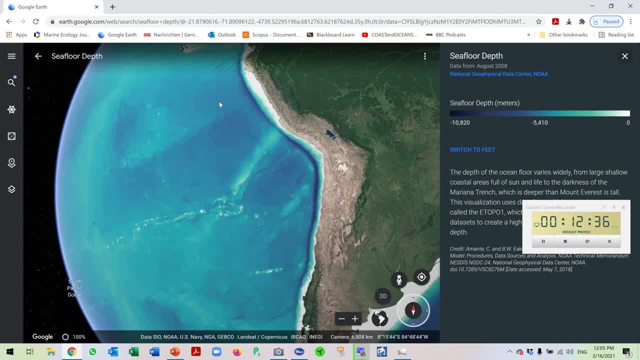 is that whoa? hey, look at South America. and I was so lucky that we just managed, and I was so lucky that we just managed, and I was so lucky that we just managed to get to, to, to uh chile just before that, uh chile, just before that. 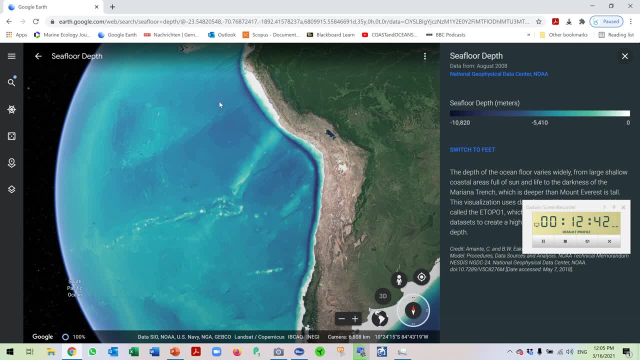 uh chile. just before that, kovit had really uh properly. we took. kovit had really uh properly, we took. kovit had really uh properly. we took the second last plane out of Santiago, the second last plane out of Santiago, the second last plane out of Santiago. and if you ever wonder why they have so, 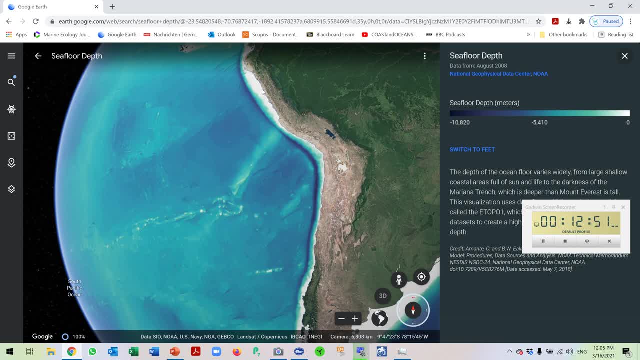 and if you ever wonder why they have so, and if you ever wonder why they have so many earthquakes in chile. look at this: many earthquakes in chile. look at this many earthquakes in chile. look at this. there's the coast and there's a little. 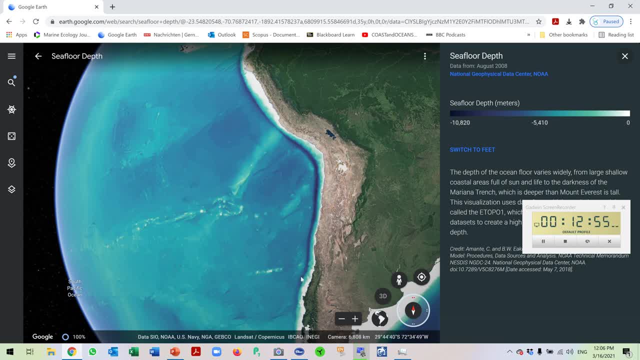 there's the coast and there's a little. there's the coast and there's a little bit of a continental shaft and an bit of a continental shaft and an bit of a continental shaft and an enormously big, enormously big, enormously big, big, 8 000 meter trench hugging the. 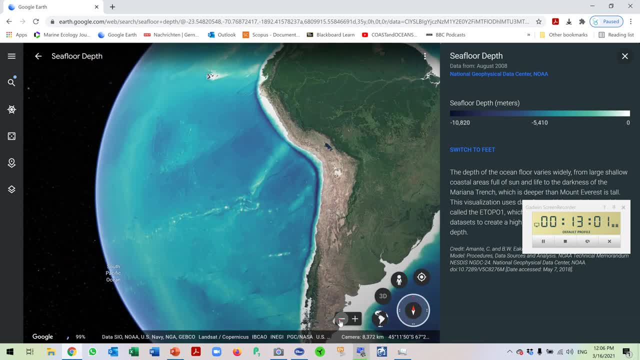 big 8 000 meter trench hugging the big 8 000 meter trench hugging the coastline, coastline, coastline. so so, so, basically, it doesn't matter where you go. basically it doesn't matter where you go, basically it doesn't matter where you go around the world and look at this weird. 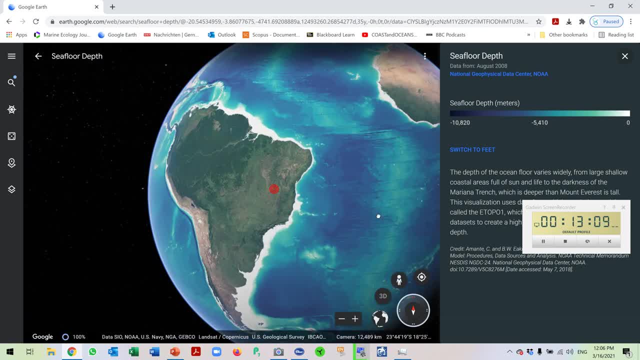 around the world and look at this weird around the world and look at this weird thing, thing, thing. there's africa, there's south america. if there's africa, there's south america. if there's africa, there's south america. if we go, we go, we go like here: 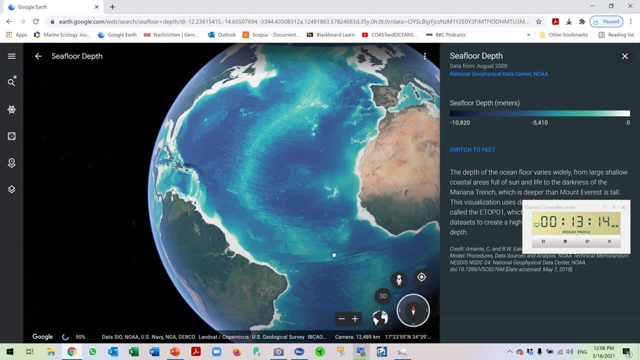 like here. like here, there's this huge, huge, long mountain. there's this huge, huge, long mountain. there's this huge, huge, long mountain range right going up all the way, all the range, right going up all the way, all the range, right going up all the way, all the way past the canary into our saw. 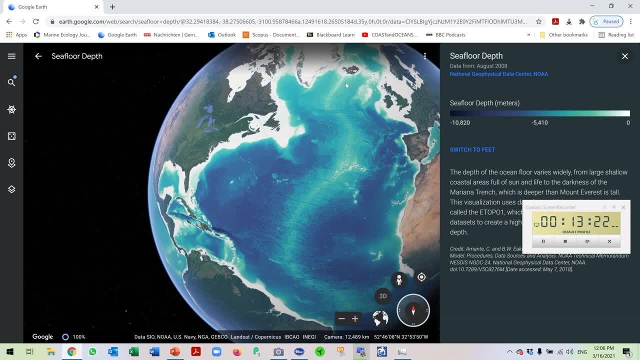 way past the canary into our saw, way past the canary into our saw islands. that's what i saw is a wonderful islands. that's what i saw is a wonderful islands. that's what i saw is a wonderful place to go, place to go, place to go, and then you get shallow and it actually 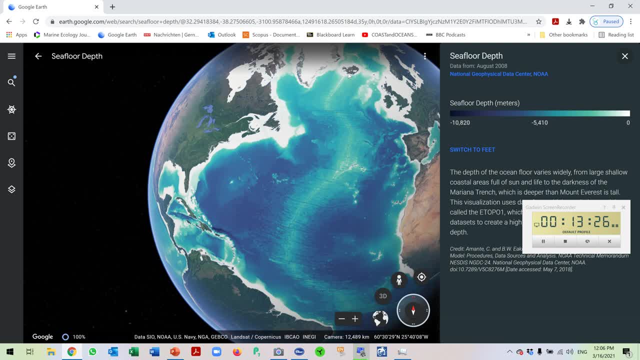 and then you get shallow and it actually. and then you get shallow and it actually pops out in iceland, pops out in iceland, pops out in iceland. so the ocean floor has features which we so. the ocean floor has features which we so. the ocean floor has features which we cannot even imagine sitting on land. 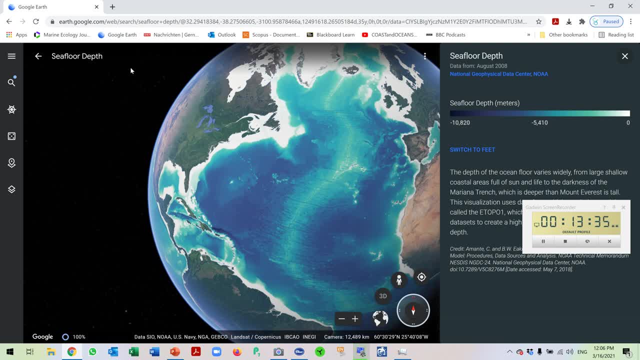 cannot even imagine sitting on land. cannot even imagine sitting on land until we had this kind of technology, until we had this kind of technology, until we had this kind of technology. looking at maps is fun, but this is looking at maps is fun, but this is looking at maps is fun, but this is much funner. so 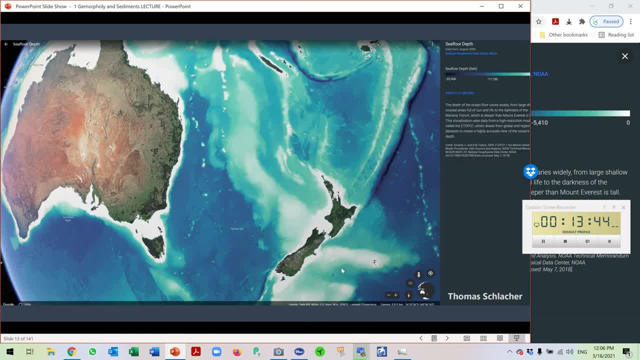 much funner, so much funner. so one thing you actually have to ask, one thing you actually have to ask, one thing you actually have to ask yourself then is yourself, then is yourself, then is having those incredibly vast basins, having those incredibly vast basins, having those incredibly vast basins we call basically 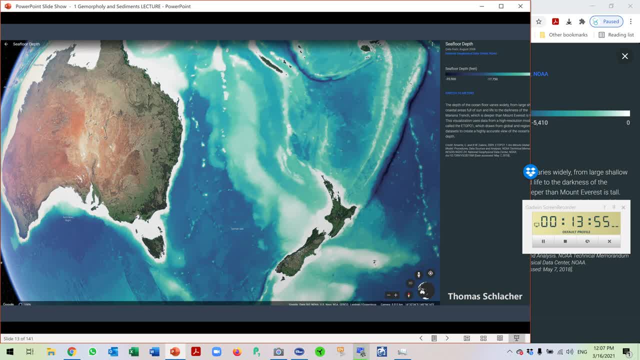 we call basically. we call basically the vessel in which you know if you want, the vessel in which you know if you want, the vessel in which you know, if you want to the water, the ocean water sits an to the water. the ocean water sits an to the water. the ocean water sits an ocean basin. 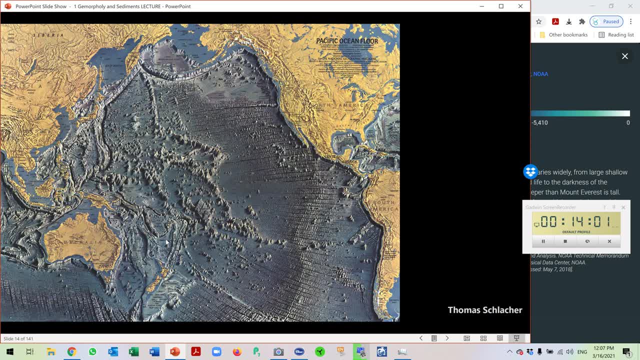 ocean basin, ocean basin, and it actually which has this and it actually which has this and it actually which has this. you know, you know, you know. amazing as flamboyant i would say it's amazing as flamboyant, i would say it's amazing as flamboyant, i would say it's flamboyant. geology. 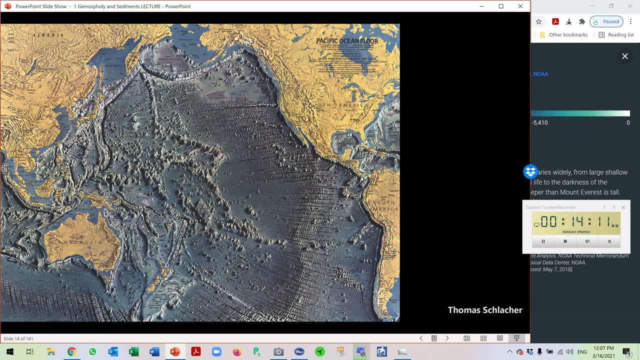 flamboyant geology, flamboyant geology, and you have to ask yourself: how did it? and you have to ask yourself: how did it? and you have to ask yourself: how did it actually come to that? what created the? actually come to that. what created the? 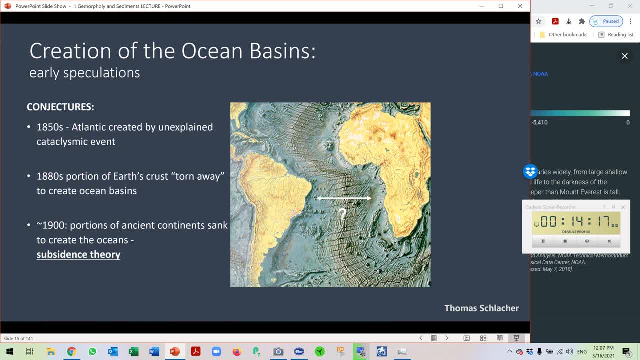 actually come to that. what created the ocean basins, ocean basins, ocean basins- and that's a curious question, and that's a curious question, and that's a curious question. uh, uh, uh, i have disappeared. oh, that's a bit you. i have disappeared. oh, that's a bit you. 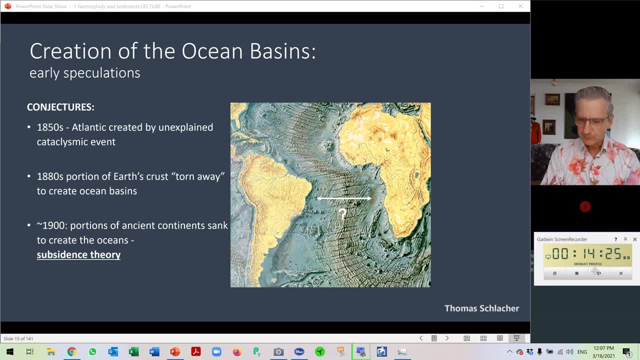 i have disappeared. oh, that's a bit, you know, let's do it that way, right, know, let's do it that way, right know, let's do it that way, right because? because, because think about it, uh, it's not. because think about it, uh, it's not an entirely trivial question nowadays. we 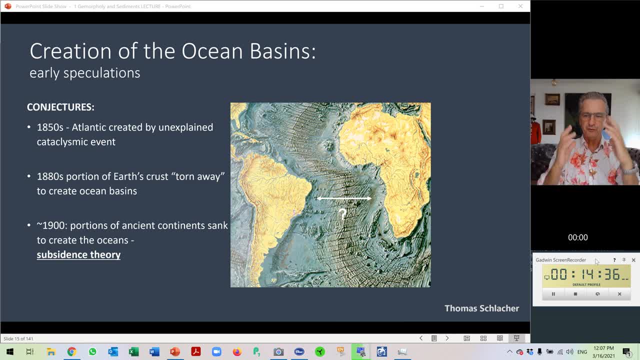 an entirely trivial question nowadays we. an entirely trivial question nowadays we. you know we used to be able to fly. you know we used to be able to fly. you know we used to be able to fly anywhere. we want to do in a very short anywhere we want to do in a very short. 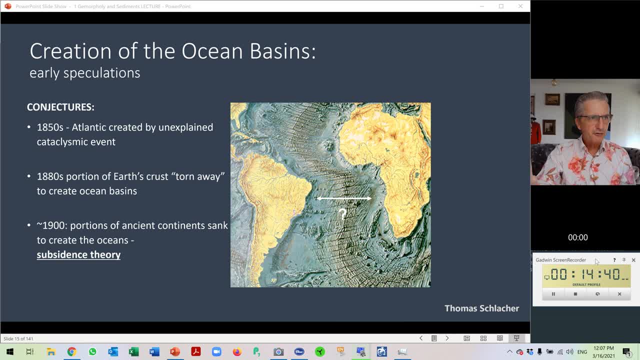 anywhere. we want to do, in a very short period of time, where, if you're speaking, period of time, where, if you're speaking, period of time where, if you're speaking, and if you fly from australia, and if you fly from australia and if you fly from australia to 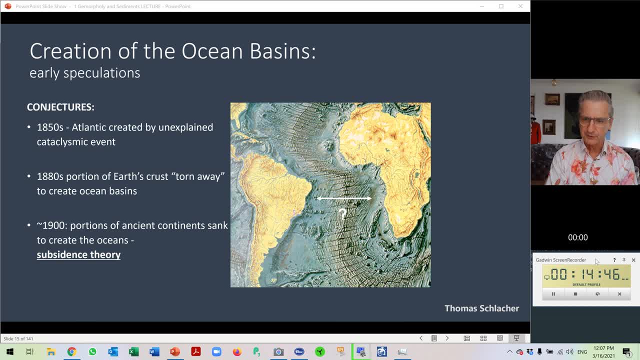 to to los angeles. you have 12 hours of blue los angeles. you have 12 hours of blue los angeles. you have 12 hours of blue underneath you, underneath you, underneath you. if you fly from, let's say buenos aires. if you fly from, let's say buenos aires. 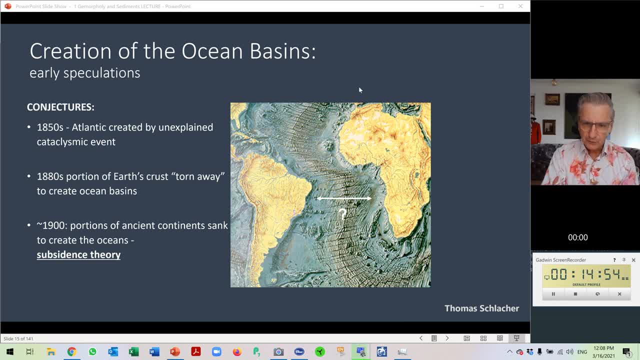 if you fly from, let's say, buenos aires, which is here highly recommended to go, which is here highly recommended to go, which is here highly recommended- to go over here to london, it takes about 10 over here to london. it takes about 10 over here to london. it takes about 10 hours and we look down and it's also 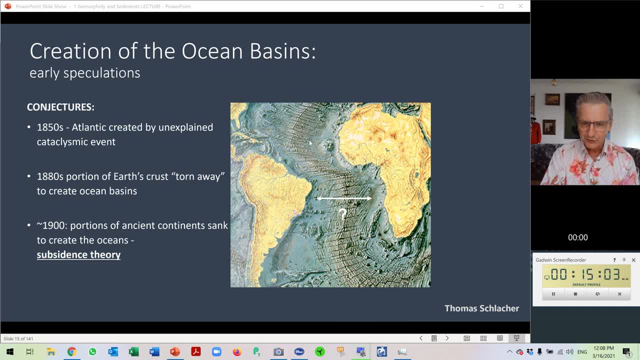 hours and we look down and it's also hours and we look down and it's also blue ocean, 90 of the time. blue ocean, 90 of the time. blue ocean, 90 of the time. except this is actually a very cool, except this is actually a very cool. 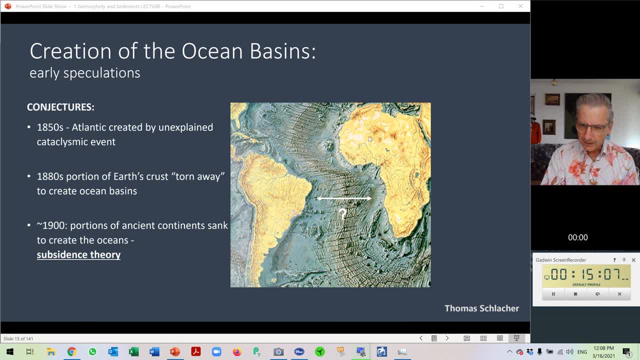 except this is actually a very cool flight because it goes over the sahara flight, because it goes over the sahara flight, because it goes over the sahara desert to come in here and on a desert to come in here and on a desert to come in here and on a on a on a nice morning flying, you know. 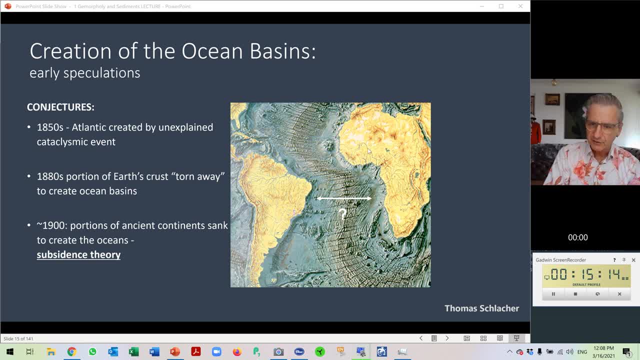 on a nice morning flying. you know on a nice morning flying. you know along the. you know crossing the coast along the. you know crossing the coast along the. you know crossing the coast here and then getting within like 20 here and then getting within like 20. 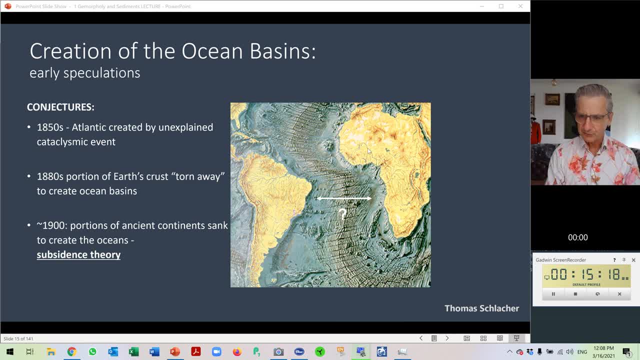 here and then getting within like 20 minutes, into minutes, into minutes, into major, major big sand dunes with little, major major big sand dunes with little, major major big sand dunes with little dust storms coming off, dust storms coming off, dust storms coming off. that's, you know, being a scientist, it's. 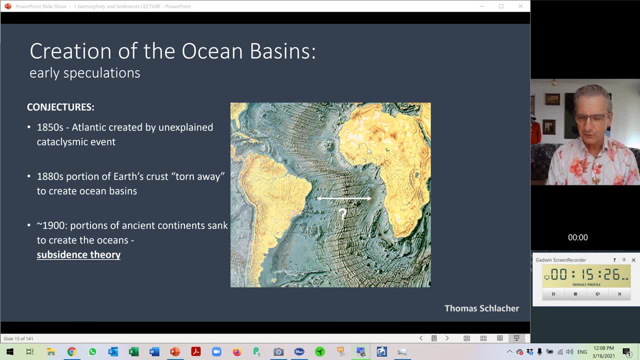 that's you know being a scientist. it's that's you know being a scientist. it's really fun being on planes. really fun being on planes. really fun being on planes. always gotta sit and look down. always gotta sit and look down, always gotta sit and look down. so uh, 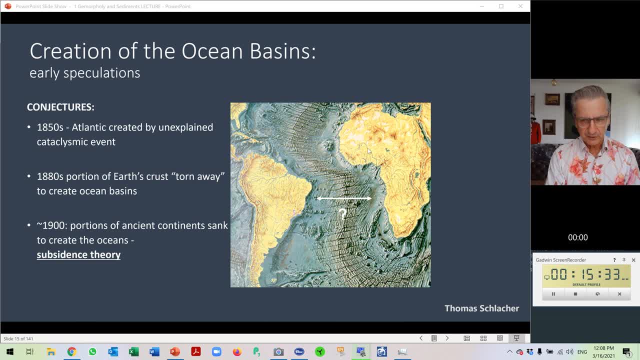 so, uh, so, uh, people just basically didn't have any idea. people just basically didn't have any idea. people just basically didn't have any idea. some cataclysmic event, some cataclysmic event, some cataclysmic event, and it followed the idea, the idea. 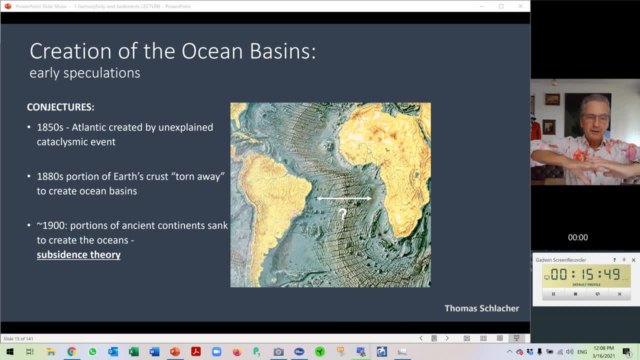 and it followed the idea, the idea, and it followed the idea. the idea followed from. that is like: well, what followed from that is like: well, what followed from that is like: well, what actually happened. is everything was land actually happened? is everything was land actually happened? is everything was land, and then bits and pieces flew off into 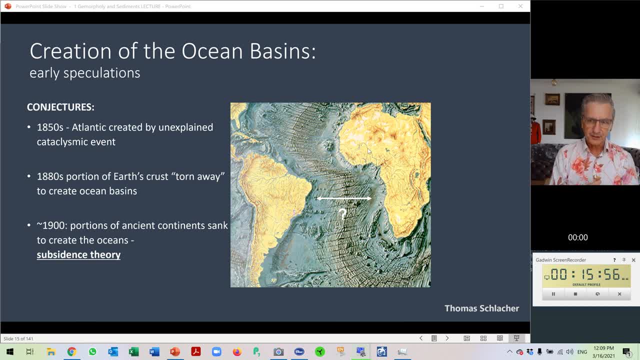 and then bits and pieces flew off into, and then bits and pieces flew off into space, space, space. now that's a fairly interesting theory. now that's a fairly interesting theory. now, that's a fairly interesting theory. but that's what it was. but that's what it was. 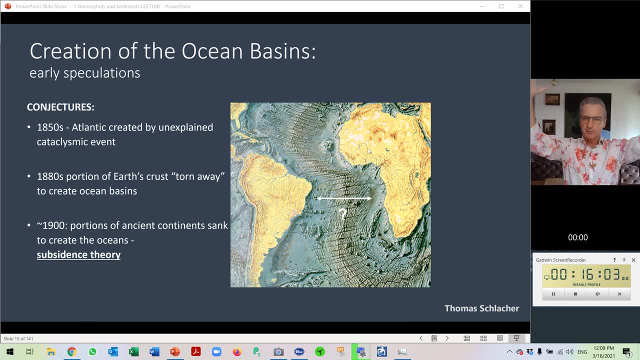 but that's what it was. and then people said no, it didn't. and then people said no, it didn't. and then people said no, it didn't actually fly into space. it didn't actually fly into space. it didn't actually fly into space, it didn't disappear. 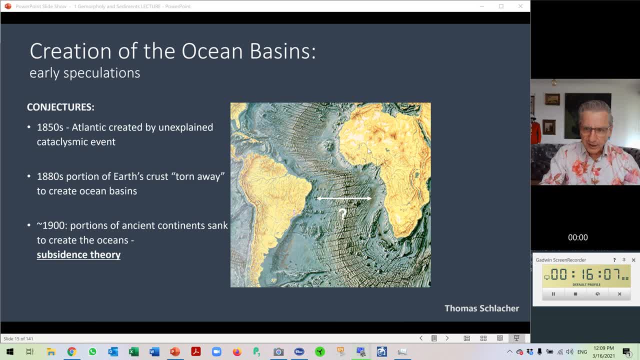 disappear, disappear, like sort of rock from the sun. he like sort of rock from the sun, he like sort of rock from the sun. he basically sank, basically sank, basically sank. below the current sea level, below the current sea level, below the current sea level. now, none of those theories had any any. 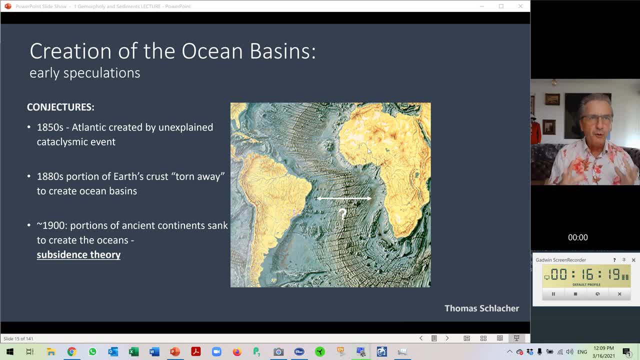 now, none of those theories had any any. now, none of those theories had any any. evidence but evidence, but evidence. but that's what we believe because we had. that's what we believe because we had. that's what we believe because we had no idea, zero idea of how it works. 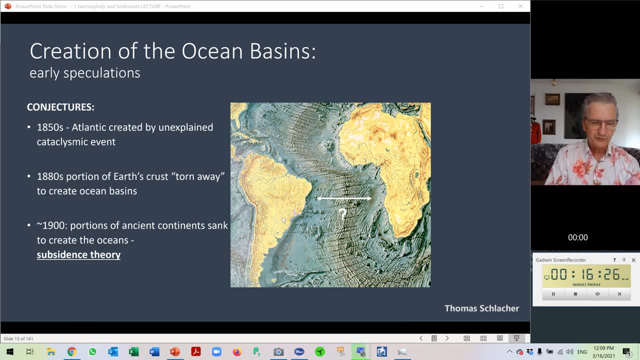 no idea, zero idea of how it works. no idea, zero idea of how it works. and people are still going off, and, and people are still going off, and, and people are still going off and actually looking for the lost continent, actually looking for the lost continent, actually looking for the lost continent atlantis, because it sank into the 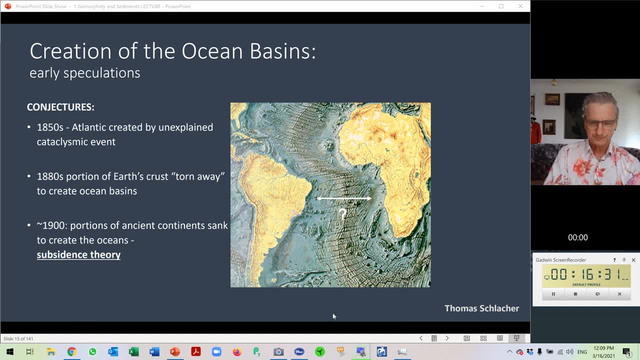 atlantis, because it sank into the atlantis, because it sank into the atlantic, that kind of stuff, atlantic, that kind of stuff, atlantic, that kind of stuff. now then we have to enter, now then we have to enter, now then we have to enter. oops, why doesn't this go? 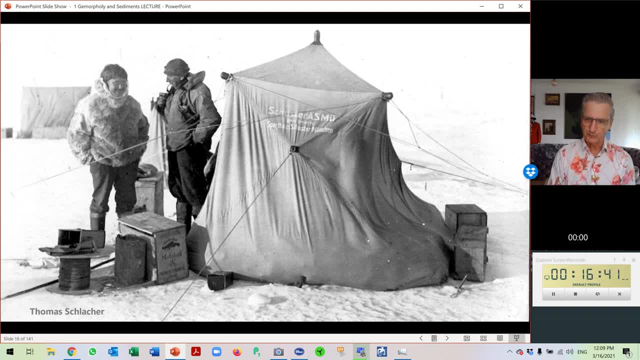 oops, why doesn't this go? oops, why doesn't this go? come on, come on, come on. so, uh, all good scientists really should. so, uh, all good scientists really should. so, uh, all good scientists really should look like this, or that's what they look. look like this, or that's what they look. 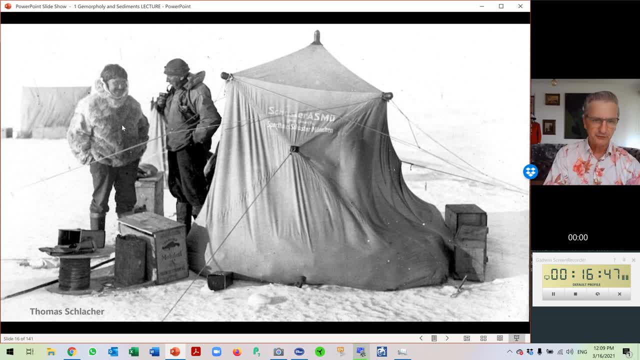 look like this, or that's what they look like, you know in the like. you know in the like. you know in the early 1900s. you know standing here, you, early 1900s. you know standing here, you, early 1900s. you know standing here. you know it's a big, you know. 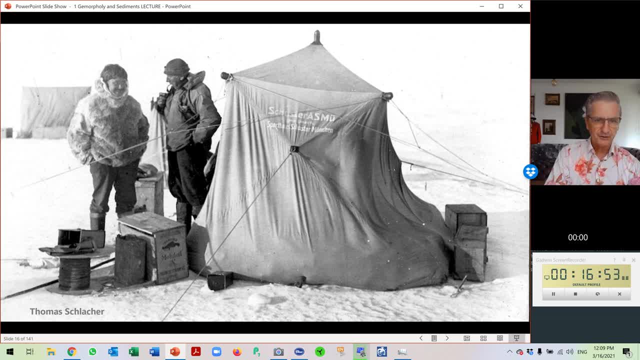 know it's a big. you know, know it's a big. you know barbie bowler bear, barbie bowler bear, barbie bowler bear. you know parker, and of course you can. you know parker, and of course you can. you know parker, and of course you can always smoke a pot and have a cap on, and 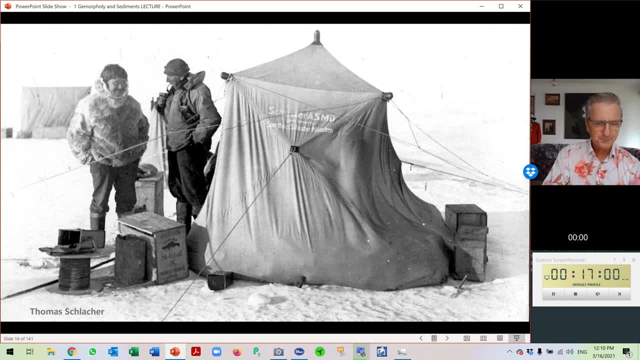 always smoke a pot and have a cap on and always smoke a pot and have a cap on and you know sleeping a tent at minus 40. you know sleeping a tent at minus 40. you know sleeping a tent at minus 40, that kind of stuff. 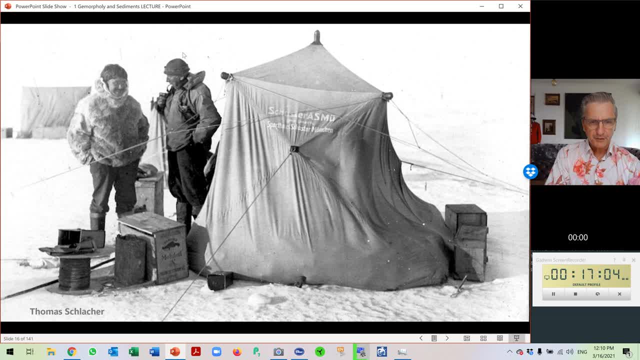 that kind of stuff. that kind of stuff. but this chap, here he is. but this chap here he is. but this chap here. he is an austrian professor of what used to an austrian professor, of what used to an austrian professor of what used to be of meteorology, and his name was. 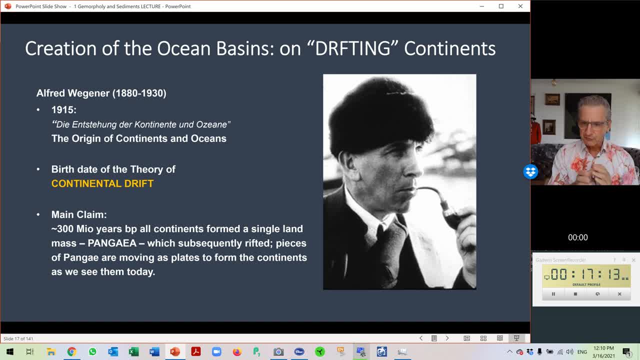 be of meteorology and his name was be of meteorology and his name was alfred wegener and he wrote a book in alfred wegener and he wrote a book in alfred wegener and he wrote a book in 1915, in the middle of the first world. 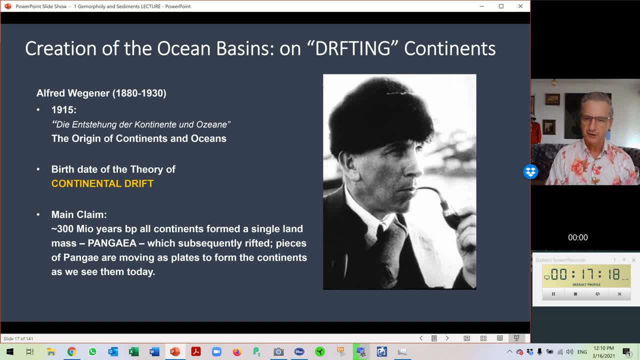 1915, in the middle of the first world, 1915, in the middle of the first world war, called war, called war, called the engineering the continent on the, the engineering, the continent on the, the engineering, the continent on the ocean basically means the origin. ocean basically means the origin. 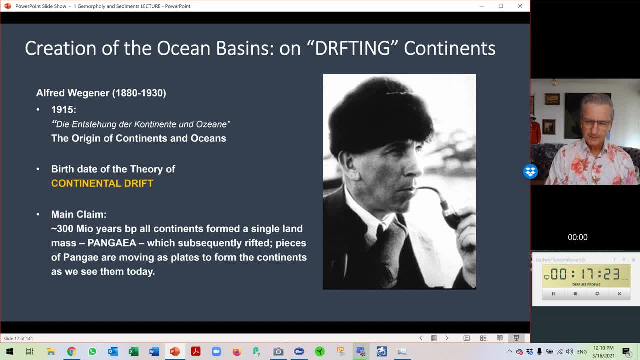 ocean basically means the origin or the development of the continents and or the development of the continents and or the development of the continents and oceans, oceans, oceans, and he basically come up with some crazy and he basically come up with some crazy and he basically come up with some crazy idea called continental drift and he 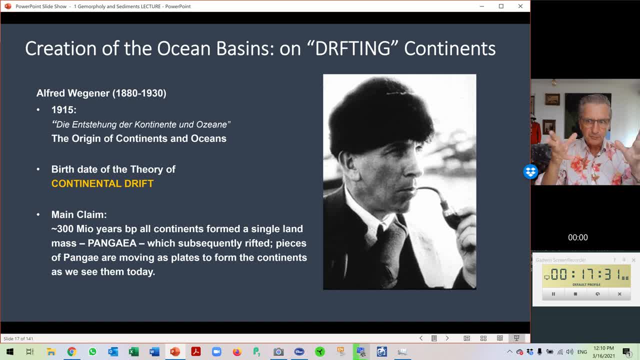 idea called continental drift and he idea called continental drift and he basically said: look how it actually basically said, look how it actually basically said: look how it actually worked, was, worked, was, worked, was in the beginning. there wasn't god you in the beginning, there wasn't god you. 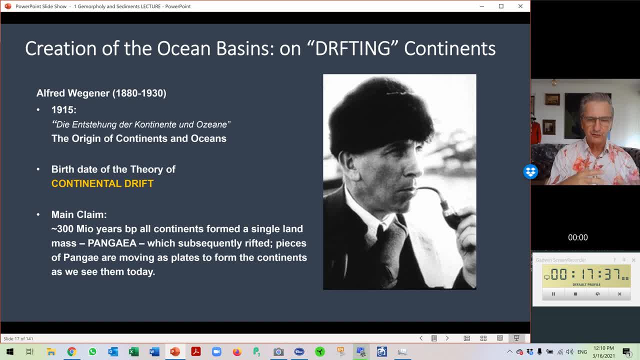 in the beginning there wasn't god, you know, playing tetris. no, no know playing tetris. no, no know playing tetris. no, no, in the beginning, about 300 million years in the beginning, about 300 million years in the beginning, about 300 million years ago. 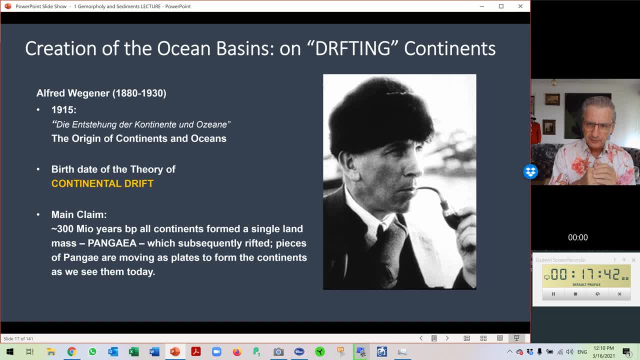 ago ago, everything clustered together, all the everything clustered together, all the everything clustered together, all the continents clustered together, continents clustered together, continents clustered together. they were called pangaea and all of that. they were called pangaea and all of that. they were called pangaea, and all of that was surrounded by one gigantic ocean. 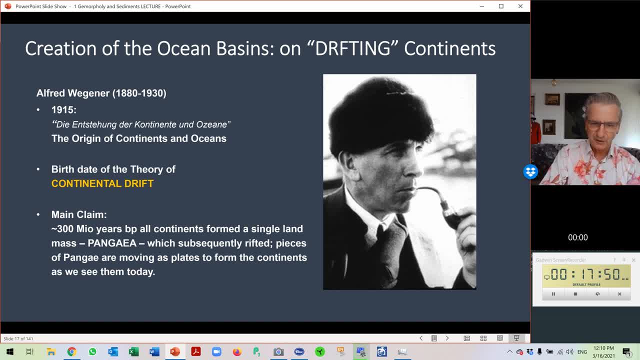 was surrounded by one gigantic ocean, was surrounded by one gigantic ocean called pantalasia, and then it actually called pantalasia, and then it actually called pantalasia, and then it actually would drifted apart, would drifted apart, would drifted apart. now he was actually declared. you know not. 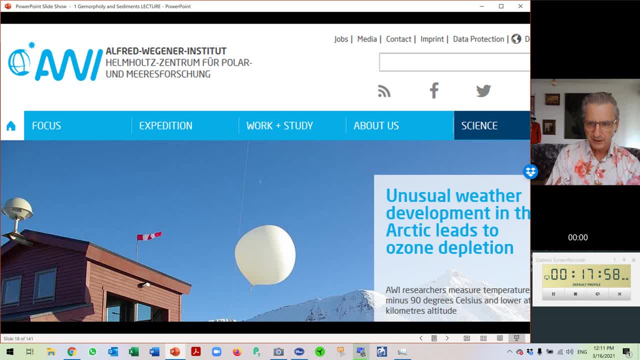 now he was actually declared. you know, not now he was actually declared, you know, not quite right in his head, but later on, of quite right in his head but later on, of quite right in his head, but later on, of course, about a hundred years later, course, about a hundred years later. 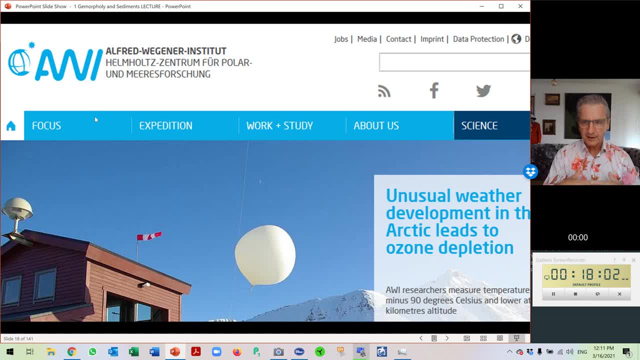 course, about a hundred years later, one of the world's most prestigious and one of the world's most prestigious and one of the world's most prestigious and active, active, active research institutes is actually named research institutes is actually named research institutes is actually named after him in germany. so 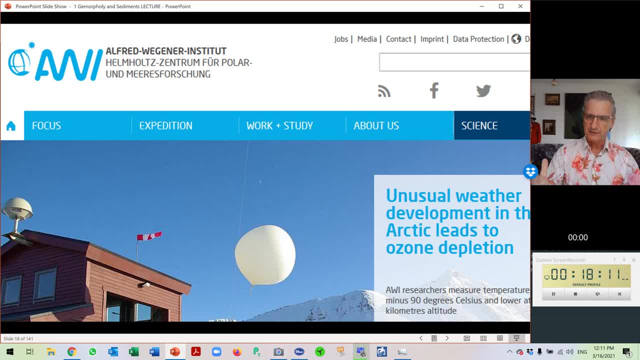 after him in germany, so after him in germany. so he might have been on to something. he might have been on to something, he might have been on to something. but as they say, sometimes fame comes. but as they say, sometimes fame comes, but as they say, sometimes fame comes late. 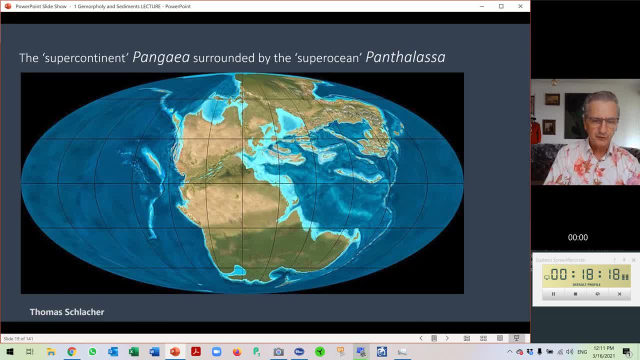 late, late, i'm waiting, never mind, i'm waiting, never mind, i'm waiting, never mind. there's lots of you know, there's lots of you know, there's lots of you know. fun, fun, fun. animations you can actually look like, but animations you can actually look like, but 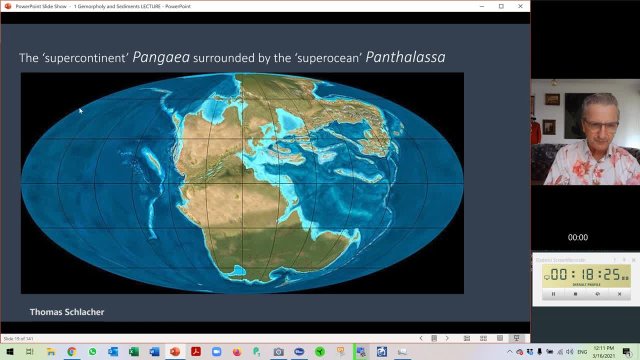 animations you can actually look like. but that's what people said. well, you know i, that's what people said. well, you know i. that's what people said. well, you know i. might have looked in the beginning, a might have looked in the beginning, a might have looked in the beginning- a gigantic ocean, pantalasia, surrounding 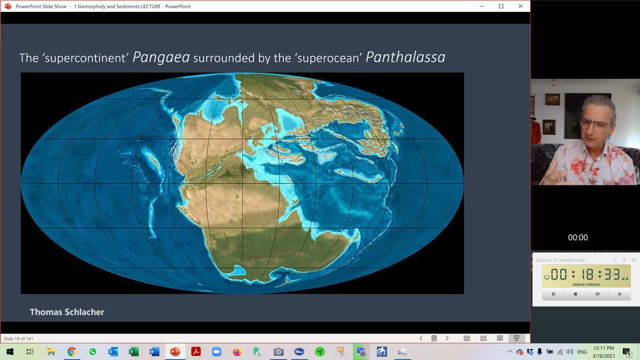 gigantic ocean, pantalasia, surrounding, gigantic ocean, pantalasia, surrounding. you know, you know, you know. the entire globe pan for everything, the entire globe pan for everything, the entire globe pan for everything: talasia for sea in greek, talasia for sea in greek, talasia for sea in greek, and basically, here is the land masses. 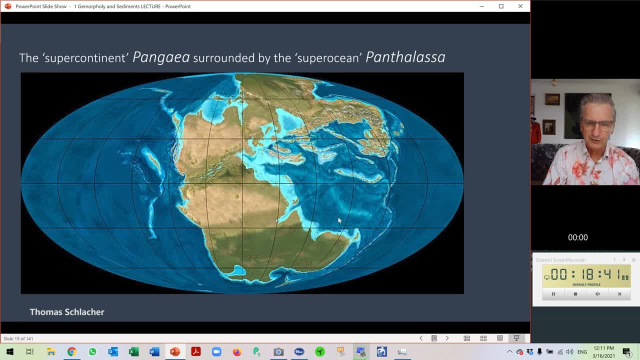 and basically here is the land masses and basically here is the land masses, that's what they, that's what they, that's what they come on, that's what they look like. come on, that's what they look like. come on, that's what they look like. some people differentiate that kind of 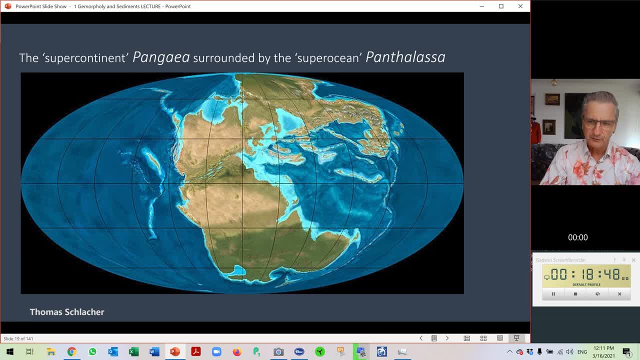 some people differentiate that kind of. some people differentiate that kind of shallow inland sea called the tetis. you shallow inland sea called the tetis, you shallow inland sea called the tetis, you will actually sometimes come across that, will actually sometimes come across, that will actually sometimes come across that. but basically this was the starting. 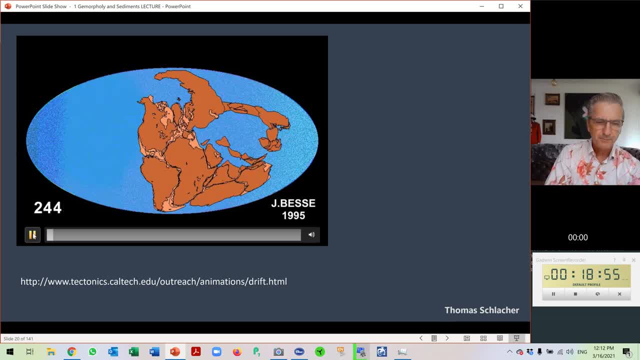 but basically this was the starting, but basically this was the starting, point 250, 300 million years ago. point 250 300 million years ago, point 250 300 million years ago. and then you can actually look at many and then you can actually look at many. 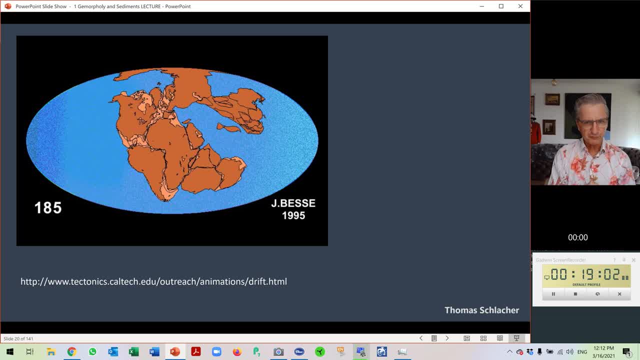 and then you can actually look at many, many, many, many animations on the web- truly good fun. animations on the web, truly good fun. animations on the web, truly good fun. and then it all started to actually drift, and then it all started to actually drift and then it all started to actually drift apart. 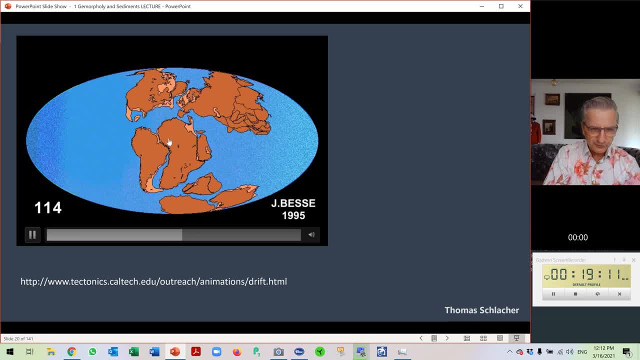 apart, apart- and i love this really- you can actually and i love this really, you can actually and i love this really. you can actually see, see, see south america and africa separated quite. south america and africa separated quite. south america and africa separated quite late. and then india. 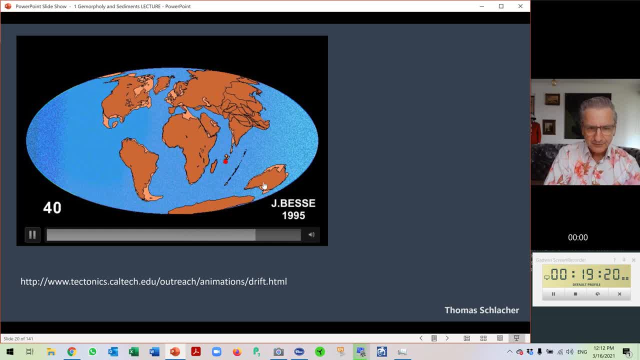 late, and then india, late and then india. yeah, it really starts to raise up and yeah, it really starts to raise up, and yeah, it really starts to raise up. and look at it, look at it, look at it. it actually has such a speed that, when it actually has such a speed that when 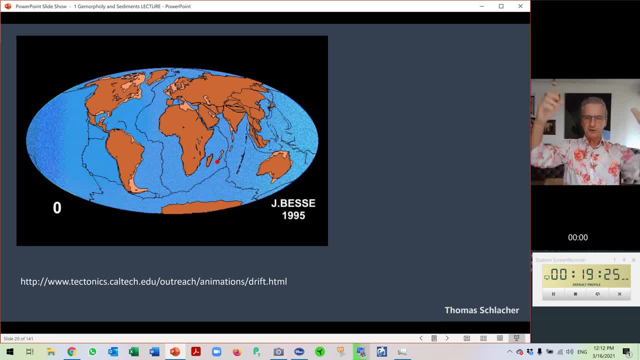 it actually has such a speed that when it actually crashes, it actually crashes. it actually crashes into asia. it forms the himalayan into asia. it forms the himalayan into asia. it forms the himalayan. mountains, mountains, mountains, and you know australia. let's do this. 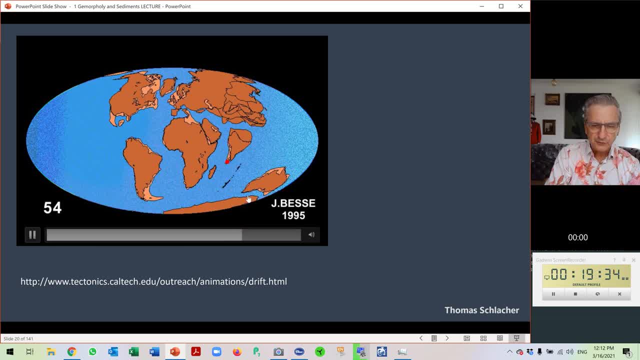 and you know australia, let's do this. and you know australia, let's do this again. let's go here again. let's go here again. let's go here. we started to separate from antarctica. we started to separate from antarctica. we started to separate from antarctica and drifted sort of east and north. 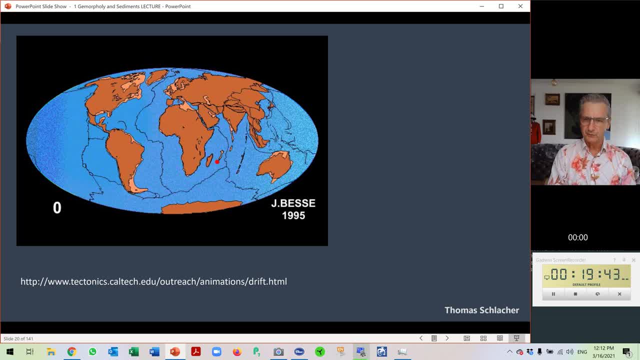 and drifted sort of east and north and drifted sort of east and north. but this is actually very uh important, but this is actually very uh important, but this is actually very uh important to remember. to remember: we are still drifting, we are still. we are still drifting, we are still. 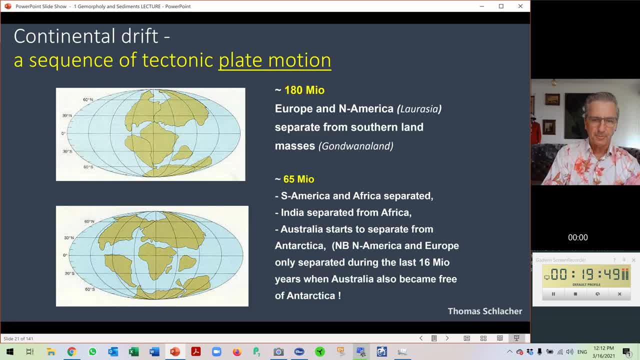 we are still drifting, we are still going up towards asia, going up towards asia, going up towards asia. so this, basically, we have just seen, so this, basically we have just seen. so this, basically we have just seen. so the idea was what we're going to. so the idea was what we're going to. 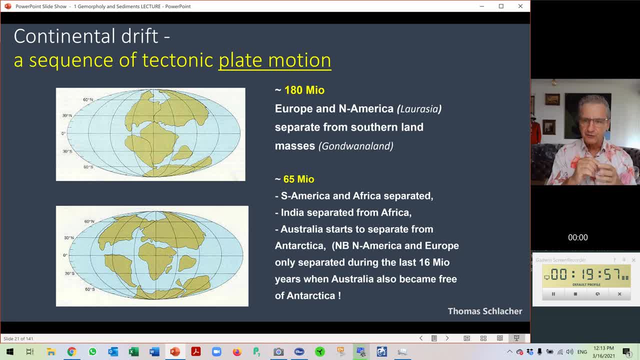 so the idea was: what we're going to said is said is said is: continents sit on plates like on bits. continents sit on plates like on bits. continents sit on plates like on bits and pieces of crust and they float on and pieces of crust and they float on. 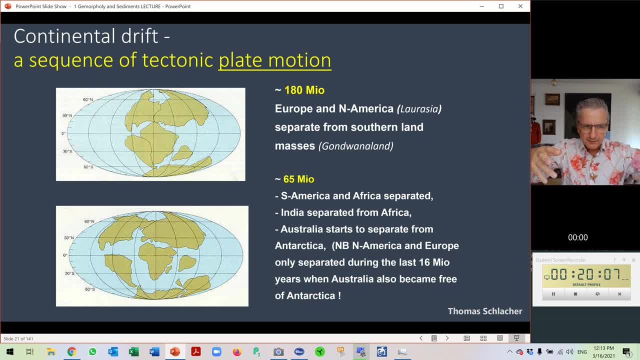 and pieces of crust and they float on a molten, a molten, a molten on a deformable, on a deformable, on a deformable. basically mess of rock, basically mess of rock, basically mess of rock. and that movement when it all broke up. and that movement when it all broke up, 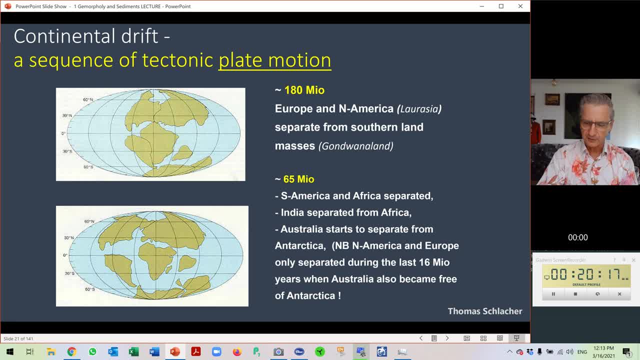 and that movement, when it all broke up, created the continents and ocean basins, created the continents and ocean basins, created the continents and ocean basins as we see them, as we see them, as we see them today, now, today, now, today. now you can basically, you know, write the. 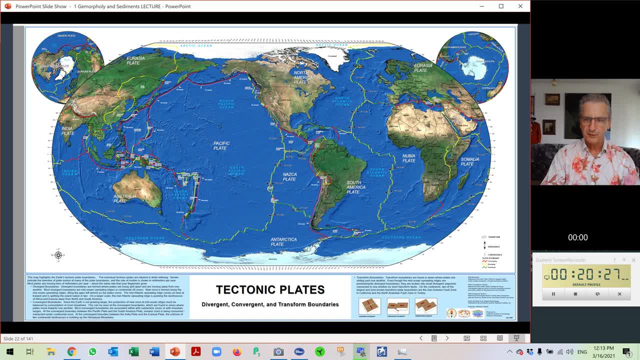 you can, basically, you know, write the. you can, basically, you know, write the lecture today and lecture today and lecture today and tomorrow there will be new material. i, tomorrow, there will be new material. i tomorrow, there will be new material. i just discovered that like a super high. 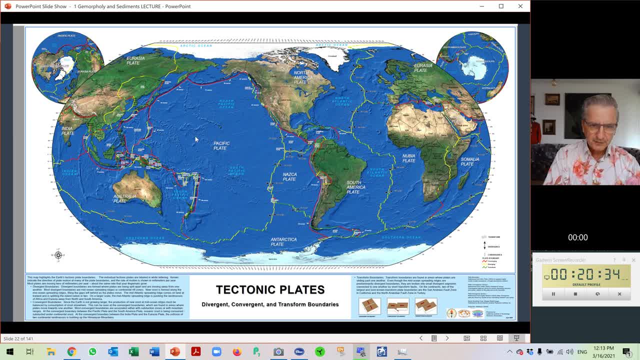 just discovered that like a super high, just discovered that like a super high resolution map of the continental plates resolution map of the continental plates resolution map of the continental plates. now, what you see immediately here, we now what you see immediately here. we now what you see immediately here. we have some very, very huge plates like the: 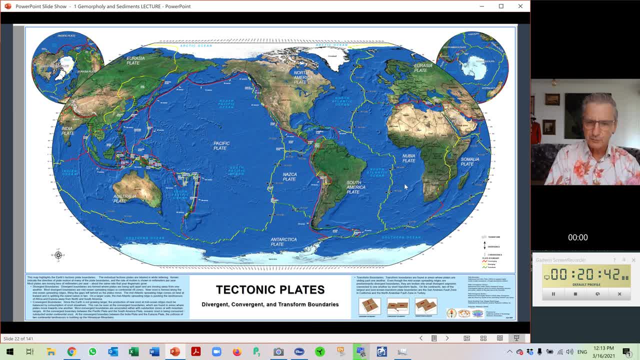 have some very, very huge plates like the. have some very, very huge plates like the pacific one, the nesca one pacific one. the nesca one- pacific one, the nesca one, the nubian one, named after the nubian. 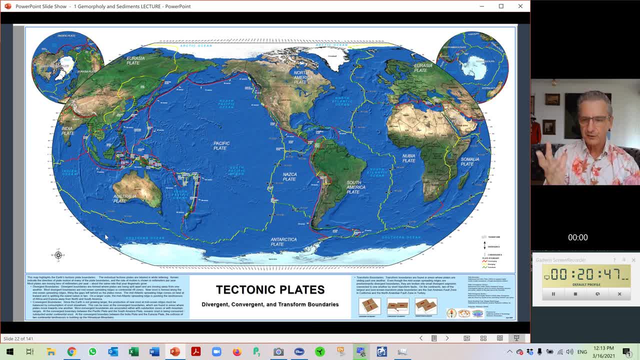 the nubian one named after the nubian, the nubian one named after the nubian. desert, the somali one, and so forth. desert, the somali one, and so forth, desert, the somali one, and so forth. now, of course, we got our own blade, the. 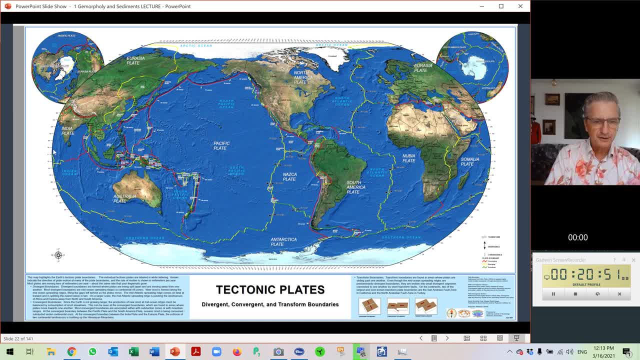 now, of course, we got our own blade, the now, of course we got our own blade, the australian blade, australian blade, australian blade. and to the north, we, you know, basically, and to the north, we, you know, basically, and to the north, we, you know, basically, bought the indian blade. 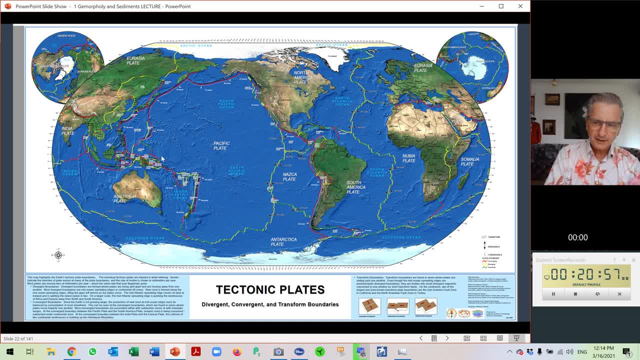 bought the indian blade, bought the indian blade and the pacific plate here and the pacific plate here and the pacific plate here. now that map, when you study it quite now. that map, when you study it quite now, that map, when you study it quite carefully. 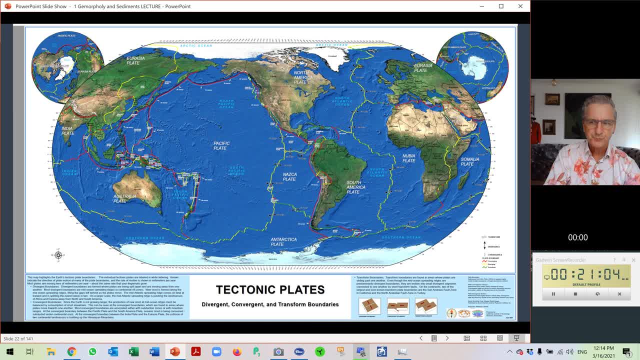 carefully, carefully will give you a very good understanding, will give you a very good understanding, will give you a very good understanding. why geologically speaking australia? why geologically speaking australia? why, geologically speaking, australia is boring as watching paint. right? because is boring as watching paint right because 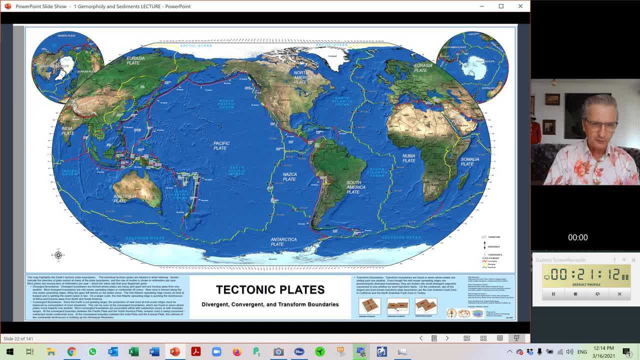 is boring as watching paint right, because we're sitting right in the middle. we're sitting right in the middle. we're sitting right in the middle. you know it's hundreds of kilometers to, you know it's hundreds of kilometers to. you know it's hundreds of kilometers to either blade boundary. so 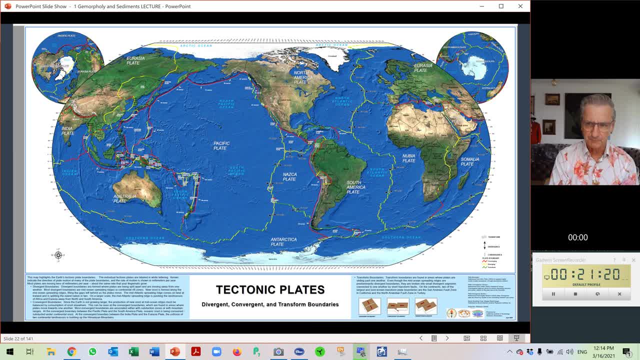 either blade boundary so, either blade boundary so. it's very old, it's very flat, it's very. it's very old, it's very flat, it's very. it's very old, it's very flat, it's very boring. we got lots of things in the boring. we got lots of things in the. 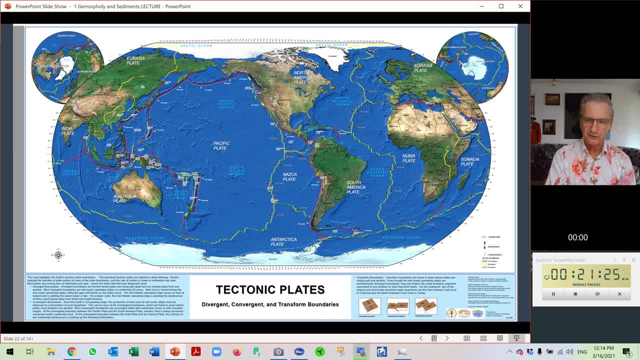 boring. we got lots of things in the ground which we can actually dig out, ground which we can actually dig out, ground which we can actually dig out, make some people very rich like gina, make some people very rich like gina, make some people very rich like gina reinhardt, and. 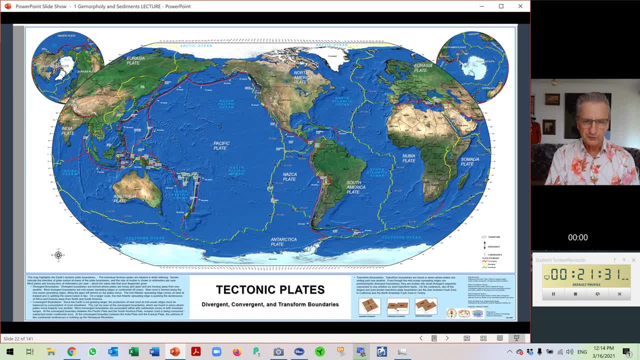 reinhardt and reinhardt and tricky forester, and we just ship the tricky forester and we just ship the tricky forester and we just ship the stuff to stuff to stuff to china. uh no, human rights questions are china. uh no, human rights questions are china. uh no, human rights questions are together and that's what keeps our 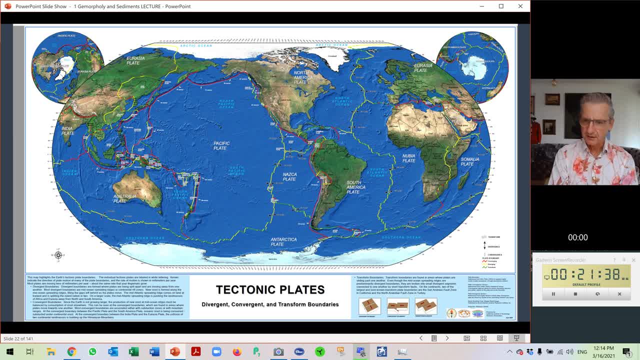 together and that's what keeps our together, and that's what keeps our economy going, economy going, economy going, but geologically speaking, and how many? but geologically speaking, and how many? but geologically speaking, and how many earthquakes do we have earthquakes? do we have earthquakes? do we have? luckily almost none. why? because we sit. 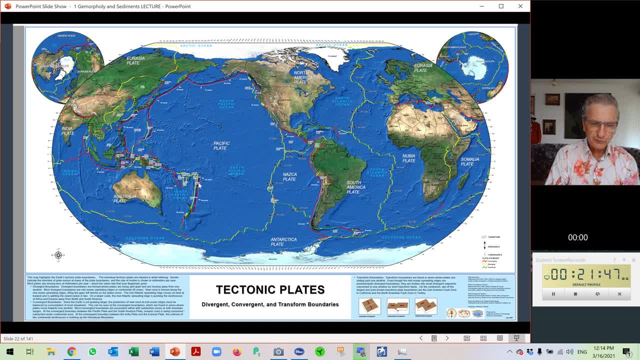 luckily almost none. why? because we sit, luckily almost none. why? because we sit right in the middle of one of those, right in the middle of one of those, right in the middle of one of those plates, plates, plates. how many earthquakes do the new? how many earthquakes do the new? how many earthquakes do the new zealanders have? how many earthquakes do zealanders have? how many earthquakes do the poor chaps up in bali zealanders have? how many earthquakes do the poor chaps up in bali zealanders have? how many earthquakes do the poor chaps up in bali png? japan. 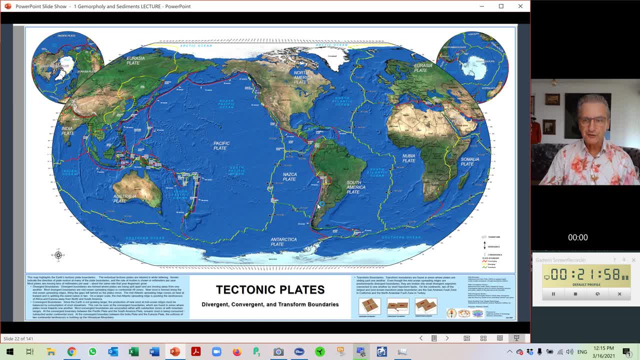 png- japan. png. japan. california and chile have tons. because california and chile have tons, because california and chile have tons because they're sitting right at the boundary. they're sitting right at the boundary. they're sitting right at the boundary of two plates and when they actually 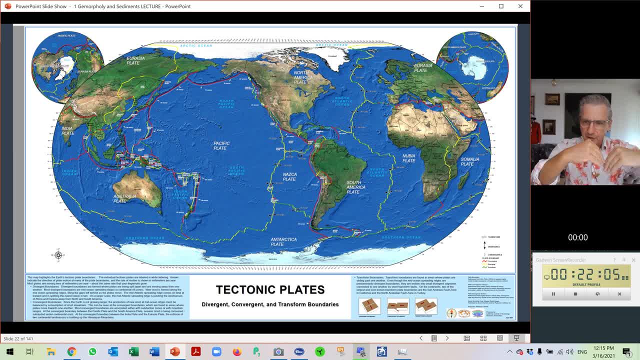 of two plates and when they actually of two plates and when they actually because they still move, and some of it because they still move and some of it because they still move, and some of it slips a little bit down, or they actually slips a little bit down or they actually. 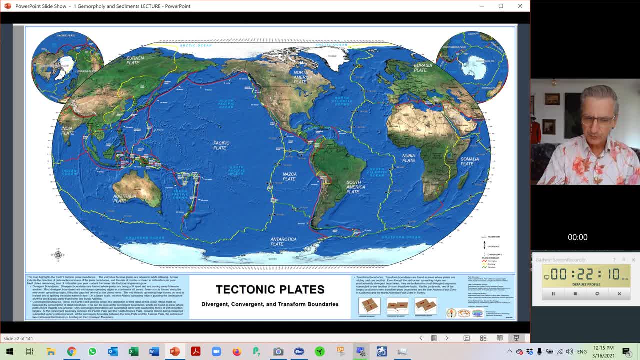 slips a little bit down, or they actually start rubbing parallel to each other, start rubbing parallel to each other, start rubbing parallel to each other. you've got major earthquakes, so that you've got major earthquakes. so that you've got major earthquakes. so that gives you an idea. 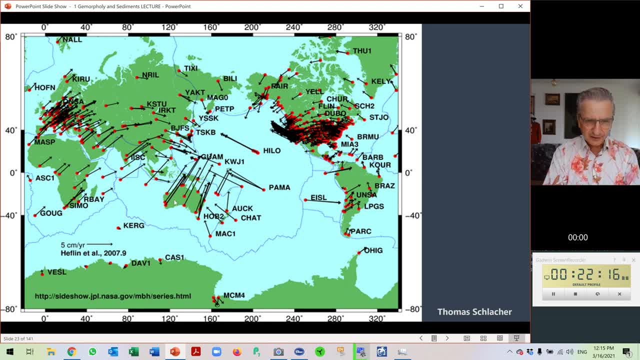 gives you an idea, gives you an idea of the speed of blade movement, basically of the speed of blade movement, basically of the speed of blade movement. basically, we have one of the, we have one of the. we have one of the fastest moving blades in australia going. fastest moving blades in australia going. 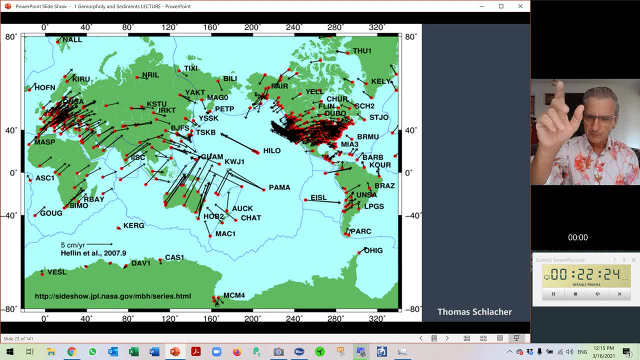 fastest moving blades in australia, going at least, at least at least two inches per year up towards asia, two inches per year up towards asia, two inches per year up towards asia. uh, now, if actually some of our uh, now if actually some of our uh, now if actually some of our politicians- and i'm 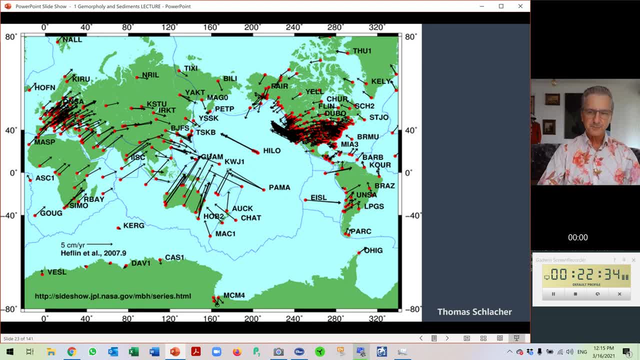 politicians and i'm politicians and i'm not going to name any names. think we not going to name any names? think we not going to name any names. think we actually, actually actually, are still a colony of you know great, are still a colony of you know great. 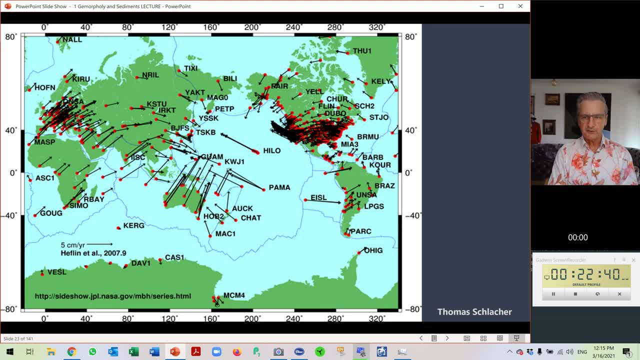 are still a colony of, you know, great britain telly hole and all the rest of britain telly hole and all the rest of britain telly hole and all the rest of it, it, it and we shouldn't really follow paul and we shouldn't really follow paul. 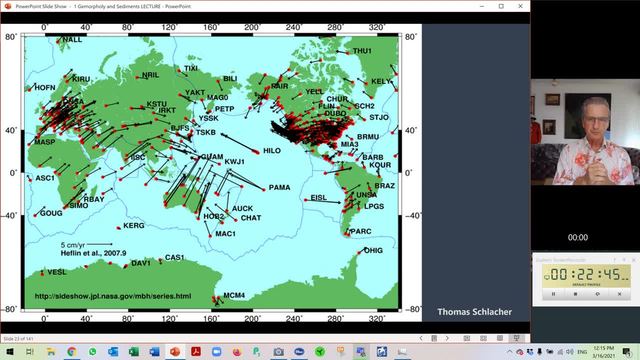 and we shouldn't really follow paul keating's metro, that we're actually part keating's metro, that we're actually part keating's metro, that we're actually part of asia, not of great britain of asia, not of great britain. of asia, not of great britain. well, you know what geology? 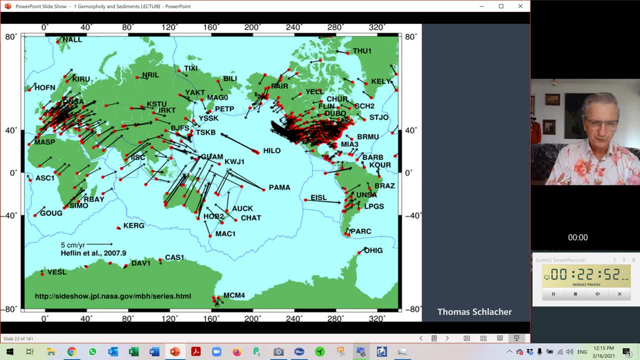 well, you know what geology, well, you know what geology will actually take care of that. because will actually take care of that, because will actually take care of that, because we're just moving north. we're just moving north. we're just moving north in the white room. 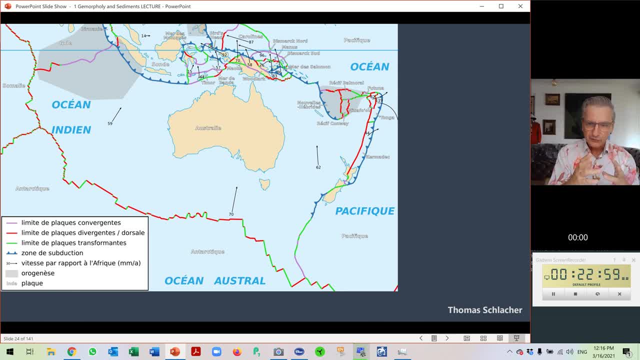 in the white room. in the white room, there's another one you can have, there's another one you can have, there's another one. you can have hundreds of dollars, but basically for us, hundreds of dollars, but basically for us, hundreds of dollars, but basically for us, what actually counts is 70 millimeters. 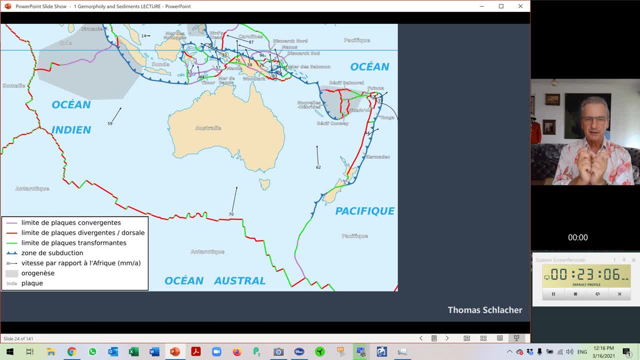 what actually counts is 70 millimeters. what actually counts is 70 millimeters a year. it's about that long in a year. it's about that long in a year. it's about that long in geologically time. that's geologically time. that's geologically time. that's massive. we're just pushing up north. 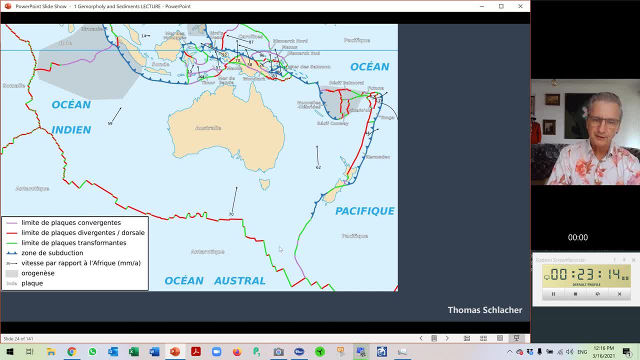 massive, we're just pushing up north. massive, we're just pushing up north. we're actually rubbing our new zealand. we're actually rubbing our new zealand. we're actually rubbing our new zealand. uh friends a little bit here, but they. uh friends a little bit here, but they. 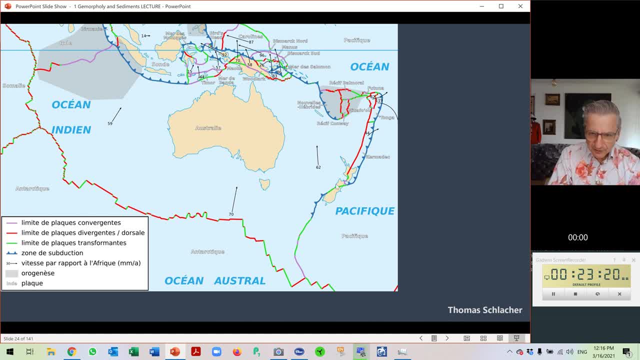 uh, friends, a little bit here, but they literally have their earthquakes. because literally have their earthquakes, because literally have their earthquakes, because right to the middle here, right to the middle here, right to the middle here is a blade boundary, it is the most is a blade boundary, it is the most. 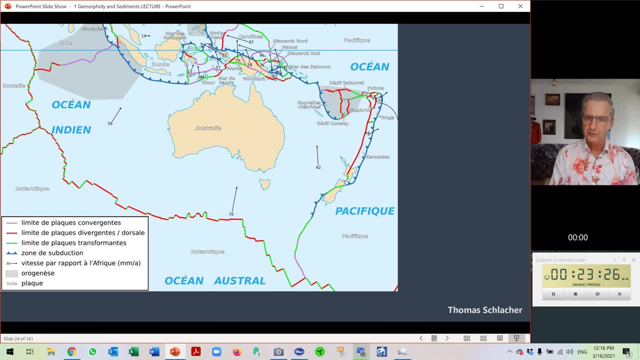 is a blade boundary. it is the most unfortunate, basically spot, unfortunate, basically spot, unfortunate, basically spot. they actually live on an island. of course they actually live on an island. of course they actually live on an island. of course they had no idea when they settled that. they had no idea when they settled that. 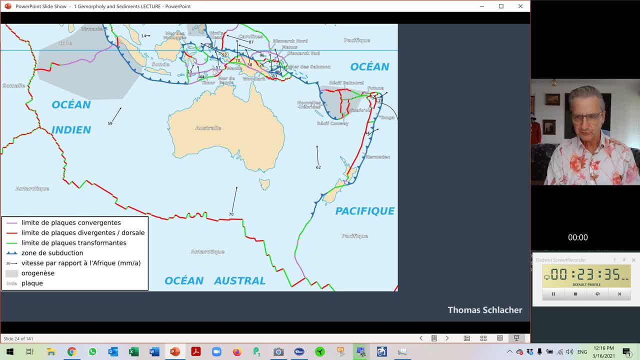 they had no idea when they settled that. and of course up here it's a complete mess. and of course up here it's a complete mess. and of course up here it's a complete mess. that's just like geologically chamber. that's just like geologically chamber. 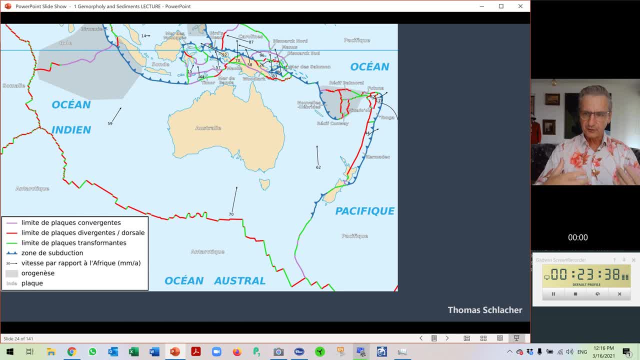 that's just like geologically chamber: bummer, bummer, bummer, but again we think about big tsunamis. and but again we think about big tsunamis. and but again we think about big tsunamis and earthquakes, earthquakes, earthquakes, they happen at blade boundaries. 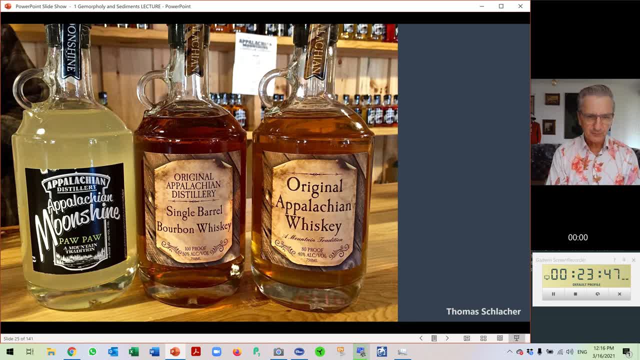 they happen at blade boundaries. they happen at blade boundaries. now, this is whiskey from the now. this is whiskey from the now. this is whiskey from the appalachian mountains, and you might appalachian mountains and you might appalachian mountains, and you might think like: 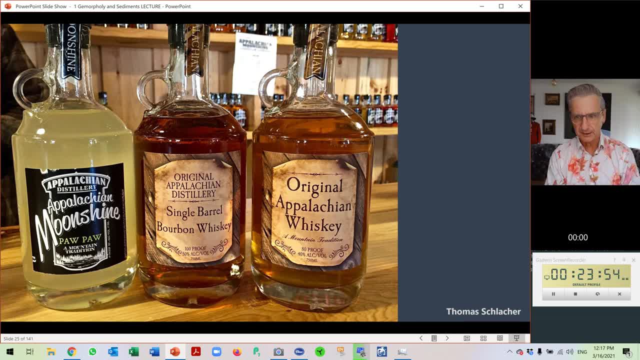 think, like, think, like: has thomas gone completely mad now? has thomas gone completely mad now? has thomas gone completely mad now? that probably yes, that probably yes, that probably yes, but never mind, here we've got some, but never mind, here we've got some, but never mind, here we've got some moonshine as well. 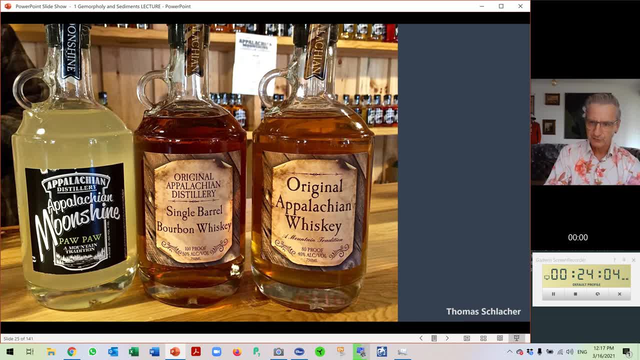 moonshine as well. moonshine as well. why is this significant? why is this significant? why is this significant? firstly, i actually drank the first. firstly, i actually drank the first. firstly, i actually drank the first american whiskey the other day. it's kind american whiskey the other day, it's kind. 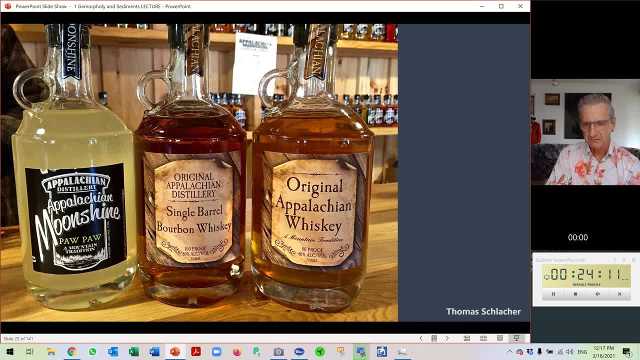 american whiskey the other day. it's kind of interesting, it's kind of sweet. it's a of interesting, it's kind of sweet, it's a of interesting, it's kind of sweet. it's a bit like bourbon, so probably stick to. bit like bourbon, so probably stick to. 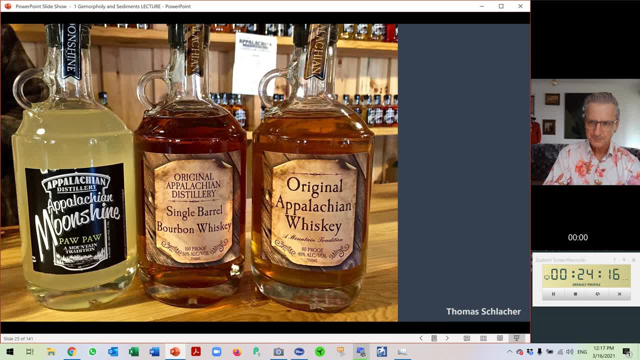 bit like bourbon. so probably stick to the rights, the rights, the rights in other original stuff, or in other original stuff, or in other original stuff, or the stuff from tasmania, never mind the stuff from tasmania. never mind the stuff from tasmania, never mind the appalachian mountains, geologically. 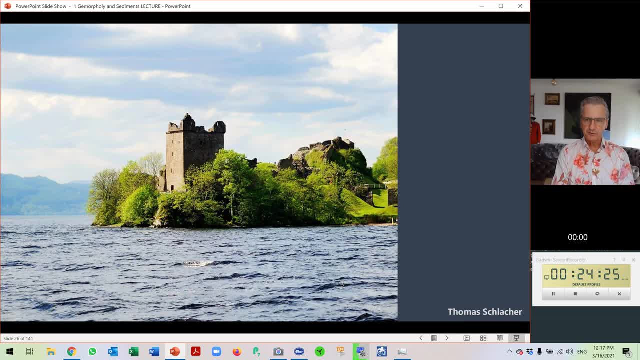 the appalachian mountains geologically. the appalachian mountains, geologically speaking, are very similar. speaking are very similar. speaking are very similar to the scottish highlands and people to the scottish highlands and people to the scottish highlands and people noticed that. 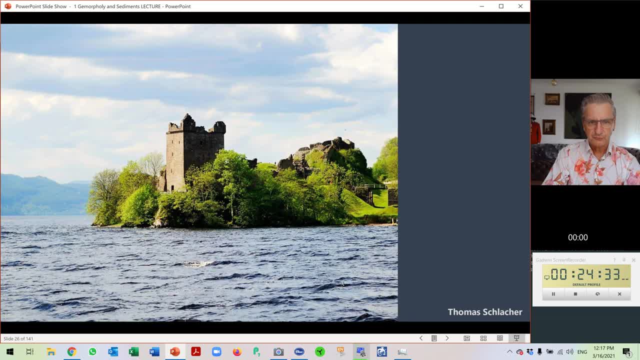 noticed that, noticed that about 100 years ago, about 100 years ago, about 100 years ago. and of course we got you know moonshine, and of course we got you know moonshine, and of course we got you know moonshine distilled in america. and we've got. 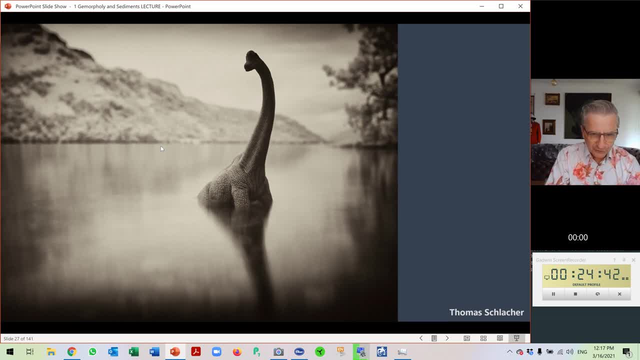 distilled in america and we've got distilled in america and we've got loch ness monster here. i love this one loch ness monster here. i love this one loch ness monster here. i love this one. look, look how hazy everything else is. look, look, how hazy everything else is. 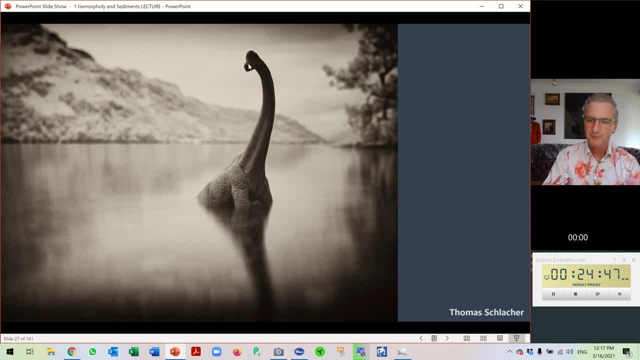 look, look, how hazy everything else is, and then got this beautifully defined. and then got this beautifully defined, and then got this beautifully defined: perfectly sharp dinosaur coming up here, perfectly sharp dinosaur coming up here, perfectly sharp dinosaur coming up here. great, great, great, um, um, um. we also noticed that right in the middle. 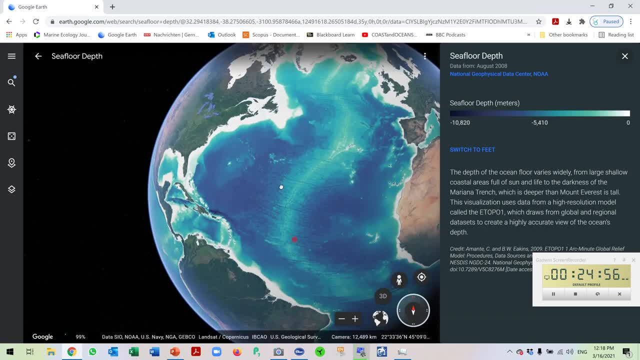 we also noticed that right in the middle. we also noticed that right in the middle, and let's have a look here again, and let's have a look here again, and let's have a look here again. we have this. you can actually well you. we have this. you can actually well you. 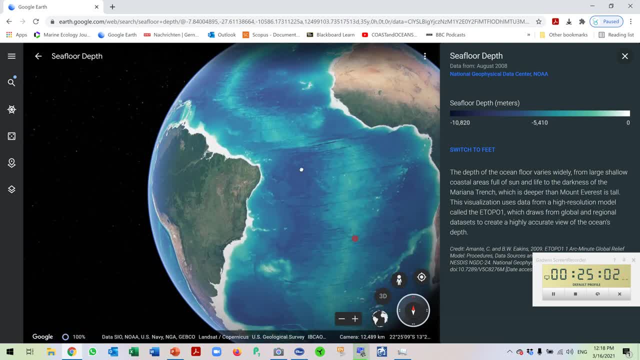 we have this. you can actually- well, you can't see it live, but you can actually can't see it live, but you can actually can't see it live, but you can actually exploit for yourself. you've got this exploit for yourself. you've got this exploit for yourself. you've got this massively big mountain chain. 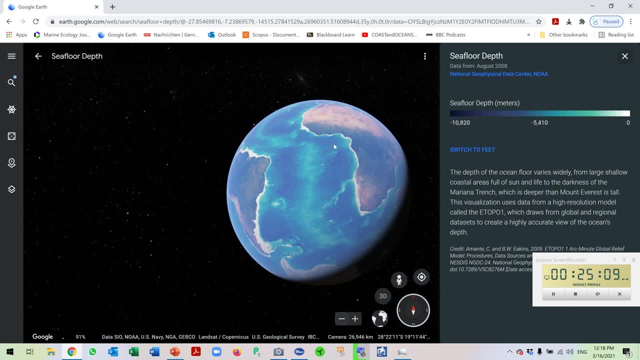 massively big mountain chain. massively big mountain chain. and even if you are terribly bad, and even if you are terribly bad, and even if you are terribly bad, crossword puzzles right. crossword puzzles right. crossword puzzles, right. we still actually have you know. we still actually have you know, we still actually have you know. a very good fit between 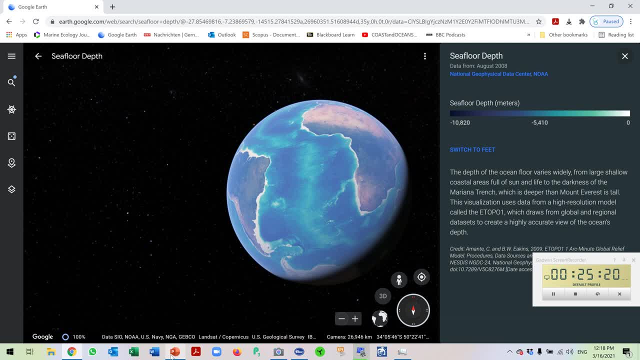 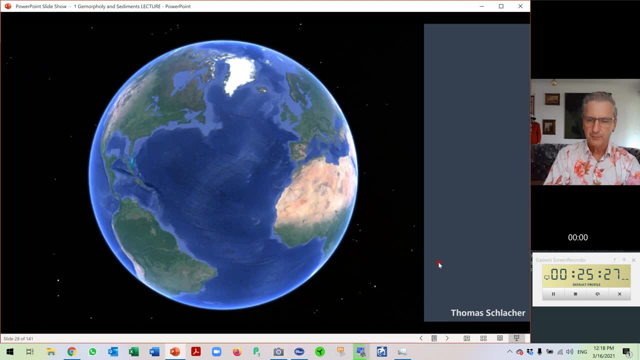 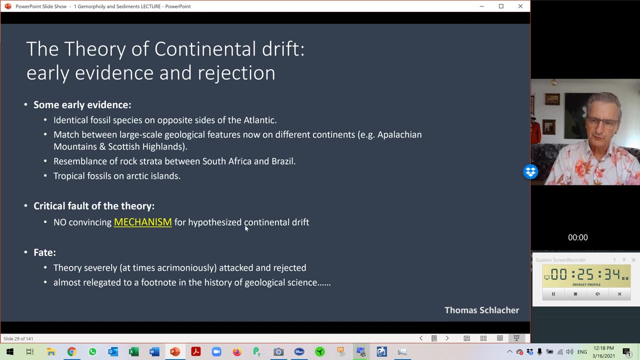 a very good fit between, a very good fit between south america and south america and south america and africa, africa, africa, right, right, right, on here, um, on here, um, on here, um, essentially people, essentially people, essentially people, you know, you know, you know, started to scratch their heads and says: 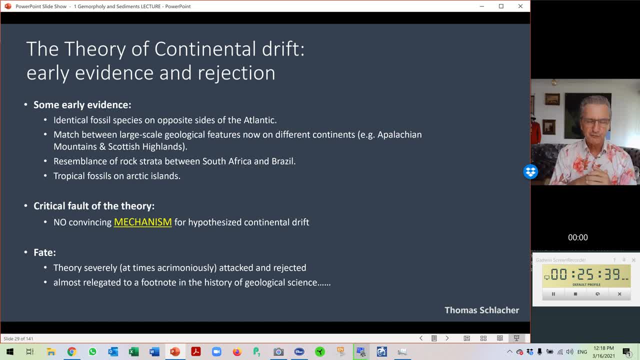 started to scratch their heads and says: started to scratch their heads and says: we've got all these, you know weird, we've got all these. you know weird, we've got all these. you know weird. fossil, fossil, fossil concurrences. we even got some concurrences. we even got some. 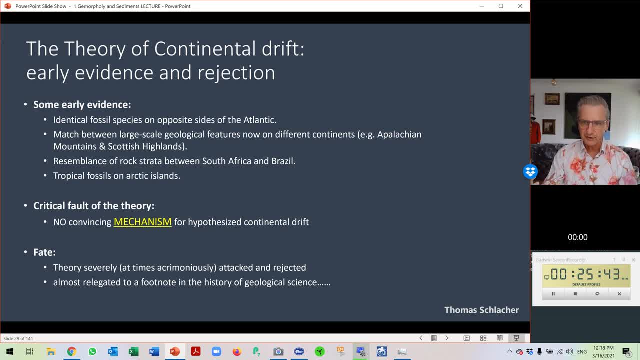 concurrences. we even got some very old plants that live in south, very old plants that live in south, very old plants that live in south america, antarctica and australia. how, america, antarctica and australia. how, america, antarctica and australia. how could that actually happen? 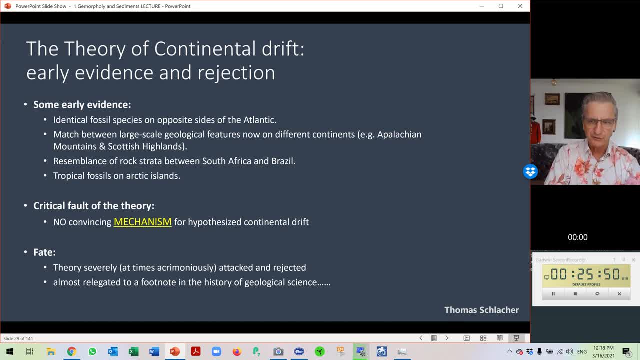 could that actually happen? could that actually happen? you know basically the geological, you know basically the geological. you know basically, the geological layering is the same in south africa as layering is the same in south africa, as layering is the same in south africa as it is in brazil. 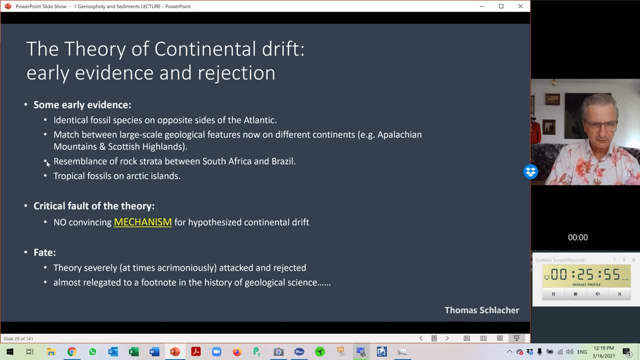 it is in brazil. it is in brazil and nowadays we get actually you know, and nowadays we get actually you know, and nowadays we get actually you know, remnants, as i just said, of tropical remnants, as i just said, of tropical remnants, as i just said, of tropical fossils on arctic islands. 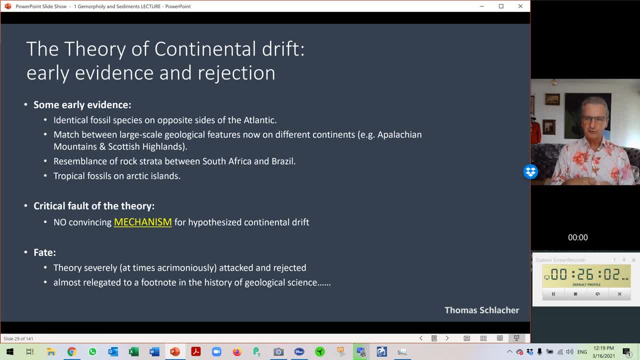 fossils on arctic islands. fossils on arctic islands, so so. so all of that seemed to actually support, all of that seemed to actually support, all of that seemed to actually support wegener's. you know theory of continental wegener's. you know theory of continental wegener's. you know theory of continental drift. 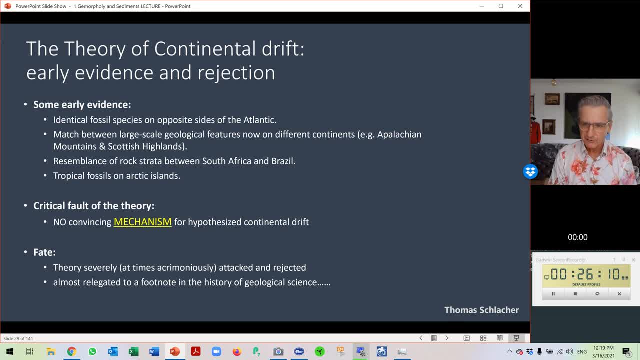 drift, drift. so why isn't he? why wasn't he more so? why isn't he? why wasn't he more so? why isn't he? why wasn't he more famous? as a matter of fact, he had to famous. as a matter of fact, he had to famous. as a matter of fact, he had to resign his position as professor of. 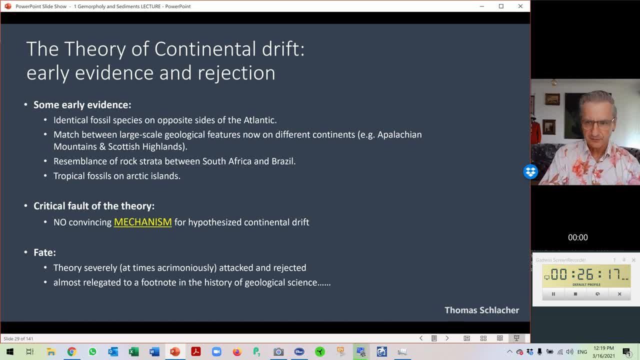 resign his position as professor of resign his position as professor of climatology, climatology, climatology. because people just said you know you're. because people just said you know you're. because people just said you know you're nuts, your theory, nuts, your theory, nuts, your theory theory got rejected and it remained so. 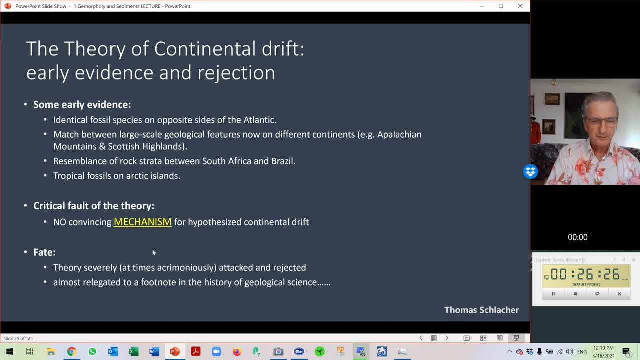 theory got rejected and it remained so. theory got rejected and it remained so until the 1950s, until the 1950s, until the 1950s, and basically, and basically, and basically. the problem was in science, you cannot. the problem was in science, you cannot. 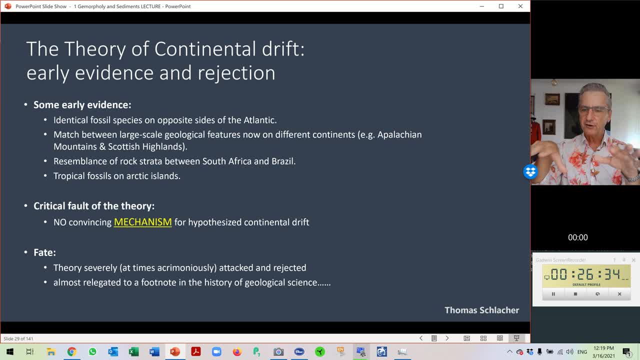 the problem was in science, you cannot just say, just say, just say, ah, i think this is actually how it, ah, i think this is actually how it, ah, i think this is actually how it happened. even if the pattern happened, even if the pattern happened, even if the pattern is very strong, you need to come up with 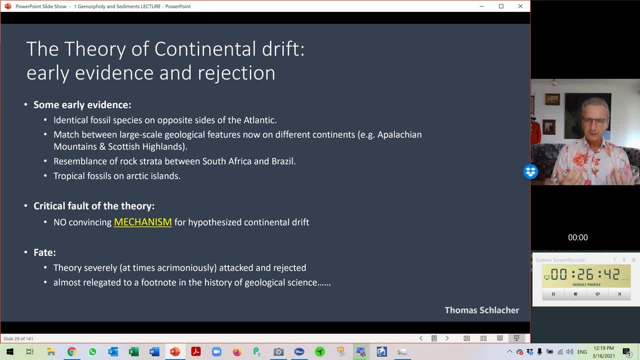 is very strong. you need to come up with is very strong. you need to come up with an explanation with a mechanism, an explanation with a mechanism, an explanation with a mechanism that actually drives it. so we're gonna that actually drives it. so we're gonna that actually drives it. so we're gonna. didn't have that. 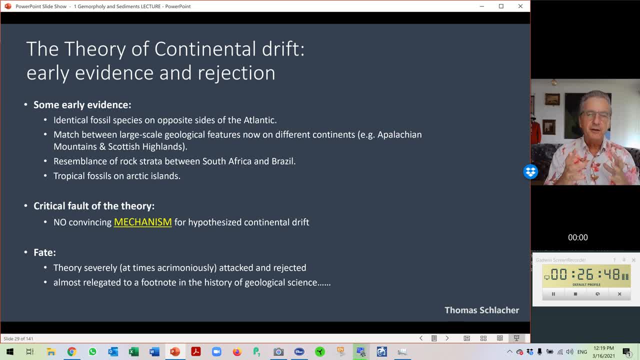 didn't have that, didn't have that, and we as a science community had no, and we as a science community had no, and we as a science community had no idea, idea, idea about the mechanism of continental drift, about the mechanism of continental drift, about the mechanism of continental drift, until about. 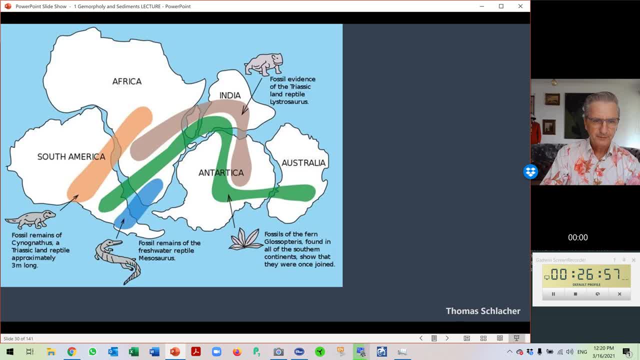 until about, until about 60 years ago. quite odd, isn't it 60 years ago? quite odd, isn't it 60 years ago? quite odd, isn't it? so here we here, you see all the. so here we here. you see all the. so here we here, you see all the concurrences. 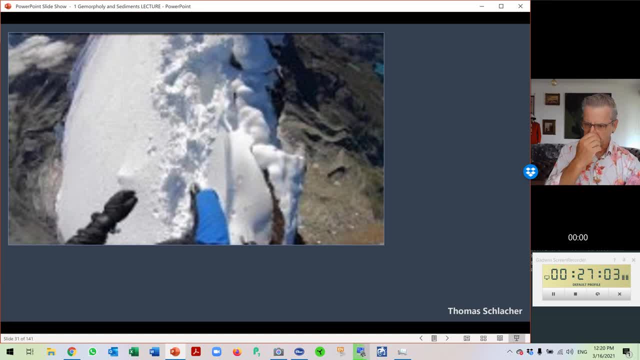 concurrences, concurrences. you know that's easy now. you know that's easy now. you know that's easy now. here's something very, very strange. if here's something very, very strange, if here's something very, very strange, if you are, you are, you are easily uh. 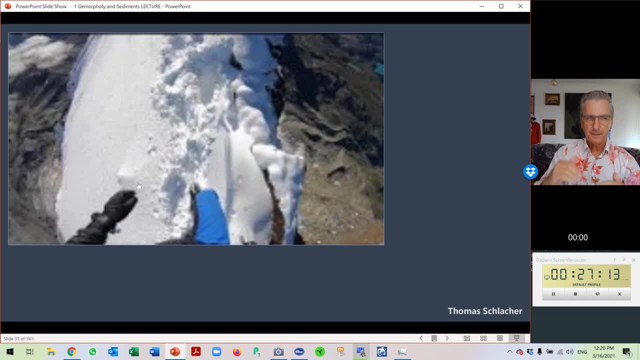 uh, uh, yeah. if your sense of, yeah. if your sense of, yeah. if your sense of uh, uh, uh, uh. your balance, sense of balance is not uh. your balance, sense of balance is not uh. your balance, sense of balance is not very good and you get slightly dizzy. 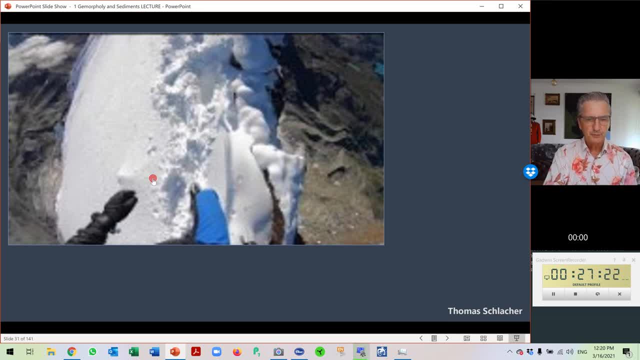 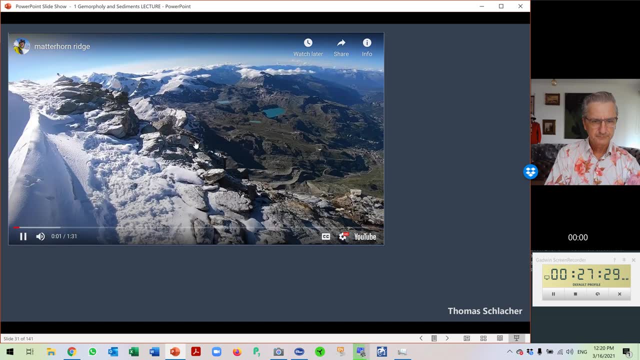 very good and you get slightly dizzy. very good, and you get slightly dizzy. don't watch this one. don't watch this one. don't watch this one. now, come on, if you actually climb a mountain, what happens is you get to the top, and what happens is you get to the top and 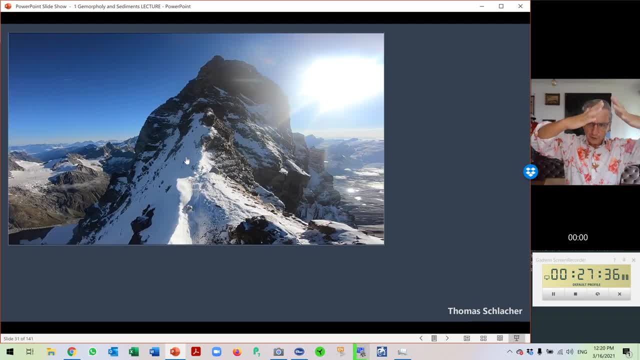 what happens is: you get to the top and there's usually a peak, there's usually a peak, there's usually a peak. or there's a ridge and it goes down on, or there's a ridge and it goes down on, or there's a ridge and it goes down on both sides. 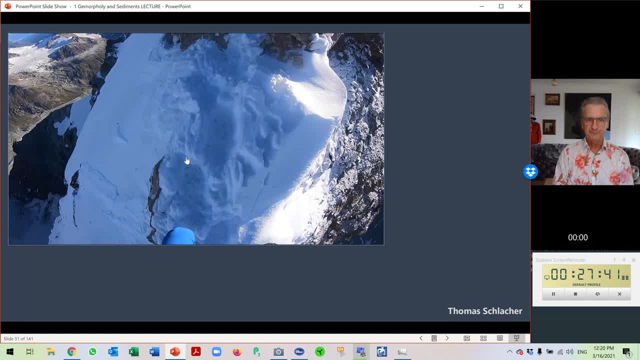 both sides, both sides. i just love it. i just love it. i just love it. it's a fisheye lens, but never mind. it's a fisheye lens, but never mind. it's a fisheye lens, but never mind, it's cool, isn't it? 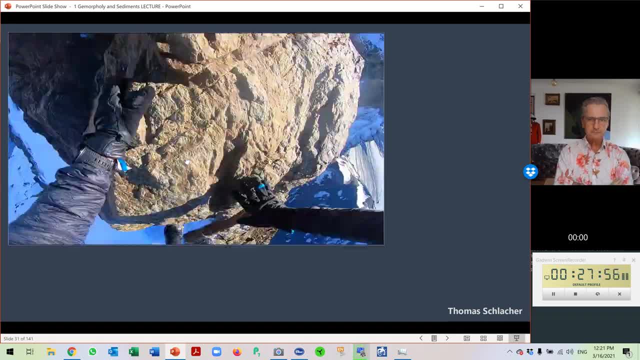 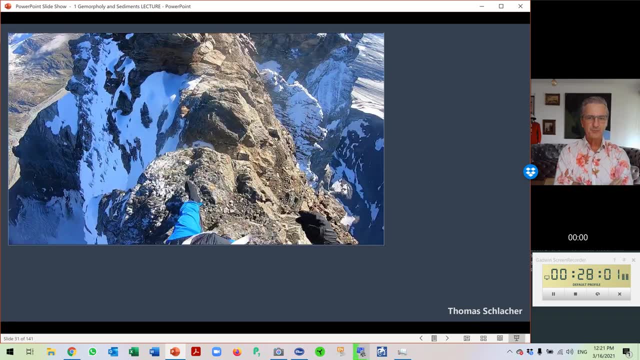 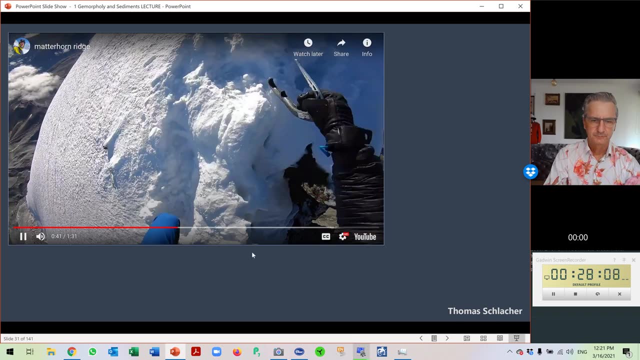 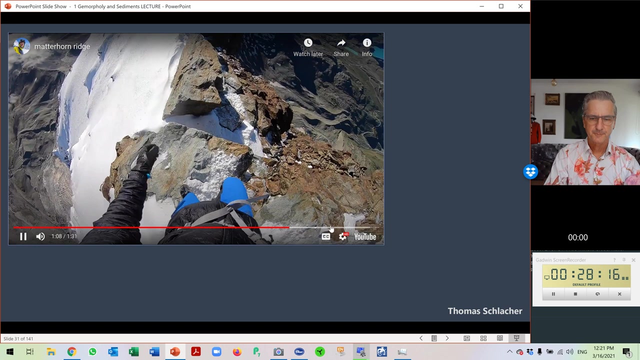 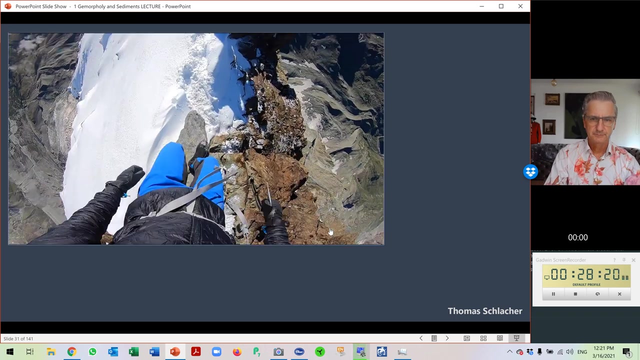 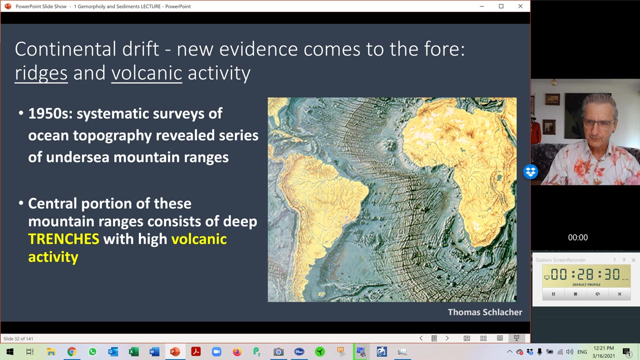 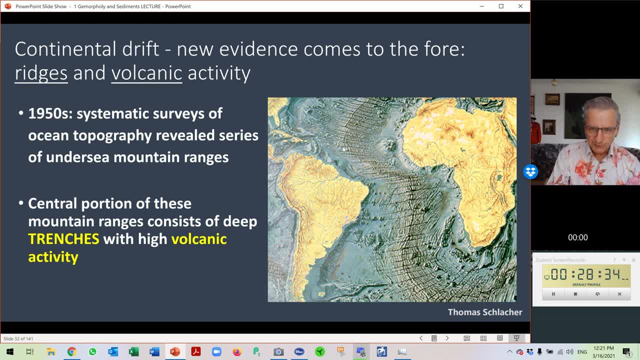 i think everybody get the idea now what is actually very odd. now, what is actually very odd now what is actually very odd when you go into the deep sea, when you go into the deep sea, when you go into the deep sea and you examine some of those mountain. 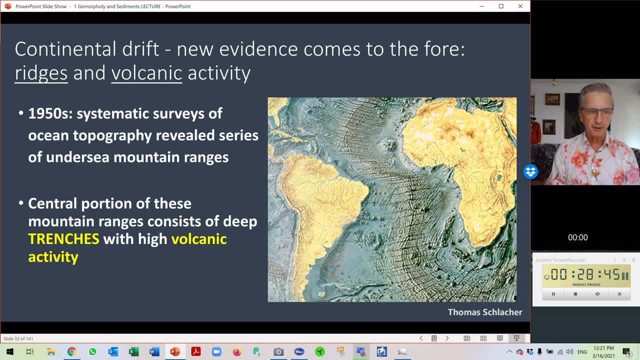 and you examine some of those mountain and you examine some of those mountain ranges here. here we've got the ranges here. here we've got the ranges here. here we've got the mid-atlantic bridge, mid-atlantic bridge, mid-atlantic bridge. it actually is not like the matter one. 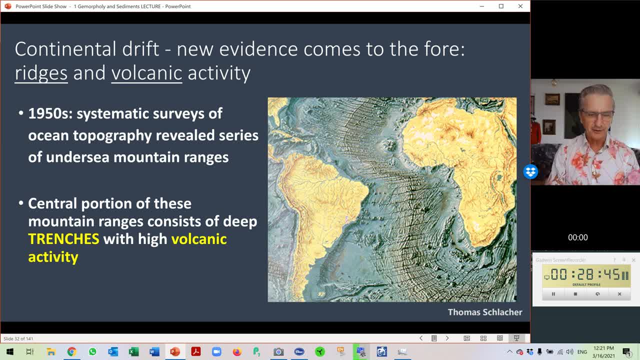 it actually is not like the matter one. it actually is not like the matter one. there's actually a valley at the top. so there's actually a valley at the top. so there's actually a valley at the top. so you actually climb up. he's like: oh i 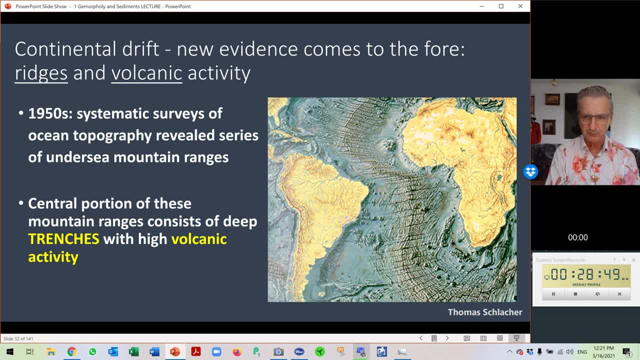 you actually climb up, he's like, oh, i, you actually climb up. he's like, oh, i must you know. think about sir edmund, must you know. think about sir edmund, must you know. think about sir edmund. hillary, climbing the mount everest. hillary, climbing the mount everest. 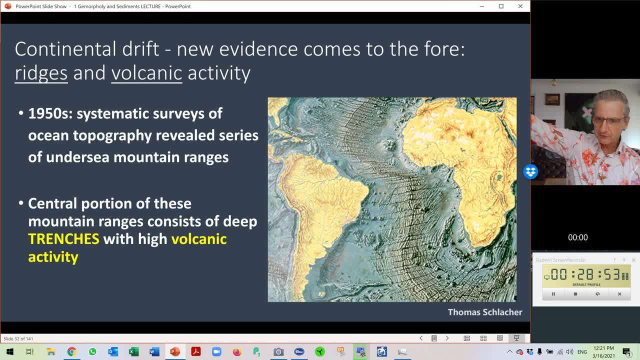 hillary, climbing the mount everest, climbing up on the bum, and i look down, climbing up on the bum, and i look down climbing up on the bum, and i look down into a valley, and there's another into a valley, and there's another into a valley and there's another peak or another ridge about. you know 20. 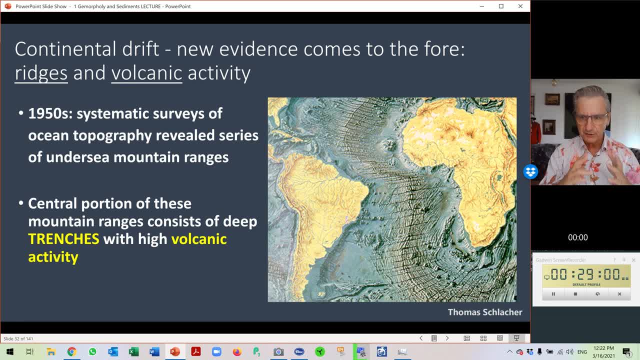 peak or another ridge about you know 20 peak, or another ridge about you know 20 kilometers across or 100.. now that's kilometers across or 100.. now that's kilometers across or 100.. now that's completely ridiculous, completely ridiculous, completely ridiculous. but yet the undersea. 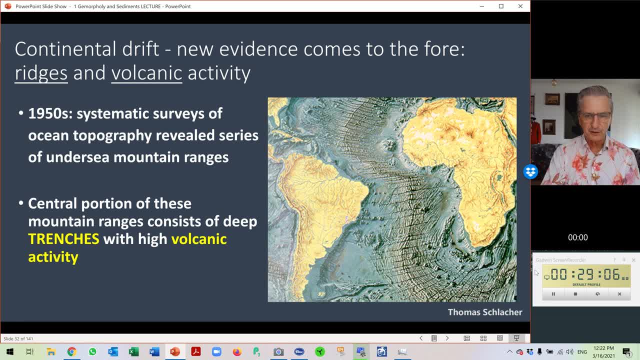 but yet the undersea, but yet the undersea mountain ranges. got a big big, massive mountain ranges. got a big big, massive mountain ranges. got a big big, massive trench right here in the middle. if you trench right here in the middle, if you trench right here in the middle, if you don't actually believe me, go to google. 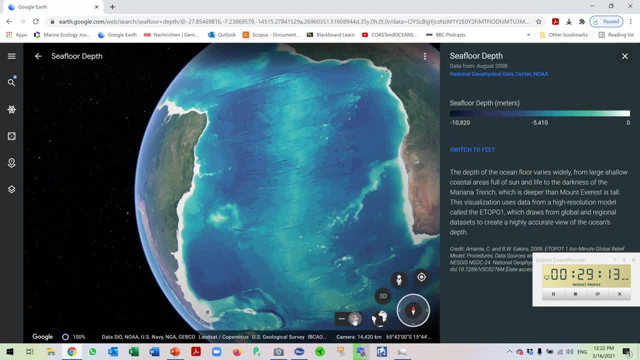 don't actually believe me, go to google, don't actually believe me. go to google earth and check it all out earth, and check it all out earth, and check it all out, and we can go to nowhere, and we can go to nowhere, and we can go to nowhere saying: what do we see? 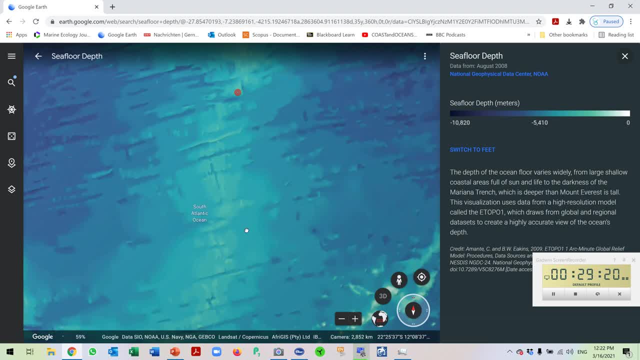 saying: what do we see? saying: what do we see? you know, you know, you know. you got the mid-atlantic ridge, and yet you got the mid-atlantic ridge, and yet you got the mid-atlantic ridge, and yet in the middle, here, in the middle here. 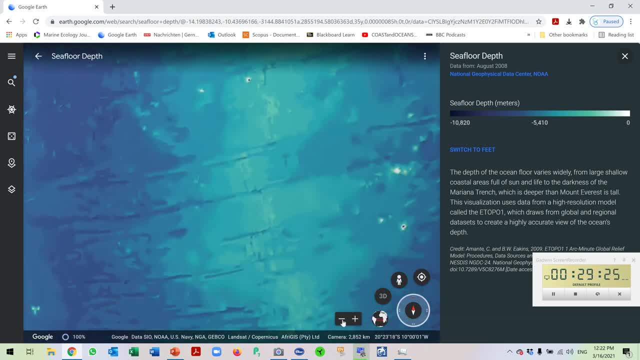 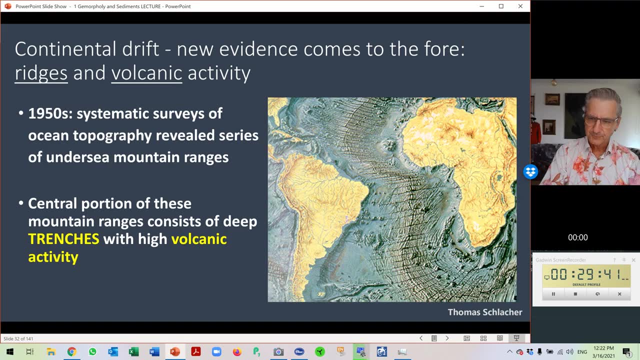 in the middle. here is, for most part, is for most part, is for most part, a deep valley, a deep valley, a deep valley. how very, very odd, how very, very odd. and you can actually see it going up, and you can actually see it going up, and you can actually see it going up here, blah, blah, blah, blah. 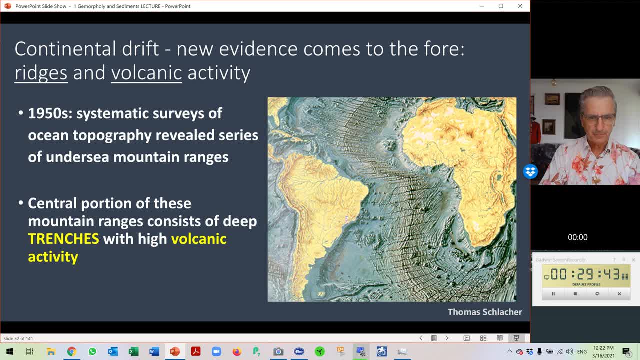 here, blah, blah, blah, blah. here, blah, blah, blah, blah. so so, so we have, we have, we have a ridge on a ridge, on a ridge on our top of the undersea mountains, our top of the undersea mountains, our top of the undersea mountains. now, now. 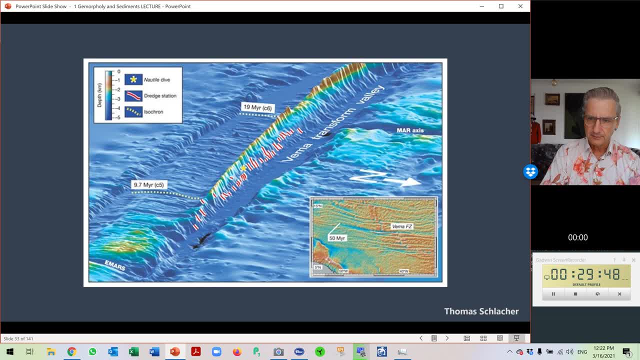 now, um, um, um, if that would not be strange enough, you, if that would not be strange enough, you, if that would not be strange enough, you see a, see a, see a. you know detailed, you know detailed, you know detailed. topography of a symmetry, i should say. 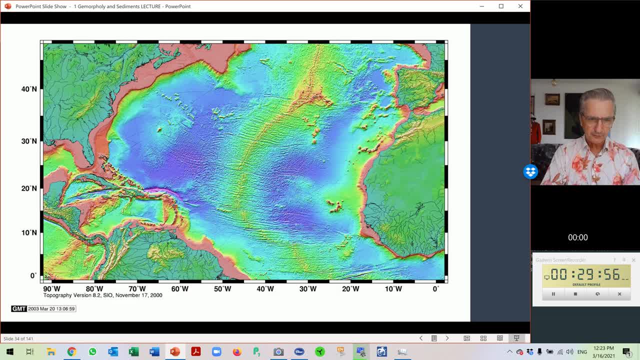 topography of a symmetry. i should say: topography of a symmetry, i should say from the north atlantic, from the north atlantic, from the north atlantic. and here you see another depiction of, and here you see another depiction of, and here you see another depiction of it all you've got, you know. 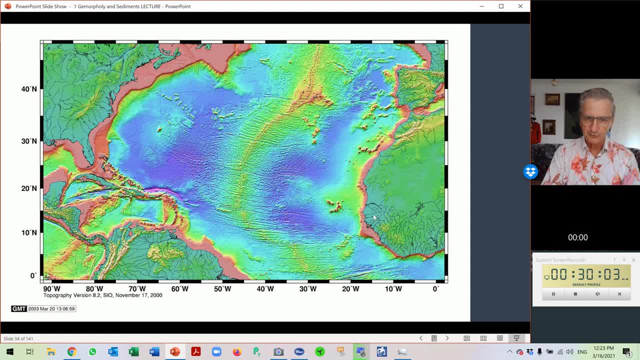 it all you've got. you know it all you've got, you know: mauritania, here west africa, gabon. mauritania, here west africa, gabon. mauritania, here west africa, gabon, senegal, and all of this dakar, the dakar, senegal, and all of this dakar, the dakar. 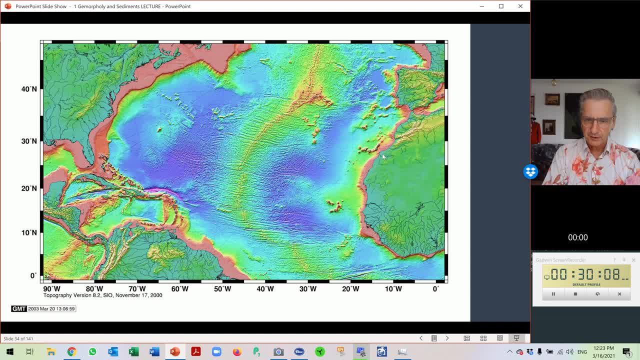 senegal and all of this. dakar, the dakar valley, valley, valley, and here baritaka and here baritaka and here baritaka. mauritania going up towards morocco, mauritania going up towards morocco, mauritania going up towards morocco. portugal, spain, france, 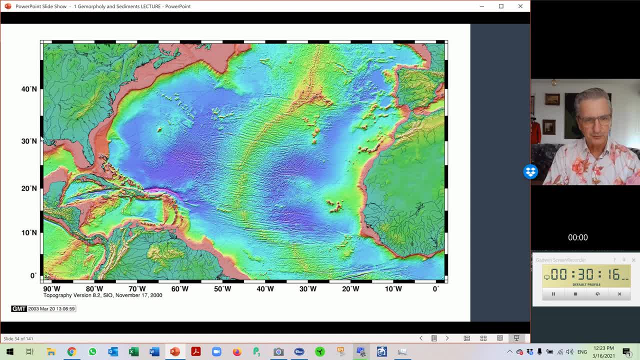 portugal, spain, france, portugal, spain, france. this is sort of used to be trump land. this is sort of used to be trump land. this is sort of used to be trump land. now it's the proper united states of. now it's the proper united states of. 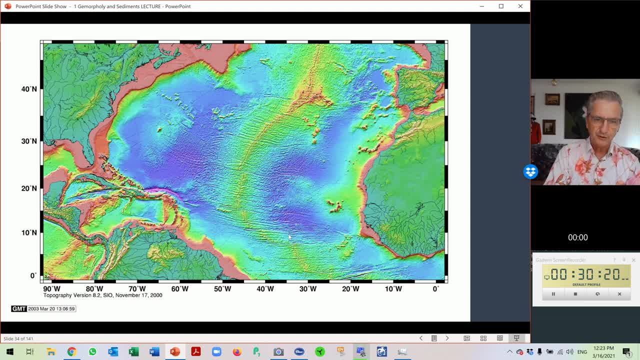 now it's the proper. united states of america again got a deep trench here. america again got a deep trench here. america again got a deep trench here called the puerto rico trench, called the puerto rico trench, called the puerto rico trench. but this central long mountain range, but this central long mountain range. 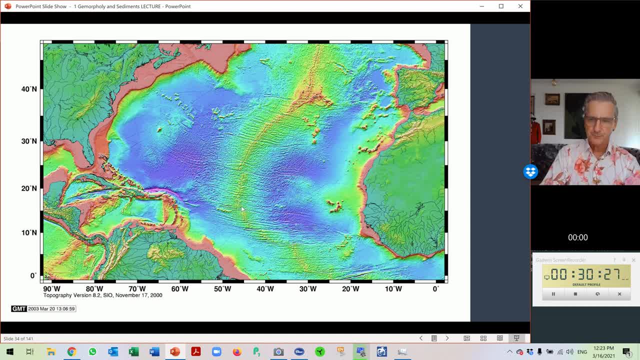 but this central long mountain range has a big valley in the middle, has a big valley in the middle, has a big valley in the middle. we have nothing like this on land at all. we have nothing like this on land at all. we have nothing like this on land at all, by the way. 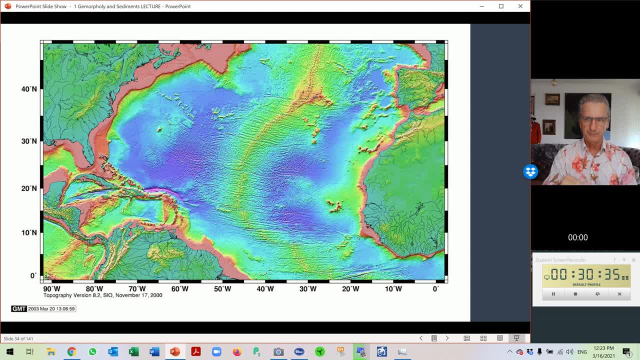 by the way, by the way. trivial pursuit question. what is the trivial pursuit question? what is the trivial pursuit question? what is the longest mountain range in the world? longest mountain range in the world? longest mountain range in the world? it's the middle atlantic ridge. i once 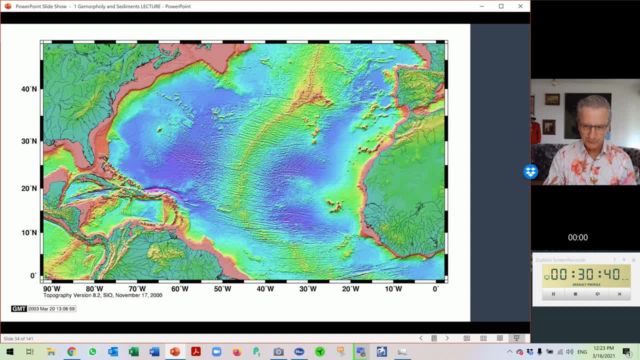 it's the middle atlantic ridge, i once. it's the middle atlantic ridge, i once want a pair of. want a pair of. want a pair of uh earphones for that. so here you go- uh earphones for that. so here you go, uh earphones for that. so here you go. something useful coming out on this. 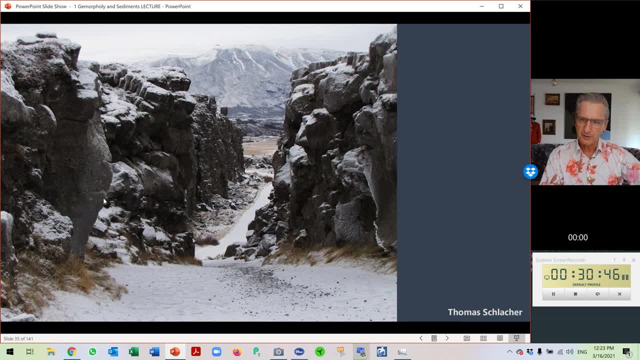 something useful coming out on this, something useful coming out on this: lecture, lecture, lecture, uh, i highly recommend, uh, i highly recommend, uh, i highly recommend. going to iceland is just mind-blowing if going to iceland is just mind-blowing, if going to iceland is just mind-blowing if you're a scientist. 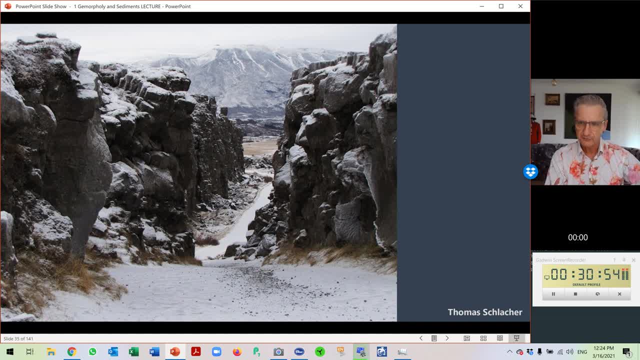 you're a scientist, you're a scientist. it is truly mind-blowing. it's mind, it is truly mind-blowing. it's mind, it is truly mind-blowing. it's mind-blowing as well. you know, just don't blowing as well. you know, just don't. 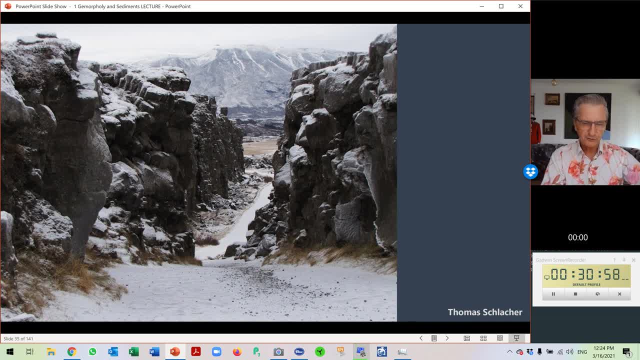 blowing as well. you know, just don't go out and have anything. go out and have anything. go out and have anything normal to eat, because you actually you normal to eat, because you actually you normal to eat, because you actually you know, know, know, pay a weak salary, never mind, this is. 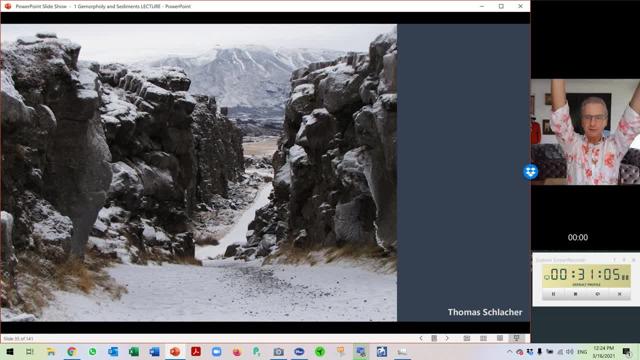 pay a weak salary, never mind. this is pay a weak salary, never mind. this is actually actually actually the mid-atlantic ridge coming out of the. the mid-atlantic ridge coming out of the. the mid-atlantic ridge coming out of the sea, sea. 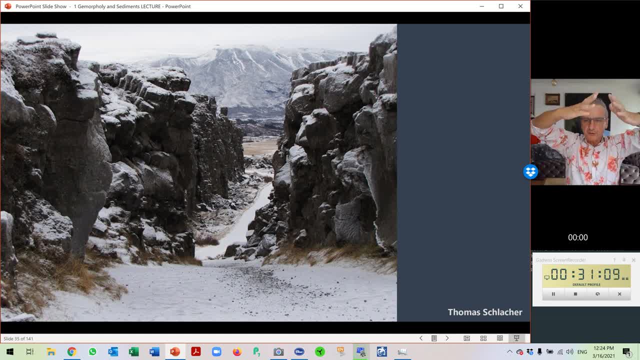 sea, and this is that valley, of course, the, and this is that valley, of course, the. and this is that valley, of course, the very, very beginning. so it's not actually very, very beginning, so it's not actually very, very beginning, so it's not actually that deep. 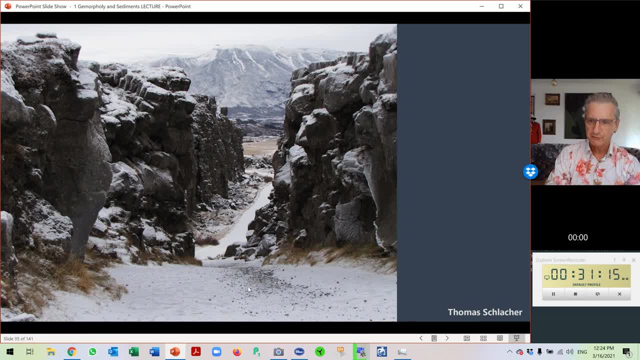 that deep, that deep. i just couldn't actually help myself. i just couldn't actually help myself. i just couldn't actually help myself actually picking up, actually picking up, actually picking up a few stones here, stuffing them into my. a few stones here stuffing them into my, a few stones here, stuffing them into my sailing jacket, and two years later i had 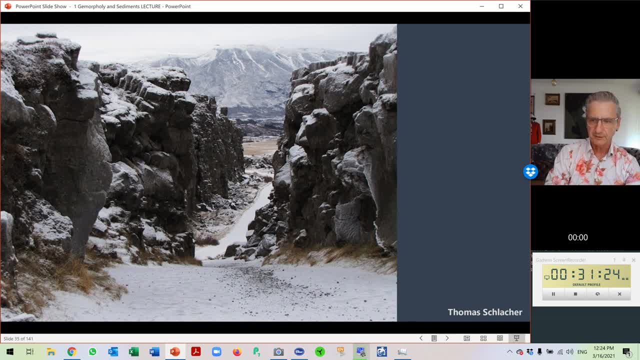 sailing jacket, and two years later i had sailing jacket, and two years later i had a body search, a body search, a body search. i forgot about all of that in canada at. i forgot about all of that in canada at. i forgot about all of that in canada at the airport. and then 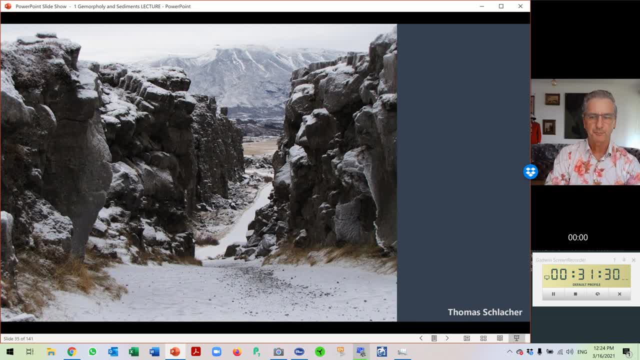 the airport, and then the airport. and then: why are you carrying stones and yep? why are you carrying stones and yep? why are you carrying stones and yep? it took two hours in a perfectly. it took two hours in a perfectly. it took two hours in a perfectly stainless steel room and, yep, the 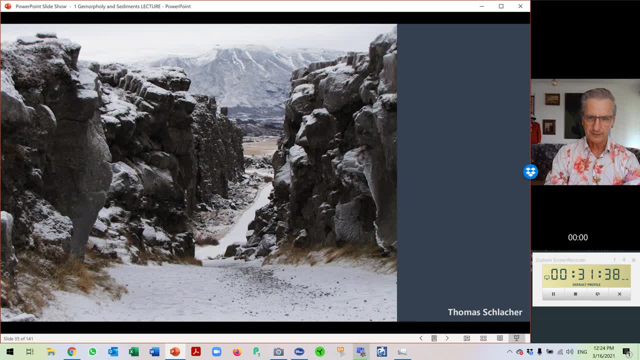 stainless steel room, and yep, the stainless steel room, and yep, the examination was not pleasant, that's all. examination was not pleasant, that's all. examination was not pleasant, that's all i can say. never mind, so don't carry. i can say never mind, so don't carry. 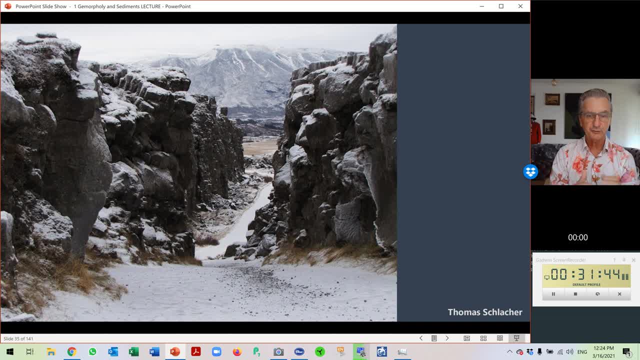 i can say: never mind, so don't carry stones in your pocket which you can't stones in your pocket, which you can't stones in your pocket, which you can't explain, or which you have a weird explain, or which you have a weird explain or which you have a weird explanation. no, no, i'm a scientist, i'm 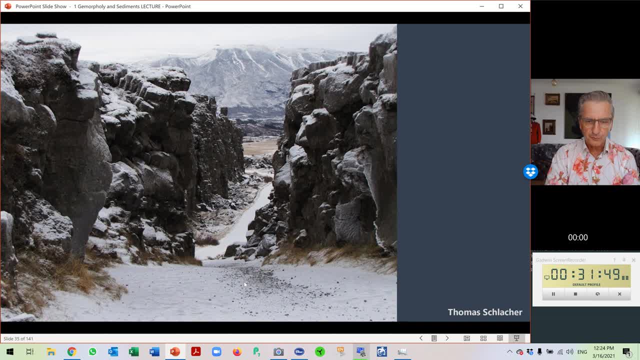 explanation: no, no, i'm a scientist. i'm explanation. no, no, i'm a scientist. i'm really yeah, i was really excited to pick. really yeah, i was really excited to pick. really yeah, i was really excited to pick up a few rocks on the mid-atlantic. 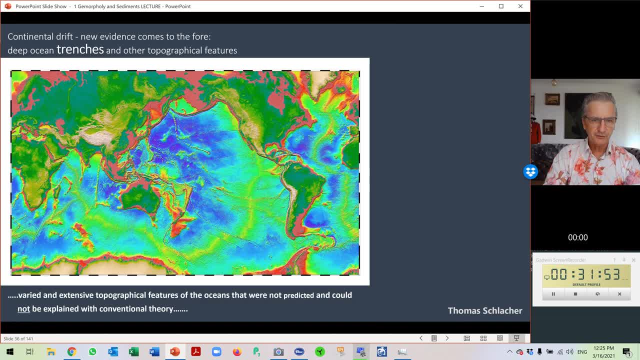 up a few rocks on the mid-atlantic, up a few rocks on the mid-atlantic. bridge, bridge, bridge. yeah right, any case, yeah right any case, yeah right, any case. the other thing which people couldn't, the other thing which people couldn't, the other thing which people couldn't really quite explain: where those deep? 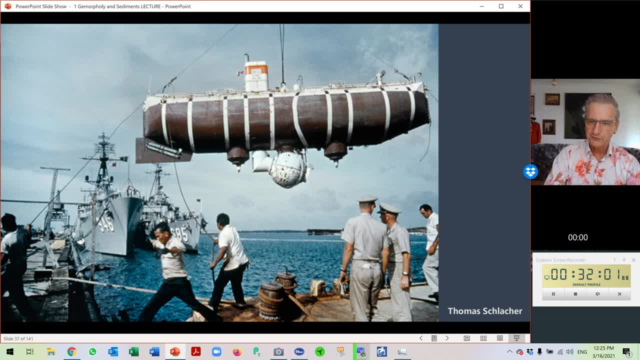 really quite explain where those deep, really quite explain where those deep sea trenches, sea trenches, sea trenches. if you are quite, this is a. if you are quite, this is a. if you are quite, this is a shot of the first betty's cape, basically. shot of the first betty's cape, basically. 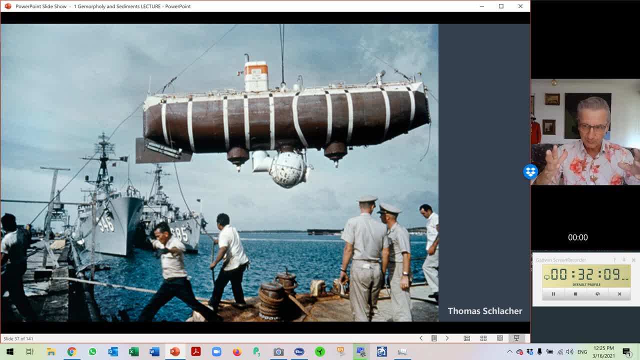 shot of the first betty's cape. basically a submarine which didn't have much a submarine which didn't have much, a submarine which didn't have much maneuverability. it was just a big block. maneuverability it was just a big block. maneuverability it was just a big block to actually go down as deep as was. 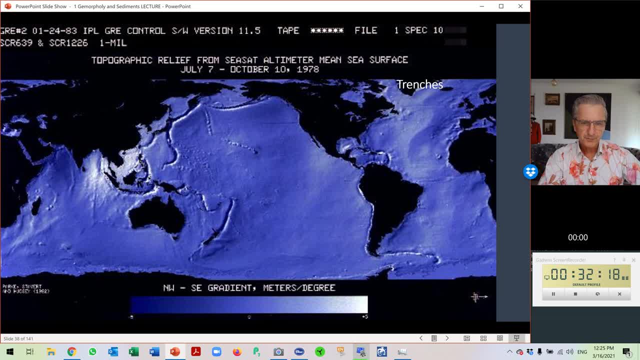 to actually go down as deep as was, to actually go down as deep as was possible at the time in the mariana, possible at the time in the mariana, possible at the time in the mariana, trench, trench, trench. and we in the pacific right in our 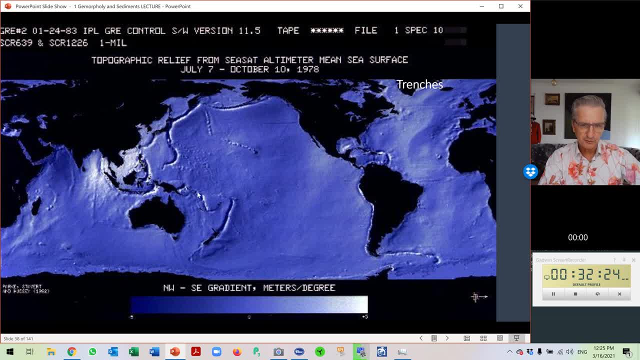 and we in the pacific right in our and we in the pacific right in our neighborhood have the biggest strangers neighborhood, have the biggest strangers neighborhood, have the biggest strangers in the world. the tonga camera track in the world, the tonga camera track in the world, the tonga camera track trench here. 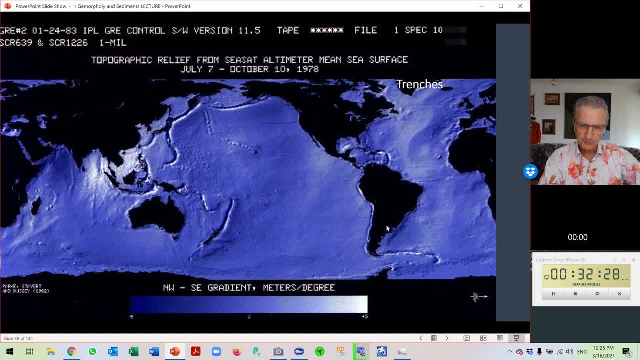 trench here, trench here, and then going up to the mariana, and then going up to the mariana and then going up to the mariana trench system. here you've got the chile trench system. here you've got the chile trench system. here you've got the chile trench to be up to rick range. but this: 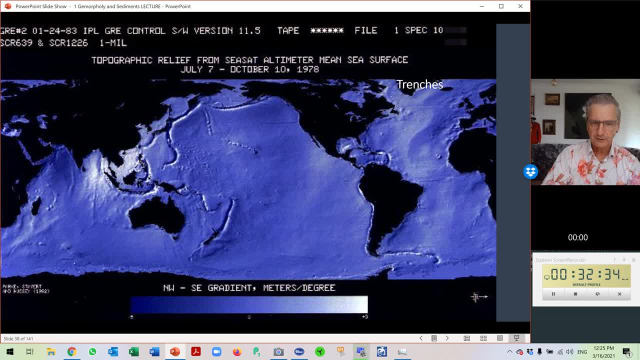 trench to be up to rick range, but this trench to be up to rick range, but this is basically where it goes down. all the is basically where it goes down. all the is basically where it goes down all the way to about 11 000 meters. 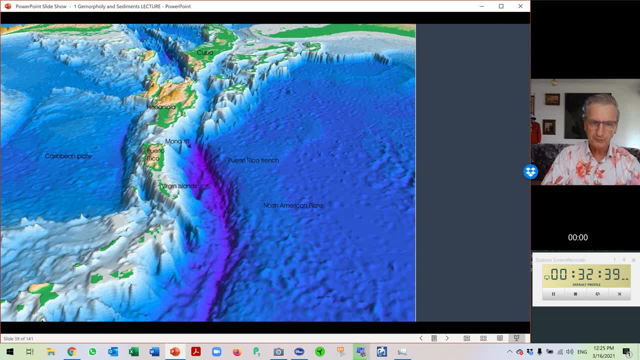 way to about 11 000 meters. way to about 11 000 meters. now people are usually here. you go to now people are usually here. you go to now people are usually here. you go to berkeley range. you know going down from berkeley range. you know going down from. 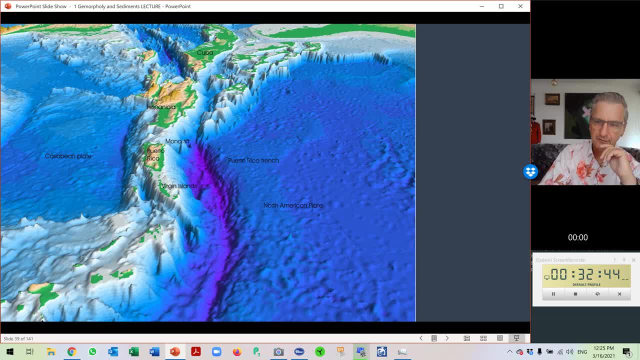 berkeley range, you know, going down from cuba towards cuba, towards cuba, towards the east, the east, the east, northeast tip of south america, northeast tip of south america, northeast tip of south america. here's our neighborhood, again you can. here's our neighborhood, again you can. 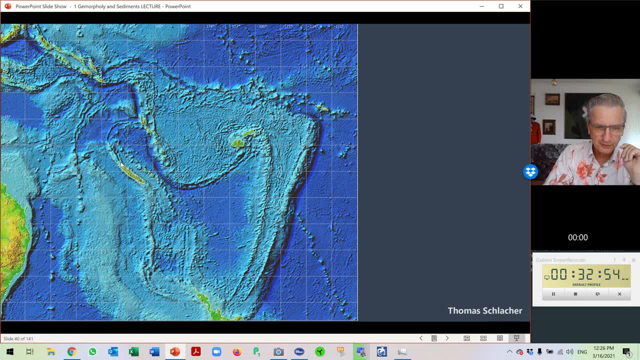 here's our neighborhood again. you can see, see, see. feature here in california. here there's a feature here in california. here there's a feature here in california. here there's a ridge system down here. but look at this ridge system down here. but look at this ridge system down here. but look at this massive deep trench going all the way up. 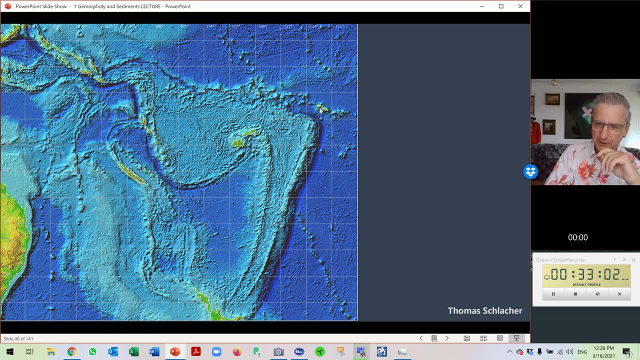 massive deep trench going all the way up, massive deep trench going all the way up here, here, here, it wants to go down from tonga and it wants to go down from tonga and it wants to go down from tonga. and you actually put out here like 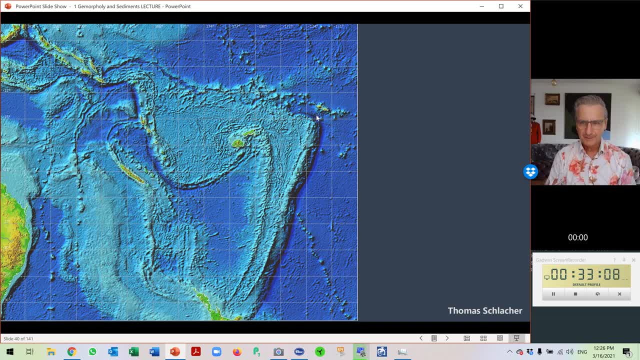 you actually put out here like, you actually put out here, like, and then you actually can feel, and then you actually can feel, and then you actually can feel how the swell changes the moment you go, how the swell changes the moment you go, how the swell changes the moment you go over. 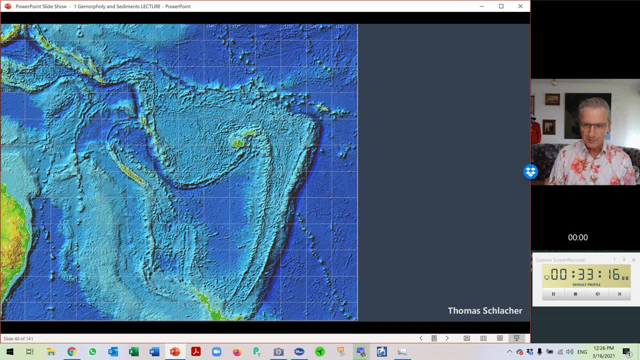 over, over 10 000 meters below you. it's literally 10 000 meters below you. it's literally 10 000 meters below you. it's literally like, like, like, like. it becomes deep blue, and as well it's. it becomes deep blue and as well it's. 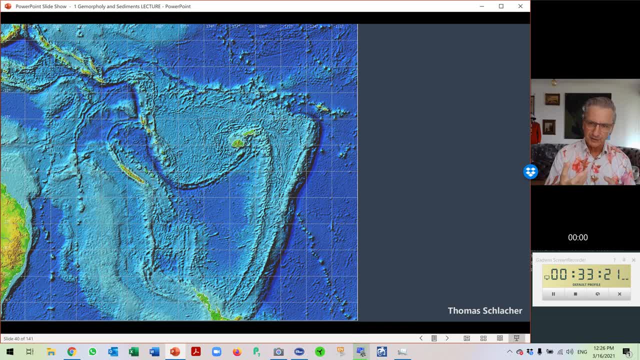 it becomes deep blue and as well. it's hard to describe, but hard to describe, but hard to describe. but if you actually spend time on boats, you, if you actually spend time on boats, you, if you actually spend time on boats, you, you get a feel for that, you kind of i. 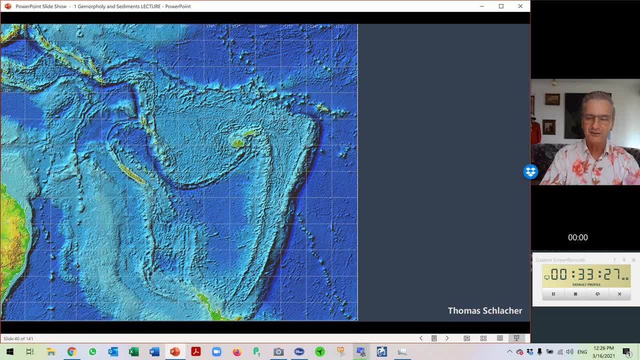 you get a feel for that, you kind of i. you get a feel for that, you kind of i mean i. i knew there was. you know a mean i. i knew there was. you know a mean i. i knew there was. you know a trench below us, but still. 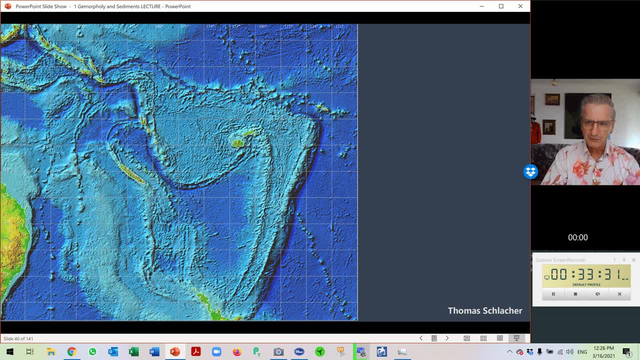 trench below us, but still trench below us, but still. most people actually said it was on an. most people actually said it was on an. most people actually said it was on an inter-island ferry. they would say inter-island ferry. they would say inter-island ferry. they would say it's a bit odd, you know, it's like well. 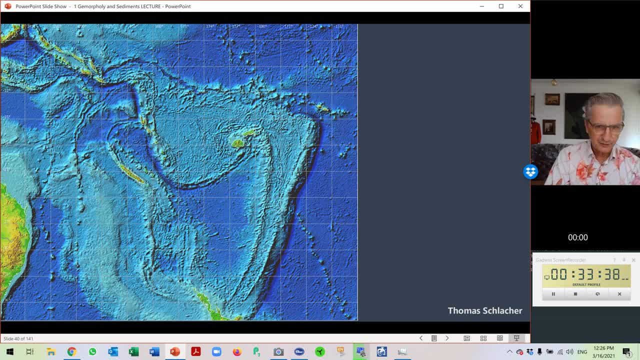 it's a bit odd, you know it's like: well, it's a bit odd. you know it's like: well, you know, because the water actually moves. you know because the water actually moves. you know because the water actually moves quite differently if it doesn't feel, quite differently if it doesn't feel. 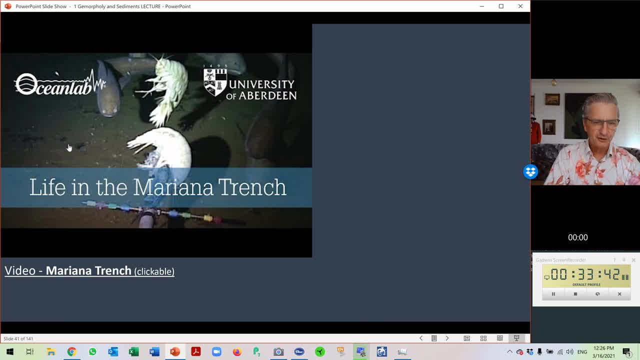 quite differently if it doesn't feel the bottom at all, the bottom at all, the bottom at all. now let's say, if you know, uh, have a look now. let's say, if you know, uh, have a look now. let's say, if you know, uh, have a look at people, always fascinated and say, oh what? at people always fascinated and say, oh what? at people always fascinated and say, oh what lives in deep sea trenches? well, yeah, lives in deep sea trenches. well, yeah, lives in deep sea trenches. well, yeah, a few very odd creatures or scavengers. a few very odd creatures or scavengers. 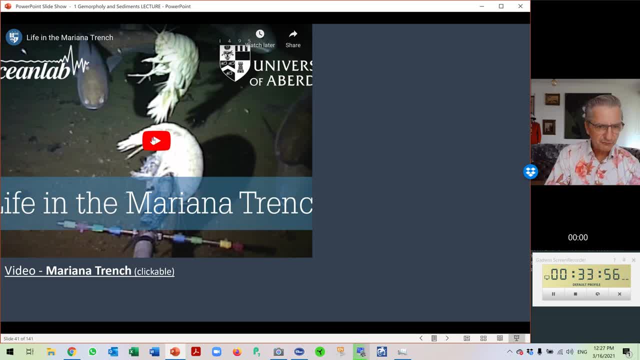 a few very odd creatures or scavengers um and my friend um and my friend um and my friend jamie jameson from you know other dean, jamie jameson from you know. other dean, jamie jameson from you know other dean you know and you know and. 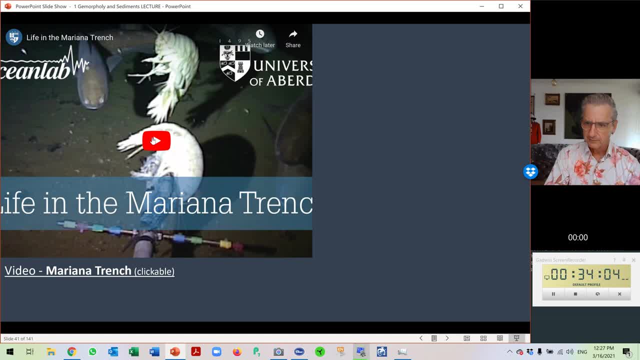 you know, and when you go to see with him, you know when you go to see with him, you know when you go to see with him, you know you have to actually, you have to actually, you have to actually make sure to leave enough space for, make sure to leave enough space for. 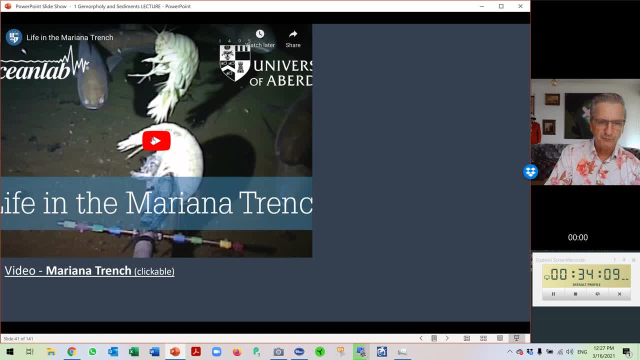 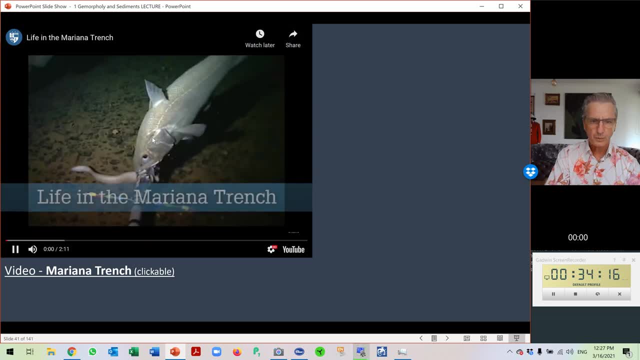 make sure to leave enough space for whiskey crates, whiskey crates, whiskey crates. um has actually built a. you know very, um has actually built a. you know very, um has actually built a. you know, very, very impressive career documenting this. so very impressive career documenting this. so very impressive career documenting this. so let's just have a look on that. 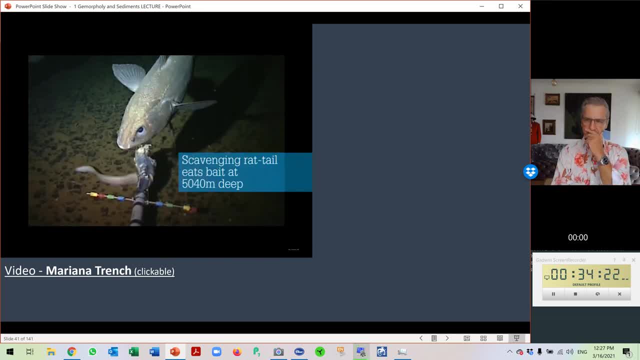 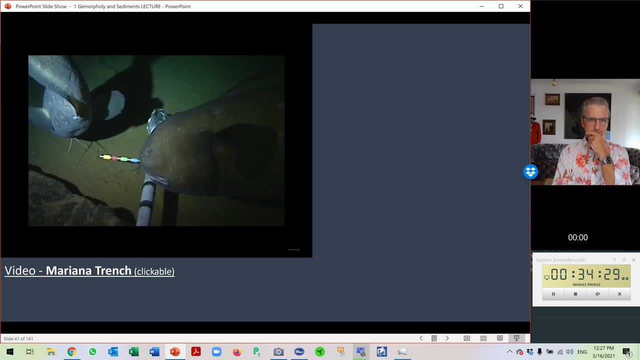 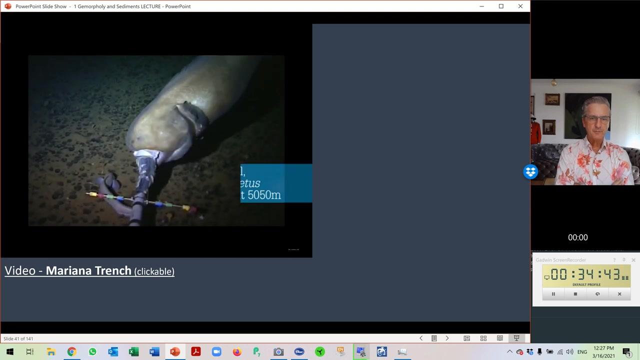 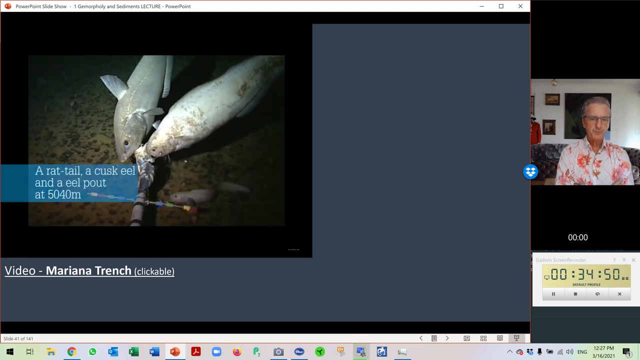 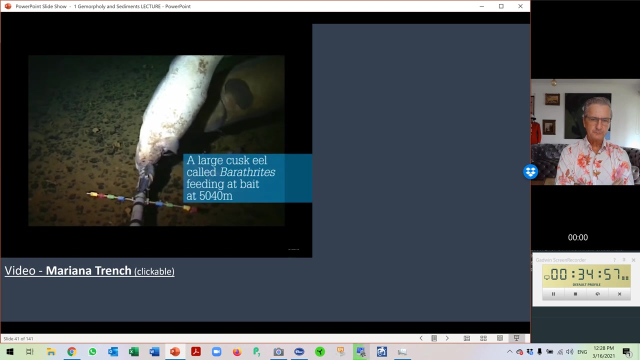 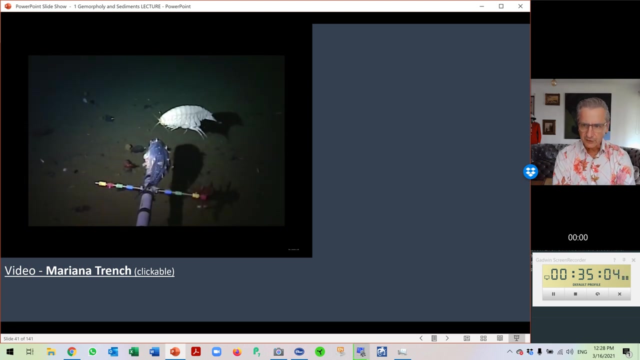 i don't quite know who actually chooses. i don't quite know who actually chooses. i don't quite know who actually chooses the music for that. the music for that, the music for that. this is an amphibody. this is an amphibody. this is an amphibody. i showed the amphibodes in the lecture on. 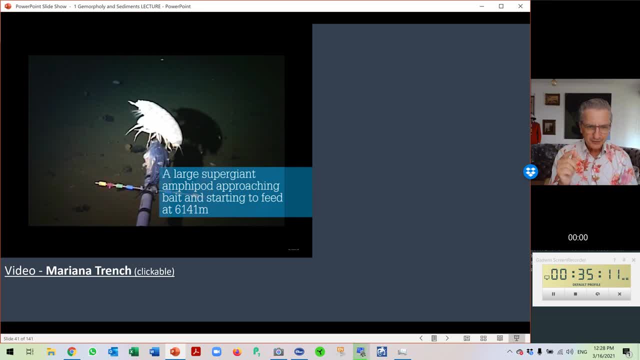 i showed the amphibodes in the lecture on. i showed the amphibodes in the lecture on center beaches being about center beaches being about center beaches being about a centimeter, a centimeter, a centimeter. this thing, this thing, this thing is dead, is dead, is dead size. 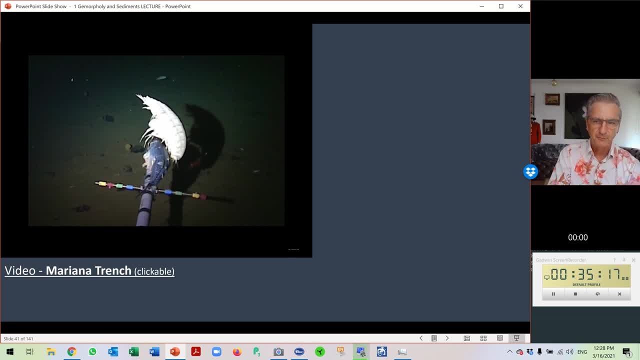 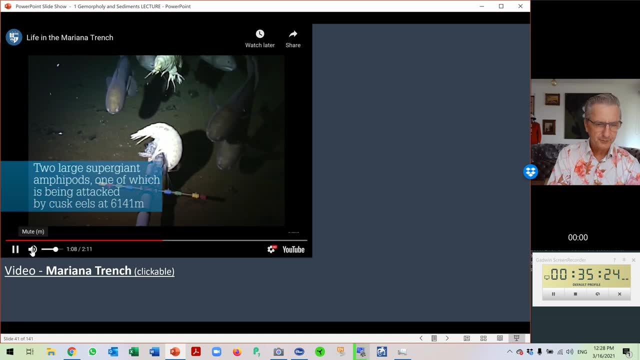 size, size. it's a four or five inches long. it's a four or five inches long. it's a four or five inches long. mess, mess, mess. there's a bit of a theory about, there's a bit of a theory about, there's a bit of a theory about gigantism in the deep sea. 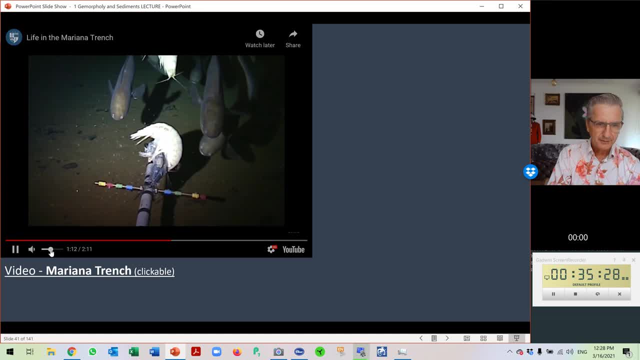 gigantism in the deep sea. gigantism in the deep sea. there's somebody who wrote paper about. there's somebody who wrote paper about. there's somebody who wrote paper about that. that that i can update, that i can update that. i can update that. but there's also. 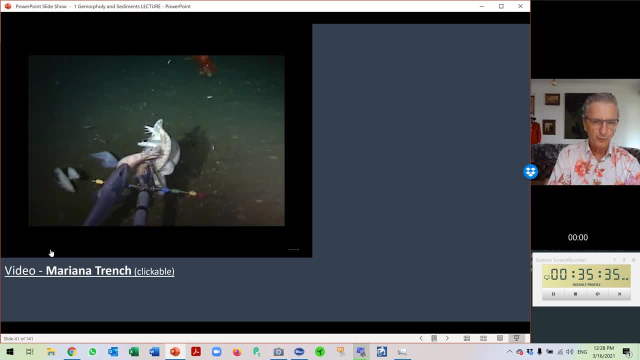 but there's also- but there's also complete evidence, complete evidence, complete evidence. small sizes, small sizes, small sizes. but there are several taxes which grow, but there are several taxes which grow, but there are several taxes which grow enormously, but there are several taxes which grow enormously large. 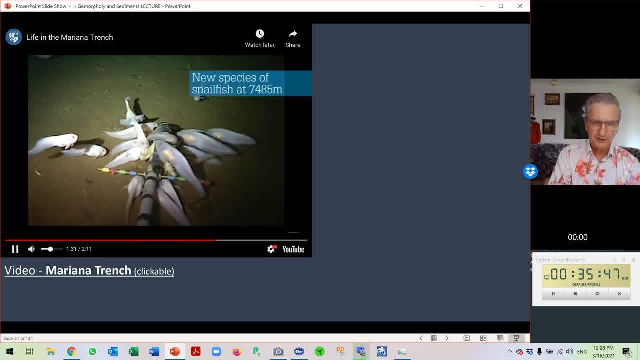 large, large environments, environments, environments- so just retails. retails are really so just retails. retails are really so just retails, retails. retails are really the funny fish that could stay fish, the funny fish that could stay fish, the funny fish that could stay fish with, basically. 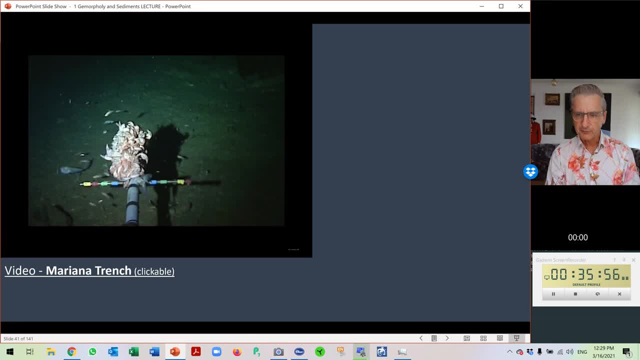 with basically with basically mackerels, mackerels, mackerels, because they've got a very soft flesh. so because they've got a very soft flesh, so because they've got a very soft flesh, so many actually get them out from. many actually get them out from. 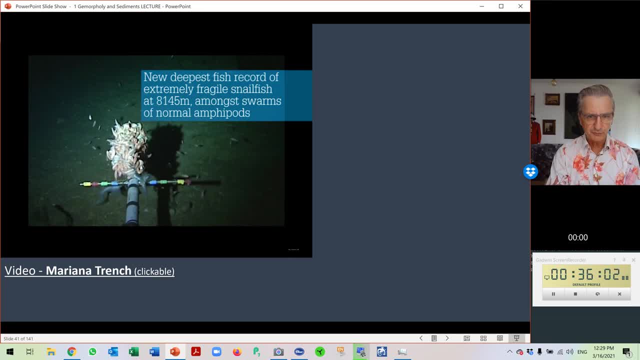 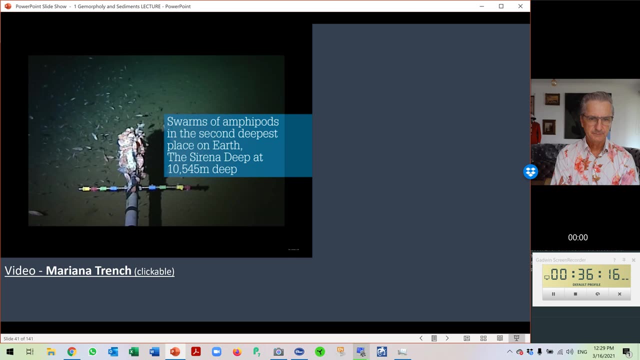 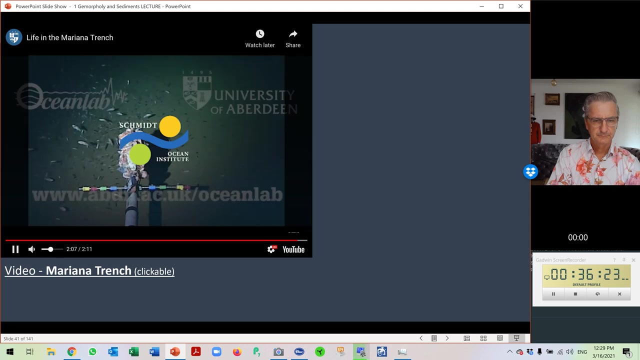 many actually get them out from the, the, the. you know from deep samples, you know from deep samples, you know from deep samples. oh, he actually says that. oh, he actually says that. oh, he actually says that, if i try to help you, here you go. oh, he actually says that, if i try to help you, here you go. 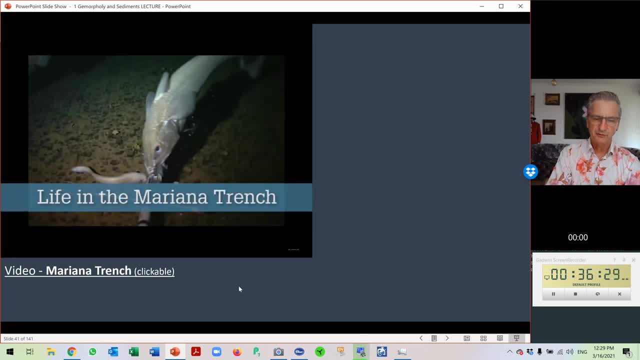 so, so, so, glide on. we got enormously big trenches. glide on, we got enormously big trenches. glide on, we got enormously big trenches in the deep sea, in the deep sea, in the deep sea. now this is a chart which actually shows. now, this is a chart which actually shows. 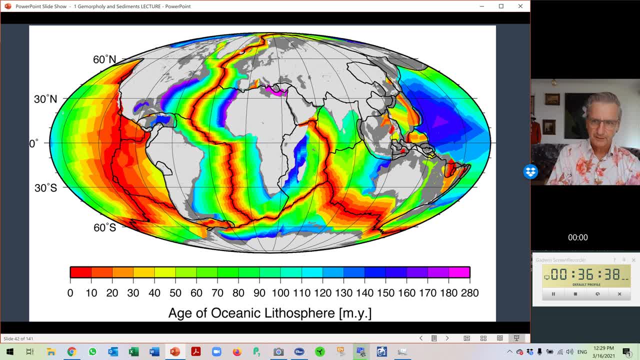 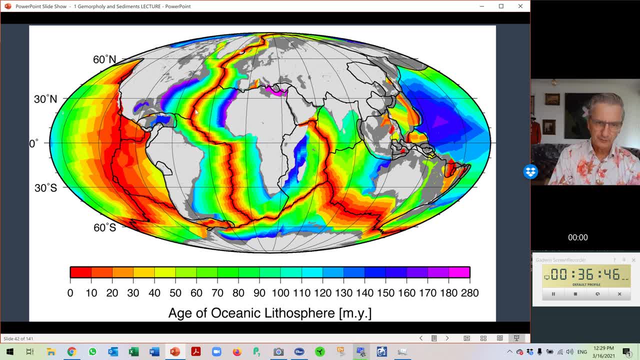 is is in the middle of the oceans, in the middle of the oceans, in the middle of the oceans, along the plate boundaries. the rock is along the plate boundaries. the rock is along the plate boundaries. the rock is literally, literally, literally fresh. that's got it extremely young. 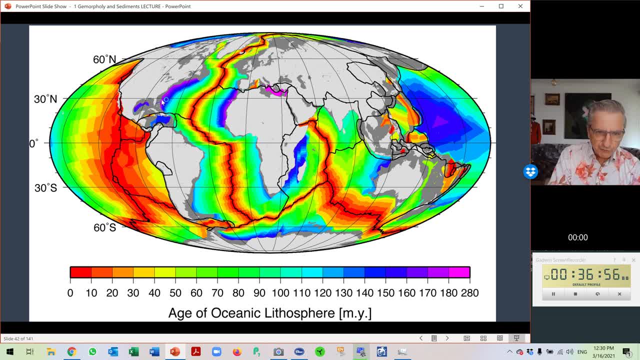 fresh, that's got it extremely young. fresh that's got it extremely young, right a few million years, right a few million years, right a few million years. and the further you move away and the further you move away and the further you move away, look along here, along the 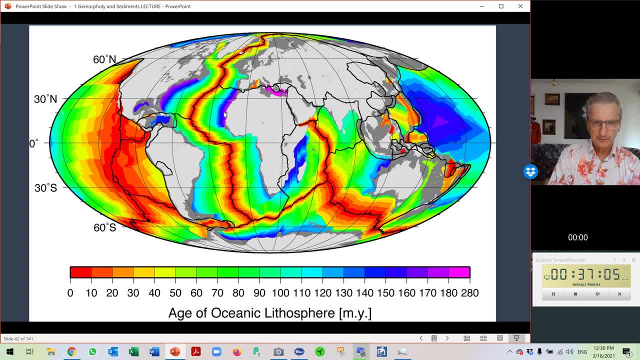 look along here, along, the look along here, along the eastern seaboard of the states, eastern seaboard of the states, eastern seaboard of the states, along the saharan, along the saharan, along the saharan, margin here, margin here, margin here, and also here in the middle of the. 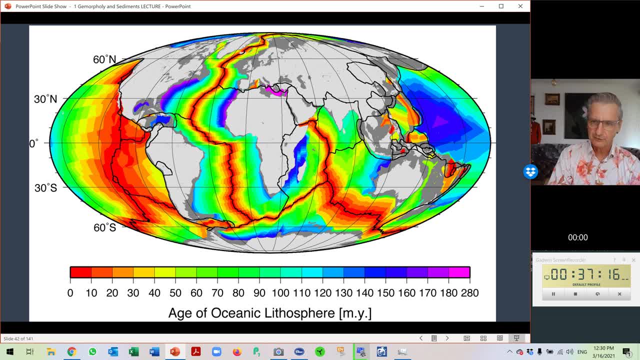 and also here in the middle of the, and also here in the middle of the pacific. it's very, very pacific. it's very, very pacific. it's very, very old. it's like the oldest one, so old, it's like the oldest one, so old, it's like the oldest one. so, basically, as you move away from, 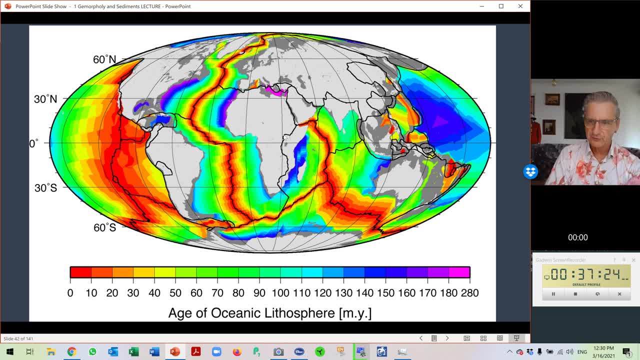 basically, as you move away from, basically, as you move away from the, the, the ridges and trenches, ridges and trenches, ridges and trenches, it actually gets, it actually gets. it actually gets younger, younger, younger, older and older, older and older, older and older now in our part of the world, as you can. 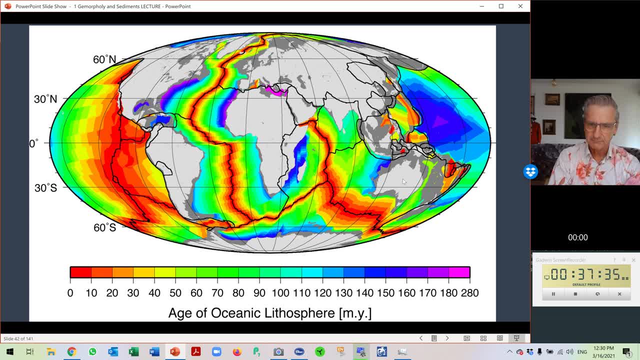 now in our part of the world, as you can now in our part of the world, as you can see, you know you're just right down the see. you know you're just right down the see. you know you're just right down the middle here and not having much happens. 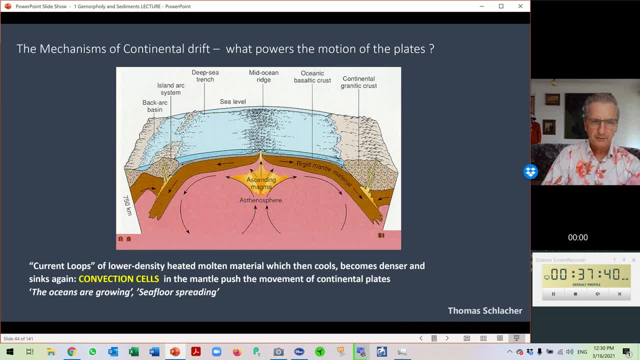 middle here and not having much happens, middle here and not having much happens at all, but it's mostly old at all, but it's mostly old at all, but it's mostly old now, now. now, the mechanism, the mechanism, the mechanism which, which, which makes blade boundaries, makes blade boundaries. 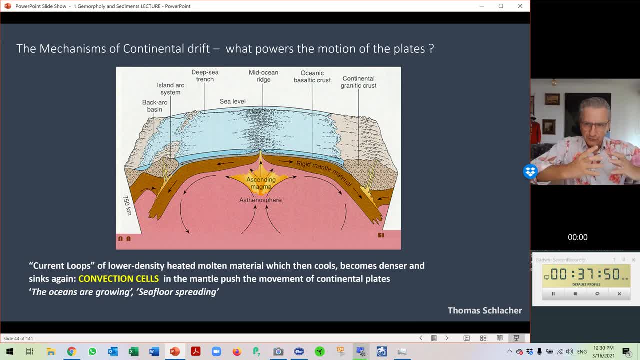 makes blade boundaries crack, crack, crack and which makes basically oceans basins and which makes basically oceans basins and which makes basically oceans basins to become bigger and bigger over time. to become bigger and bigger over time. to become bigger and bigger over time is something called sea flow spreading. 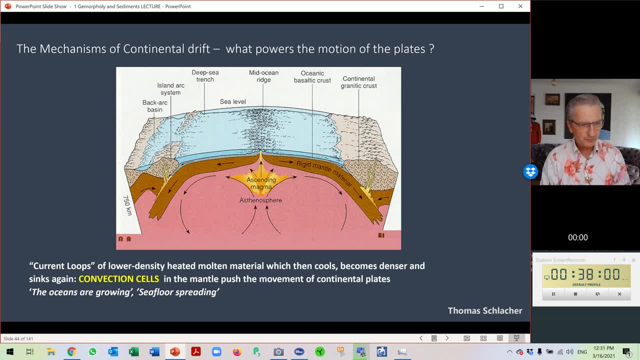 is something called sea flow spreading, is something called sea flow spreading? wire convection cells, wire convection cells, wire convection cells, now, now, now, you might actually think you know, if you might actually think you know, if you basically, you, basically, you basically jump off a cliff and there is no. 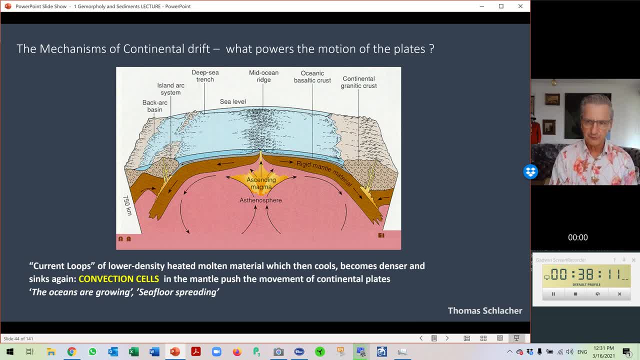 jump off a cliff, and there is no jump off a cliff and there is no ocean below you. rocks are very hard and ocean below you, rocks are very hard and ocean below you. rocks are very hard. and it will kill you, yes, it will. it will kill you, yes, it will. 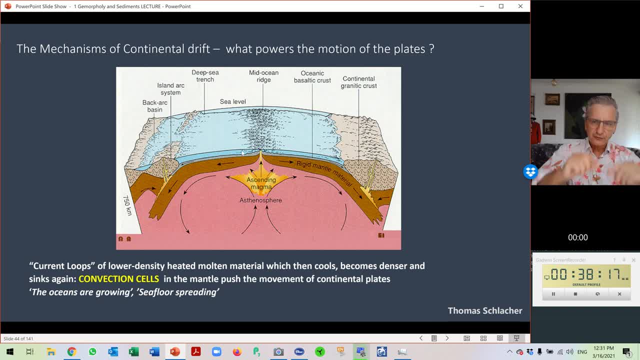 it will kill you. yes, it will. however, that hard bit of rock is just. however, that hard bit of rock is just. however, that hard bit of rock is just a very thin crust a few kilometers deep. a very thin crust a few kilometers deep, a very thin crust a few kilometers deep, and we, as humans, exist. 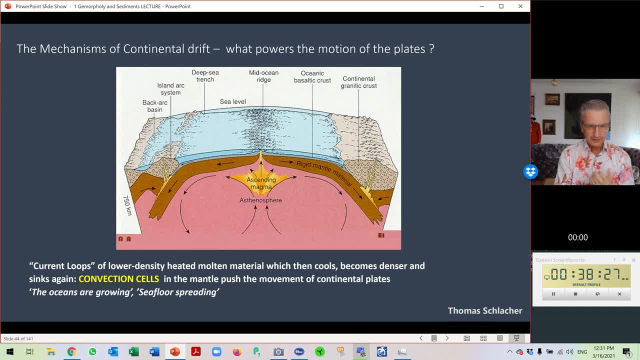 and we as humans exist, and we as humans exist on that crusty bit called on that crusty bit called on that crusty bit called basically, basically, basically. you know terrestrial, you know terrestrial, you know terrestrial. the continental grass, the continental grass, the continental grass floating on a semi-molten. 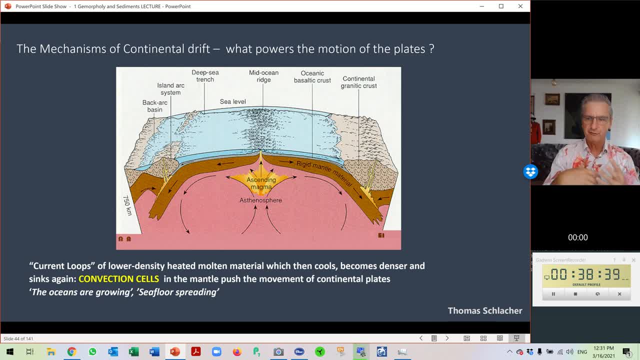 floating on a semi-molten. floating on a semi-molten in a huge ball of hot deformable rock, in a huge ball of hot deformable rock, in a huge ball of hot deformable rock. now, when you boil something, you usually. now, when you boil something, you usually. 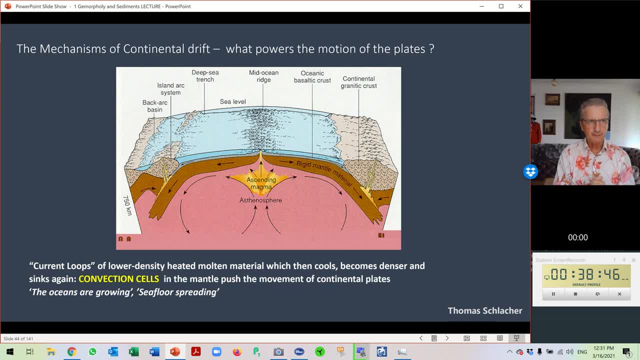 now, when you boil something, you usually get, get, get bubbles. if you boil bubbles, if you boil bubbles, if you boil custard, because what actually starts to happen, because what actually starts to happen, because what actually starts to happen is is is if there is heat from the core, and that 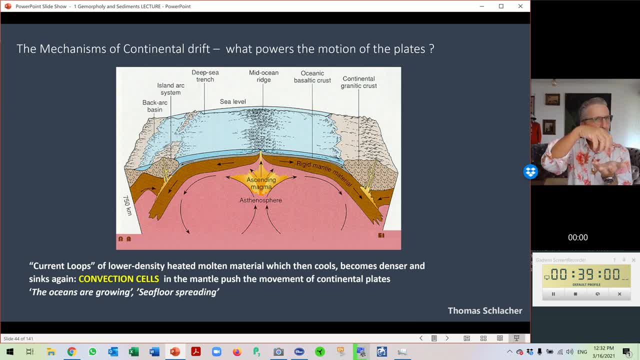 if there is heat from the core and that if there is heat from the core and that can be a hot plate on your stove can be a hot plate on your stove, can be a hot plate on your stove or it can be the core of the earth. 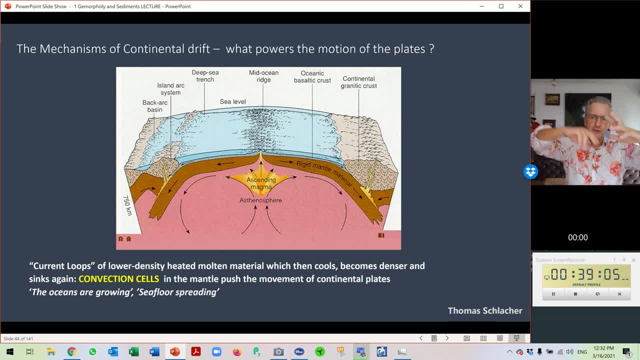 or it can be the core of the earth, or it can be the core of the earth. heat doesn't actually dissipate. heat doesn't actually dissipate, heat doesn't actually dissipate. you know uniformly, you know uniformly, you know uniformly: it actually, it actually, it actually gets. 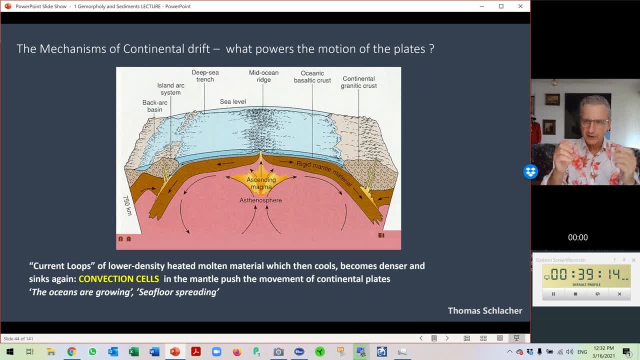 gets, gets it moves around. i should say in it moves around. i should say in it moves around. i should say in convection cells and that's why you get convection cells. and that's why you get convection cells and that's why you get when you basically boil a basic soup. 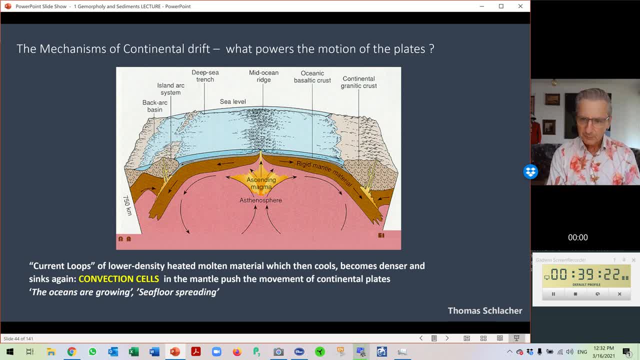 when you basically boil a basic soup, when you basically boil a basic soup- potato soup or custard, or whatever potato soup or custard or whatever potato soup or custard or whatever- and pretty much the same thing actually, and pretty much the same thing actually, and pretty much the same thing actually happens. 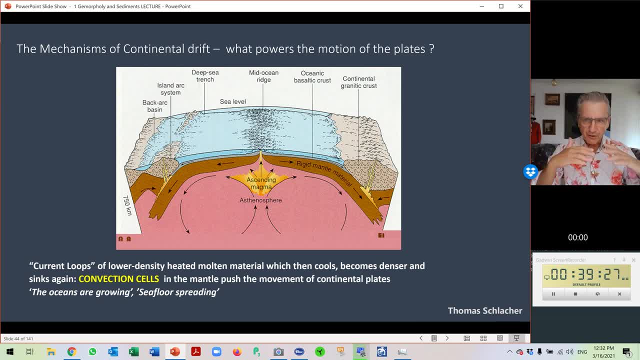 happens happens. very brittle but cold. very brittle but cold, very brittle but cold. solidified crust called the continental solidified crust, called the continental solidified crust, called the continental crust, or the oceanic plates doesn't crust, or the oceanic plates doesn't crust, or the oceanic plates doesn't really matter. 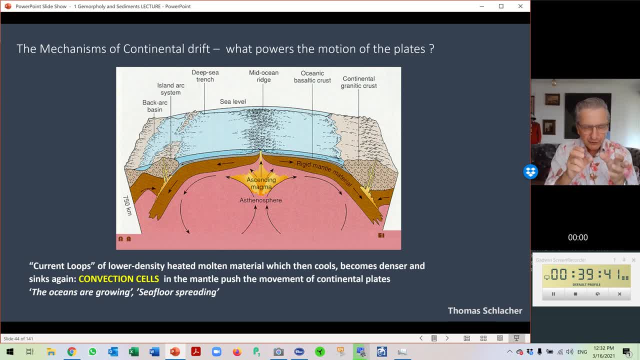 really matter, really matter. but below us, things are bubbling all the but below us things are bubbling all the but below us things are bubbling all the time and they're bubbling in the times time and they're bubbling in the times time and they're bubbling in the times that you know. at certain points, 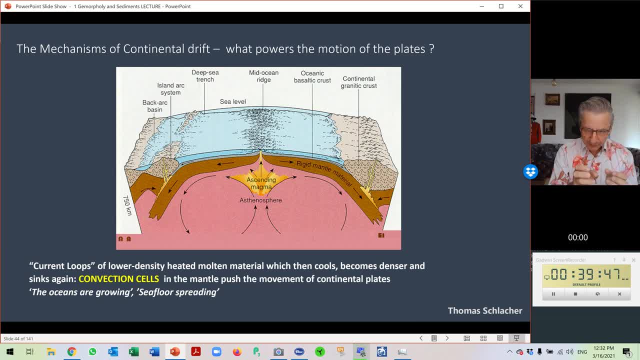 that you know at certain points, that you know at certain points along the earth, and this is along the along the earth, and this is along the along the earth, and this is along the plate boundaries, plate, boundaries, plate, boundaries: magna rises, magna rises, magna rises. now, most of it does not actually push. 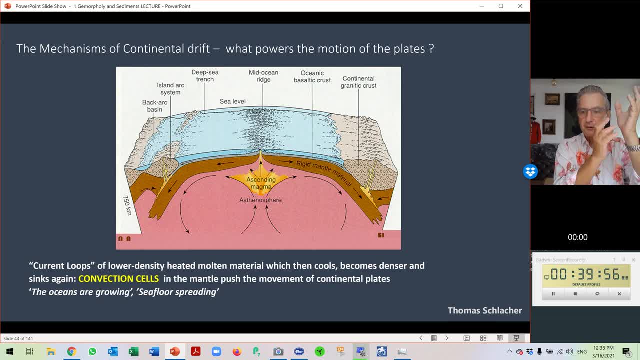 now, most of it does not actually push. now, most of it does not actually push out out out. they actually form little volcanoes. some they actually form little volcanoes. some they actually form little volcanoes. some of them do of them, do of them, do, and this is how we get all the islands in. 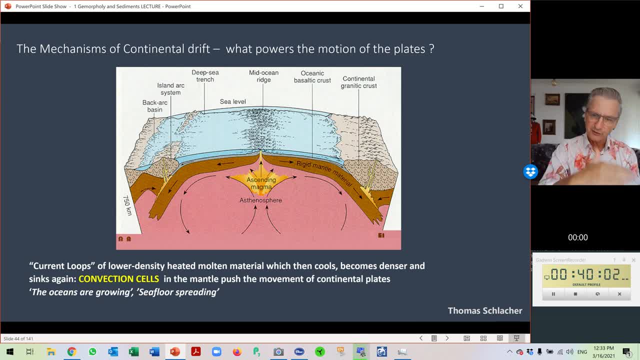 and this is how we get all the islands in, and this is how we get all the islands in the pacific, the pacific, the pacific, or most of them, except the coral echoes, or most of them, except the coral echoes, or most of them, except the coral echoes, which actually have 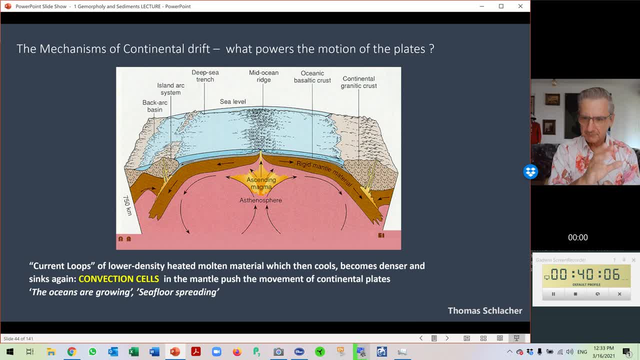 which actually have, which actually have a volcanic base at the bottom, and then a volcanic base at the bottom and then a volcanic base at the bottom, and then corals grow, corals grow, corals grow. but that top bit doesn't really matter all, but that top bit doesn't really matter all. 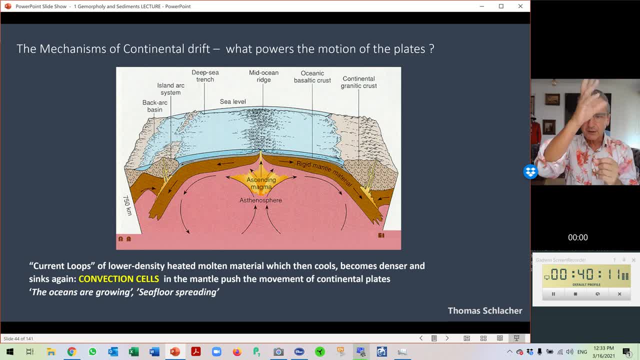 but that top bit doesn't really matter all that much from a geological point of that much from a geological point of that much from a geological point of view, view, view, some of them, you know, actually spurt out. some of them, you know, actually spurt out. 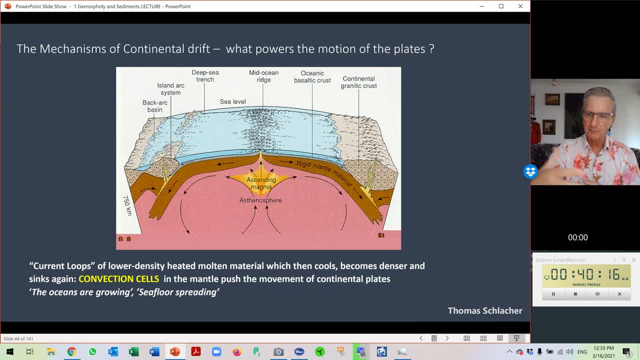 some of them, you know, actually spurt out lava. you get new islands forming in the lava. you get new islands forming in the lava. you get new islands forming in the pacific. you get pumice watching up on pacific. you get pumice watching up on. 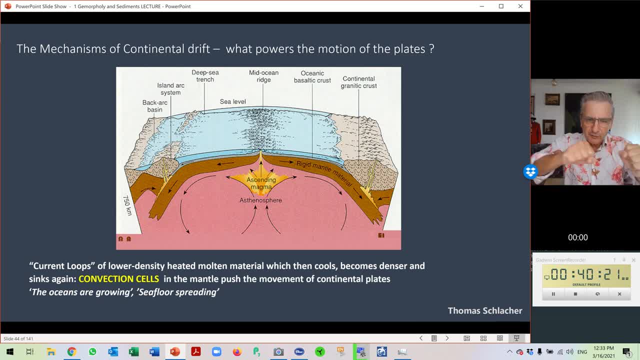 pacific, you get pumice watching up on our beaches, but most of it doesn't our beaches but most of it doesn't our beaches, but most of it doesn't actually come out. it actually moves, actually come out. it actually moves, actually come out. it actually moves sideways, sideways, under that same grass. 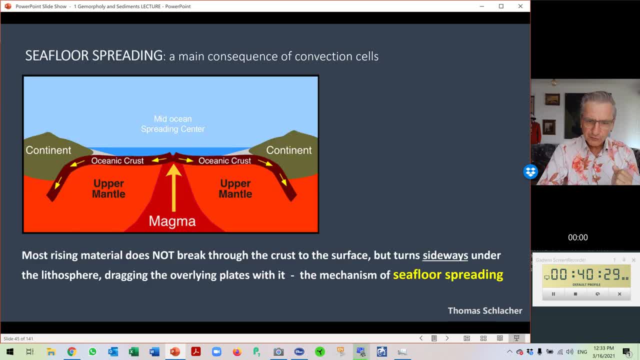 sideways, sideways, under that same grass, sideways, sideways, under that same grass called the mantle, called the mantle, called the mantle, and as it actually moves sideways, and as it actually moves sideways and as it actually moves sideways, it, it, it spreads the ocean basins apart by spreads the ocean basins apart by. 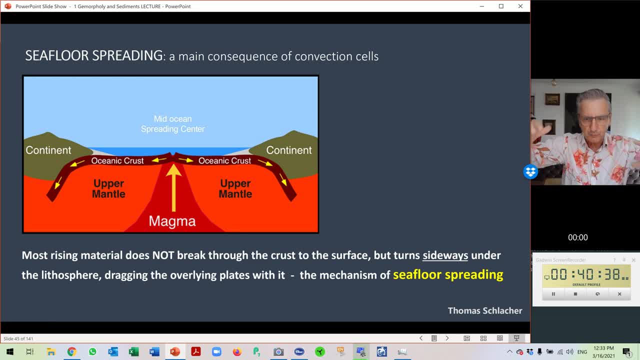 spreads the ocean basins apart by dragging, dragging, dragging that crusty material on top with that crusty material on top with that crusty material on top with- and that mechanism is called sea floor and that mechanism is called sea floor and that mechanism is called sea floor spreading. 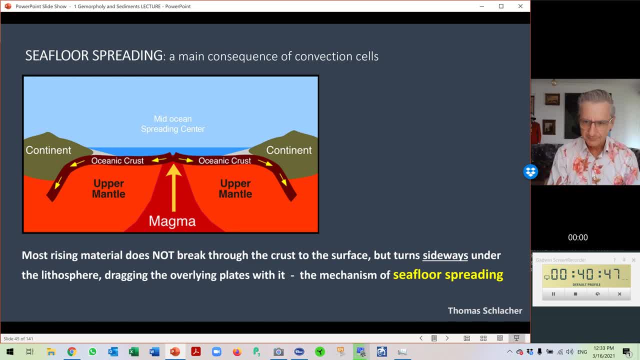 spreading, spreading, and it is seafloor spreading which can, and it is seafloor spreading which can, and it is seafloor spreading which can explain, explain, explain, and this is what we're gonna couldn't do, and this is what we're gonna couldn't do. 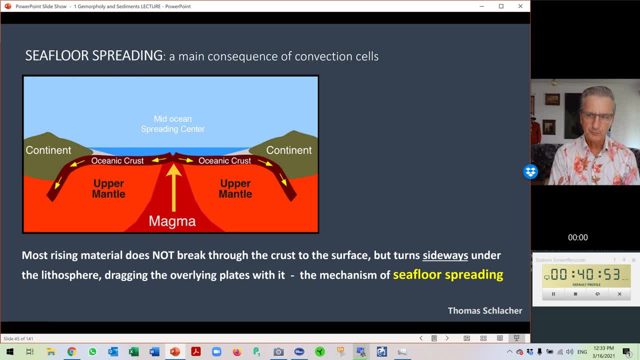 and this is what we're gonna, couldn't do, how the continental plates actually, how the continental plates actually, how the continental plates actually move, move, move about. so we have those bubble bubble about. so we have those bubble bubble about. so we have those bubble bubble bubble. convection cells. 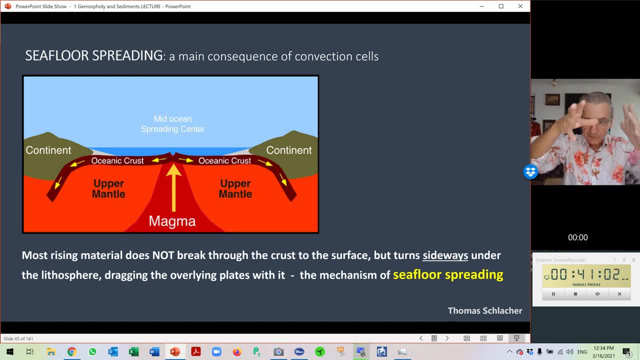 bubble convection cells. bubble convection cells. we live on a crusty bit below. we live on a crusty bit below. we live on a crusty bit below, basically on an odd think about an, basically on an odd think about an, basically on an odd think about an orange, and we are just a peel but the. 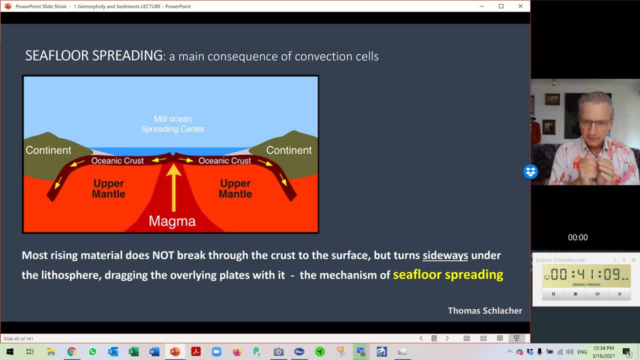 orange and we are just a peel, but the orange and we are just a peel, but the peel is hard, peel is hard, peel is hard. and inside the orange everything is, and inside the orange everything is, and inside the orange everything is boiling. there, we know. and then, like a 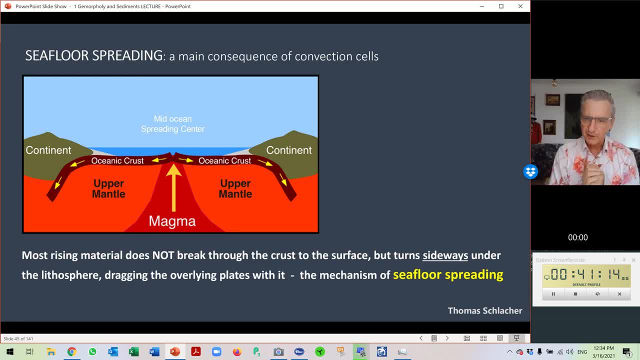 boiling there, we know. and then like a boiling there, we know. and then like a boop wants to come out and they all come. boop wants to come out, and they all come. boop wants to come out and they all come out along the plate boundaries but not. 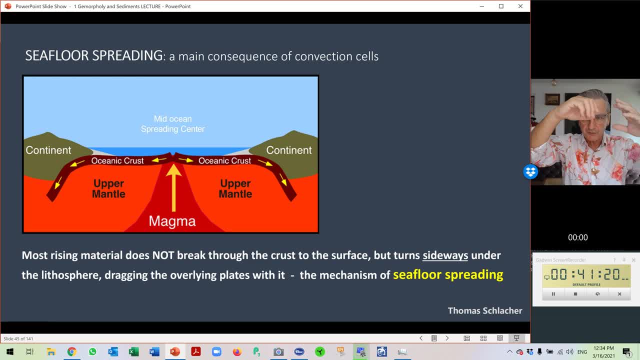 out along the plate boundaries but not out along the plate boundaries. but not terribly much material except the odd. terribly much material except the odd. terribly much material except the odd. island being formed comes out. most of it. island being formed comes out. most of it. island being formed comes out. most of it actually moves to the side and goes. 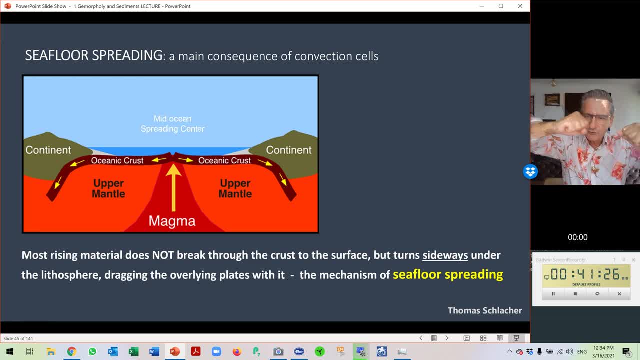 actually moves to the side and goes, actually moves to the side and goes down again, only to go like bloop again, down again, only to go like bloop again, down again, only to go like bloop again. and then it actually does that, and then it actually does that. 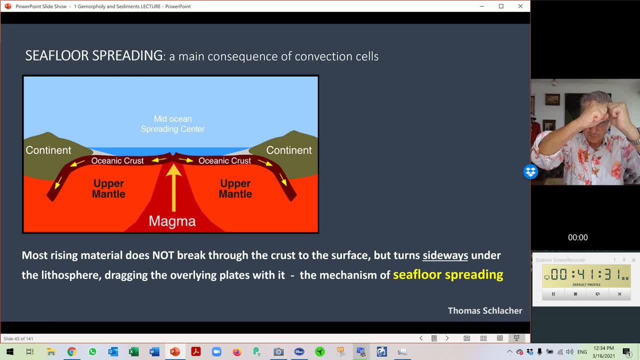 and then it actually does that. that is. that is, that is where new rock is formed in the middle, where new rock is formed in the middle, where new rock is formed in the middle and it actually drags the crust to and it actually drags the crust to. 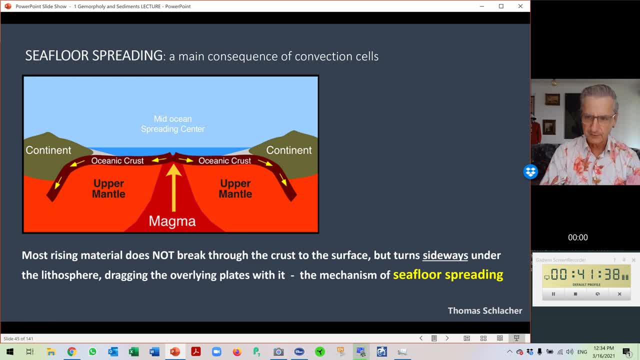 and it actually drags the crust to either side and creates the ocean basins either side and creates the ocean basins either side and creates the ocean basins ta-da, ta-da, ta-da, now, now, now, and of course, and of course, and of course, if you have new rock coming out from the 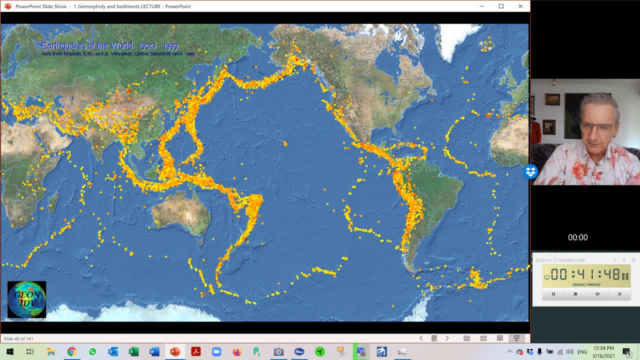 if you have new rock coming out from the, if you have new rock coming out from the middle of the earth, middle of the earth, middle of the earth, and trying to actually spread and trying to actually spread and trying to actually spread blade boundaries apart, blade boundaries apart. 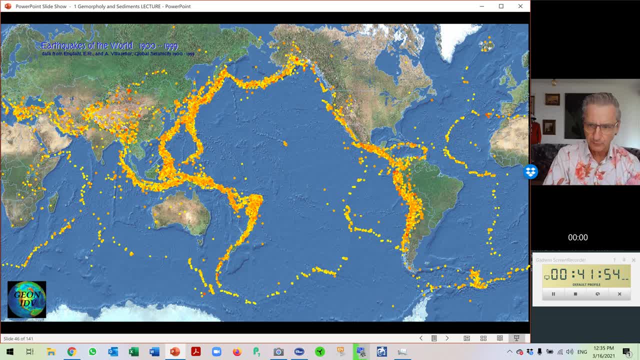 blade boundaries apart, it usually makes the earth shatter and it usually makes the earth shatter and it usually makes the earth shatter, and this is what we call you know this kind? this is what we call you. know this kind? this is what we call you. know this kind of. 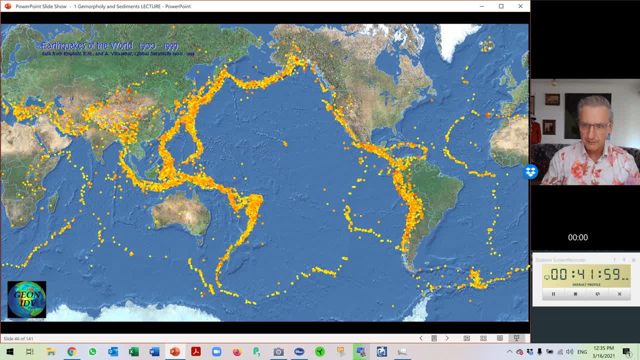 of of movement. movement- movement of the mantle where we sit, of the mantle where we sit, of the mantle where we sit- is basically an earthquake, is basically an earthquake, is basically an earthquake, and earthquakes follow blade boundaries and earthquakes follow blade boundaries and earthquakes follow blade boundaries to a remarkable degree, even here. look at: 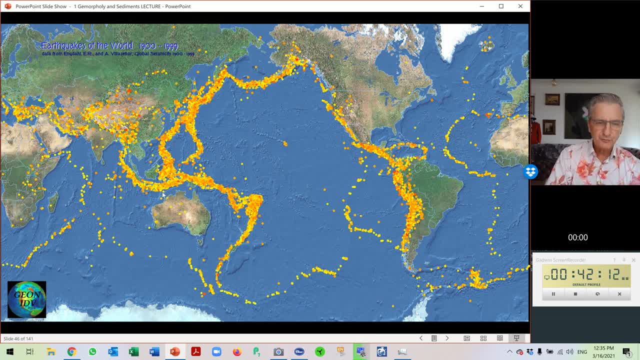 to a remarkable degree even here. look at to a remarkable degree even here. look at the hawaiian islands. you know we got that, the hawaiian islands. you know we got that, the hawaiian islands. you know we got that. and this actually explains, because we 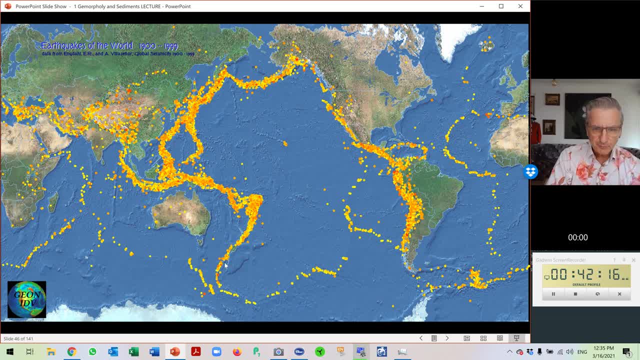 and this actually explains because we, and this actually explains because we sit in the middle of a big plate. but look, sit in the middle of a big plate. but look, sit in the middle of a big plate, but look at the pool, at the pool, at the pool. actually, new zealand is then going up to. 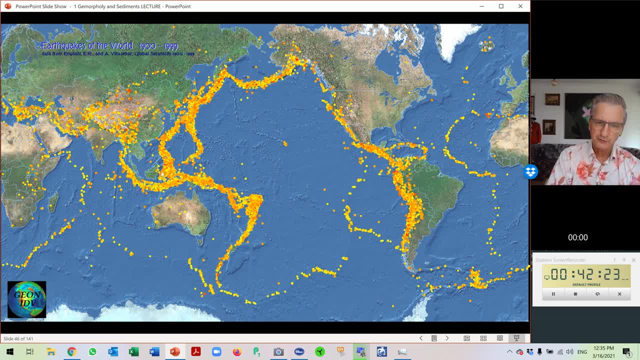 actually new zealand is then going up to actually new zealand, is then going up to tonga fiji and over into png, and so tonga fiji and over into png, and so tonga fiji and over into png and so forth, because this is where the blade 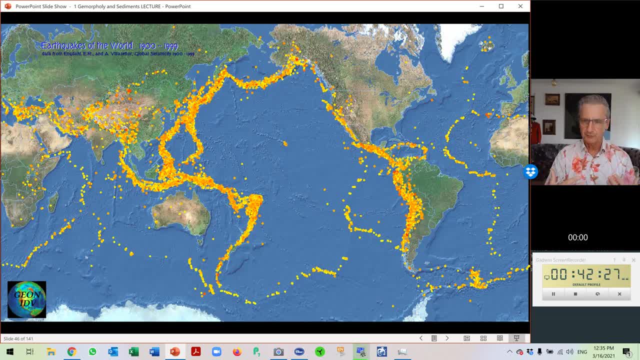 forth, because this is where the blade forth, because this is where the blade boundaries are. boundaries are, boundaries are, and what actually happens on blade and what actually happens on blade and what actually happens on blade, boundaries is, boundaries is boundaries- is either on divergent blades, either on divergent blades. 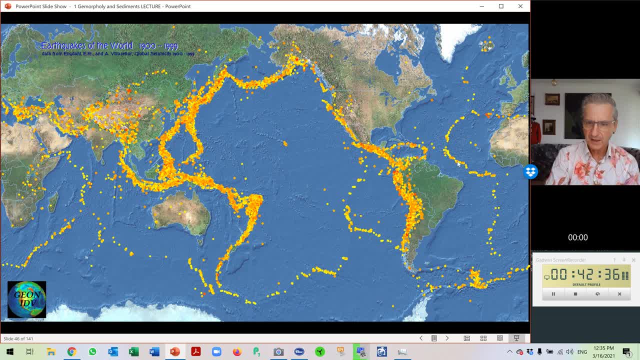 either on divergent blades- like here in the middle of the pacific, like here in the middle of the pacific, like here in the middle of the pacific- uh, the atlantic blades move apart, uh, the atlantic blades move apart, uh, the atlantic blades move apart- or they can actually meet each other as 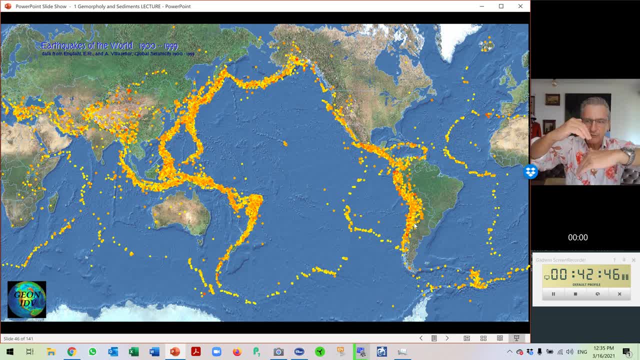 or they can actually meet each other as, or they can actually meet each other as happens here and here, and one blade happens here and here, and one blade happens here and here, and one blade dives under the other. in that case, this dives under the other. in that case, this: 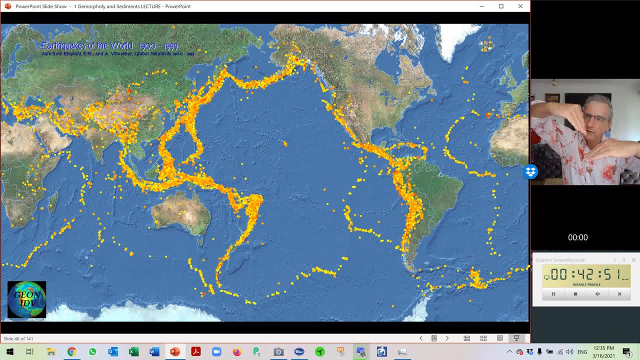 dives under the other. in that case, this is the pacific blade coming in, and it is the pacific blade coming in, and it is the pacific blade coming in and it dives under these are the andy mountains, dives under these are the andy mountains. 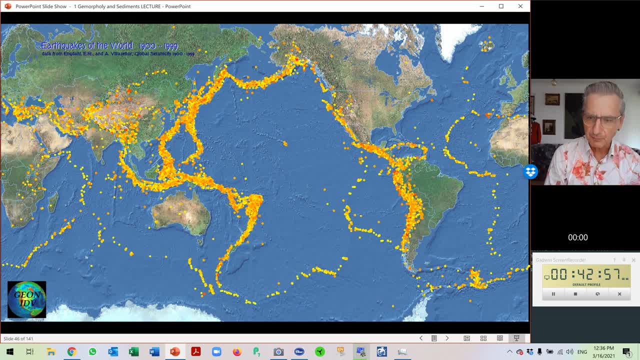 dives under. these are the andy mountains, and of course that kind of enormously, and of course that kind of enormously, and of course that kind of enormously large rubbing action, large rubbing action, large rubbing action causes earthquakes, and sometimes to such causes, earthquakes, and sometimes to such causes, earthquakes, and sometimes to such a degree that the land literally lifts. 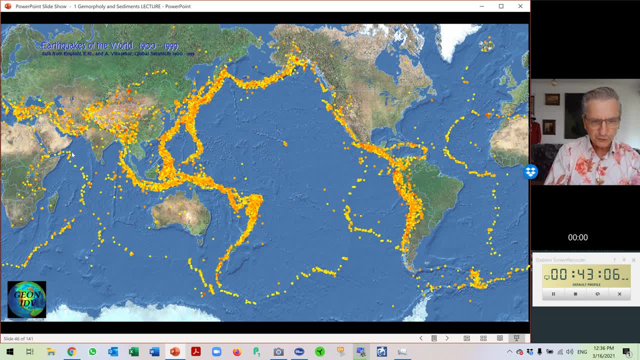 a degree that the land literally lifts, a degree that the land literally lifts a few meters up and down, and when it a few meters up and down, and when it a few meters up and down, and when it does so, does so, does. so has happened here during the christmas tsunami. you can. 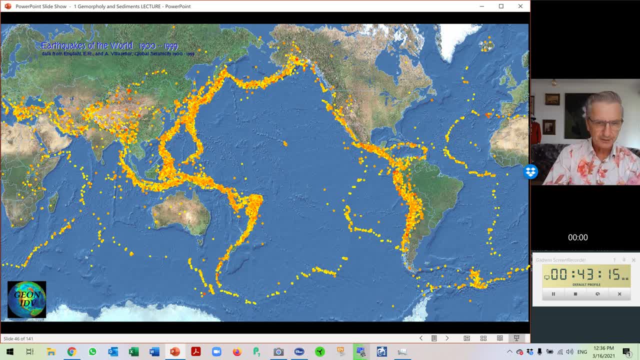 during the christmas tsunami. you can, during the christmas tsunami, you can actually get you know large water, actually get you know large water, actually get you know large water, movements and they create, you know movements and they create, you know movements and they create, you know, considerable destruction, considerable destruction. 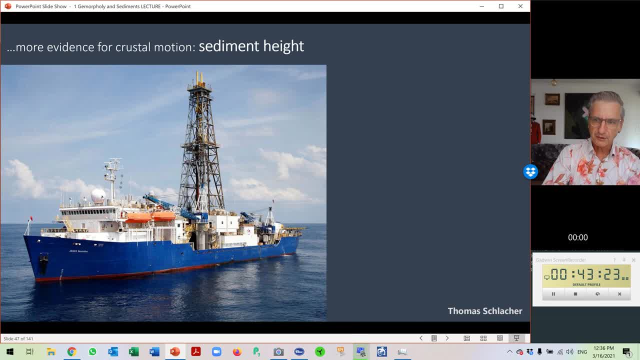 considerable destruction. another piece of evidence for another piece of evidence. for another piece of evidence for rock being created through seafloor. rock being created through seafloor. rock being created through seafloor spreading, spreading. spreading comes from measuring sediment. height comes from measuring sediment height. 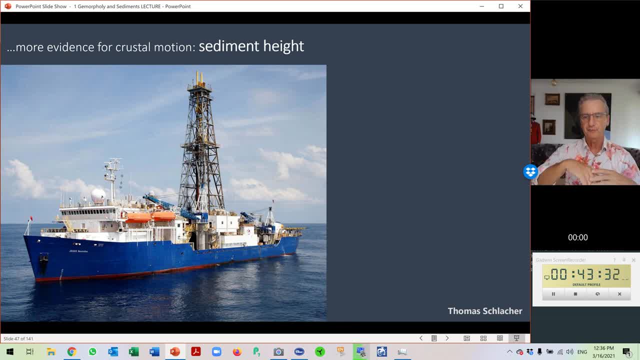 comes from measuring sediment height. this is the global challenger, and this is the global challenger and this is the global challenger and basically it's a research vessel. that basically it's a research vessel. that basically it's a research vessel that many nations play together and they run. 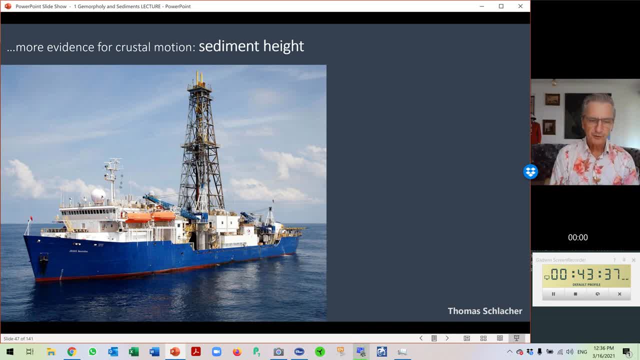 many nations play together and they run. many nations play together and they run around the walls and actually around the walls and actually around the walls and actually take deep trillings and actually study, take deep trillings and actually study, take deep trillings and actually study those cores. 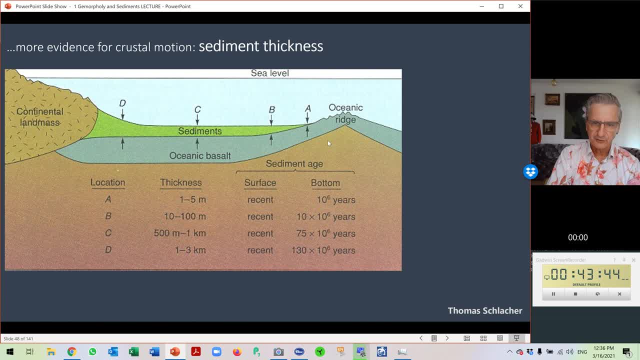 those cores, those cores, and we can actually work out from that. and we can actually work out from that and we can actually work out from that. you know what the average sediment, you know what the average sediment, you know what the average sediment. sickness is, sickness is, sickness is, and we get back to that in another. 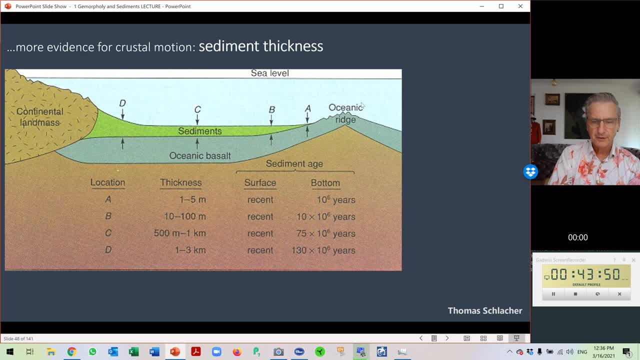 and we get back to that in another, and we get back to that in another lecture, lecture, lecture on sediments, specifically so on the on sediments, specifically so on the on sediments, specifically so on the oceanic ridges. we have, you know, almost oceanic ridges. we have, you know, almost. 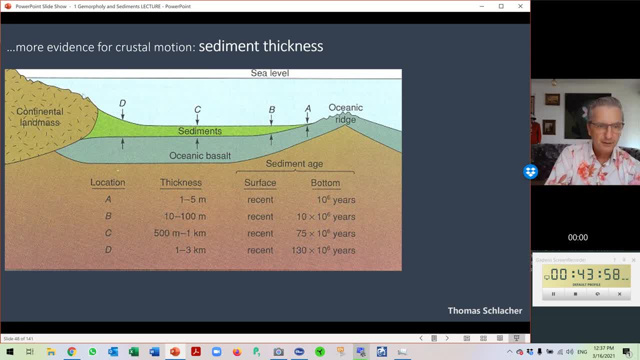 oceanic ridges, we have, you know, almost no sediment, because this is actually no sediment, because this is actually no sediment, because this is actually very young, very young, very young. the continental land masses: often they're the continental land masses, often they're the continental land masses, often they're basically. 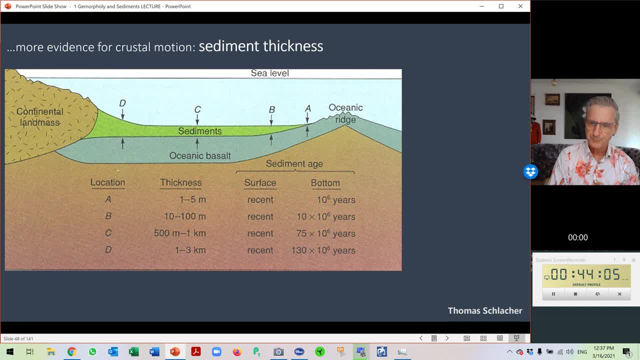 basically, basically weather and the particles. you know weather and the particles, you know weather and the particles you know, basically trundle down, basically trundle down, basically trundle down over the shelf, fall down into the deep over the shelf, fall down into the deep over the shelf, fall down into the deep basins and actually build up considerable. 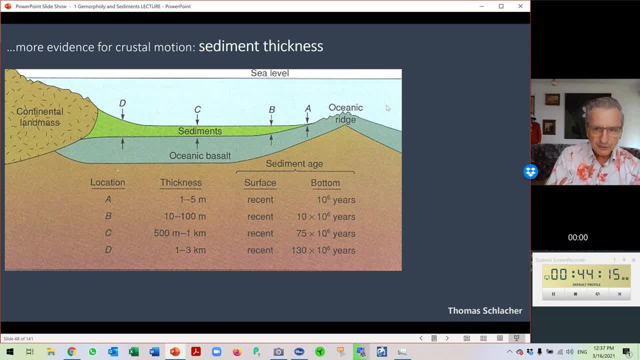 basins and actually build up considerable basins and actually build up considerable sediment, sediment, sediment deposits. but the key really is here: deposits. but the key really is here: deposits. but the key really is here: how young those rocks are because they. how young those rocks are because they. 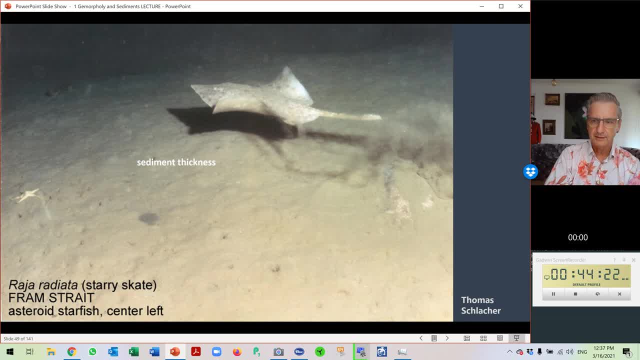 how young those rocks are, because they have not had time to accumulate sediments. the only uh difference is sediments. the only uh difference is sediments. the only uh difference is, basically, if you go to, basically, if you go to, basically, if you go to the middle of the ocean. often these are 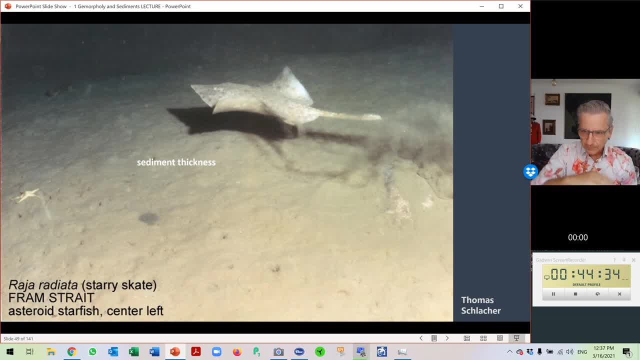 the middle of the ocean. often these are the middle of the ocean. often these are vast, vast, vast, very, very large, very, very large, very very large flat pieces called the abyssal plains and flat pieces called the abyssal plains and flat pieces called the abyssal plains, and they're actually covered. 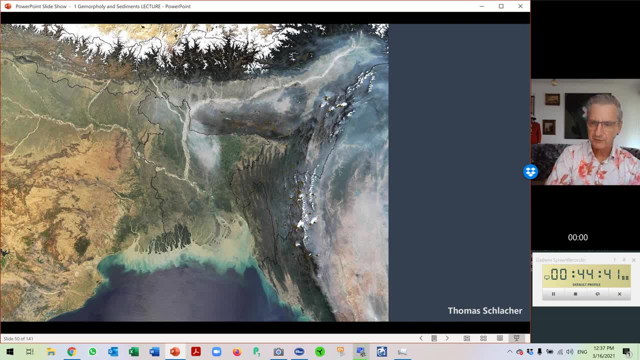 they're actually covered. they're actually covered by fine sediments, by fine sediments, by fine sediments. now those sediments come from. you know now those sediments come from. you know now those sediments come from. you know rivers that come from the sky, rivers that come from the sky. 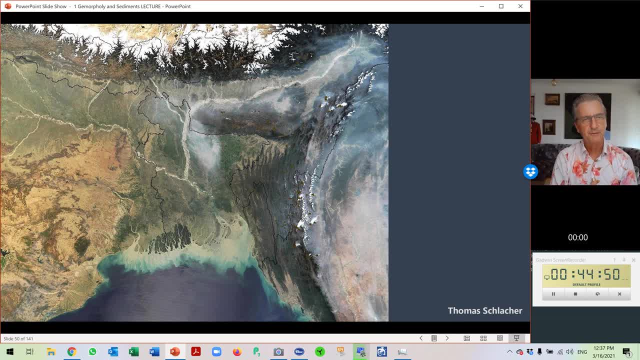 rivers that come from the sky. cosmic dust- it actually you know cosmic dust. it actually you know cosmic dust. it actually you know. contributes, about contributes, about contributes. about 10 to 30 tons of small particles, every 10 to 30 tons of small particles, every 10 to 30 tons of small particles every year. they come from volcanic eruptions. 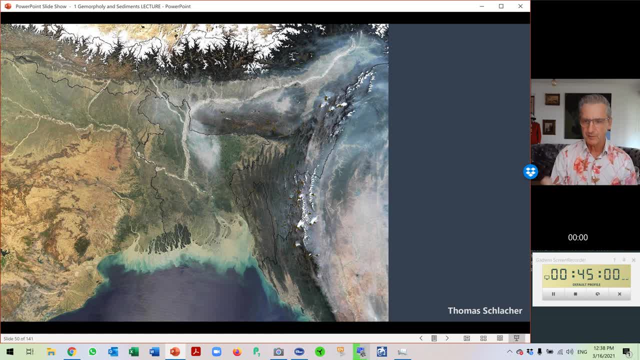 year. they come from volcanic eruptions year. they come from volcanic eruptions. agritas- they come from fires and they agritas. they come from fires and they agritas. they come from fires and they come actually from the remains of come actually from the remains of come, actually from the remains of animals, but most often it is actually. 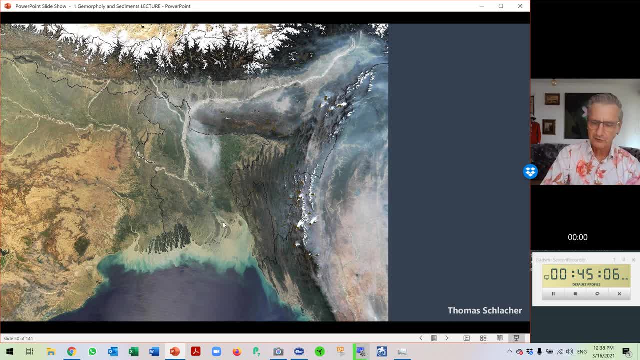 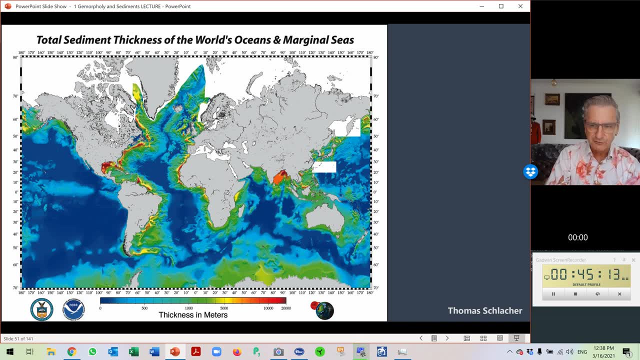 animals, but most often it is actually animals, but most often it is actually terrestrial material. terrestrial material, terrestrial material. what? because it is actually very, very what. because it is actually very, very what. because it is actually very, very fascinating for our purpose now. fascinating for our purpose now. 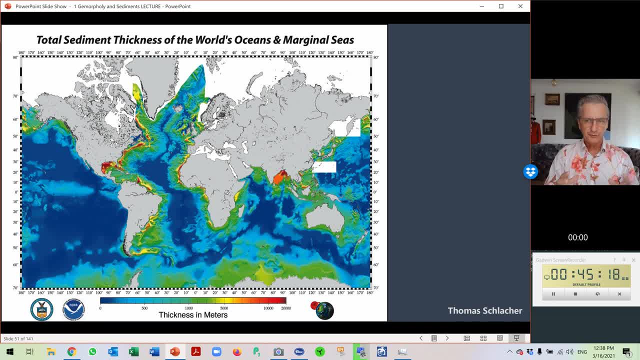 fascinating for our purpose. now you have to remember, if you have to remember, if you have to remember if ocean spreading really really happens. ocean spreading really really happens. ocean spreading really really happens. you would expect, you would expect, you would expect very, very little sediment in the middle of. 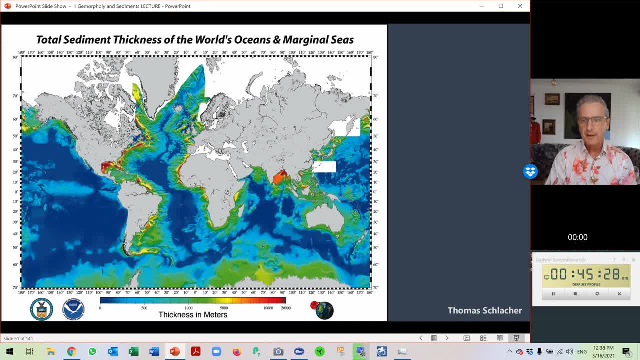 very, very little sediment in the middle of very, very little sediment in the middle of the ocean, because that's the ocean, because that's the ocean, because that's young and lots of it young and lots of it young and lots of it next to the continents, because they 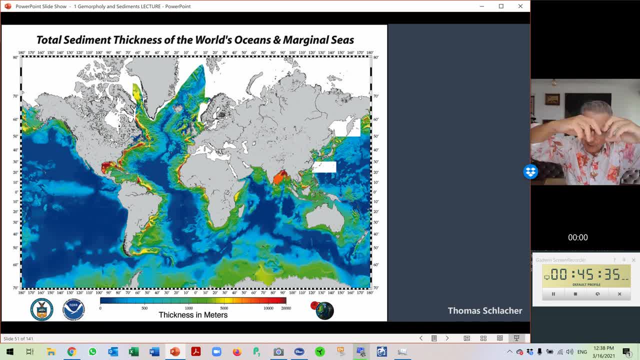 next to the continents, because they next to the continents, because they actually have been furthest away, so actually have been furthest away, so actually have been furthest away, so they must have been created earlier at. they must have been created earlier at. they must have been created earlier at some point in time and then just travel. 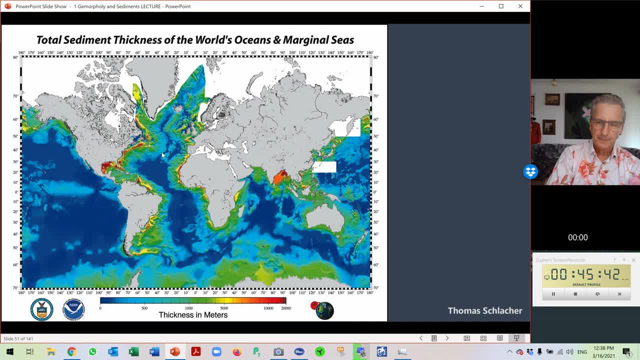 some point in time and then just travel some point in time and then just travel away, away, away. and this is exactly what happens at the and this is exactly what happens at the and this is exactly what happens at the continental margins. continental margins, continental margins kind of older and they had time to. 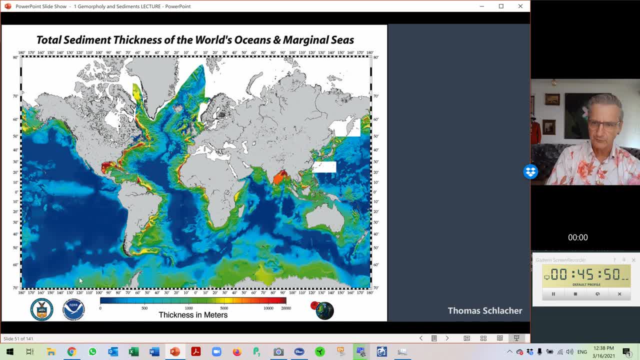 kind of older and they had time to kind of older and they had time to accumulate sediment, whereas in the accumulate sediment, whereas in the accumulate sediment, whereas in the middle of the oceans we actually have middle of the oceans, we actually have middle of the oceans, we actually have very 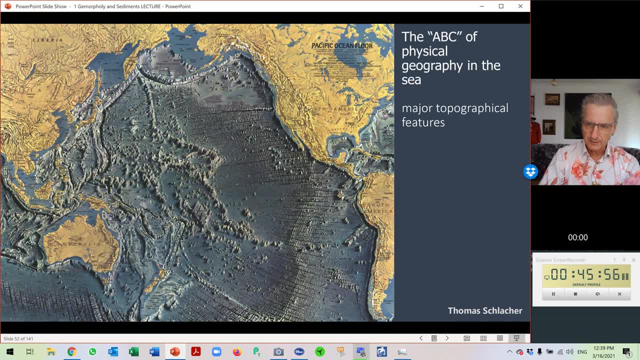 very, very little right, little right, little right, just in case, uh, i actually think, when, just in case, uh, i actually think, when, just in case, uh, i actually think, when you have a course, when you take a course, you have a course. when you take a course, you have a course when you take a course in marine biology or marine science, or 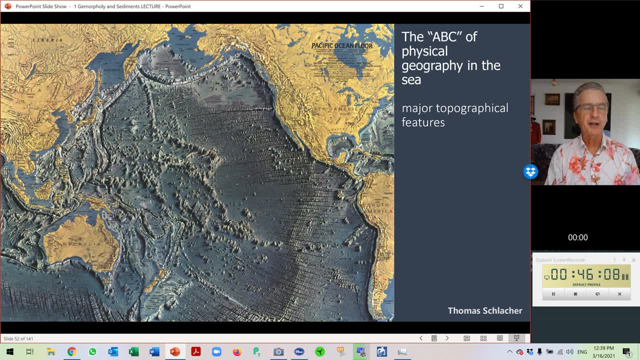 in marine biology or marine science, or in marine biology or marine science, or it's called, it's called, it's called coastal and marine ecology or whatever. coastal and marine ecology, or whatever coastal and marine ecology or whatever. biologically oceanography, biologically oceanography, biologically oceanography. you have to actually understand some of. 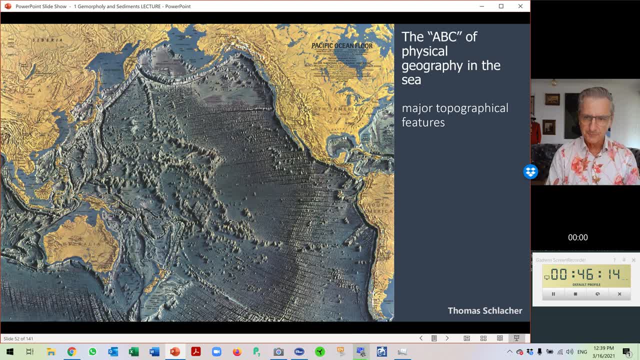 you have to actually understand some of you have to actually understand some of the terms which you might actually, the terms which you might actually the terms which you might actually encounter in your career, encounter in your career, encounter in your career. so i give you a little bit of an abc of 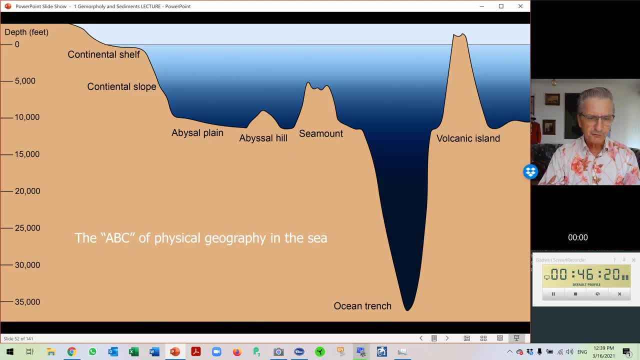 so i give you a little bit of an abc of. so i give you a little bit of an abc of physical geography here, physical geography here, physical geography here. the first thing you might actually note, the first thing you might actually note, the first thing you might actually note, is if you open a textbook, you know you. 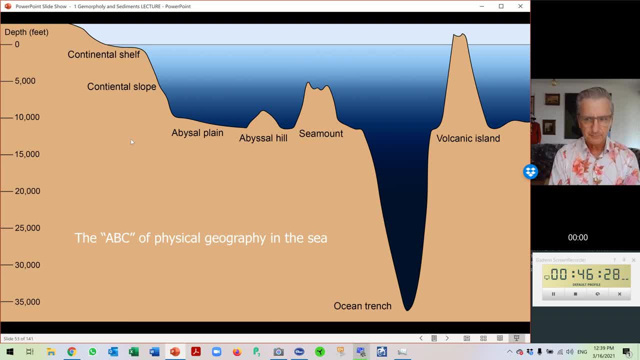 is. if you open a textbook, you know you is. if you open a textbook, you know you get something like this, get something like this, get something like this, and you go like um, do they actually? and you go like um, do they actually? and you go like um, do they actually really exist? you know, i mean everybody. 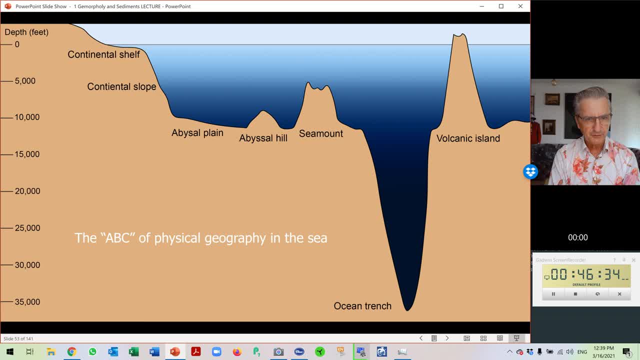 really exist. you know, i mean everybody really exist. you know, i mean everybody can control, can control, can control. you know a funny looking diagram, like you know a funny looking diagram. like you know a funny looking diagram like this, this, this, and if you start off fairly close to 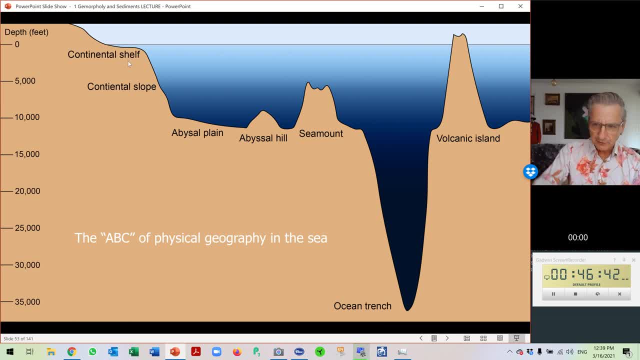 and if you start off fairly close to, and if you start off fairly close to the dry land, the dry land, the dry land, you hear about something like the. you hear about something like the. you hear about something like the continental shelf, continental shelf, continental shelf, the continental slope, maybe the 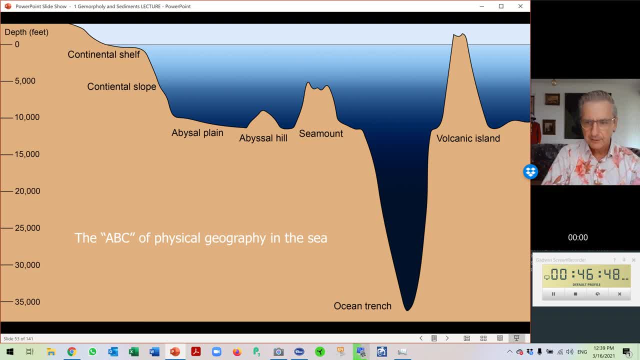 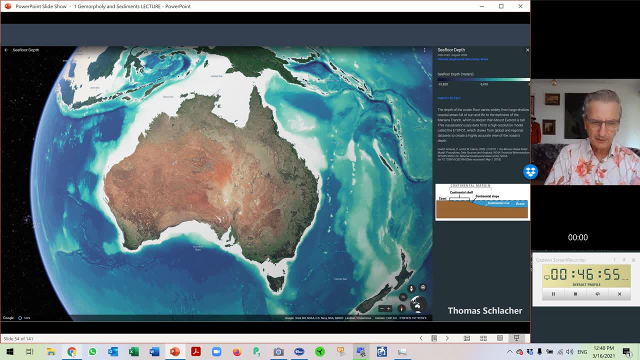 the continental slope, maybe the the continental slope, maybe the continental rise, and then the abyssal continental rise, and then the abyssal continental rise, and then the abyssal plane, plane, plane. let's actually examine this for a minute. let's actually examine this for a minute. let's actually examine this for a minute. now again, we can go back to. 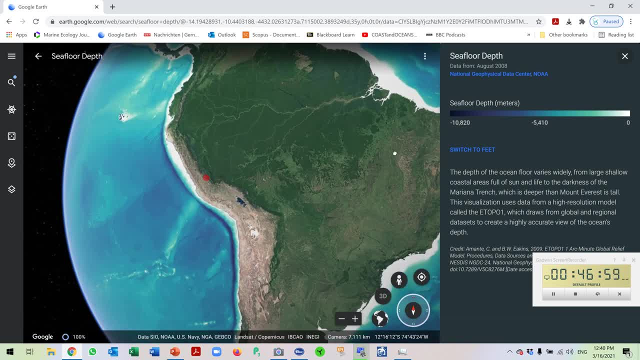 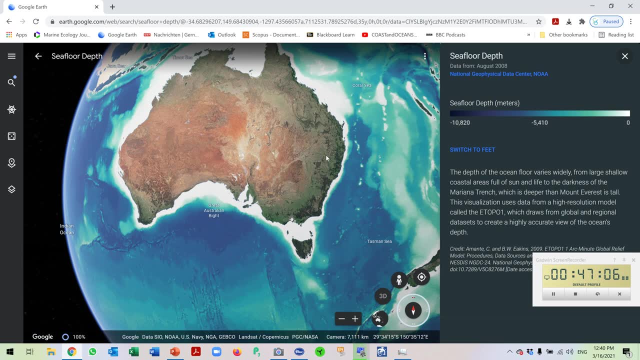 now again we can go back to now again. we can go back to taking your life here, to get over here, get over here, get over here, taking your life here to australia and taking your life here to australia. and taking your life here to australia and what you can see here. 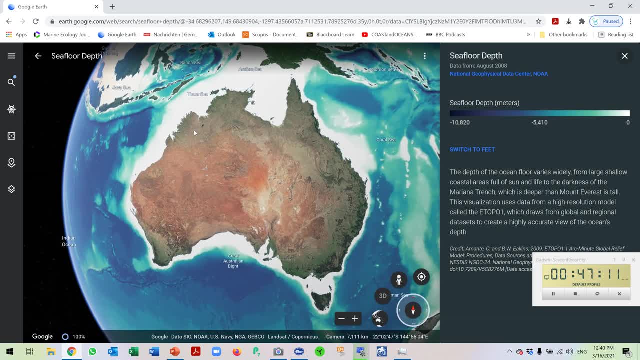 what you can see here, what you can see here- and i think this is quite fascinating, and i think this is quite fascinating, and i think this is quite fascinating really- is really, is really is. well, the true boundary of australia is a. well, the true boundary of australia is a. 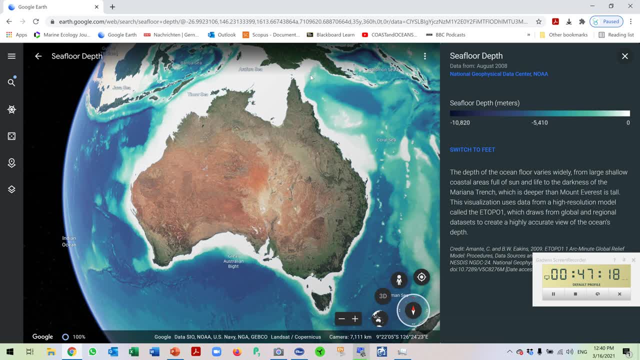 well, the true boundary of australia is a few hundred kilometers out to sea, up few hundred kilometers out to sea, up few hundred kilometers out to sea, up here, here, here, and, and, and in the taurus strait, in the taurus strait, in the taurus strait, where we actually live around. 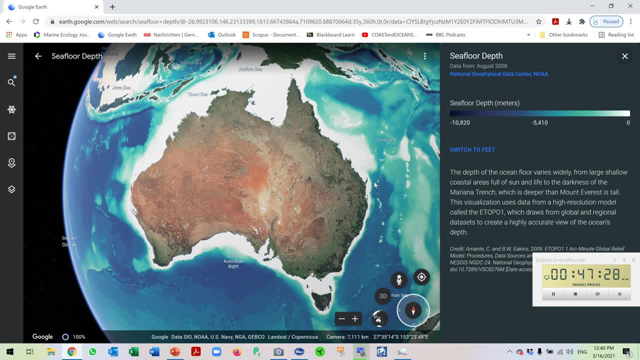 where we actually live around. where we actually live around this phrase island, this phrase island, this phrase island, morton, australia, morton australia. morton australia. the continental boundary, the continental boundary, the continental boundary is only maybe 50 kilometers out. it's a is only maybe 50 kilometers out, it's a. 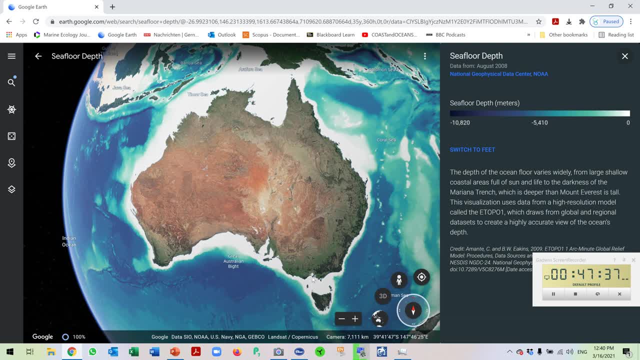 is only maybe 50 kilometers out. it's a very, very, very, very narrow continental shelf. here we've got a narrow continental shelf. here we've got a narrow continental shelf. here we've got a broader one again in best strait in the broader one again in best strait in the. 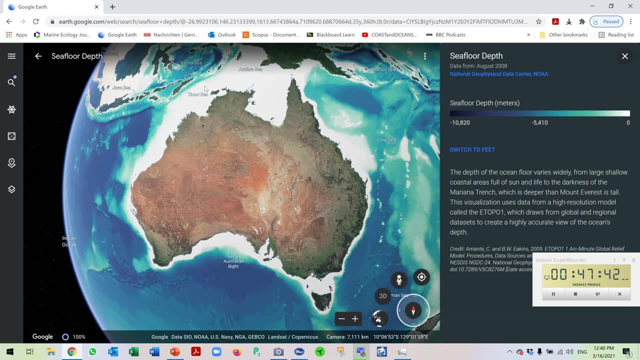 broader one again in best strait, in the great australian bite and so forth, and great australian bite and so forth, and great australian bite and so forth and so forth. so so so, essentially, essentially, essentially, you can examine for yourself, you can examine for yourself. 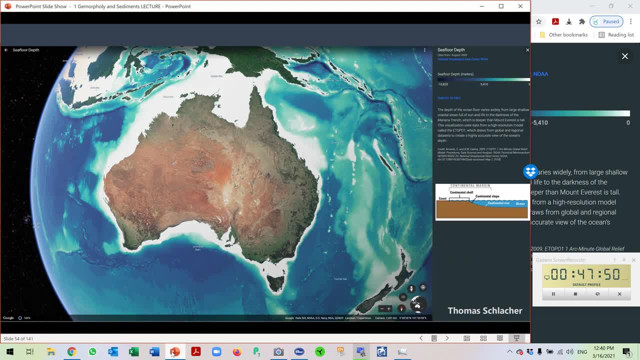 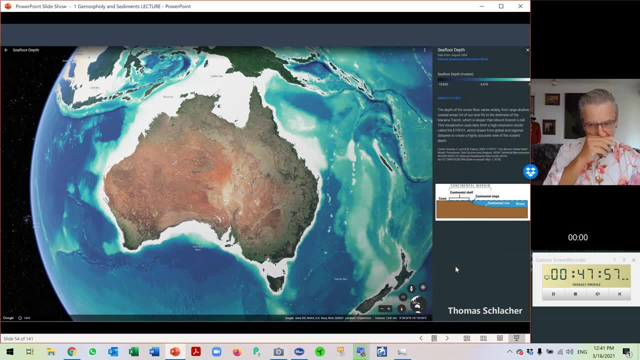 you can examine for yourself whether the textbook is right by whether the textbook is right, by whether the textbook is right by having a look at, having a look at, having a look at those, by having a look at, by having a look at, by having a look at imagery which is available to everybody. 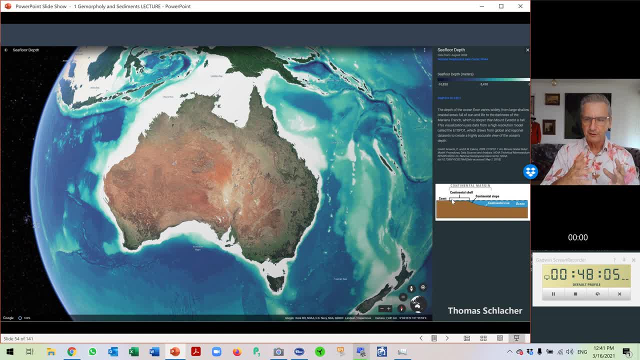 imagery which is available to everybody, imagery which is available to everybody now, now, now so that bit of the continent which really so, that bit of the continent which really so that bit of the continent which really is part normally, you know when sea is part. normally, you know when sea. 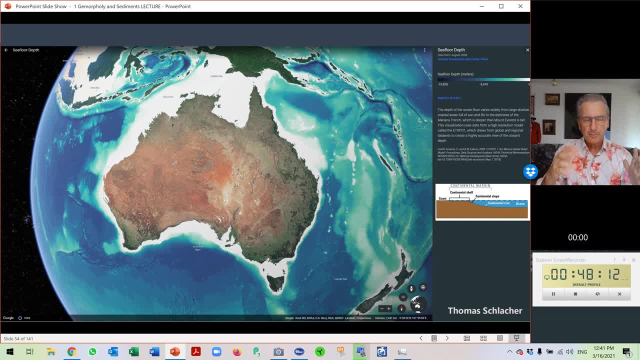 is part. normally, you know when sea levels go up and down of the drylands, levels go up and down of the drylands, levels go up and down of the drylands, counter-continental shelf, counter-continental shelf, counter-continental shelf, and you know where it actually ends. 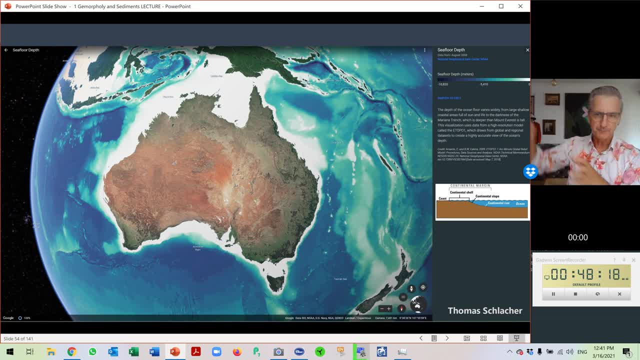 and you know where it actually ends. and you know where it actually ends because if you would actually take a, because if you would actually take a, because if you would actually take a boat out here from muloraba, boat out here from muloraba, boat out here from muloraba, well enough, today. 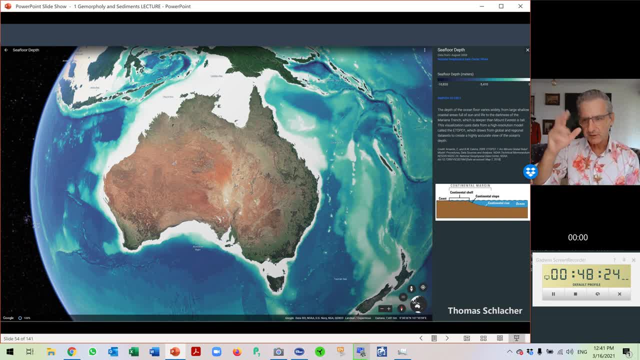 well enough today. well enough today, dramatically, if you actually do dramatically, if you actually do dramatically, if you actually do something like this and you can go dive something like this, and you can go dive something like this and you can go dive in, in, in on some of the, you know, pacific islands. 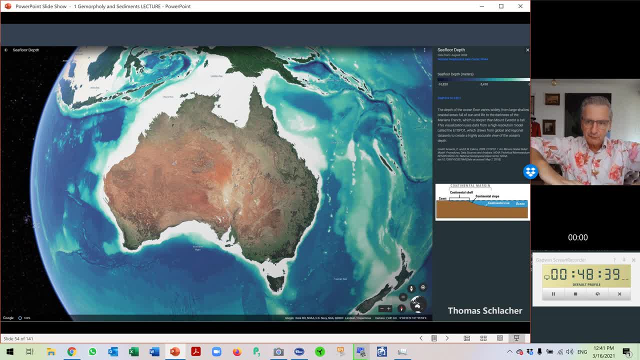 on some of the you know pacific islands, on some of the you know pacific islands. when you do one of those dives for the, when you do one of those dives for the, when you do one of those dives for the first time where you go off this, 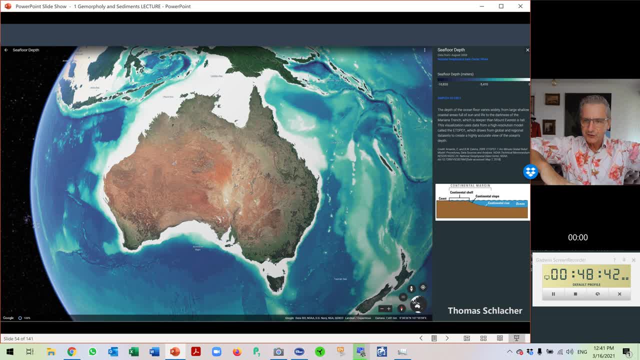 first time where you go off this, first time where you go off this off the island, uh, off the island, uh off the island, uh, basically edge, so to speak, on the water, basically edge, so to speak, on the water, basically edge, so to speak, on the water. and then you look down at about 4 000. 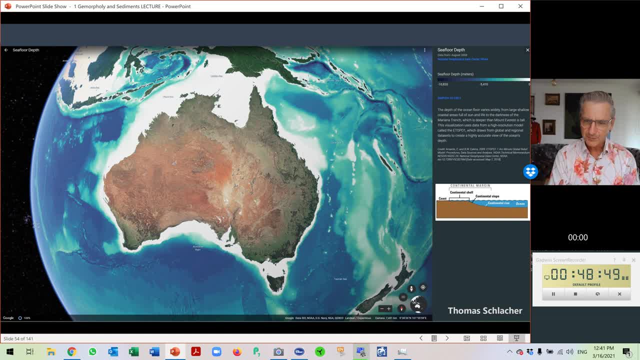 and then you look down at about 4 000 and then you look down at about 4 000 meters of water is actually meters of water is actually meters of water is actually quite scary, quite scary, quite scary. but basically we go out and then you 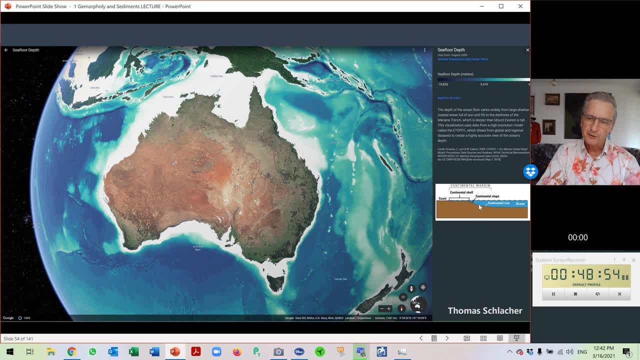 but basically we go out and then you, but basically we go out, and then you know the, you know, know the, you know, know the you know. the geological structures slope down. the geological structures slope down. the geological structures slope down fairly steeply called the continental, fairly steeply called the continental. 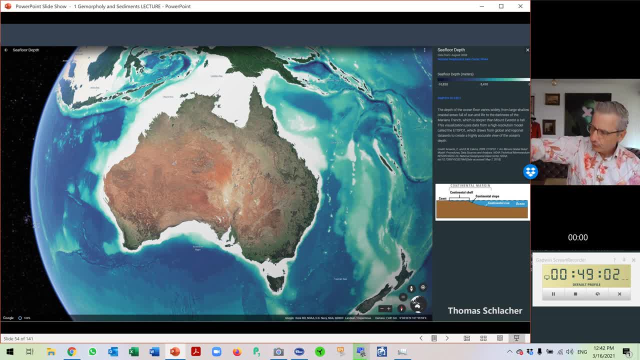 fairly steeply, called the continental slope, and it actually flattens out a bit slope and it actually flattens out a bit slope and it actually flattens out a bit and goes over into the abyssal and goes over into the abyssal and goes over into the abyssal plains. this is pretty much what actually 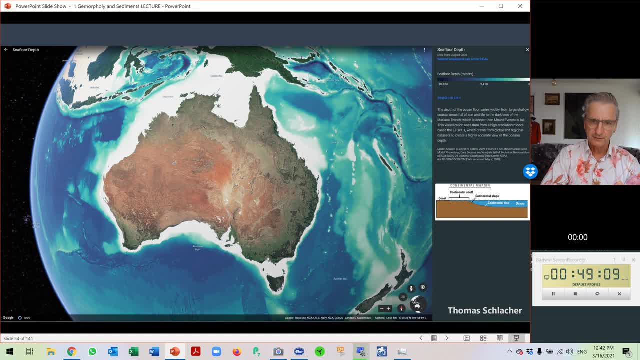 plains. this is pretty much what actually plains. this is pretty much what actually happens. happens happens around the australian island, around the australian island, around the australian island. now we work a lot now, we work a lot. now we work a lot of tasmania and we're going to have two. 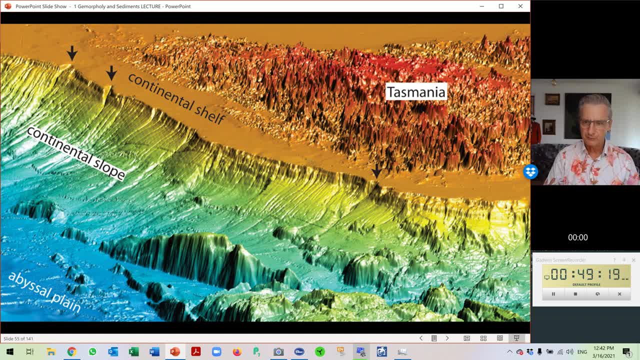 of tasmania and we're going to have two of tasmania and we're going to have two lectures on deep sea ecology. lectures on deep sea ecology. lectures on deep sea ecology: the work we're doing there on deep. the work we're doing there on deep. 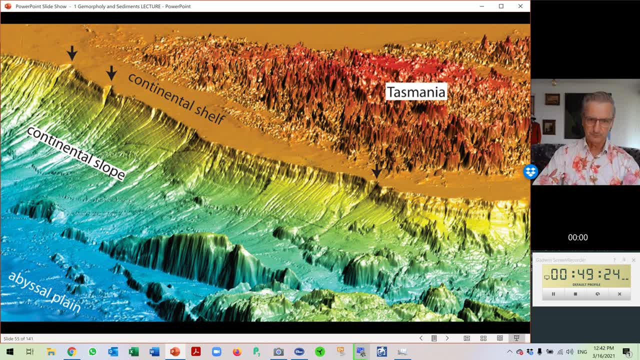 the work we're doing there on deep corals and also on corals, and also on corals, and also on submarine submarine, submarine canyons, canyons, canyons, and this is actually what it really looks, and this is actually what it really looks. 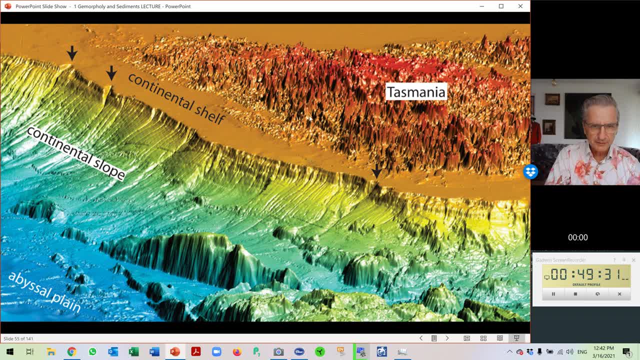 and this is actually what it really looks like. yeah, you can know all that sort of like. yeah, you can know all that sort of like. yeah, you can know all that sort of. you know fancy red bit here. you know fancy red bit here. you know fancy red bit here. it, for our purposes, there is a fairly 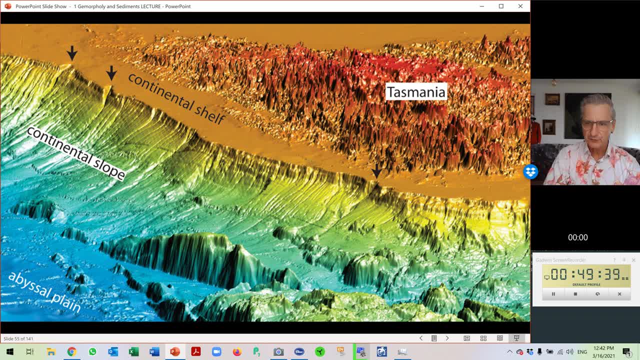 it for our purposes. there is a fairly it for our purposes. there is a fairly gentle, sloping, gentle, sloping, gentle, sloping, flattish piece of terrain called the flattish piece of terrain, called the flattish piece of terrain called the continental shore, continental shore, continental shore. a few canyons here and then it basically. 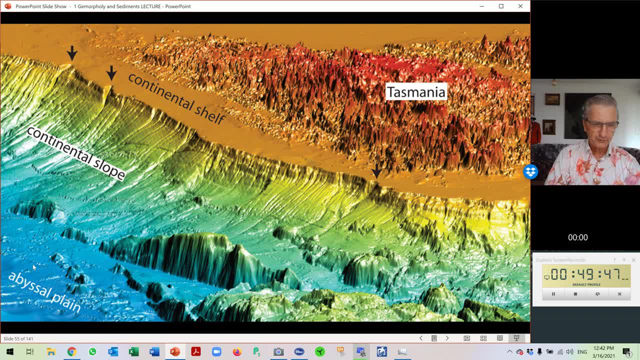 a few canyons here, and then it basically a few canyons here, and then it basically slopes down very dramatically. we have slopes down very dramatically. we have slopes down very dramatically. we have seamounts here, and then it actually seamounts here, and then it actually 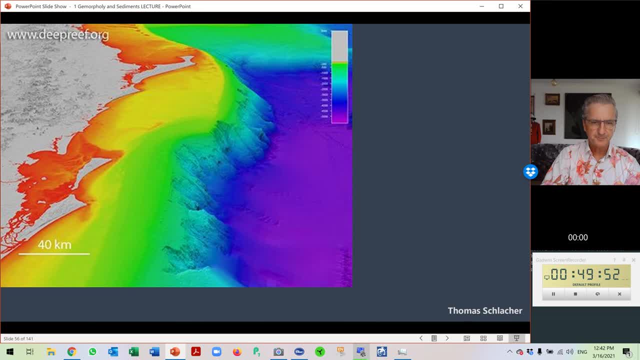 seamounts here, and then it actually flattens out the gang into the abyssal, flattens out the gang into the abyssal, flattens out the gang into the abyssal. plane, plane, plane- now part of the world. we got a nice uh. now part of the world. we got a nice uh. 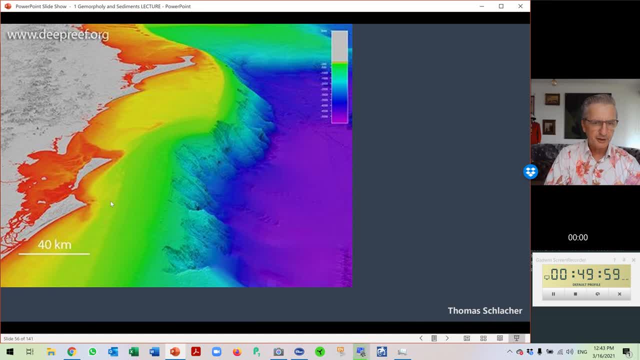 now part of the world. we got a nice, uh, basically, basically, basically computer model here of the depths and you computer model here of the depths and you computer model here of the depths and you can see in chuba morton island, can see in chuba morton island. 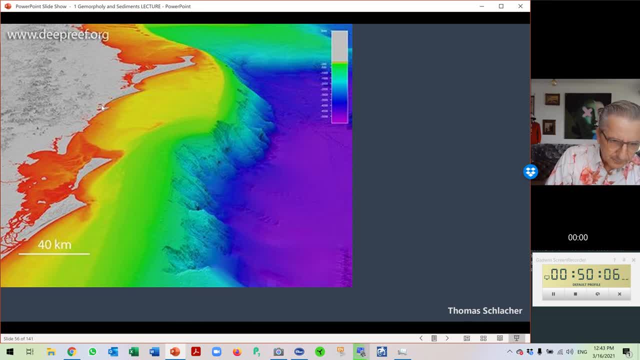 can see in chuba morton island at the moment. we sit right here at the moment, we sit right here at the moment. we sit right here against my house here, against my house here, against my house here. no, actually, is it right here, so for? no, actually is it right here, so for. 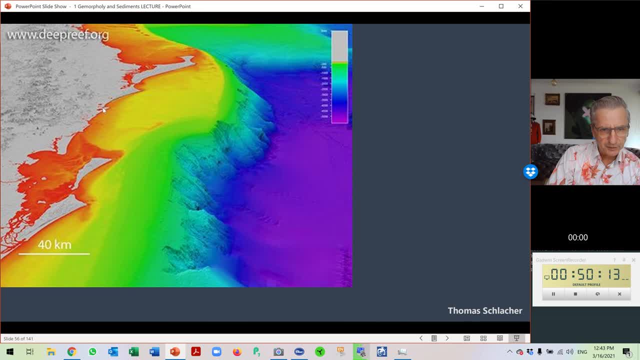 no, actually is it right here. so for that that, that this is noosa noosa national park. this is noosa noosa national park. this is noosa noosa national park headlands, and then tiva double island headlands, and then tiva double island. 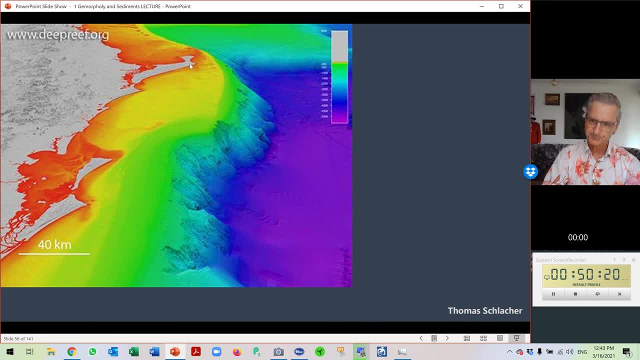 headlands and then tiva double island point, going over point, going over point, going over to kagari, fraser island, kagari, fraser island, kagari, fraser island, and, and, and this is a depiction of the sand, this is a depiction of the sand. 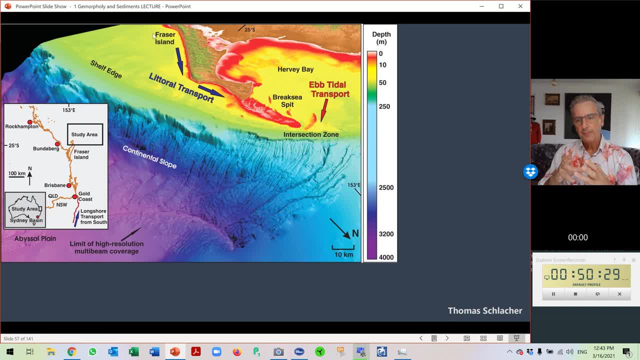 this is a depiction of the sand transport. what actually happens is the transport. what actually happens is the transport. what actually happens is the east australian current. east australian current east australian current moves millions of tons of sand a year. moves millions of tons of sand a year. 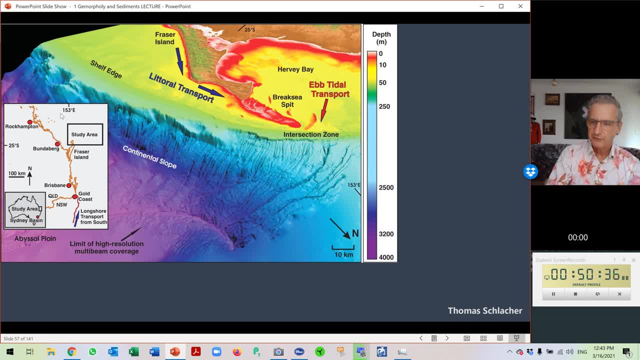 moves millions of tons of sand a year up, up, up the coast, the coast, the coast. at the very last time we actually see, at the very last time we actually see, at the very last time we actually see, most of that is right at the tip of most of that is right at the tip of. 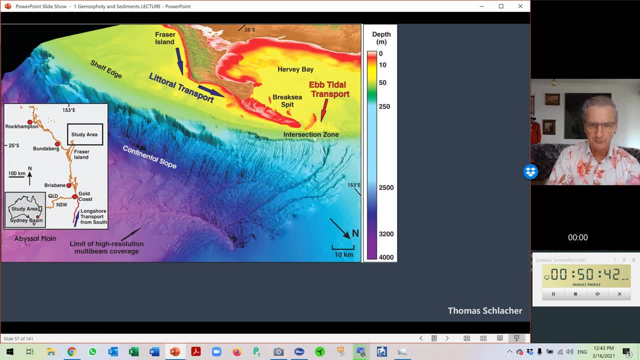 most of that is right at the tip of fraser island, where it actually goes- fraser island, where it actually goes fraser island, where it actually goes into this gigantic sand river, into this gigantic sand river, into this gigantic sand river and forms some of the largest basically. 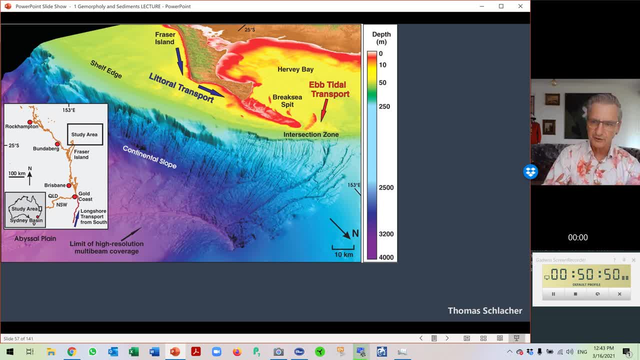 and forms some of the largest, basically, and forms some of the largest, basically, submarine waterfalls of sediment going, submarine waterfalls of sediment going submarine waterfalls of sediment going into the deep sea, into the deep sea, into the deep sea, never to be seen again. and this is why 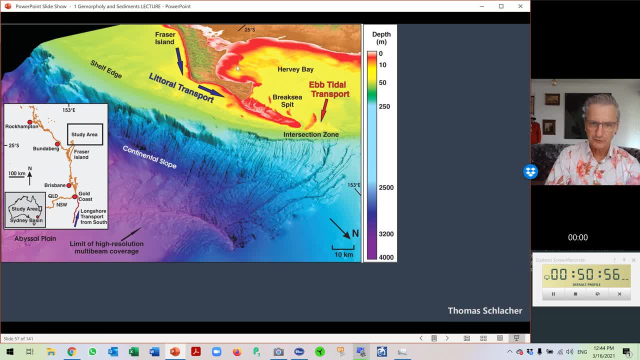 never to be seen again. and this is why never to be seen again, and this is why you don't have nice beaches further up. you don't have nice beaches further up. you don't have nice beaches further up from harvey bay. it just becomes muddy from harvey bay. it just becomes muddy. 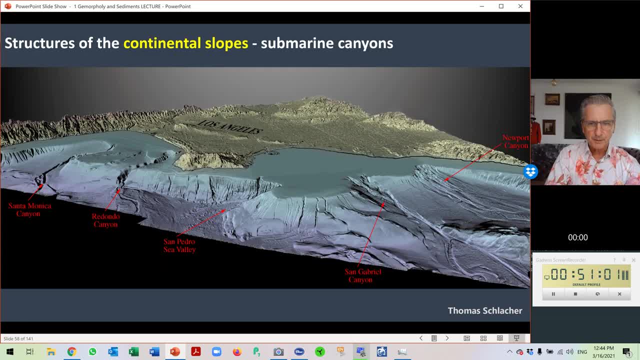 from harvey bay, it just becomes muddy. coral sand mangroves, that kind of stuff. coral sand mangroves, that kind of stuff. coral sand mangroves, that kind of stuff. uh uh uh. the continental slopes: this is basically the continental slopes. this is basically the continental slopes. this is basically once the shelf edge, basically the. 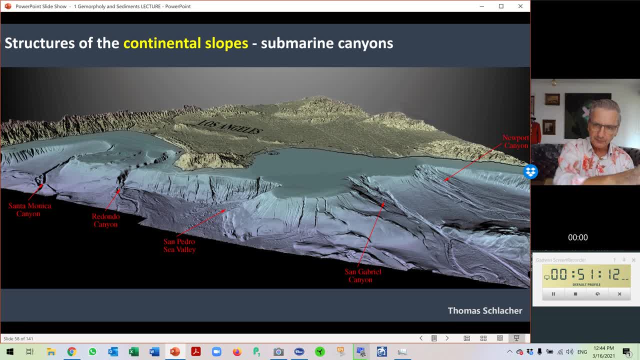 once the shelf edge, basically the once the shelf edge, basically the world true margin of the land stops, world true margin of the land stops, world true margin of the land stops, and then you have not a very smooth, and then you have not a very smooth and then you have not a very smooth margin going along. 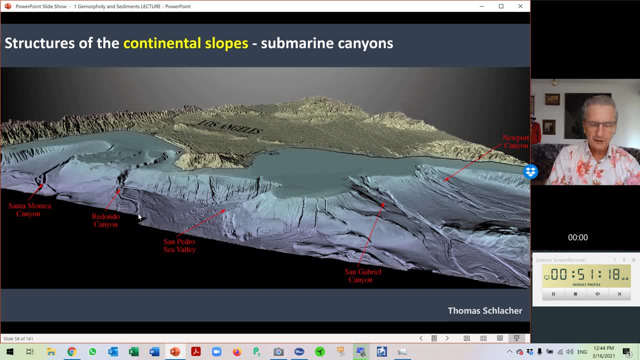 margin going along. margin going along. it's actually bisected by enormously. it's actually bisected by enormously. it's actually bisected by enormously large, large, large submarine river valleys, submarine river valleys, submarine river valleys. here is a you know? depiction of la. here is a you know depiction of la. 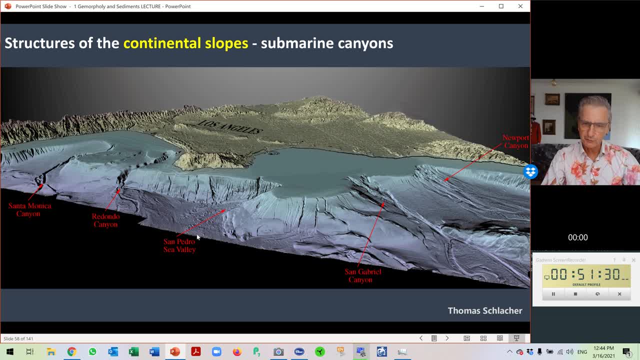 here is a- you know, depiction of la. it's got the santa monica the redundant, it's got the santa monica the redundant, it's got the santa monica the redundant, canyons and so forth, so canyons and so forth, so canyons and so forth, so, and those canyons are the size of the. 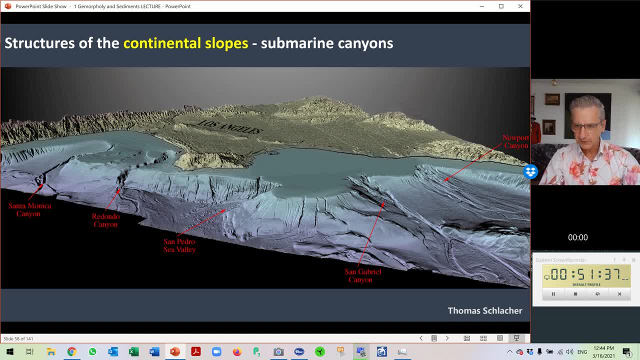 and those canyons are the size of the, and those canyons are the size of the grand canyon on land- grand canyon on land, grand canyon on land. and they used to actually deliver either and they used to actually deliver either, and they used to actually deliver either during sea level. 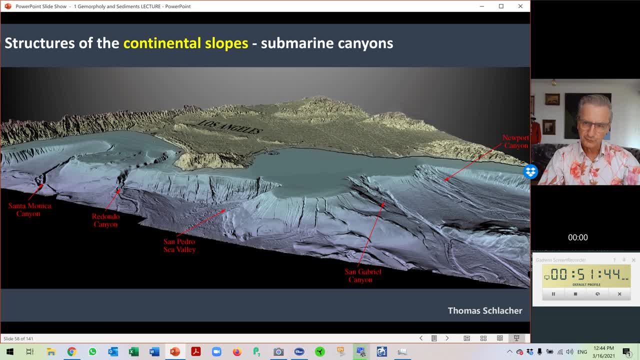 during sea level. during sea level low stands, you know fresh water or low stands. you know fresh water or low stands. you know fresh water or estuarine water down into the deep sea, estuarine water down into the deep sea, estuarine water down into the deep sea. water got actually carved for, you know. 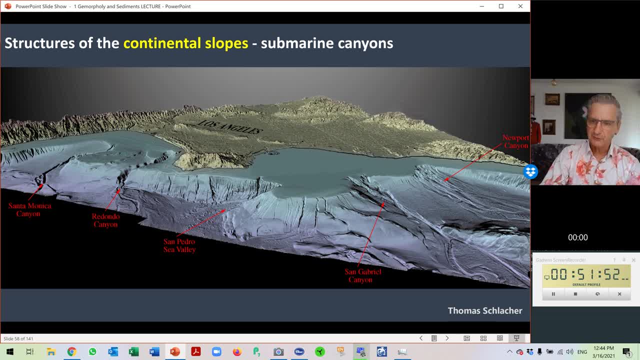 water got actually carved for. you know, water got actually carved for. you know, geologically, geologically, geologically, fault structures where sediment, then fault structures where sediment, then fault structures where sediment, then basically hollows them out, basically hollows them out, basically hollows them out. we have pretty much, you know, a good. 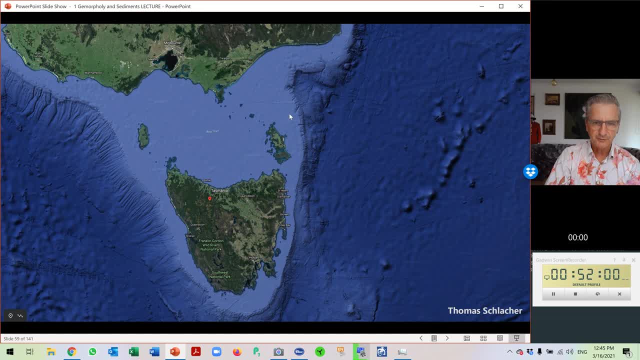 we have pretty much you know a good. we have pretty much you know a good system. you know down system, you know down system. you know down in the southern part, in the southern part, in the southern part. look at this big system, here it's called. look at this big system, here it's called. 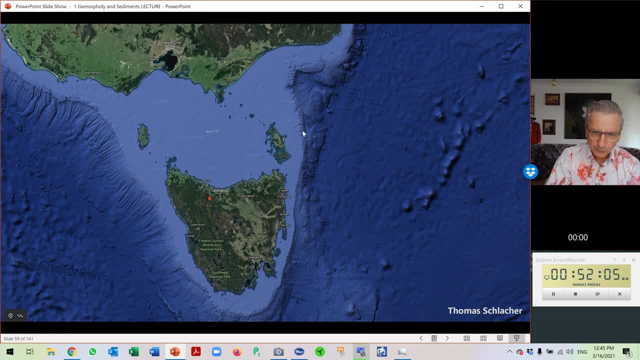 look at this big system here it's called the big horseshoe canyon. we have been the big horseshoe canyon. we have been the big horseshoe canyon. we have been working there for several years, but all working there for several years. but all working there for several years. but all these little canyons- here there's a bit. these little canyons here there's a bit these little canyons. here there's a bit of a debate. you know which ones are of a debate. you know which ones are of a debate, you know which ones are actually properly mapped on up, but never. 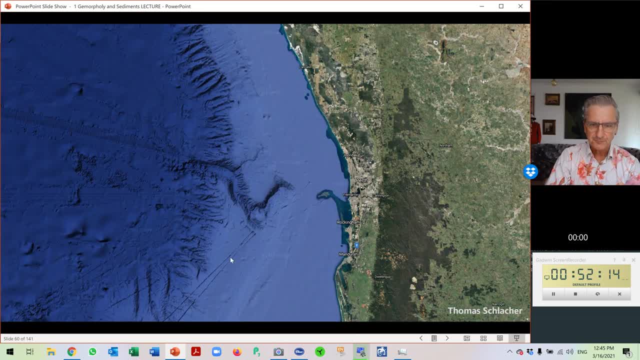 actually properly mapped on up, but never actually properly mapped on up. but never mind about it going all around here. you mind about it going all around here. you mind about it going all around here. you can actually, can, actually, can actually see this: you can go over to perth. look at. 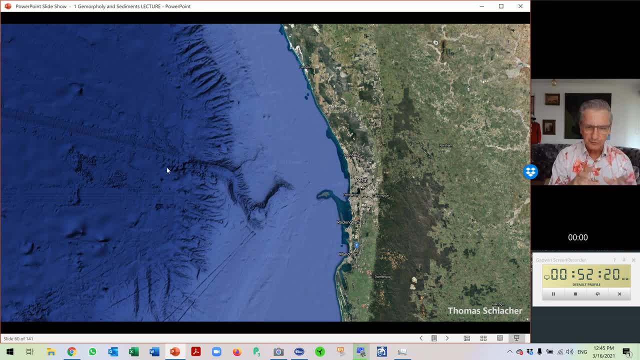 see this: you can go over to perth. look at. see this: you can go over to perth. look at the perth canyon. isn't that fantastic? the perth canyon isn't that fantastic? the perth canyon isn't that fantastic. looks like almost like a serpent, or 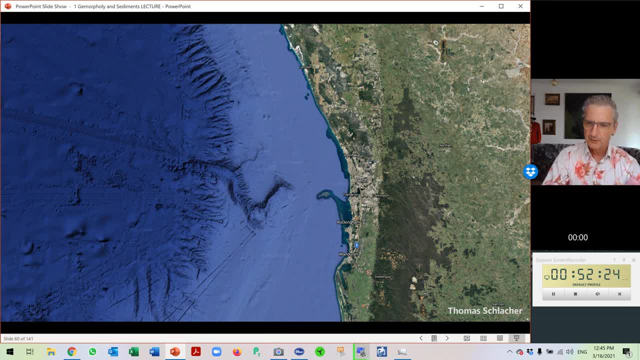 looks like almost like a serpent, or looks like a serpent, or something like this. you know coming up to something like this. you know coming up to something like this. you know coming up to eat. eat, eat, mark mcgowan. it wouldn't be a bad thing, mark mcgowan, it wouldn't be a bad thing. 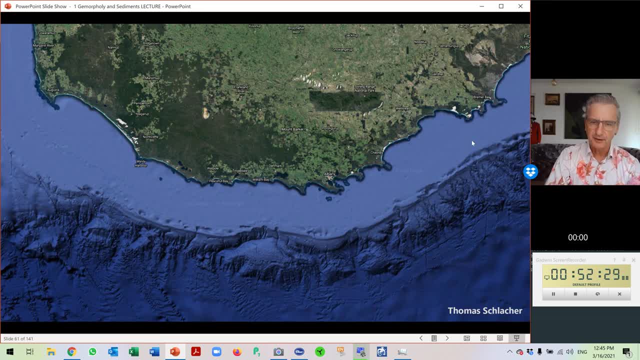 mark mcgowan, it wouldn't be a bad thing, but i haven't said that, but i haven't said that, but i haven't said that. and then of course to the south here, and then of course to the south here, and then of course to the south here, denmark area, which i think has the some 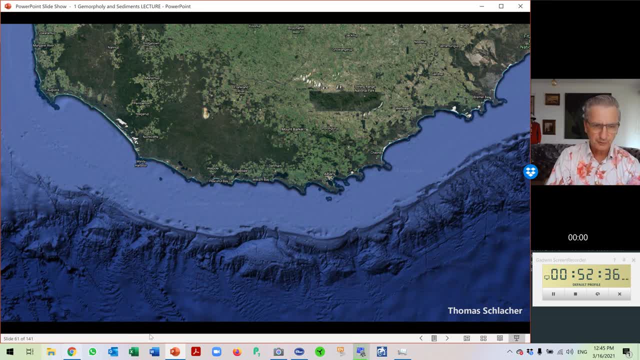 denmark area which i think has the some denmark area which i think has the some of the best upcoming, of the best upcoming, of the best upcoming: uh, cabernet sauvignon's, the landscape is, uh, cabernet sauvignon's, the landscape is, uh, cabernet sauvignon's, the landscape is really quite dramatic. you know, if you 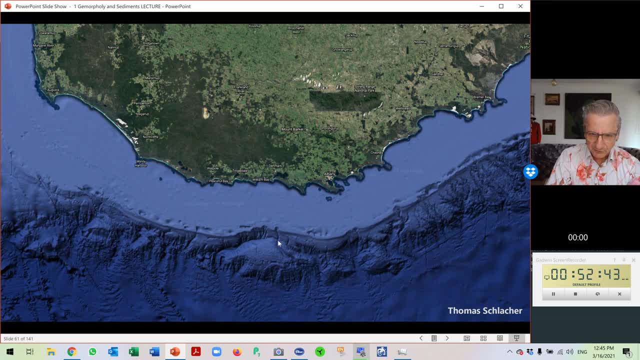 really quite dramatic. you know, if you really quite dramatic, you know if you look at the continental shelf and look, look at the continental shelf and look, look at the continental shelf and look at this sediment delta here, which at this sediment delta here, which at this sediment delta here which actually got forged here by a canyon. 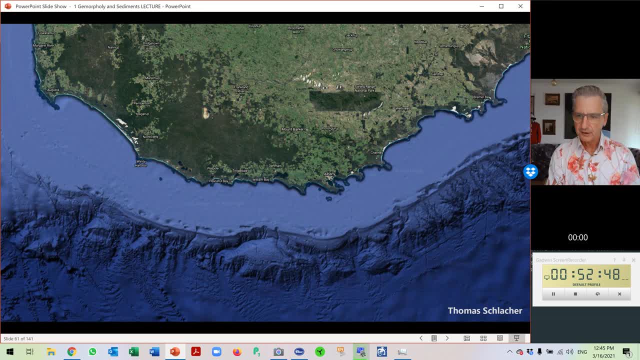 actually got forged here by a canyon. actually got forged here by a canyon. those are the canyons where you know. those are the canyons where you know. those are the canyons where you know whale researchers like to hang out. whale researchers like to hang out. 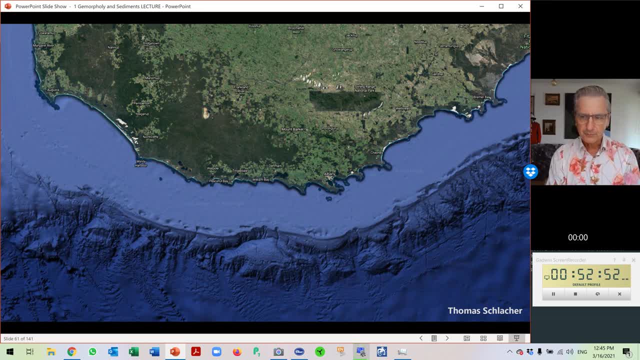 whale researchers like to hang out because they, because they, because they- apparently, you know, seem to be the apparently, you know, seem to be the apparently you know seem to be the favorite hangouts for some of the favorite hangouts for some of the favorite hangouts for some of the deep hunting sperm whales coming up. 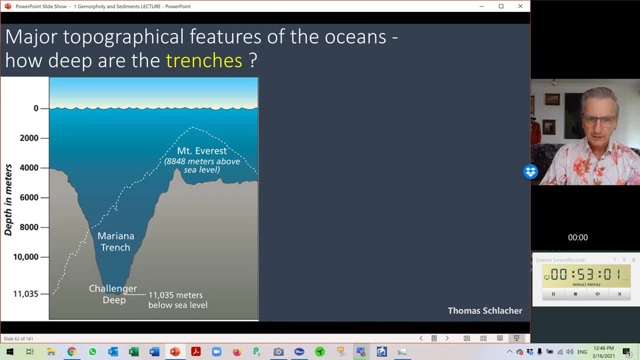 deep hunting sperm whales coming up, deep hunting sperm whales coming up into sunlit areas, into sunlit areas, into sunlit areas, uh, uh, uh. i already told you how deep the trenches. i already told you how deep the trenches. i already told you how deep the trenches are right in the beginning and i love. 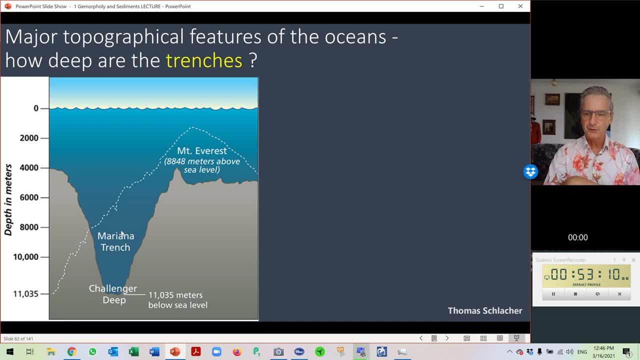 are right in the beginning and i love are right in the beginning and i love this diagram. you see it in many, this diagram. you see it in many, this diagram. you see it in many textbooks, textbooks, textbooks. if you were to, if you were to, if you were to invert, basically the mariana trench. 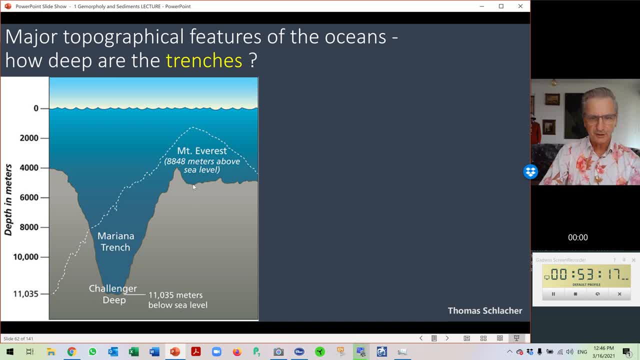 invert basically the mariana trench, invert basically the mariana trench, and you know, superimpose it to the height. and you know, superimpose it to the height and you know, superimpose it to the height of mount everest, you can actually see, of mount everest, you can actually see. 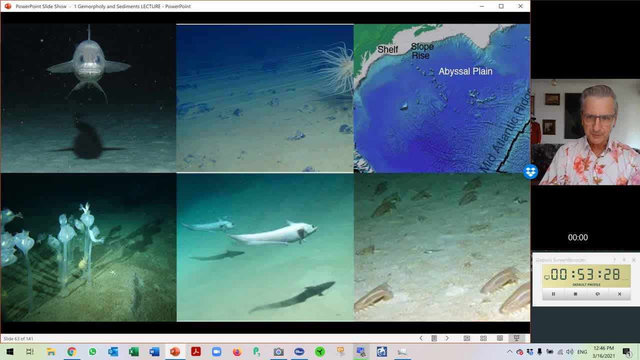 of mount everest. you can actually see thousand uh 2200 meters, thousand uh 2200 meters, thousand uh 2200 meters. deeper, deeper, deeper. now the abyssal plains, now the abyssal plains, now the abyssal plains. here you've got a good example of 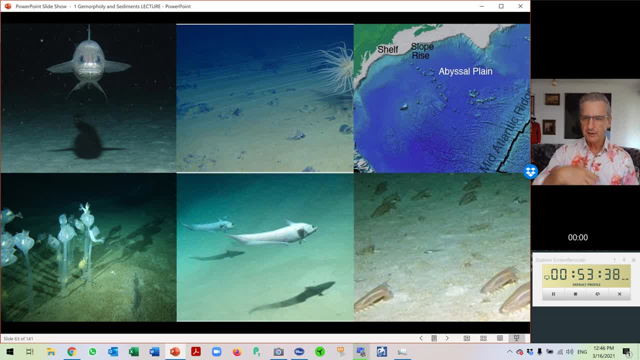 here you've got a good example of. here you've got a good example of basically, basically, basically, uh, the eastern seaboard of south america, uh, the eastern seaboard of south america, uh, the eastern seaboard of south america, north america. i just illustrated here that north america. i just illustrated here that. 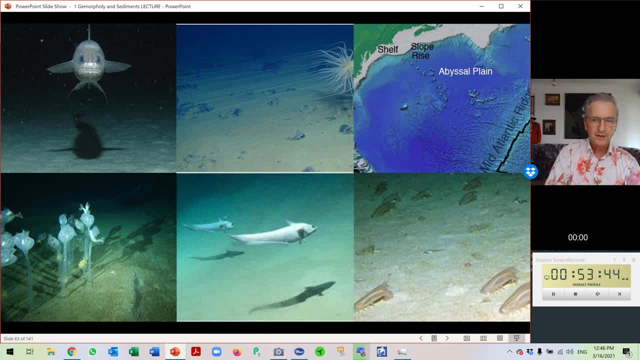 north america. i just illustrated here that they often cover, they often cover, they often cover very, very large areas, very, very large areas, very, very large areas, and they're kind of muddy and they're kind of muddy and they're kind of muddy. people used to think they're quite. 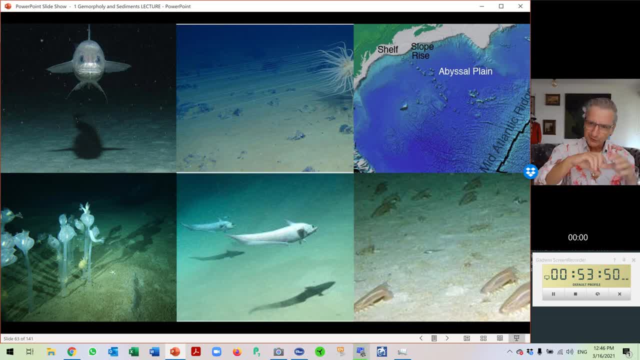 people used to think they're quite. people used to think they're quite featureless, but they're not. they've got featureless, but they're not. they've got featureless, but they're not. they've got the cause of abyssal hills. there's lots. the cause of abyssal hills: there's lots. 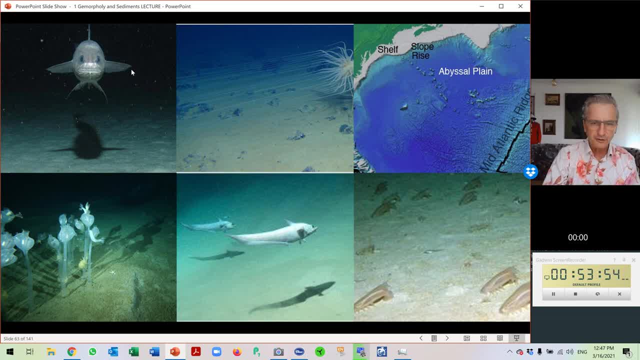 the cause of abyssal hills. there's lots of fractures and so forth. but besides of fractures and so forth, but besides of fractures and so forth, but besides all that kind of muddy nature, you get an all that kind of muddy nature. you get an all that kind of muddy nature, you get an enormously. 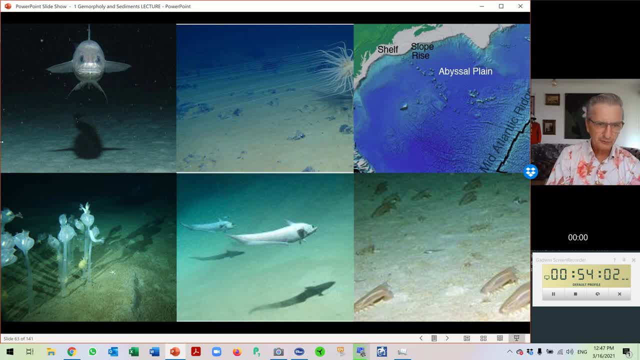 enormously, enormously fascinating array of organisms. you get fascinating array of organisms. you get fascinating array of organisms. you get those kind of very slow moving fish, those kind of very slow moving fish, those kind of very slow moving fish which almost seem to hover over the, which almost seem to hover over the. 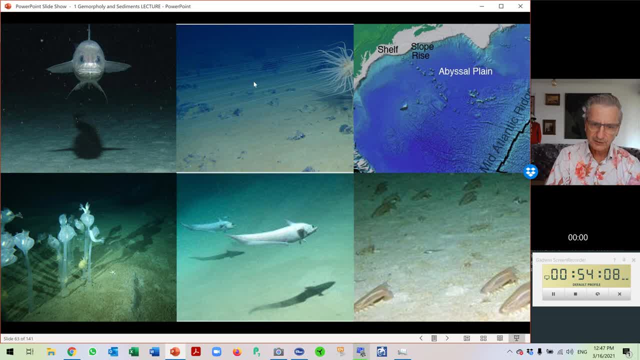 which almost seem to hover over the sediment, sediment sediment. you've got, uh, deep sea sea anemones here. you've got deep sea sea anemones. here you've got deep sea sea anemones. here you've got kind of deer fishes. you've got kind of deer fishes. 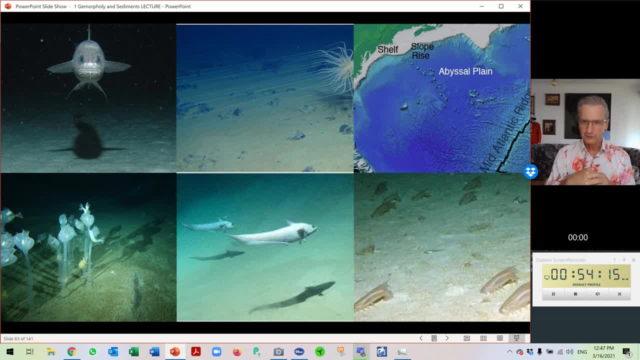 you've got kind of deer fishes. those are uh holothurians sea cucumbers. those are uh holothurians sea cucumbers. those are uh holothurians sea cucumbers we actually have little feet to actually. we actually have little feet to actually. 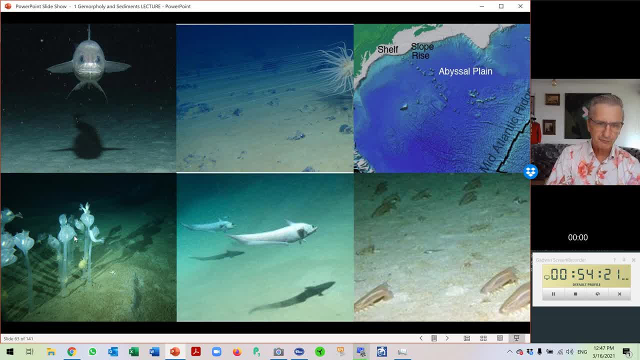 we actually have little feet to actually move along, move along, move along. and those are very, very you know, fragile and those are very, very you know fragile and those are very, very you know fragile. glass sponges, glass sponges, glass sponges- in mud got a few, what are those off? 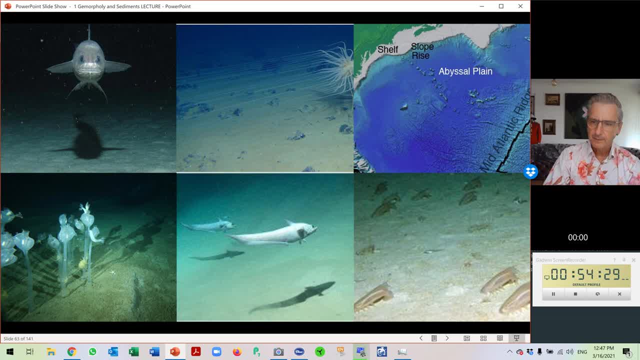 in mud? got a few. what are those off in mud? got a few. what are those off? you know sitting on those stalks here. so you know sitting on those stalks here. so you know sitting on those stalks here. so the abyssal plains, the abyssal plains. 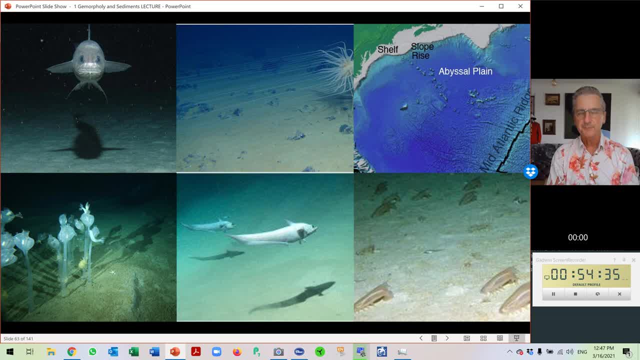 the abyssal plains might have been additionally. you might might have been additionally, you might might have been additionally. you might still actually, still, actually still actually read this in textbooks that they are read, this in textbooks that they are read this in textbooks that they are featureless, but they are not. they're. 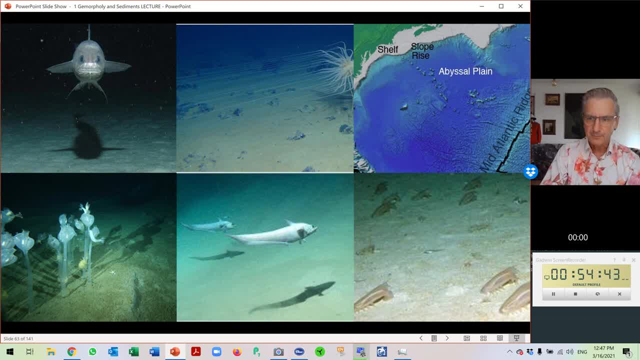 featureless, but they are not. they're featureless, but they are not, they're basically, basically, basically, you know very, very uh rich. you know very, very uh rich. you know very, very uh rich in biological life, in biological life, in biological life. here you might say: this is a big abyssal. 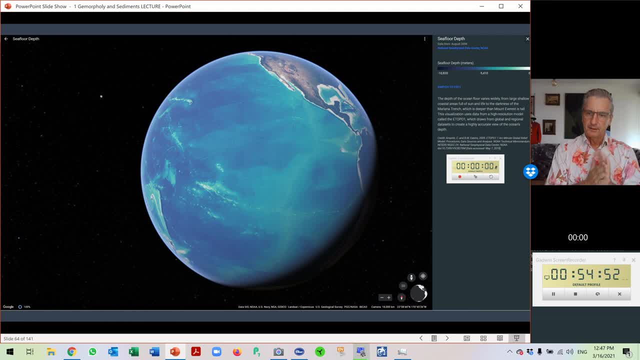 here you might say: this is a big abyssal. here you might say: this is a big abyssal, plain. and we come back to that plain. and we come back to that plain and we come back to that in the next lecture on deep ocean, in the next lecture on deep ocean. 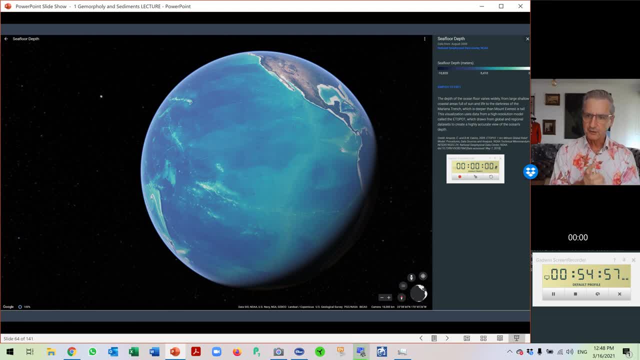 in the next lecture on deep ocean sediments. because sediments? because sediments, because this is a site of intense, this is a site of intense, this is a site of intense international. how would i say rivalry international? how would i say rivalry international? how would i say rivalry to access deep mineral deposits? 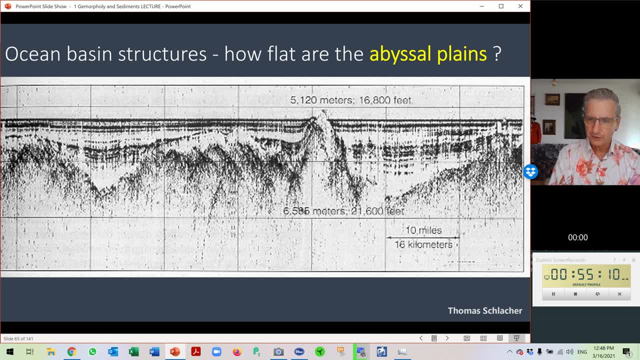 to access deep mineral deposits. to access deep mineral deposits. i love this picture. it's quite an old. i love this picture. it's quite an old. i love this picture. it's quite an old one and it's basically how you actually one and it's basically how you actually. 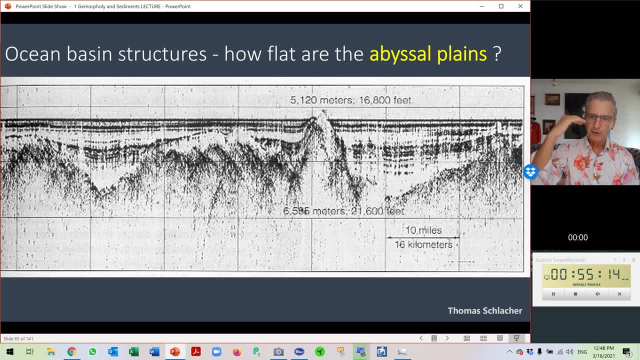 one, and it's basically how you actually create a sonogram like this. is you have create a sonogram like this, is you have create a sonogram like this, is you have a very, very strong, a very, very strong, a very, very strong sonar pose. sonar pose. 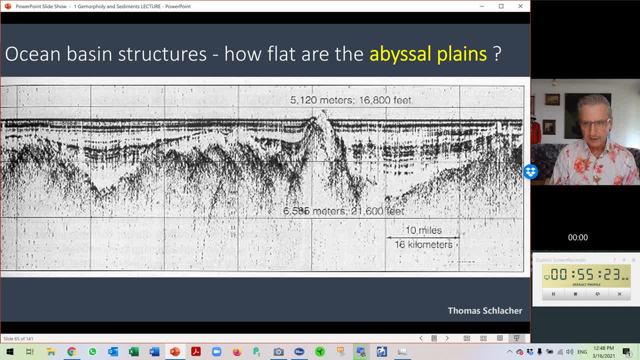 sonar pose. that goes down from the ship, penetrates. that goes down from the ship, penetrates. that goes down from the ship, penetrates. you know the layers and gets bounced. you know the layers and gets bounced. you know the layers and gets bounced back up, back up. 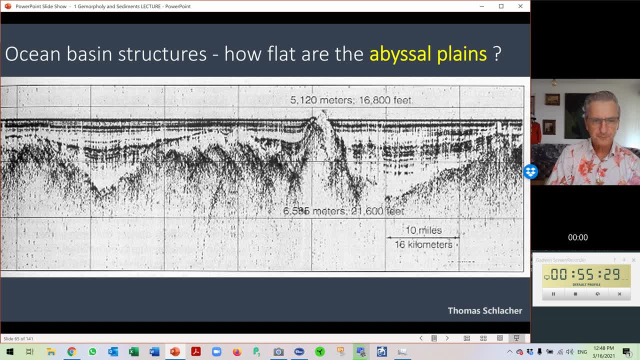 back up and you can actually record it, and because, and you can actually record it, and because and you can actually record it, and because different, different, different layers have different densities, they layers have different densities, they layers have different densities, they absorb sound to a different degree and 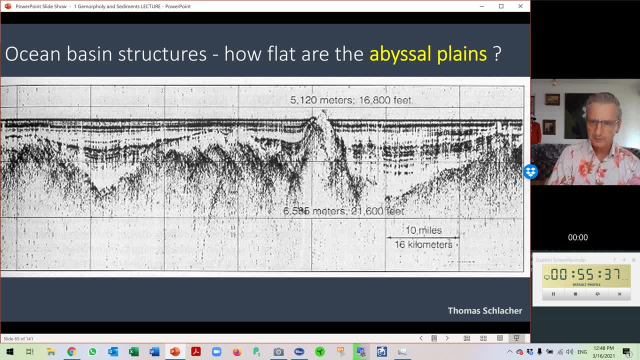 absorb sound to a different degree. and absorb sound to a different degree and bounce it back to a different degree. so bounce it back to a different degree. so bounce it back to a different degree. so you can actually work out. this is. you can actually work out. this is. 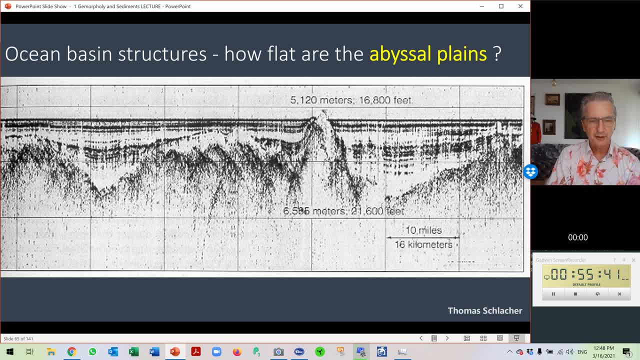 you can actually work out. this is basically the whole system, basically the whole system, basically the whole system: the theory behind having a fish finder, the theory behind having a fish finder, the theory behind having a fish finder- just a very, very strong and powerful one, just a very, very strong and powerful one. 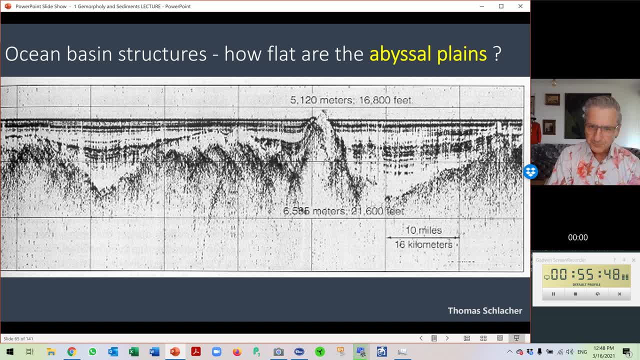 just a very, very strong and powerful one, and you can actually see this used to be and you can actually see this used to be and you can actually see this used to be the original landscape, the original landscape, the original landscape at some stage, at some stage, at some stage, and it got just smothered by sediment. 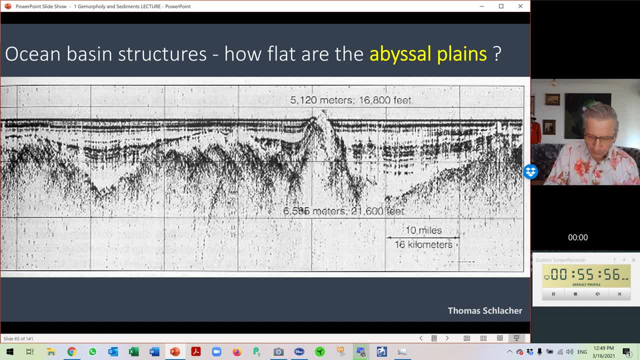 and it got just smothered by sediment. and it got just smothered by sediment, filled in it's like you know you create. filled in it's like you know you create. filled in it's like you know you create. a wonderful little you know alpine. 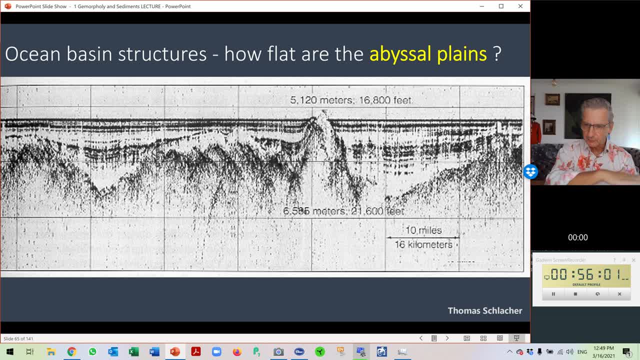 a wonderful little you know alpine. a wonderful little you know alpine scenery in a sandbox and then some scenery in a sandbox and then some scenery in a sandbox, and then some nasty kids comes and sort of just puts a. nasty kids comes and sort of just puts a. 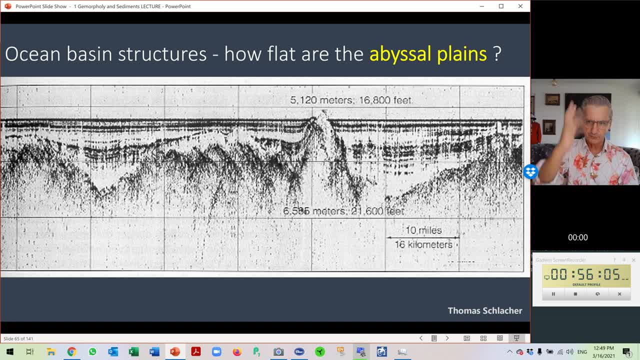 nasty kids, comes and sort of just puts a bucket of sand away, bucket of sand away, bucket of sand away. brushes the hand over it and says, well, i brushes the hand over it and says well, i brushes the hand over it and says well, i try all and say: 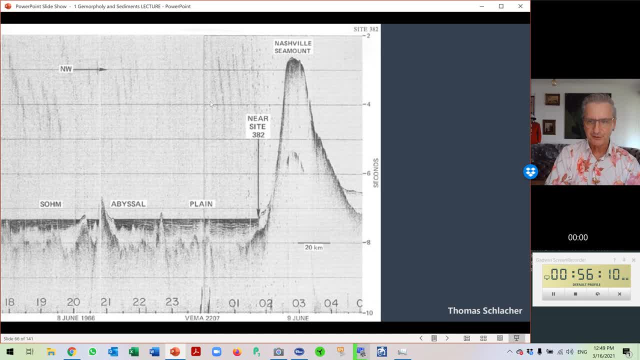 try all and say try all, and say: too bad, so sad, too bad, so sad, too bad, so sad. this one is particularly cool. this is the. this one is particularly cool. this is the. this one is particularly cool. this is the natural seamount and you see this. 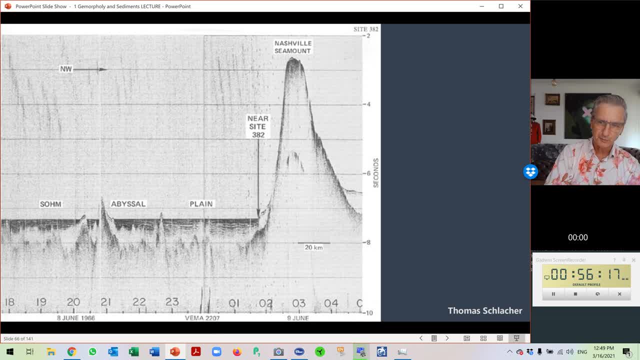 natural seamount and you see this natural seamount and you see this abyssal plane, abyssal plane, abyssal plane. and there is a movie out. i forgot the. and there is a movie out. i forgot the. and there is a movie out. i forgot the exact title. 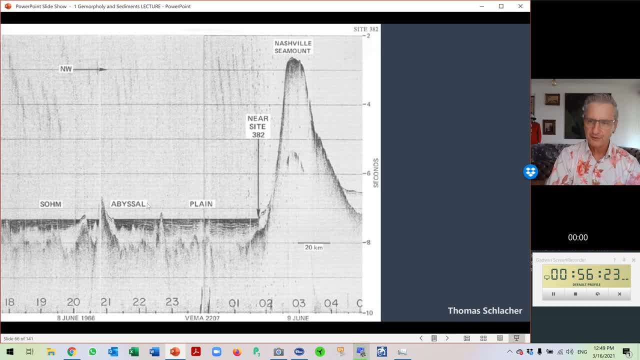 exact title. exact title: and the actual submarine crashes and the actual submarine crashes and the actual submarine crashes crashes into one of those seamounts. so you crashes into one of those seamounts. so you crashes into one of those seamounts, so you can see. 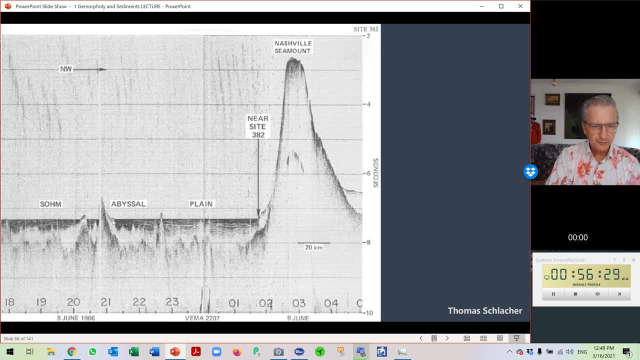 can see, can see quite clearly. yes, yes, yes, flat flat, quite clearly. yes, yes, yes, flat flat, quite clearly. yes, yes, yes, flat flat. that's actually a little bit, that's actually a little bit. that's actually a little bit poking out, and then you got a massive 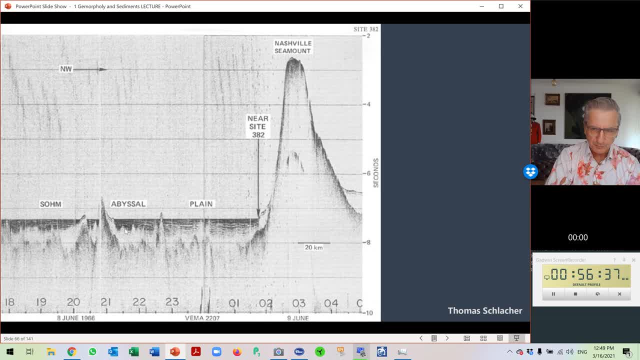 poking out, and then you got a massive poking out, and then you got a massive structure like this, and then it goes structure like this, and then it goes structure like this, and then it goes flat again. so those are the abyssal, flat again. so those are the abyssal. 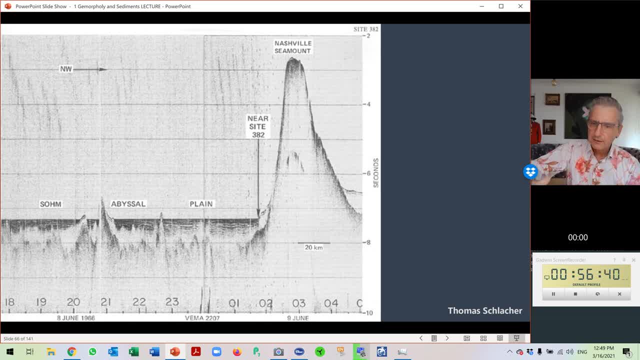 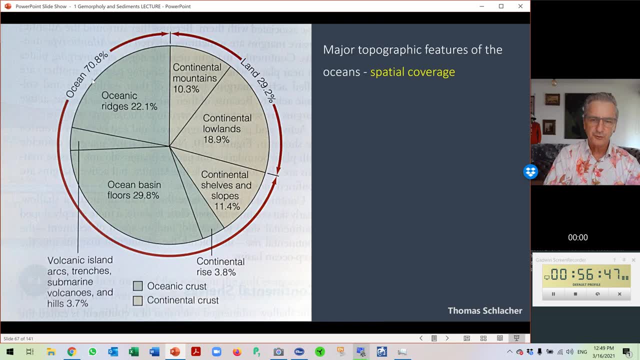 flat again. so those are the abyssal planes, they're basically the huge planes. they're basically the huge planes. they're basically the huge expanses of fine sand, expanses of fine sand, expanses of fine sand, silt and clay, silt and clay, silt and clay. when you actually do, you know the. 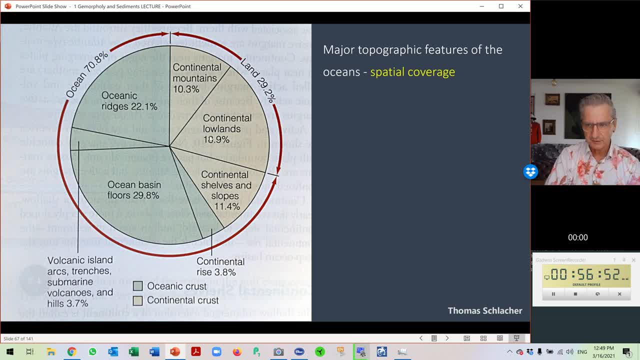 when you actually do you know the, when you actually do you know the spatial coverage. spatial coverage, spatial coverage of uh, calculation of uh. calculation of uh, calculation the ridges, and remember this is like the ridges and remember this is like the ridges and remember this is like new seafloor is being created. 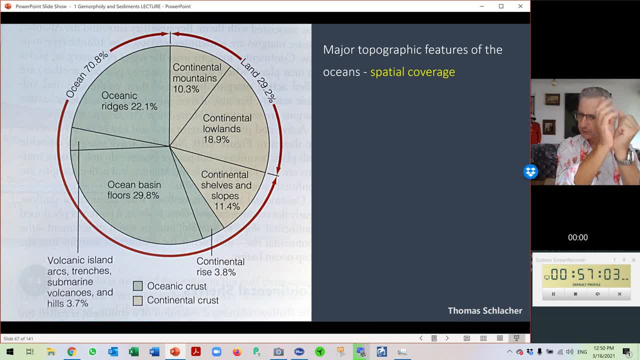 new seafloor is being created. new seafloor is being created by hot magma trying to bubble up, by hot magma. trying to bubble up by hot magma. trying to bubble up only a little bit makes it most of it. only a little bit makes it most of it. 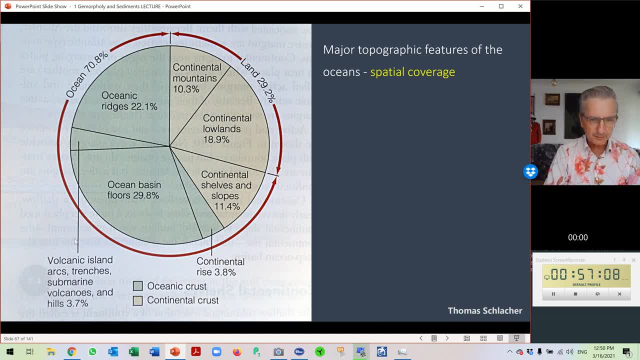 only a little bit. makes it most of it. actually goes to the side, actually goes to the side, actually goes to the side. the abyssal planes, the ocean basin, the abyssal planes, the ocean basin, the abyssal planes. the ocean basin floors cover about one third of the 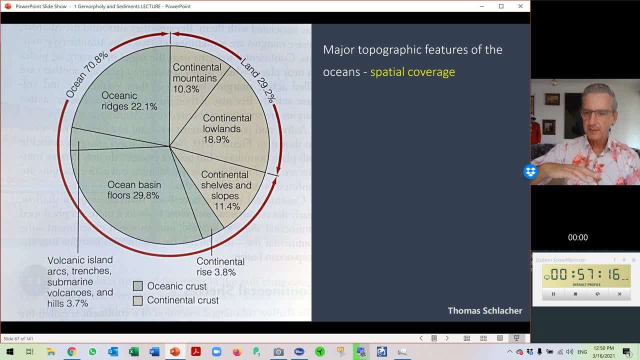 floors cover about one third of the floors, cover about one third of the planet. so this is vast expanses planet. so this is vast expanses planet. so this is vast expanses of mud and sand, of mud and sand, of mud and sand. the continental rises sit at the bottom. 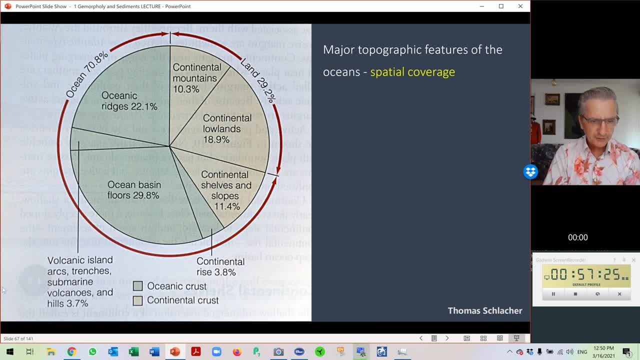 the continental rises sit at the bottom. the continental rises sit at the bottom, basically off the slopes. it's more like basically off the slopes. it's more like basically off the slopes. it's more like a transition zone, a transition zone, a transition zone. then we got something odd, because we're 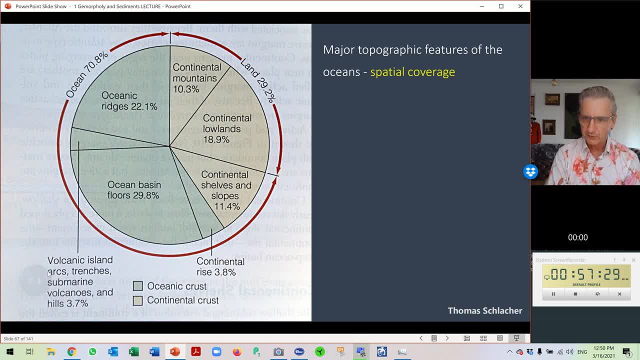 then we got something odd because we're. then we got something odd because we're talking about volcanic island arcs, talking about volcanic island arcs, talking about volcanic island arcs, we have, you know, all our neighbors are. we have, you know all our neighbors are. we have, you know all our neighbors are like that. you know, the, the tongas, the. 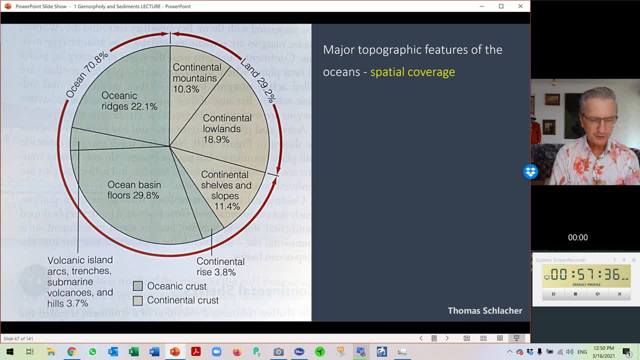 like that you know the the tongas. the like that you know the the tongas, the ronaldos, the new caledonians. the ronaldos, the new caledonians. the ronaldos, the new caledonians. the new zealand ones, new zealand ones. 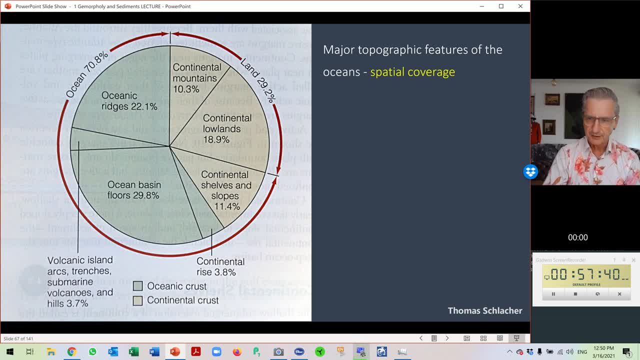 new zealand ones. and then we got something like, and then we got something like, and then we got something like submarine volcanoes- what the hell is submarine volcanoes? what the hell is submarine volcanoes? what the hell is that? that that, well, i can tell you quite a bit about. 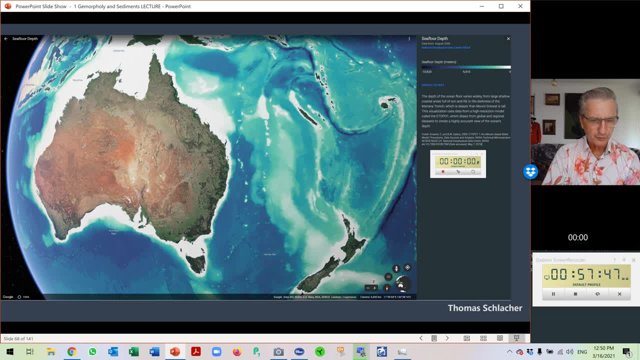 well, i can tell you quite a bit about. well, i can tell you quite a bit about submarine volcanoes, submarine volcanoes, submarine volcanoes, because, because, because, firstly, we've got tons of them in our firstly, we've got tons of them in our firstly, we've got tons of them in our neighborhood. 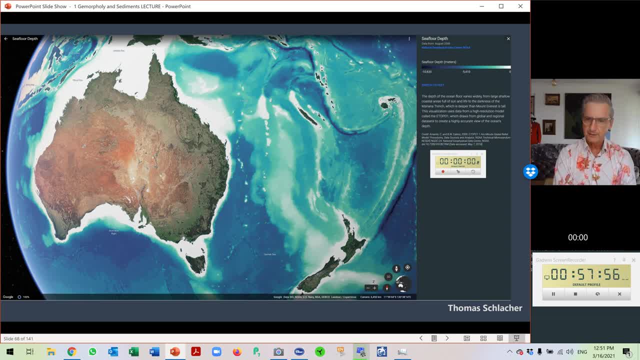 neighborhood, neighborhood. and secondly, i have spent you know, and secondly, i have spent you know, and secondly, i have spent, you know an interesting, you know a few years, you an interesting. you know a few years, you an interesting. you know a few years, you know, studying them in my career. so 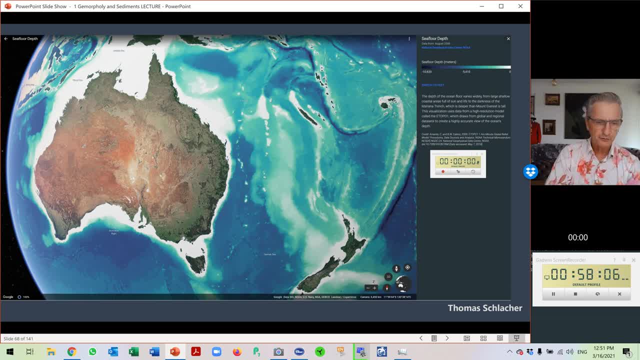 know, studying them in my career. so know, studying them in my career, so quite love them. you know we have just quite love them. you know we have just quite love them. you know we have just great and a bunch of people does this great and a bunch of people does this. 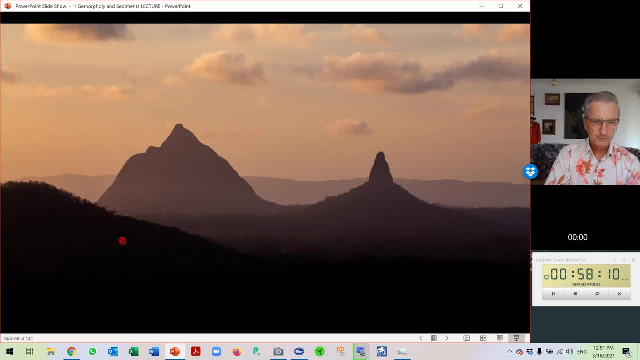 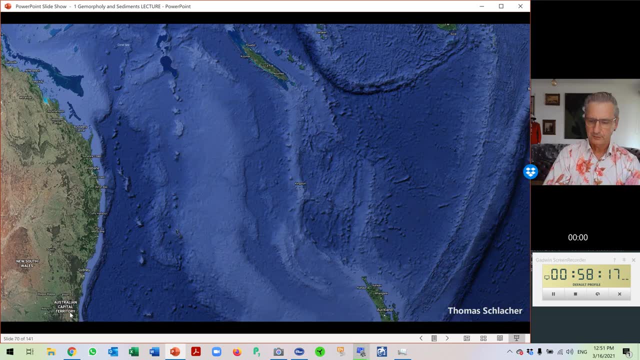 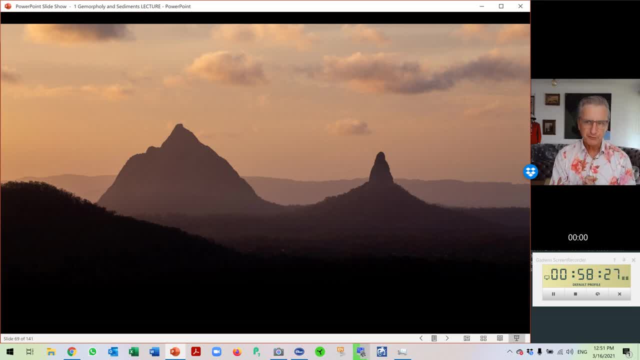 hour down the road hour down the road. you've got this landscape called the. you've got this landscape called the. you've got this landscape called the classes mountains beautiful to climb. classes mountains. beautiful to climb classes mountains beautiful to climb. beautiful to have sunset, picnics and all. 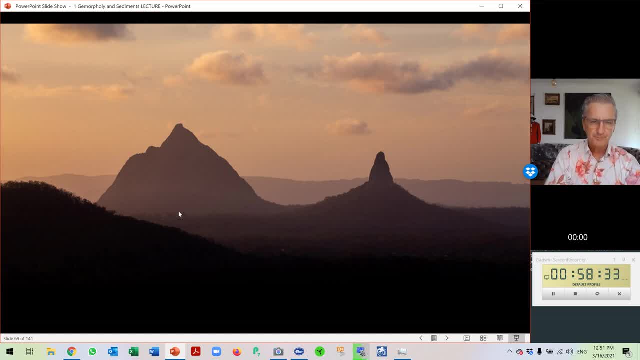 beautiful to have sunset picnics and all beautiful to have sunset picnics and all of that. you know it's all very of that. you know it's all very of that. you know it's all very victorious. this is the largest one of victorious. this is the largest one of. 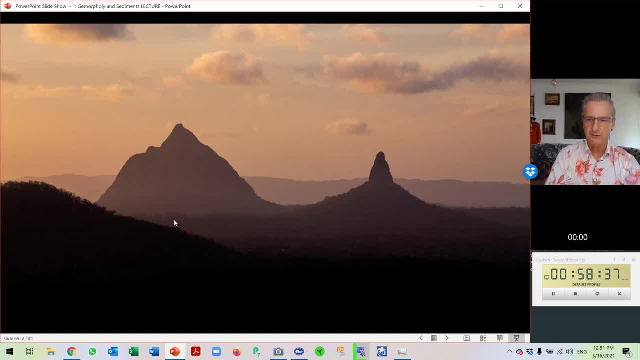 victorious. this is the largest one of them, called mount vera, and you might them called mount vera and you might them called mount vera. and you might say, oh right, you know how much is 300. say, oh right, you know how much is 300. say, oh right, you know how much is 300 meters. something like this: 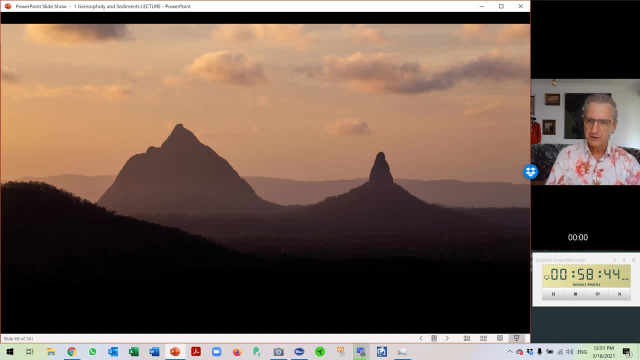 meters, something like this, meters, something like this. i can tell you the, i can tell you the. i can tell you, the glasshouse mountains are just like glasshouse mountains are just like glasshouse mountains, are just like little babies. you know they're like the little babies, you know they're like the. 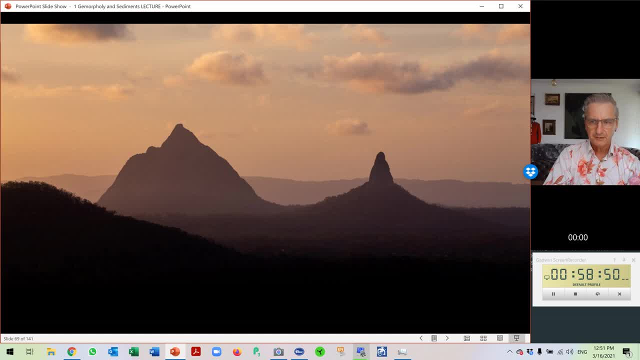 little babies. you know, they're like the suzuki chimney of the four by four world. suzuki chimney of the four by four world. suzuki chimney of the four by four world, you know. or ikea something, whatever you know, or ikea something, whatever you know, or ikea something, whatever. they're all good cars, don't get me wrong. 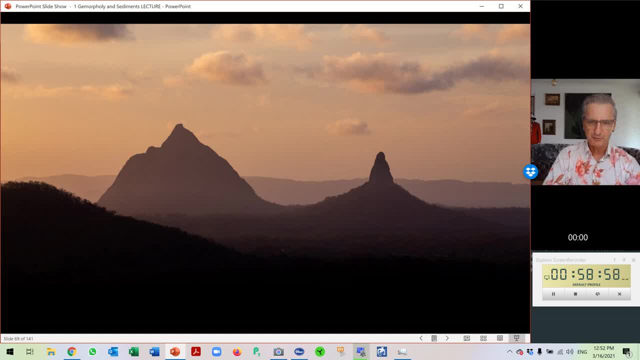 they're all good cars, don't get me wrong. they're all good cars, don't get me wrong, but they're basically small in relation. but they're basically small in relation. but they're basically small in relation to the proper big brothers, because the to the proper big brothers because the 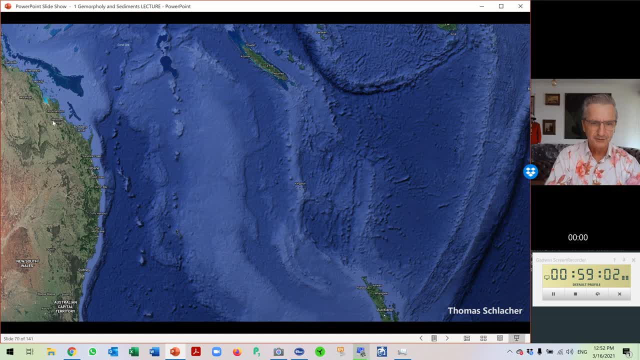 to the proper big brothers, because the proper big mountains, proper big mountains, proper big mountains, uh in southeast queensland, uh in southeast queensland, uh in southeast queensland- are sitting off the coast, so look at. are sitting off the coast, so look at. are sitting off the coast, so look at this beautiful chain. 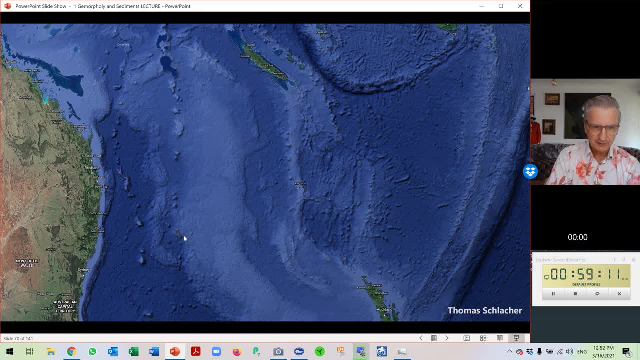 this beautiful chain, this beautiful chain of mountains, of mountains, of mountains. we've got another one coming down here. we've got another one coming down here. we've got another one coming down here. this is lord howe island, there's a lord. this is lord howe island. there's a lord. 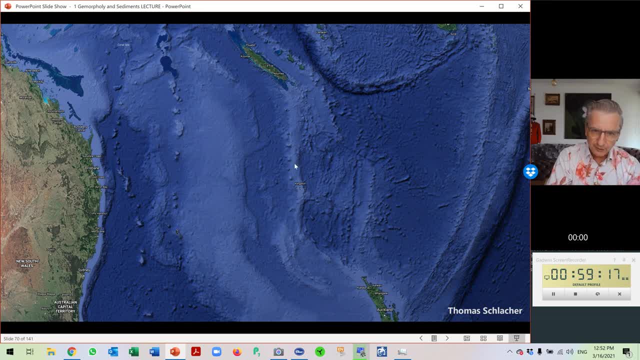 this is lord howe island. there's a lord howe ridge, chesterfield plateau. howe ridge, chesterfield plateau. howe ridge, chesterfield plateau, new caledonia. another which was lots of new caledonia, another which was lots of new caledonia, another which was lots of seamounts up here. 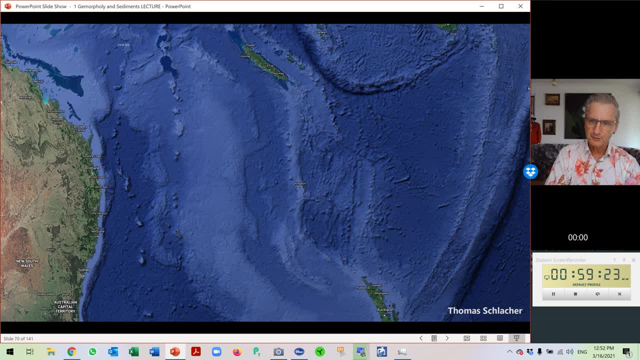 seamounts up here, seamounts up here, and it basically kicked off my and it basically kicked off my and it basically kicked off my deep sea work. i'm eternally grateful. deep sea work. i'm eternally grateful, deep sea work. i'm eternally grateful, grateful to my french collaborators and 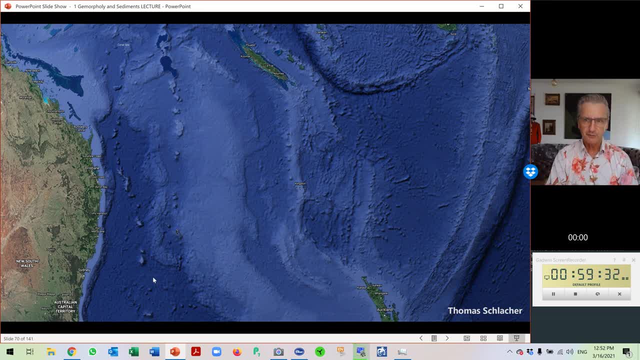 grateful to my french collaborators, and grateful to my french collaborators, and and france, and this is the north bit of and france, and this is the north bit of and france, and this is the north bit of new zealand, so basically our neighborhood, new zealand. so basically our neighborhood. 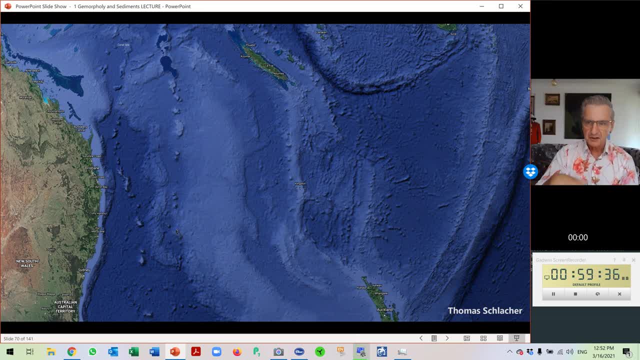 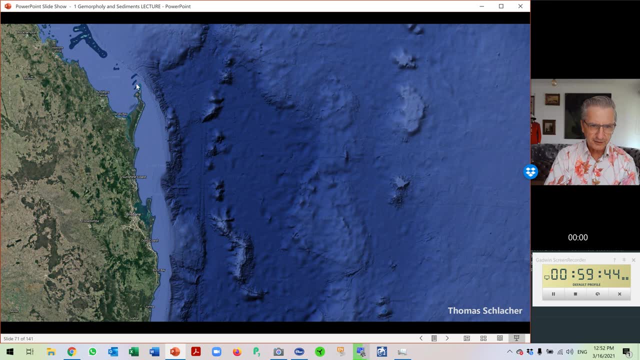 new zealand. so basically, our neighborhood has, has has, glasshouse mountains. if you want which glasshouse mountains, if you want which glasshouse mountains, if you want which? of kogari, you know harvey bay here. of kogari, you know harvey bay here. 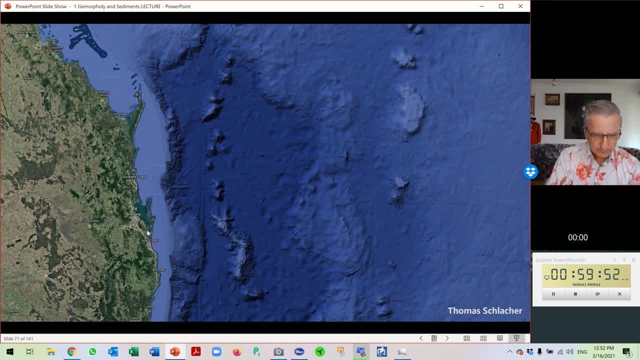 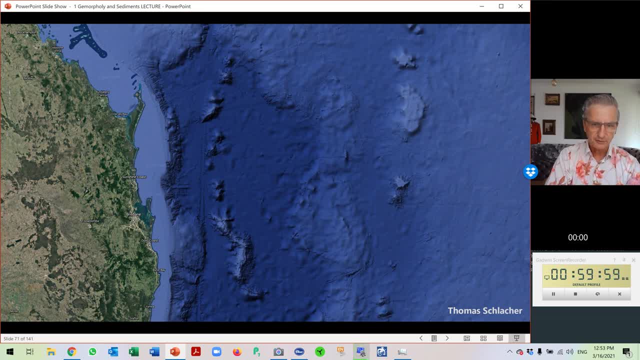 oh yeah, i heard about it. the gold coast. oh yeah, i heard about it. the gold coast. isn't that? the? isn't that the? isn't that the sunny place for shady people? something like sunny place for shady people? something like sunny place for shady people, something like that? 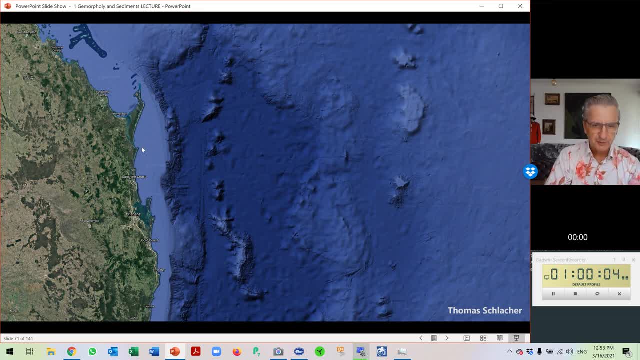 that that nevermind. oh, there's a small little nevermind. oh, there's a small little nevermind. oh, there's a small little village called brisbane, but this is village called brisbane, but this is village called brisbane. but this is basically our apache. now, right, and you. 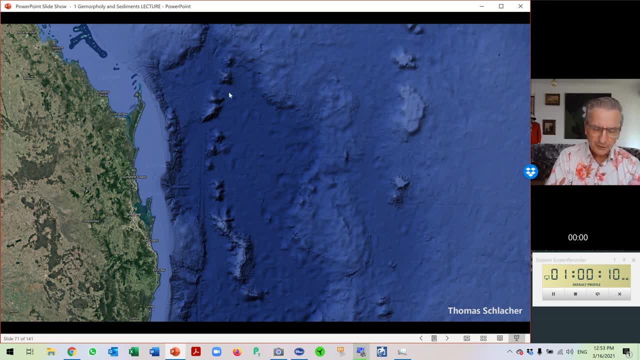 basically our apache now right, and you basically our apache now right. and you go straight out here you go about 200, go straight out. here you go about 200, go straight out here you go about 200 kilometers out and get this wonderful kilometers out and get this wonderful. 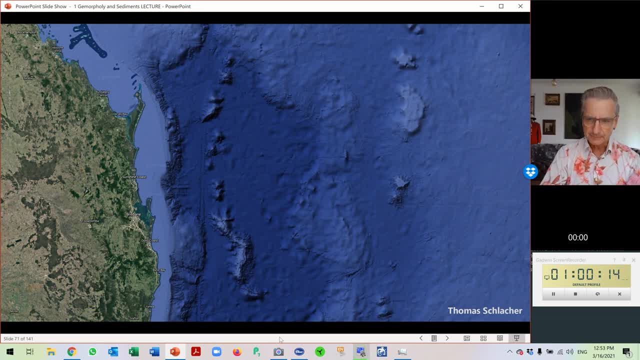 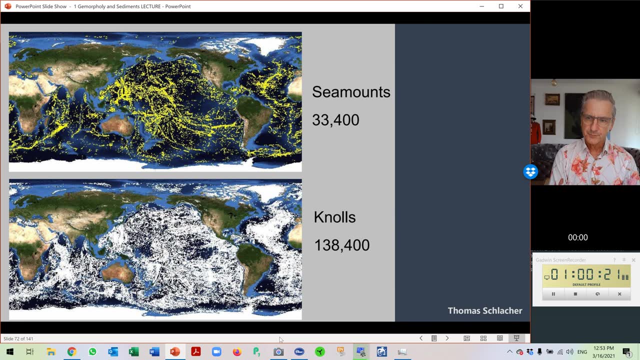 kilometers out and get this wonderful, wonderful mountain range. you know wonderful mountain range, you know wonderful mountain range. you know, in the deep sea, in the deep sea, in the deep sea now, more generally speaking, we've got now, more generally speaking. we've got now, more generally speaking, we've got a lot of seamounts and we have made this. 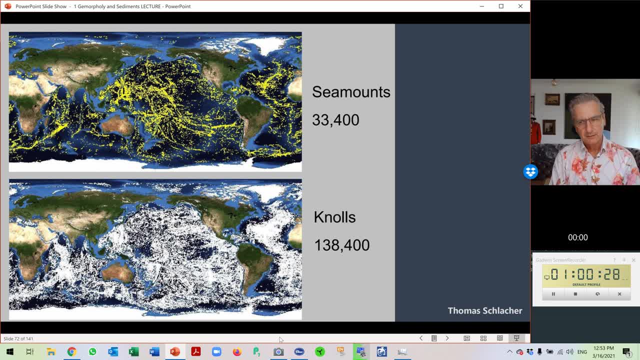 a lot of seamounts and we have made this a lot of seamounts and we have made this map. i'm a co-host of that about 10 years map. i'm a co-host of that about 10 years map. i'm a co-host of that about 10 years ago. 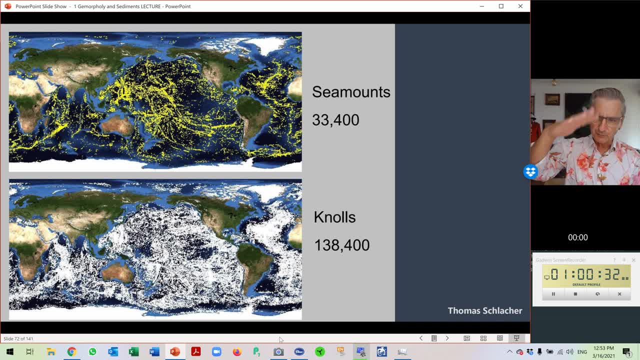 ago ago. it's very hard to actually do. because it's very hard to actually do, because it's very hard to actually do because you have to actually measure, you have to actually measure, you have to actually measure. slight tips, uh, in the sea level result. slight tips, uh, in the sea level result. 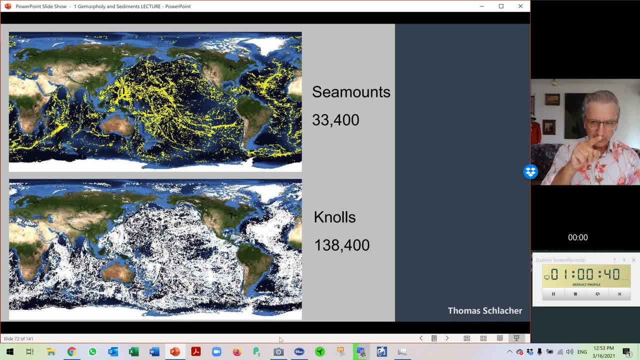 slight tips, uh, in the sea level, result with satellites. because if there is a with satellites, because if there is a with satellites, because if there is a seamount underneath seamount, underneath seamount, underneath undersea mountain, it actually drags the undersea mountain, it actually drags the 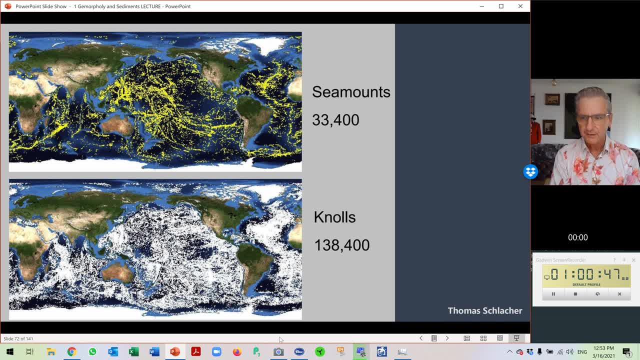 undersea mountain. it actually drags the surface down and you can actually work surface down and you can actually work surface down and you can actually work that out and from that you can work out that out, and from that you can work out that out, and from that you can work out how big the mountain is, and so forth. 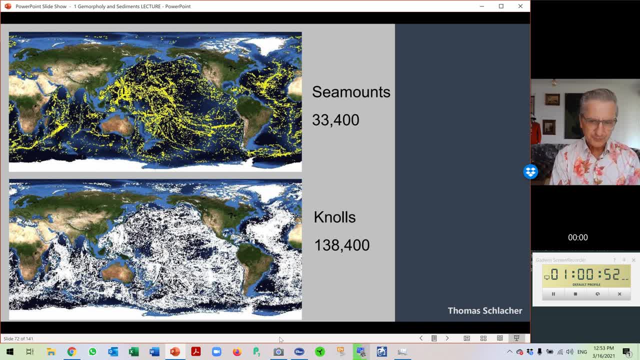 how big the mountain is and so forth. how big the mountain is, and so forth, uh, if there are thirty thousand or a? uh, if there are thirty thousand or a. uh, if there are thirty thousand or a hundred thousand, hundred thousand, hundred thousand, we don't, you know, you can actually. 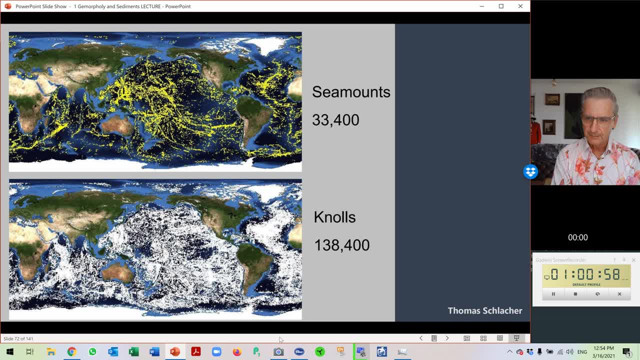 we don't you know you can actually. we don't you know you can actually. that's. that's partly a question of that's. that's partly a question of that's. that's partly a question of definition as well. definition as well, definition as well. the take home message is: whatever the 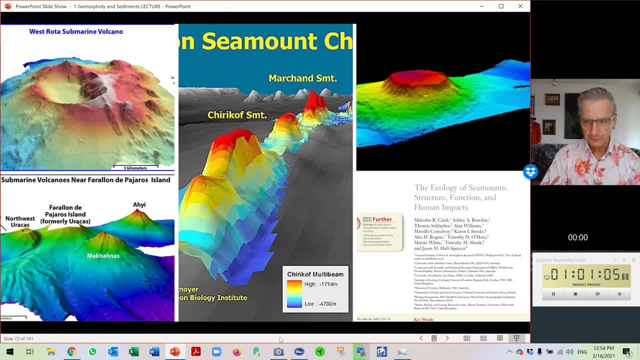 the take home message is: whatever the the take home message is, whatever the correct figure is there is correct figure is there is correct figure is there is a lot like a lot, a lot, a lot. and this is what they look like. i've always quite, you know, enjoy going to see and, you know, as you actually go over new terrain, you know. 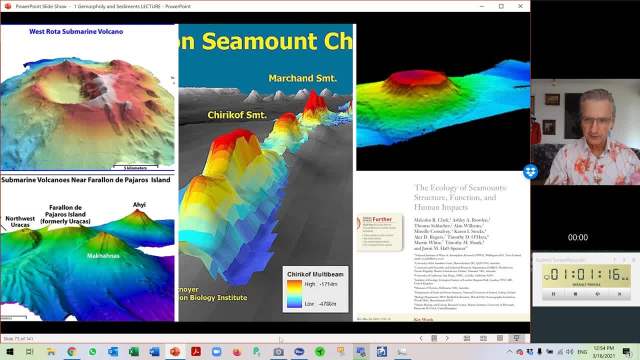 you make always new discovery. nobody usually has to be in there and you get actually the multi-beam uh sonars are very sophisticated nowadays and you go to specialized train operator doing that and here you actually have one. you know, it's a caldera in the middle here. 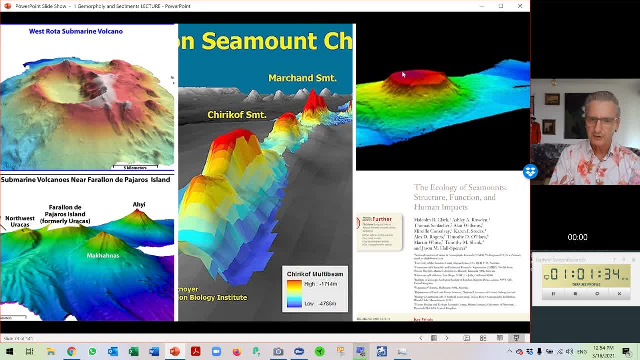 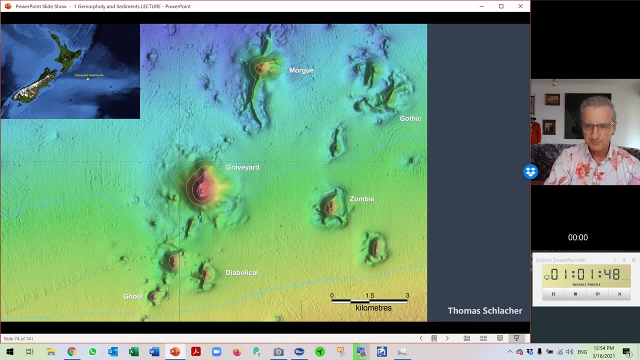 you have the ones of uh, basically russia. here is a guillot which is perfectly flat at the top because it used to actually stick out. then it sank again and the waves flattened the top off. the new zealanders have a very interesting uh way of naming some of the sealant features. uh. 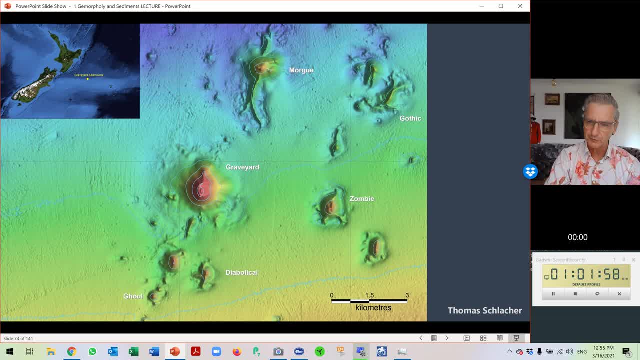 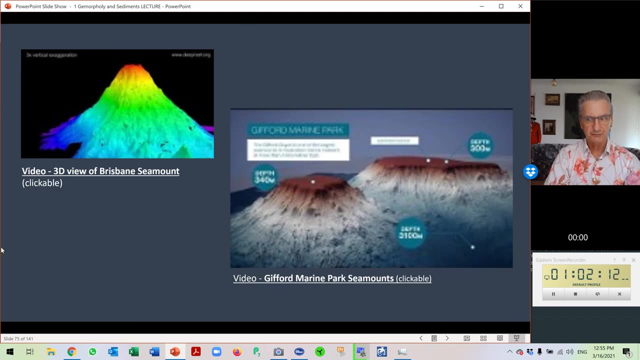 seamount features. i'm not quite sure what actually happened on that particular cruise. we've got seamount morgue, gothic, zombie, graveyard, diabolity and ghoul. would have been really fun to go on that ship, but never mind. um, we basically, you know, are not very original, although we have actually named a few. 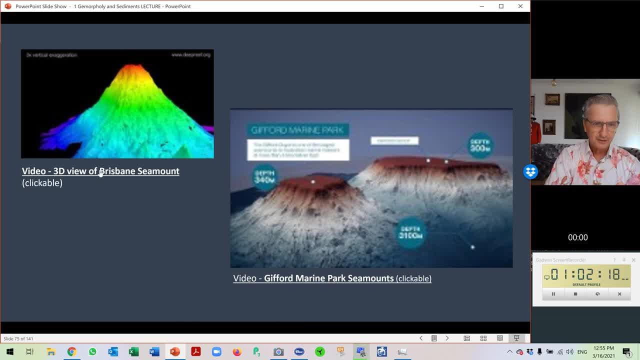 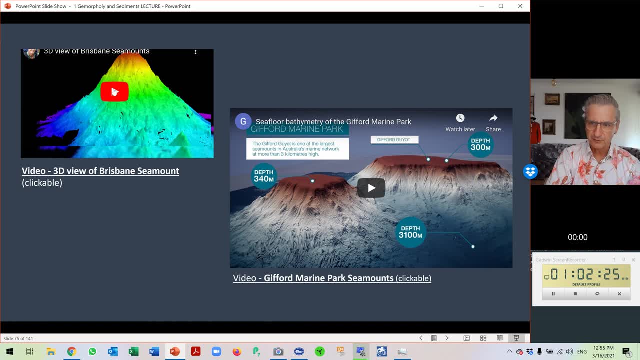 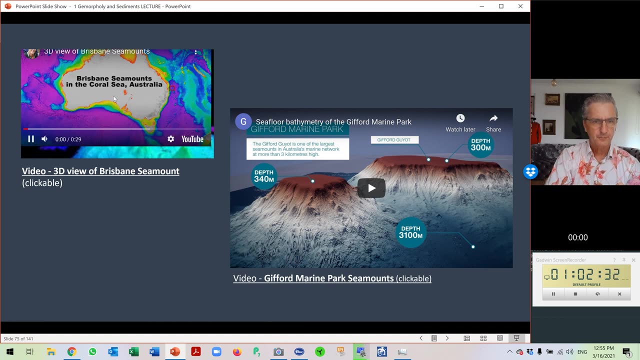 uh during this mania called the sisters and therefores i just show you two you know animations uh. the one uh of brisbane seamount, which is literally the closest one to the coast here and i really enjoy it might be even more immersive, very charming. see, here you can have uh. 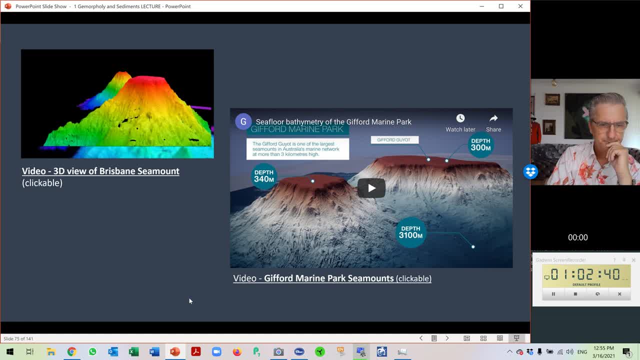 sort of- uh, the bluest kind ofhanas that we have for you, though, and that's features we can give you here, and that's the uranium and those features about 1000 to 2000 meters high we have my months now numerous times. you can't basically miss them, and next time you go around the glassh Lemon mountains, did you climb one of them and you ovIfthw east. this is how you see those features about 1000 to 2000 meters high. we have the mega beamed numerous times. you can basically miss them, and the next time you go around the glasshouse mountains, did you climb one of them? if you look to east, this is what you see- your Marvellous iris oil heats gigs- and you look too east, you see its here. 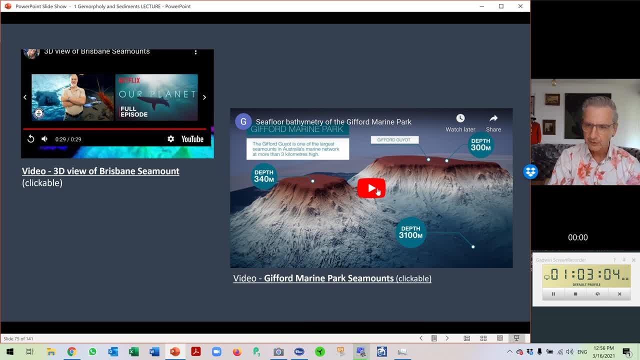 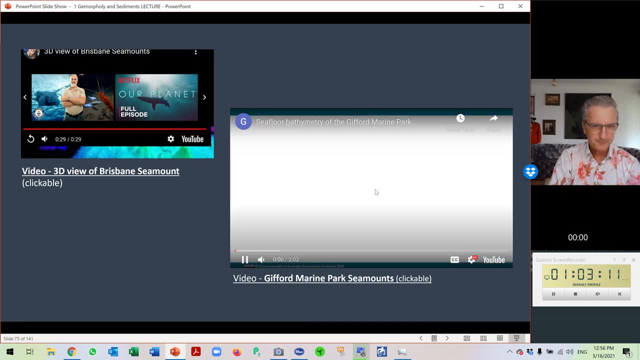 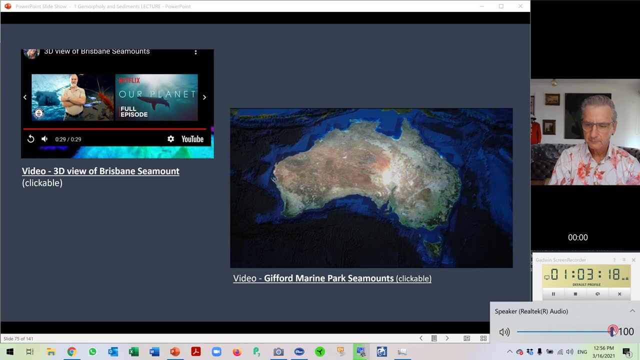 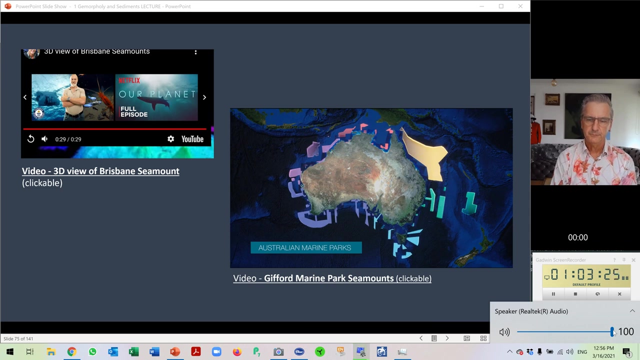 are two goyos in the Gifford Marine Park and the narration is a bit odd, but never mind does it come up. Australia is surrounded by a magnificent marine environment. our network of marine parks protect and conserve some of the most incredible seascapes and sea life. 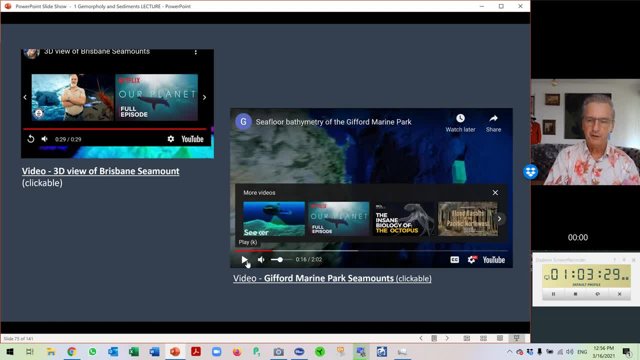 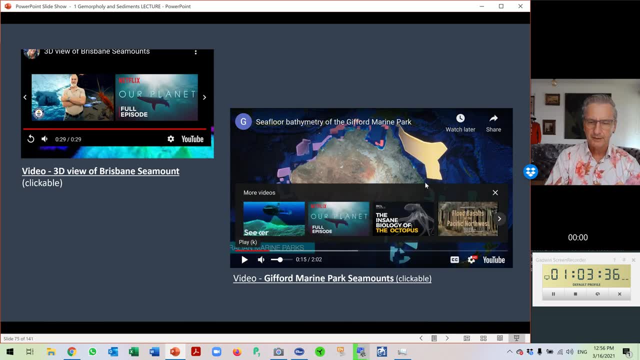 in the world? Gifford Marine Park. okay, have you actually i? i i just need to tell you that you know this is the official government line. sea life in the world. oh, look at this thing. uh, have you actually noticed that our marine parks the federal ones? 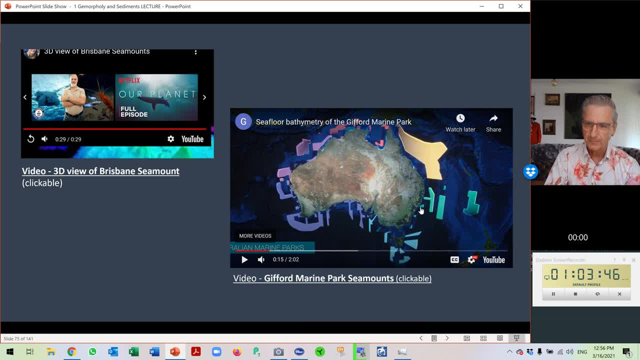 rarely come to shore. they all actually stop, um, conveniently, you know, a few kilometers offshore and they are literally in bits and pieces, uh, of the ocean, which is actually probably not as strongly stressed by human activities as it would be closer, i'm sure. yeah, lots of scientists have actually expressed their, their concern about. 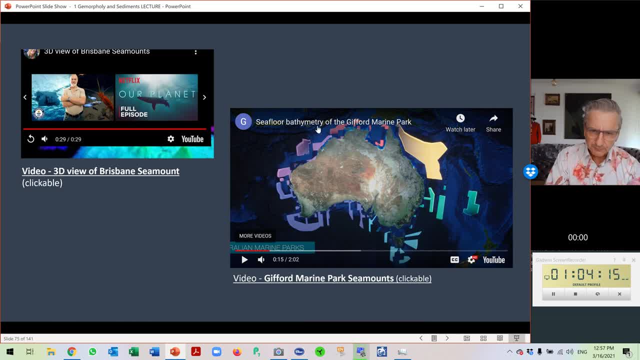 that odd placement. and also isn't it odd that what are we doing up there? the oil and gas industry, interesting. and what are we doing down here? fishing rights, in any case, we talk about that, uh, as in week 10 by 11.. just Gifford Marine Park, situated within 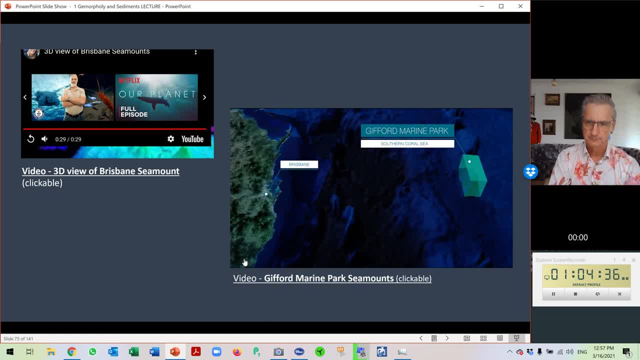 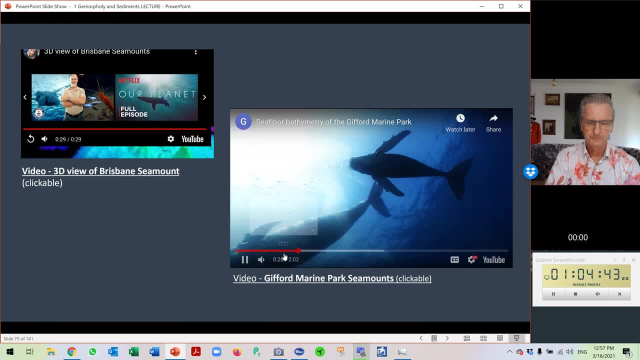 the southern coral sea is part of Australia's temperate east network of marine parks. 600 kilometers off Australia's east coast, the region is home to a number of protected whale species, including the humpback blue and sperm whales, as well as a number of migratory seabirds. 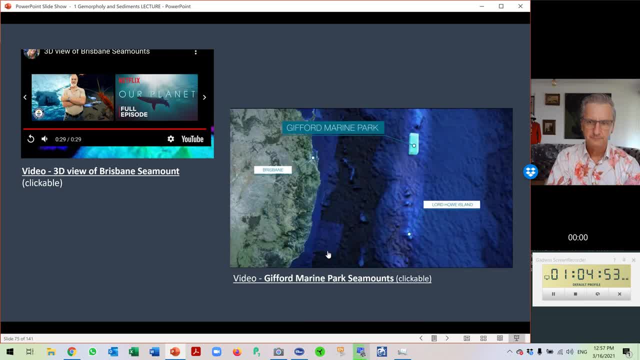 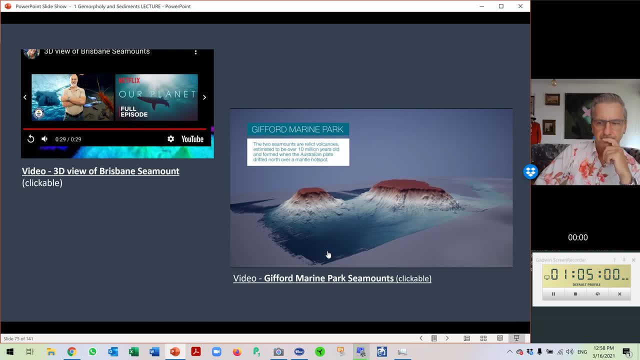 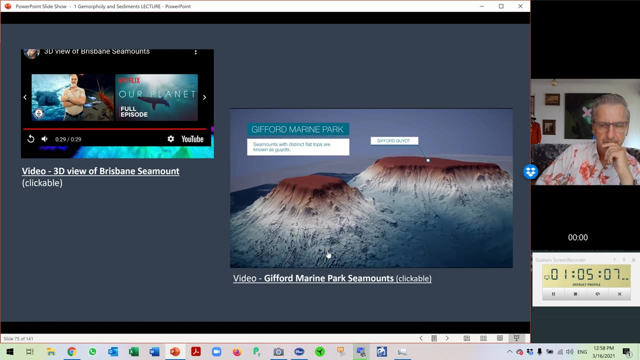 part of the Lord Howe seamount chain. Gifford's two seamounts are relative volcanoes estimated to be over 10 million years old and formed when the Australian plate drifted north over a mantle hotspot. Lord Howe island is also part of the seamount chain seamounts with distinct flat tops. 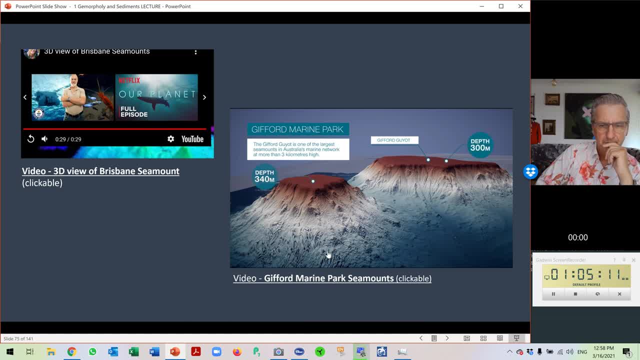 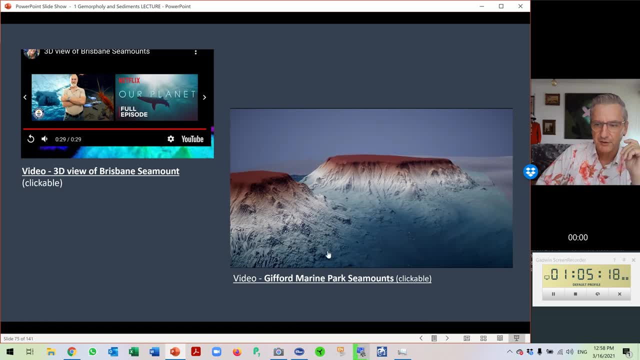 are known as Geo's. the Gifford Geo is among the largest seamounts in Australia's marine network at more than three- so we're talking about, you know- 2600 meters high, much higher than anything else we have online, with broad channels and smaller volcanoes. 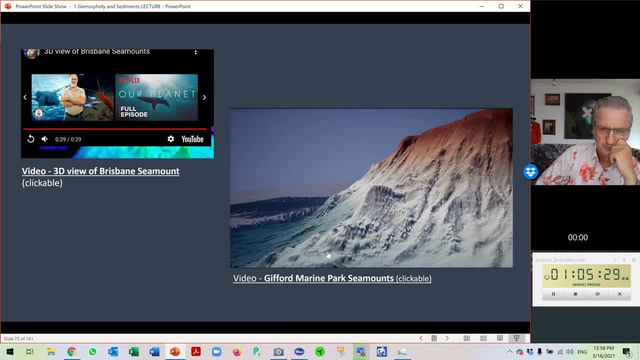 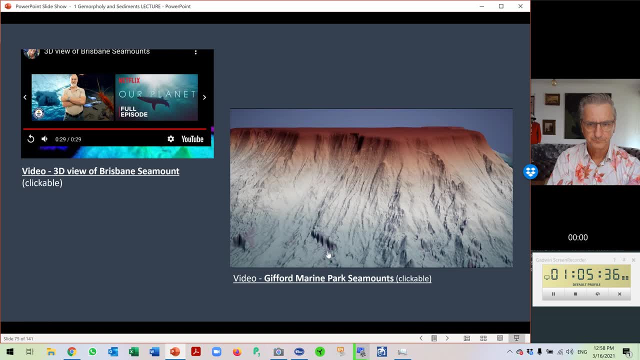 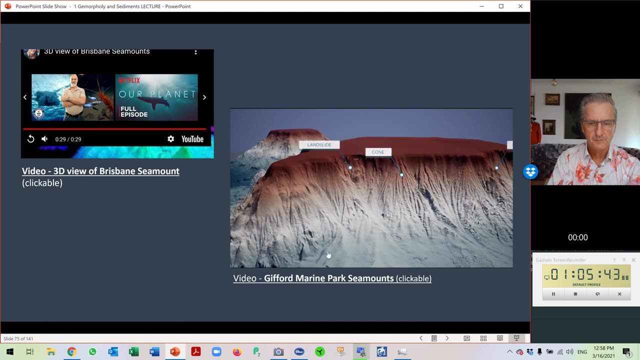 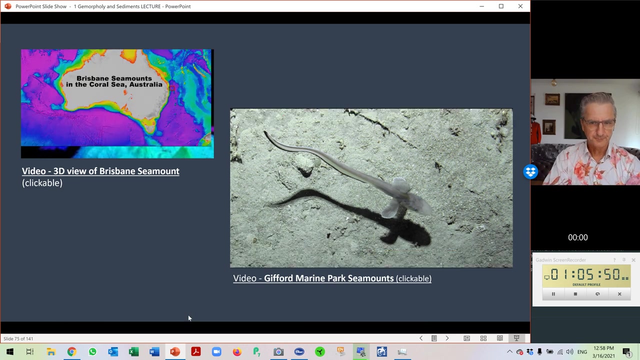 both seamounts display evidence of significant landslide activity, with a number of blocks and cones related to this activity surrounding their bases. the temperate east marine region is an area of national significance for a range of marine species. all right, I think you get that. yeah, so I can actually upload those and upload them to the. 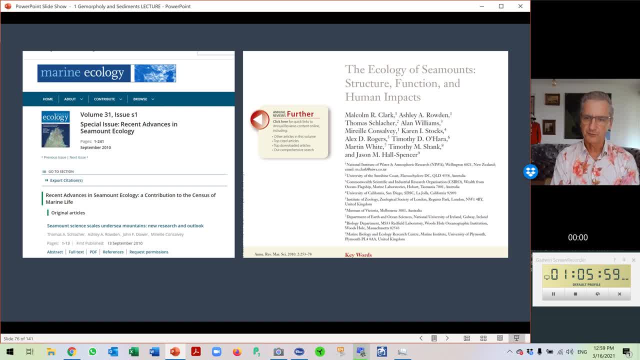 but essentially, those seamounts are extreme topographic features, so to speak, in terms of ruggedness, in terms of, you know, constituting true mountain ranges under the sea, and also because they're often islands of hard substrate, of rocky terrain and not, you know, mud as is most. 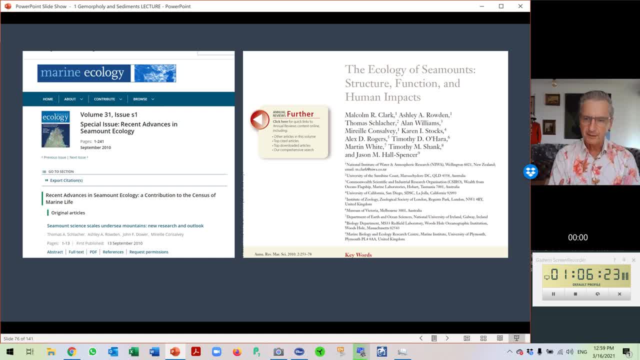 of the seafloor they actually stick from. they are literally islands of coral rain- in order to have these deep reefs in the deep sea- and much of our work has gone on sort of protecting those- you know deep reefs and also understanding how vulnerable they are to certain. 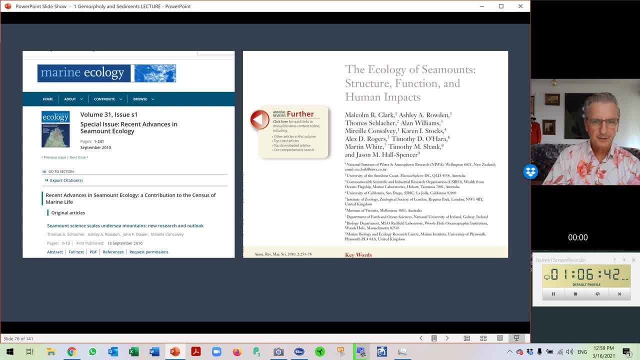 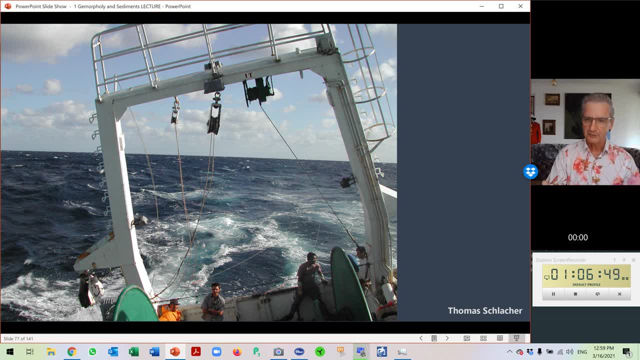 impacts, and that is something i'm going to tell you more about it. right, and you know? that concludes our lecture about the ABC of undersea inner topographic batimetric features and how the ocean basins were created, which is, you know, said about the deep sea. 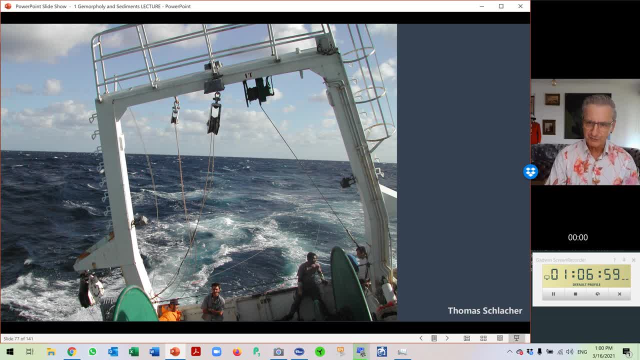 the most fundamental aspect of understanding oceanography. and you might also say, look, you know, this is all very remote and it's all deep ocean science and i'm on land. you know, i would actually say nothing. actually, really, if you really set your mind on it will actually prevent you from not.